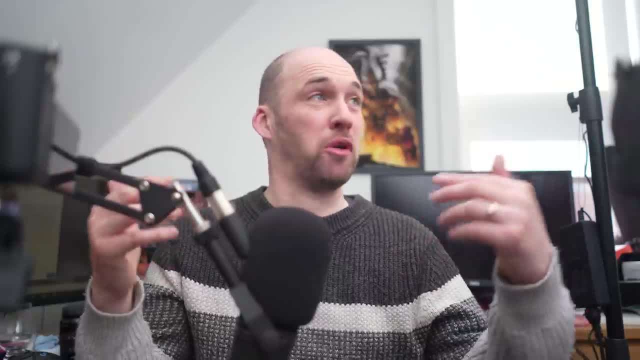 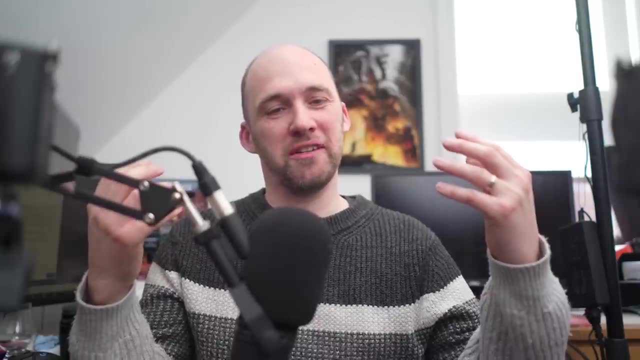 guys. You sent us some stuff. I've been painting some of the stuff. Still want more to paint. They are very, very nice. It's for me, it's like it's such a cool system and such a cool background. 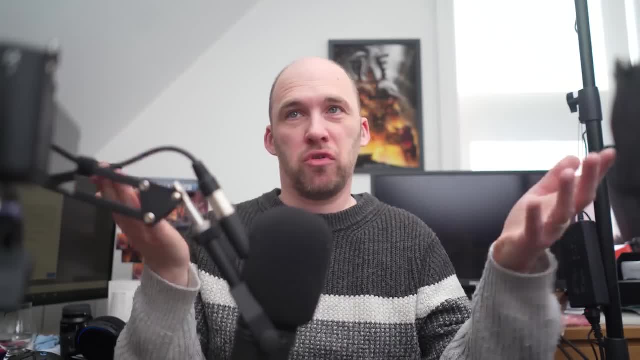 that you've made. We've invited you on one to talk about yourself, but also to talk about this product that you've made. So War on Terror. where did it come from? One day? you're just sitting there and just went. 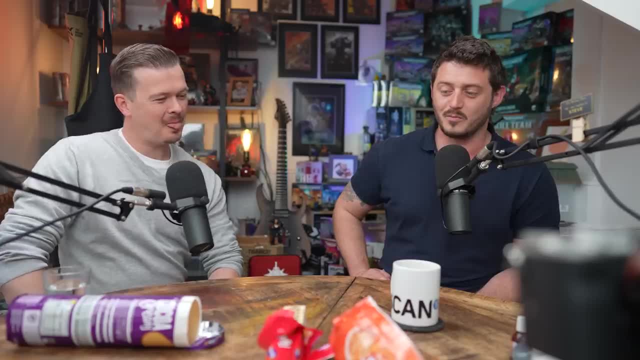 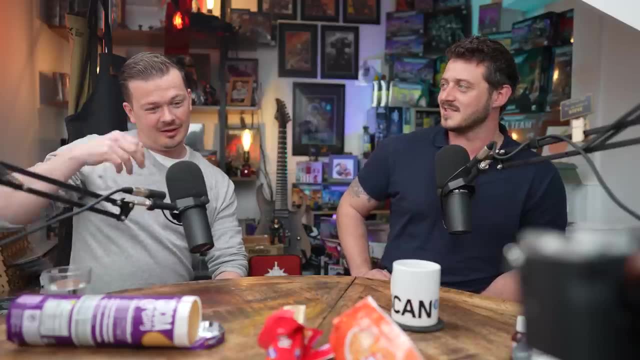 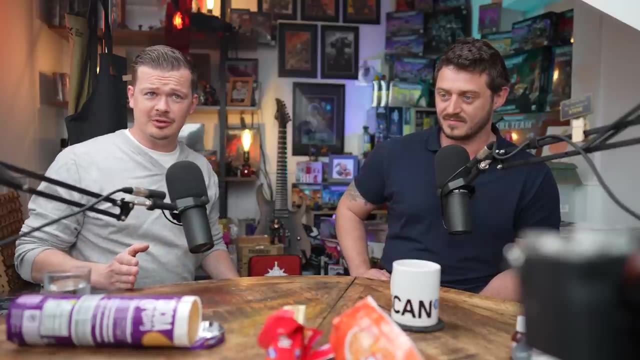 Let's make it. let's make a board game or war game, Pretty much. Well, I think I'll pass it over to you to explain the name and maybe that. but we met in weird circumstances. That's Yeah, I mean, how the game came about. I suppose is all throughout my childhood I made attempts to 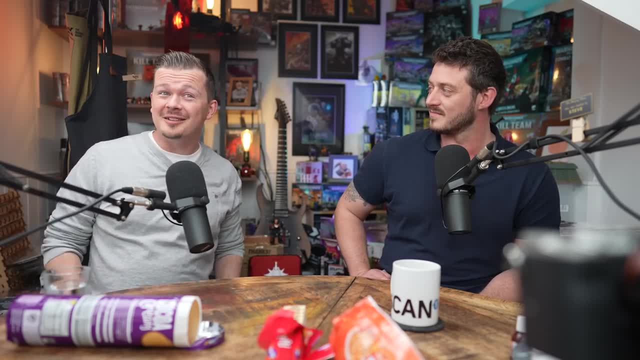 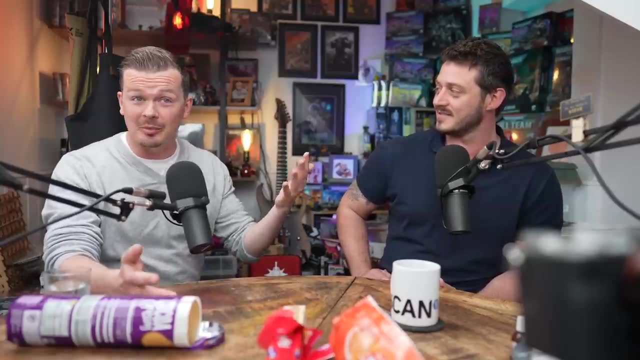 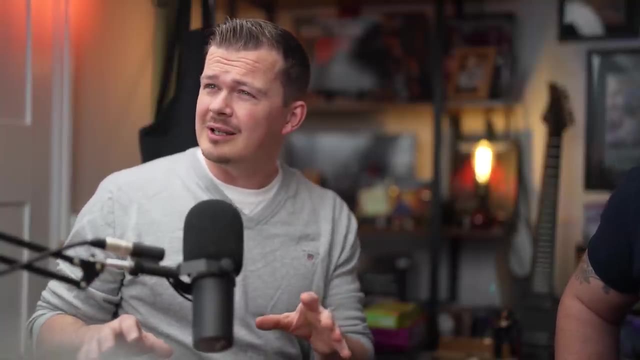 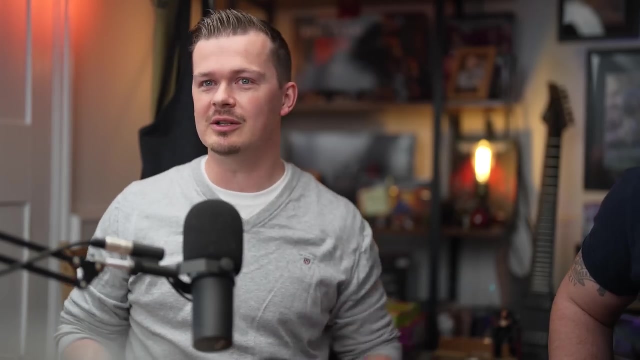 get into certain familiar game. you know game systems And what I tended to find, to be honest, was that you obviously you walk into- it was obviously Warhammer. You walk into a games workshop and they try and explain it to you- And it was probably just down to me mainly- but a lot of it I didn't understand or didn't make sense. A lot of the rules seemed a bit convoluted and so on. But I keep trying And I tried. every few years I've got boxes of unpainted Necrons and Tau. 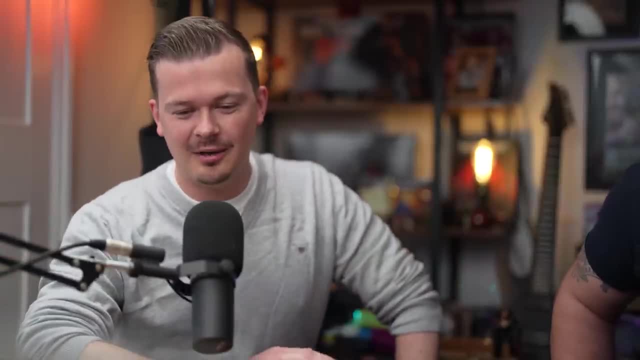 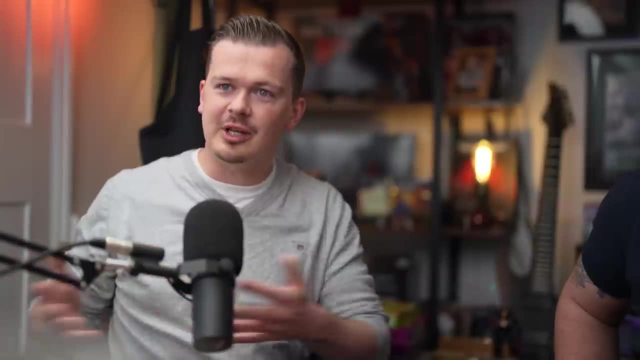 Who doesn't? I just yeah as standard And I always just thought: why not attempt to make one? Yeah, You know, you've just got to come up with a rule set. I say, you just have to Yeah. 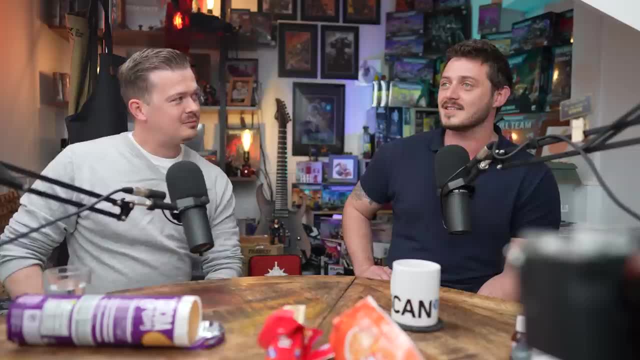 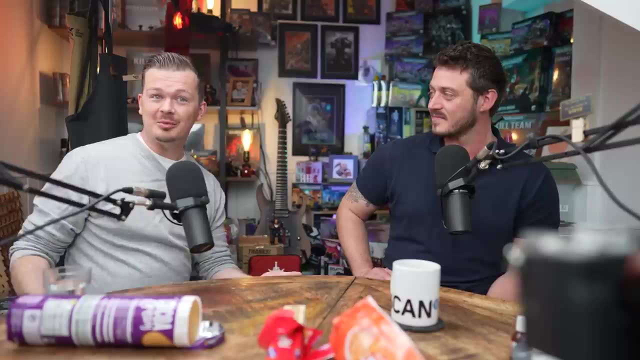 It's easier. Yeah, Yeah, let's go with the yes, Yeah And around the name as well. you mentioned around the time I was thinking that unfortunate events happened in America, Of course, And then then so there started the war on terror. 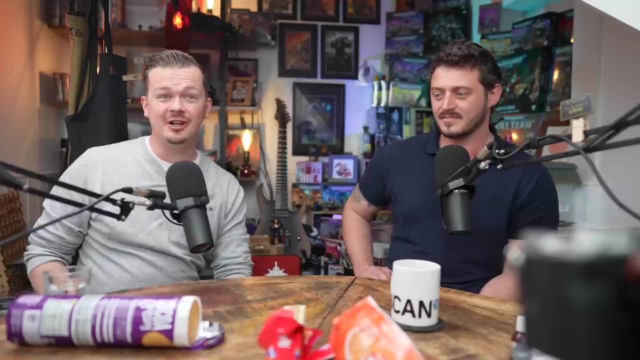 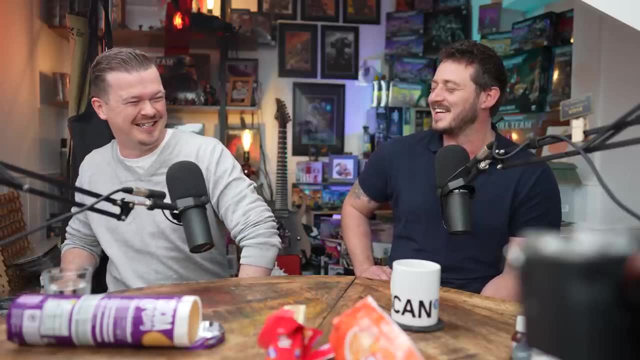 Yeah, yeah, yeah, And it just stepped onto changing it to TER And it's so, it's, it's a pun, but not Yeah, Suddenly think, oh, we're making light of a horrendous tragedy. Yeah, But also, I mean, that's the name of the earth, It's Latin right, Terror. 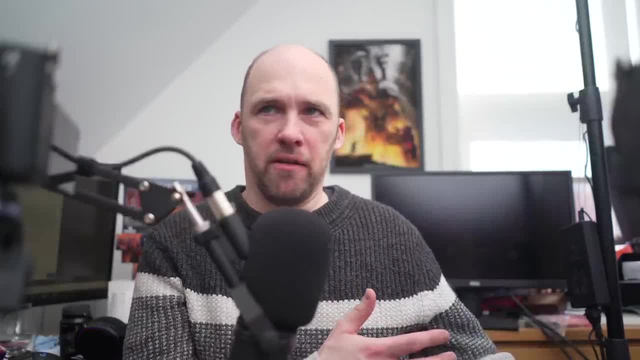 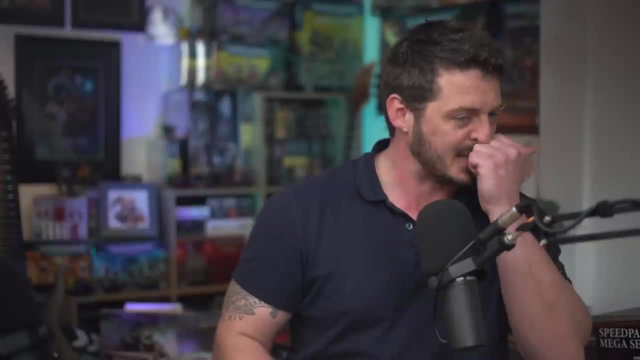 Yeah, So it makes sense. And obviously some people would say, well, that's the name of the planet, of the earth in 40K now, No, it's just, Whereas in in War on Terror we we're still calling it Earth. We've changed a couple of celestial body names, but there was no reason to change the name of Earth. Yeah, Earth still made sense. We changed the Moon to Luna again Because obviously our universe is expensive and if you're on another planet with another moon, yeah, It made sense. Yeah, no longer same as the sun is. no longer the name of the body, yeah, but more a colloquial name for. 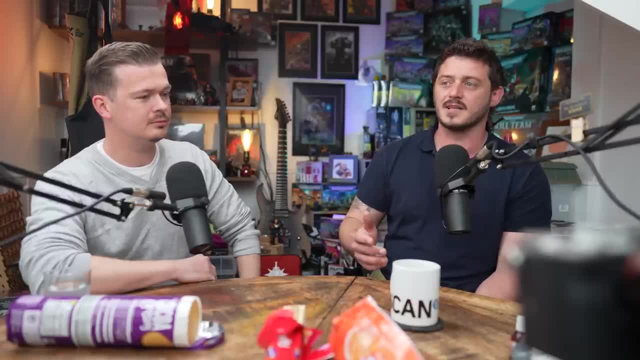 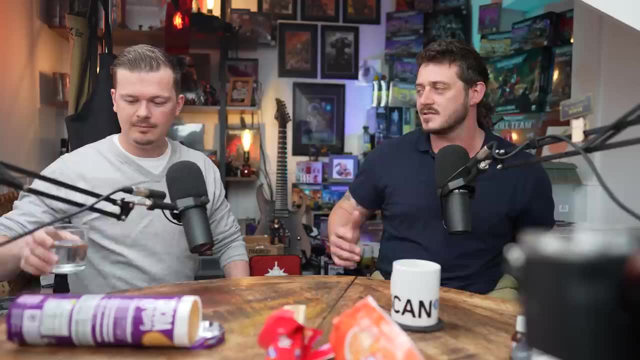 the body of the planet you're on. yeah, so it's more of a nickname. it's like, instead of: yeah, you stand on a random planet, oh, solaris is rising. no, it's the sun. yeah, yeah, it doesn't matter if it's not the sun anymore, but yeah, so that's a little bit of lore. so, with um, when you decided, hey, we're. 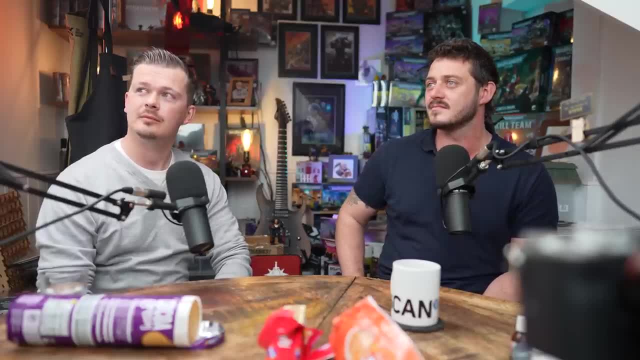 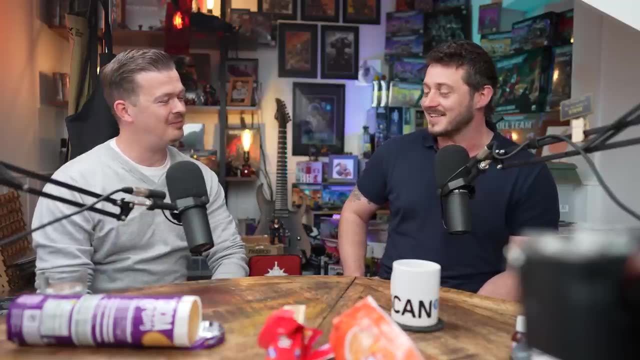 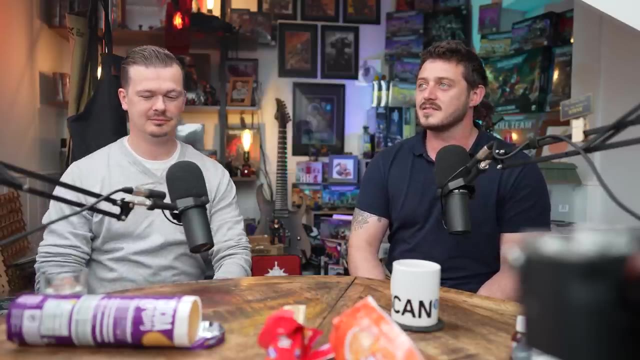 going to make our own game like: was it law first? was it miniatures first? did you have ideas initially about how it would all go? where to start? because you know, the reason why it's hard to start is because, yes to all of the above. uh, we're both massive sci-fi fans. uh, we love things. 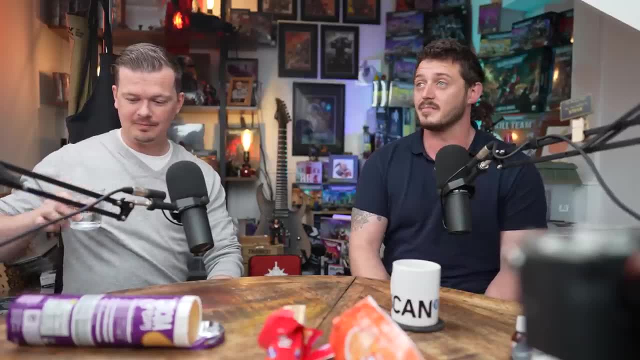 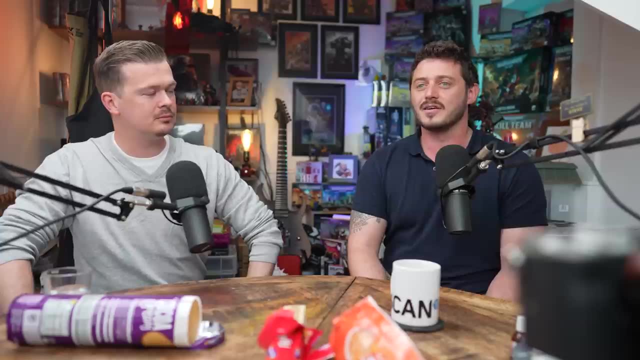 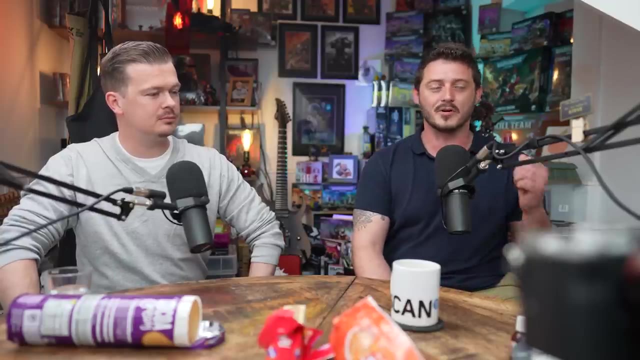 like independence day, yeah, just like loads of all of the above, all like massive sci-fi. so we love law and we're not these, we're not just these guys that watch the movie and are quite content with disappearing. um, we read, we dive, we quite like proper science, uh, science concepts and uh. so we knew we needed a good law base. 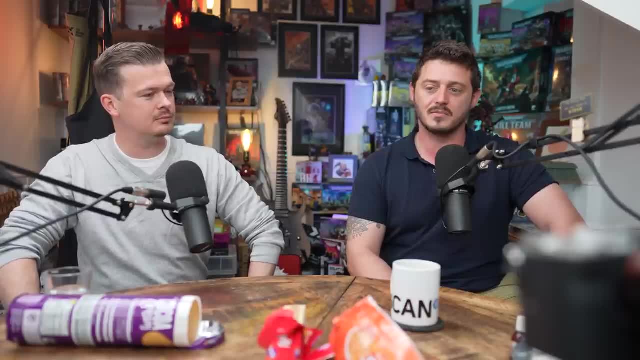 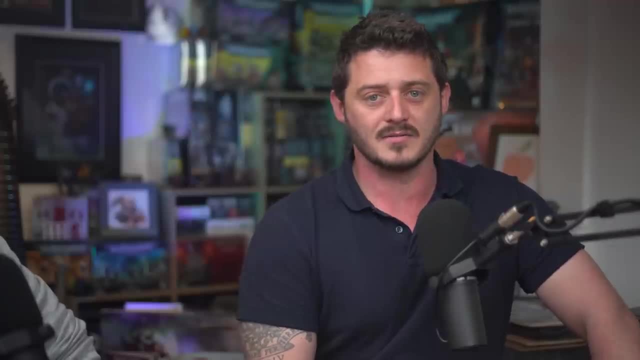 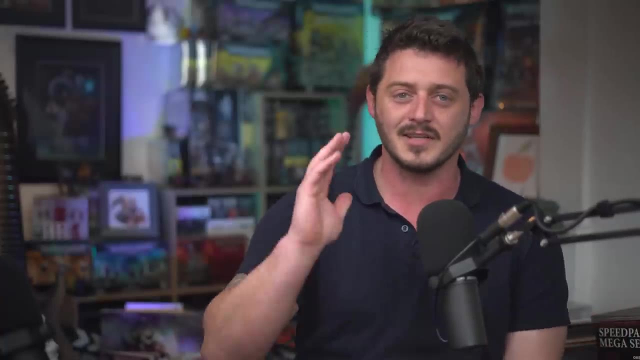 at the same time, that helped us come up with the ideas of certain races, uh, factions, models, i being military background always- and i think you mentioned it on a recent podcast. but it was like like when you watch movies and you you're counting the rounds, going through the through. 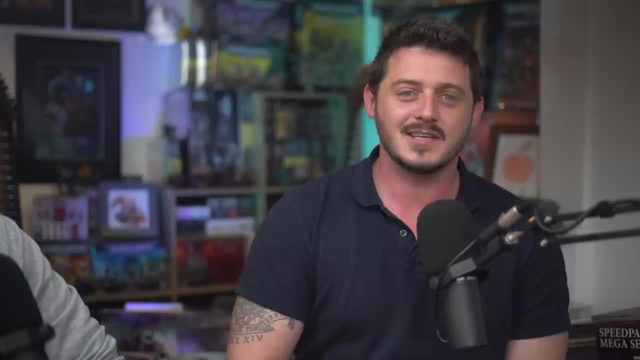 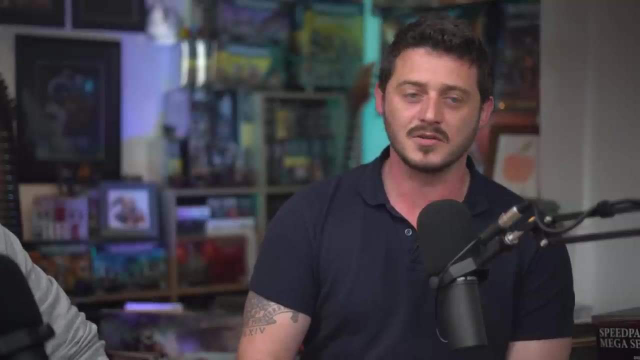 the weapon. yeah, like yeah, that mag only held nine rounds and i think he shot like 23. it's the old hollywood magazine. yeah, well, that wouldn't have exploded in that way. but i look at certain positions of models and i'm like that's not, that wouldn't be a comfortable firing position, kind of. 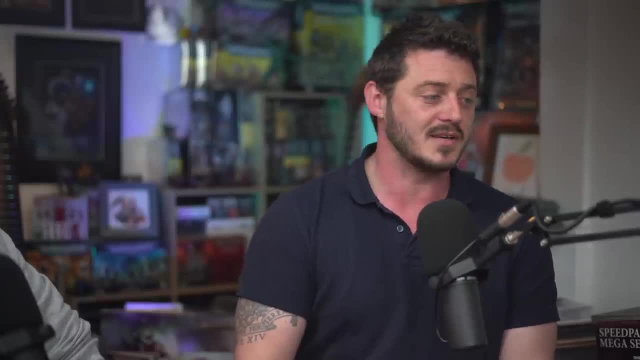 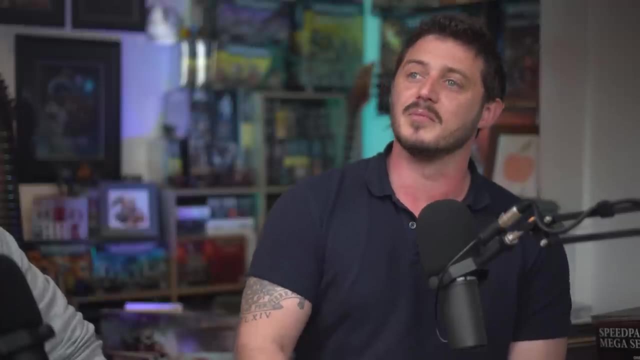 thing, or you wouldn't be able to fight in that armor. don't get me wrong. you wouldn't be able to fight in a lot of sci-fi armor- yeah, sometimes even ours- but we've done my. i've done our best, and uh, to try and make it that way. so that helped the models and the law all fit in as well, um, and. 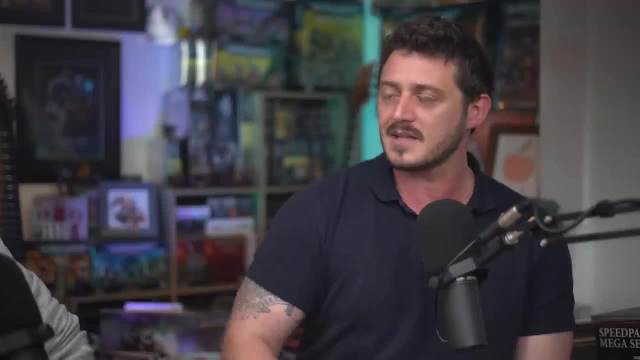 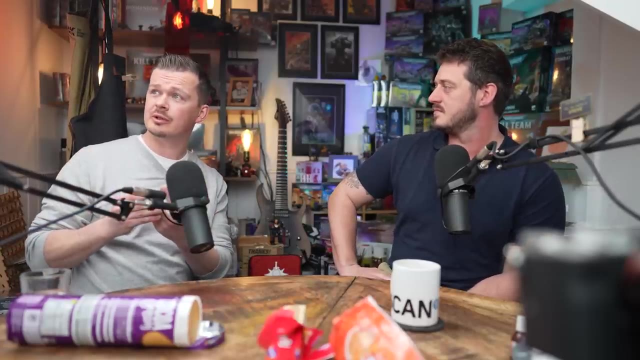 then the rules. all three came up at the same time. it's always been. that's that's why it's always been. if you look at successful tabletop games, it's always been like. that's why it's always been. there's like a trident: yeah, you've got- it's got to have great models. yeah, it's got a solid rule set. 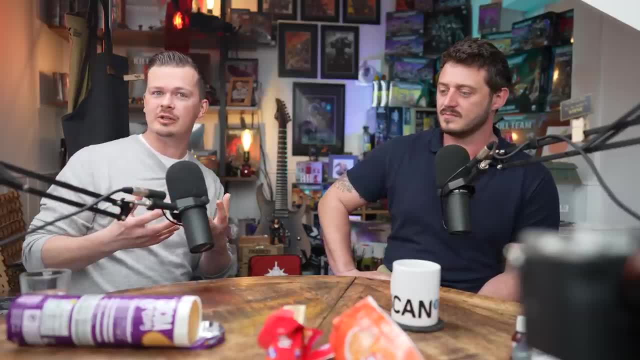 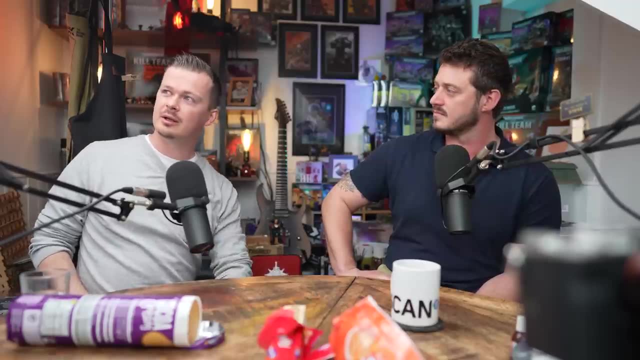 yeah, and then it's got to have a law, it's got to sit within the universe. yeah, there's obviously gonna be a lot of people that only are interested in one, maybe two of those yeah aspects. but i think if you, if you have all three, um, it just works. and then obviously, i think uniquely to us, we 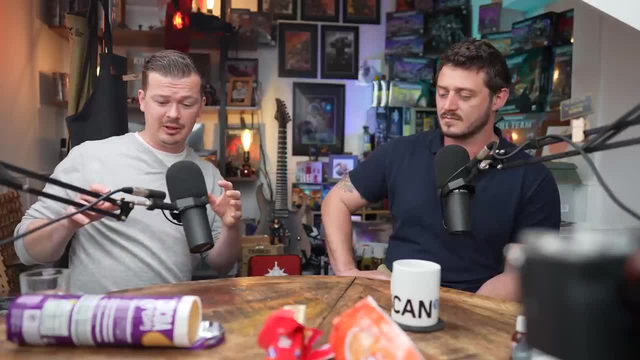 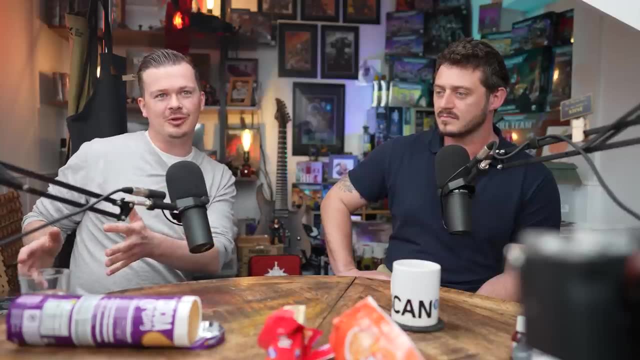 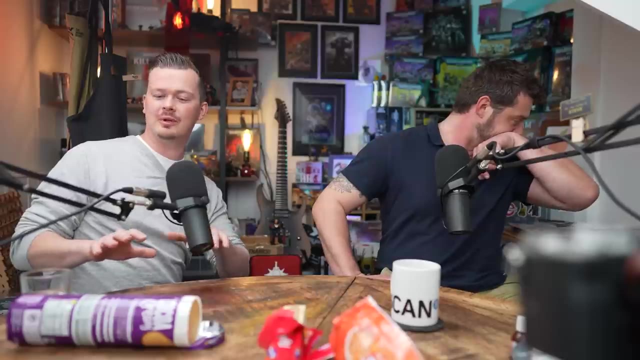 all three grew at the same time. yeah, so anything that our models have become and things that they don't so at the same time, we've gone. we've gone quite like a hard sci-fi. yeah, yeah, so everything has to be vaguely explainable. yeah, in in context. really remember when we were chatting at Chilcon. 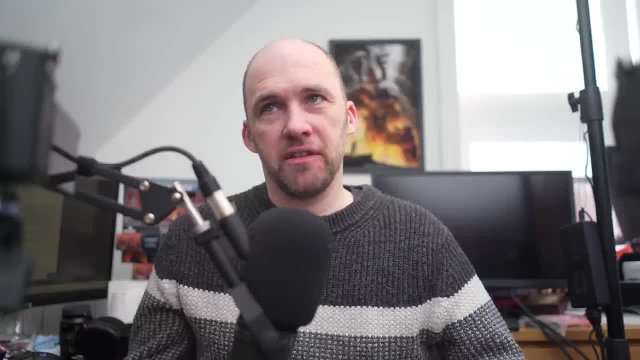 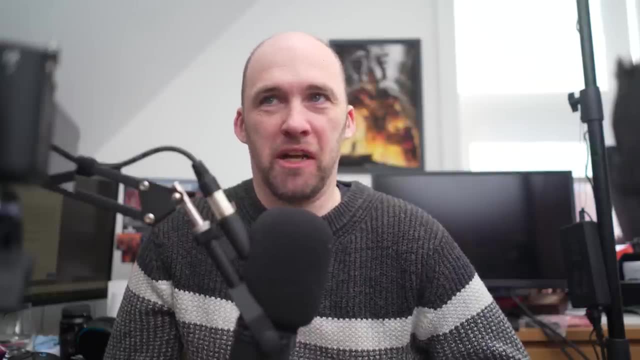 you talked about, like you want to introduce like as much realistic science into in, into the background as you can, without it being too like far-fetched. like you know, how do we fix this problem with Star Trek? oh, we'll just make up some. you know, let's fix the tri-axle in bandwidth to uh. 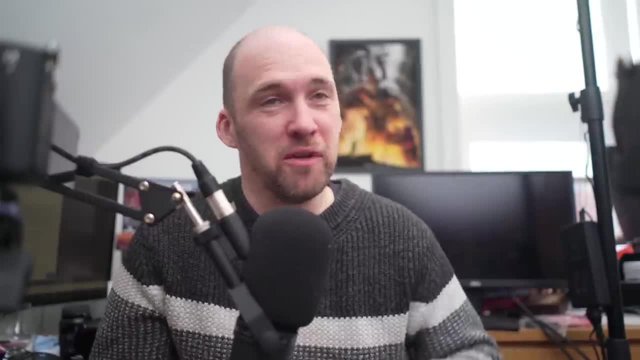 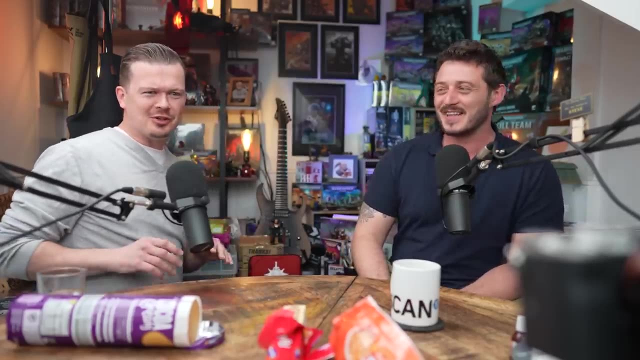 you know, reconvene the- uh, the two co-axles together and then yeah, well, it's all fine, we're sorted, it's all just happened. there's no, just there's no problems with Star Trek. oh no, don't get me wrong, I love Star Trek. so I mean with with war on terror, you've got the human factions and yes. 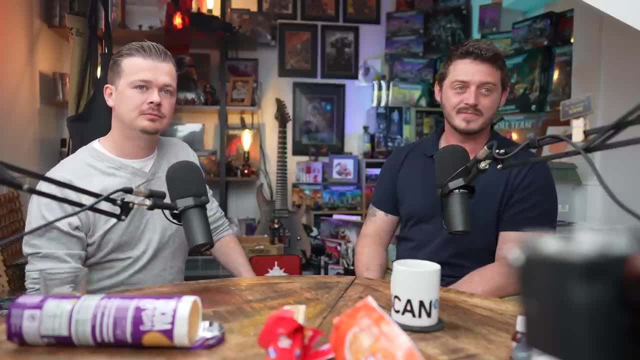 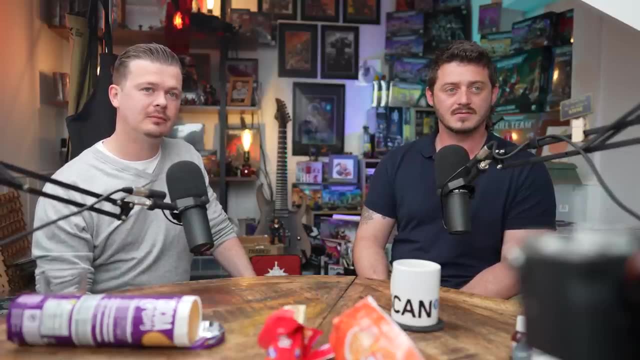 um, for my sins. I wanted to paint some stuff- I'll post up on Instagram, you've seen it- and I just want to stick some color on on those models. yeah, happy with that. for me, the the. there's two bonuses to these models. one- this: I don't want it to sound like a negative. they're not overly detailed, which 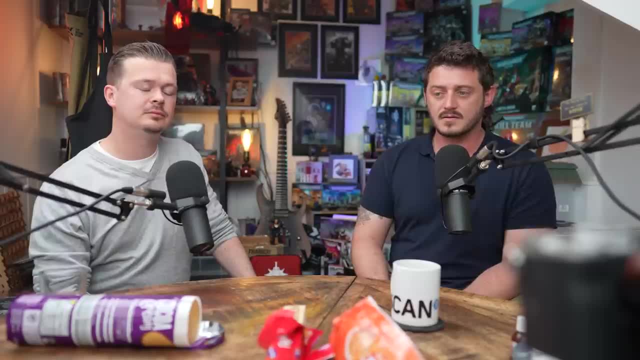 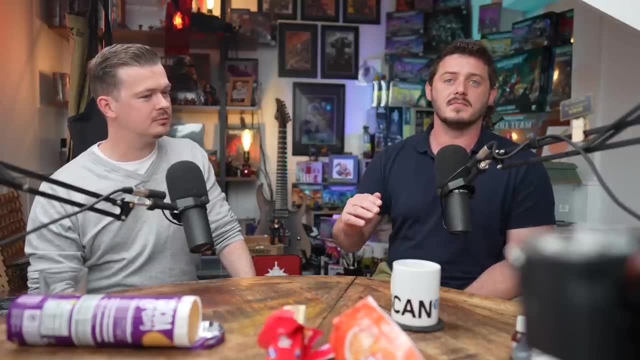 for me is a good thing because I can add: well, that's detail, that's a little bit so just to jump in there, that is, I felt like a lot of certain games, especially with the, obviously with the real um popularity of 3D printers, now being able to just 3D print. 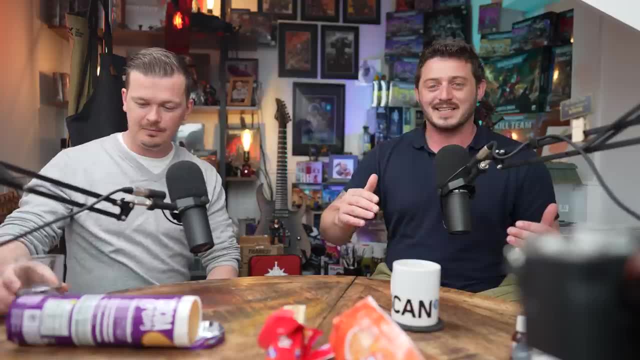 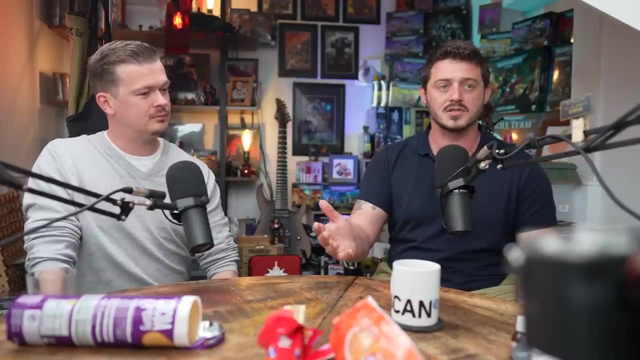 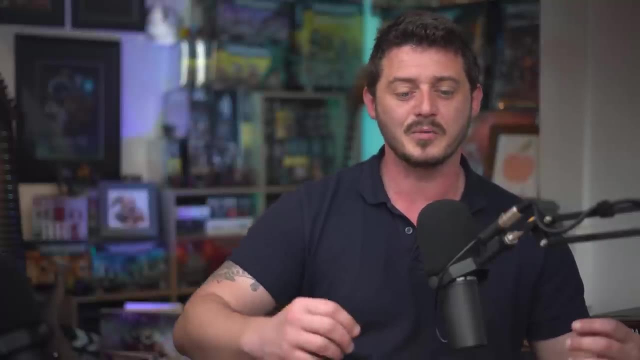 beautiful detail. it's very easy, like: well, see, I was saying less is more, yeah, yeah, more is less. and some models- um, not just GWs, but others- they're gorgeous, but when you got like an army game and a load of models, I want to be able to add detail- that I want, and to add individuality rather than. 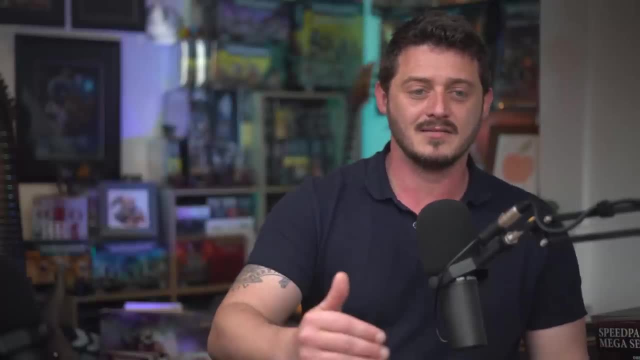 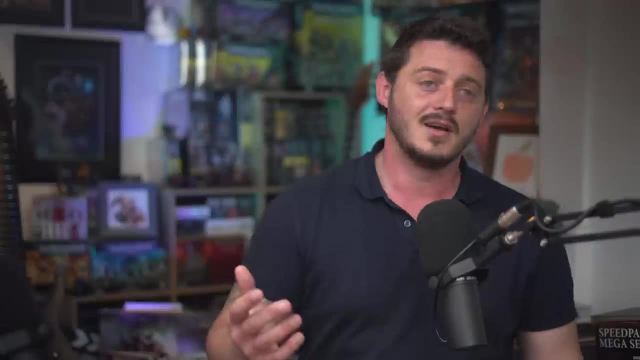 have to sculpt it away. yeah, yeah, and it's like I want to add this as a character because I've given him that little bit of detail and that's kind of why we wanted a little bit of a um again. it's going to sound a bit of a neg, but a bland model. I wouldn't say it's bland, I'll say you've. 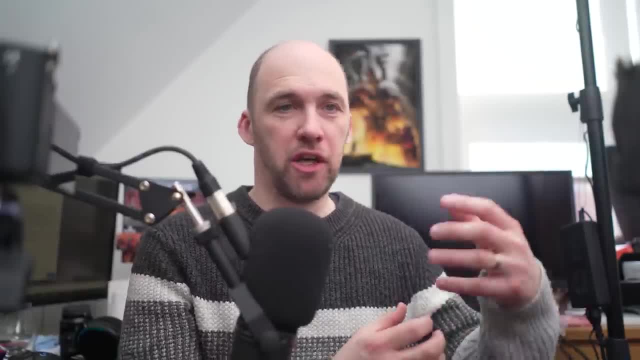 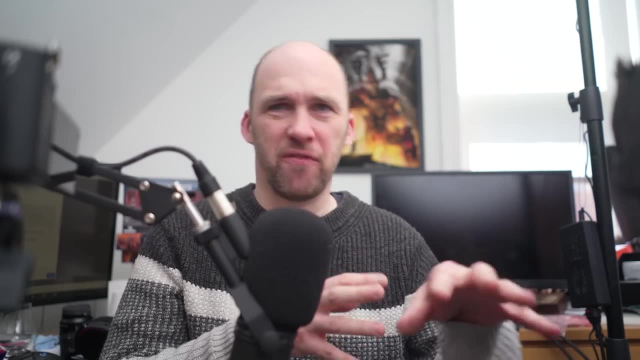 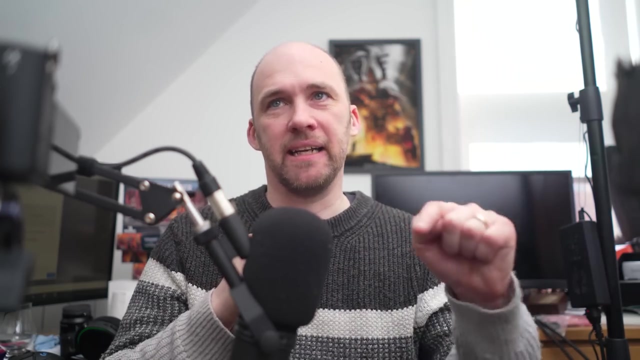 got a nice stylized uh outfit, um, so you look at you can instantly tell this is your, your iconic, and I've not seen other Troopers. I mean, there's been a few like comments on on my Instagram going: oh, it looks a little bit like um Destiny and like the guy from this or, but not like. this is exactly. 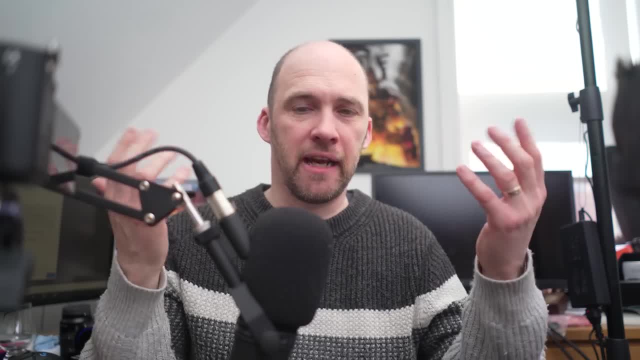 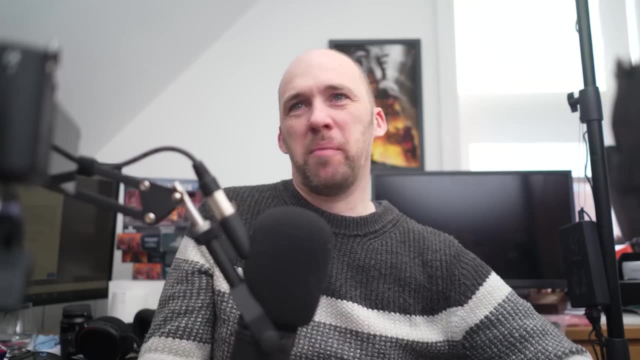 like it's like you've got like tropes and stuff you can like look at and draw inspiration from like anything. but the thing I've I like is like the armor makes sense. it's got like nice like these, like circular- I want to say Pistons, but hinges and stuff like like the leg joints and 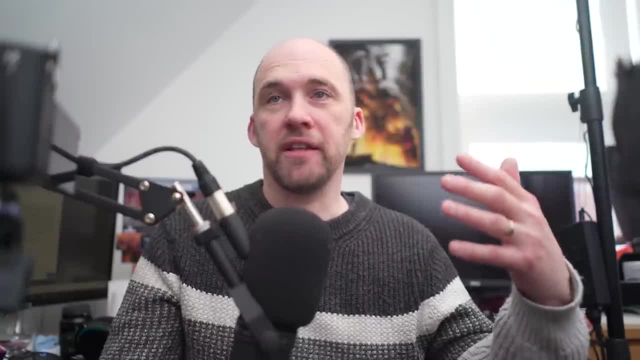 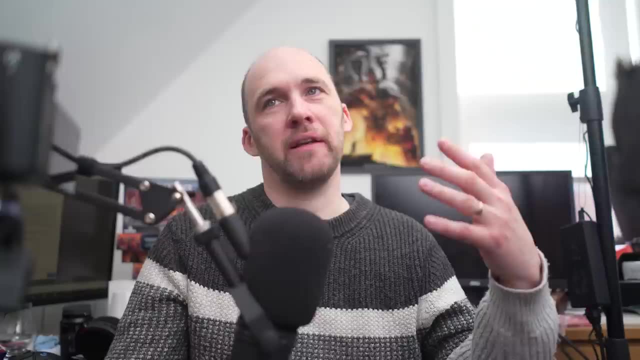 stuff, but as a a guy who likes to paint lots of things, I've really got in recently. last year or so was Legion and at first I didn't think I'd enjoy painting the clones, but having that opportunity to put like different clone markings on the clones armor. they're much smaller, uh, slightly so like. 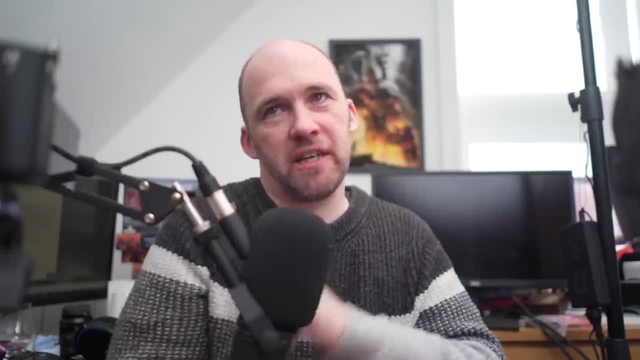 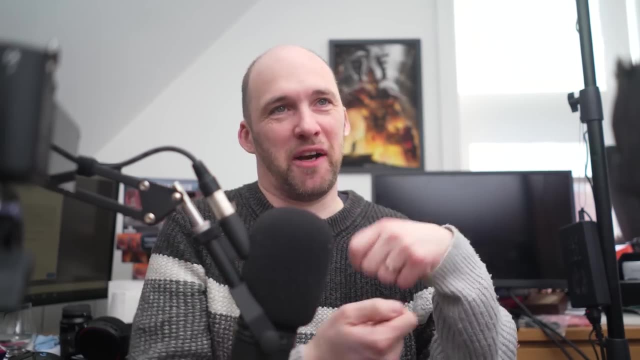 trying to do the 501st can be a bit of a ball, like when you're trying to get a proper true scale. yeah, yeah, whereas with your, your stuff, I can go a bit more to town. I've got a bit more larger space. my eyes are a bit failing, so I can like do broader lines and stuff, but I just found like doing white. 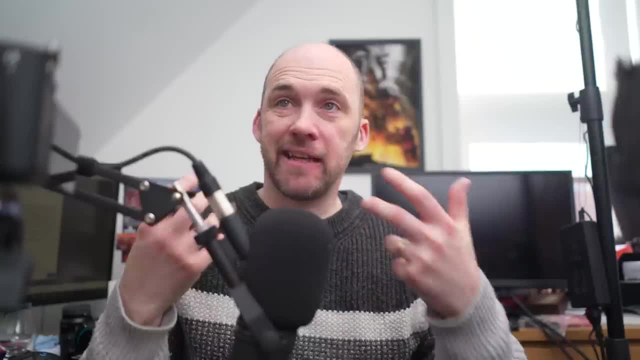 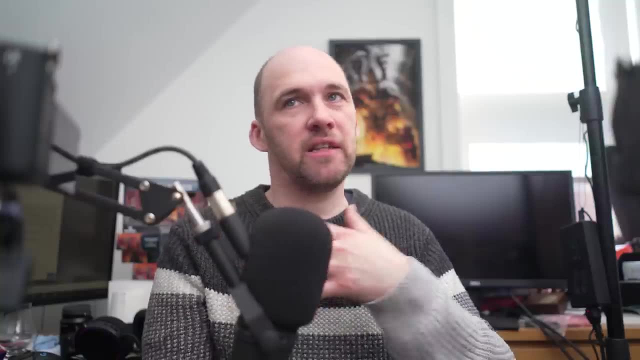 armor with red lines on it, or I've got loads of room to do camo patterns and they stand out. where you get like armor, you get like a bit of a breastplate, bit of a shoulder blade. you put the camera on it, it disappears when you put all the other colors on, just like: oh yeah, I did all that. 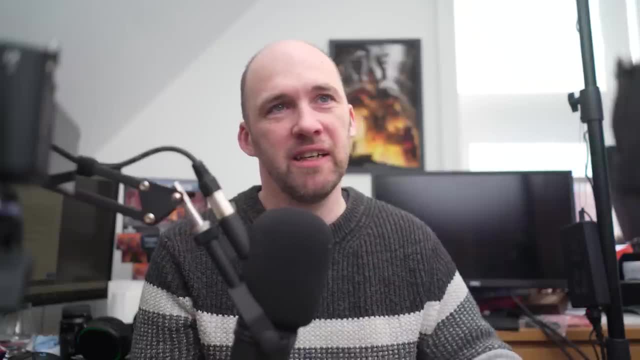 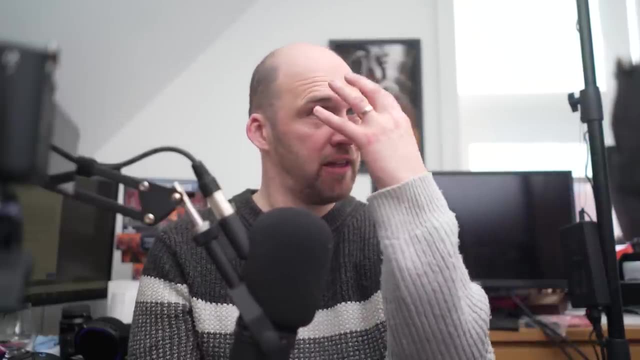 effort, and now I can't see that much of it because it's just like so small. and but this, I've got like a whole canvas of armor that I can put stuff on. I've got like some spot colors I can pick out, like the, the domed helmet, and then you've got these little buttons that I like do little glories on. 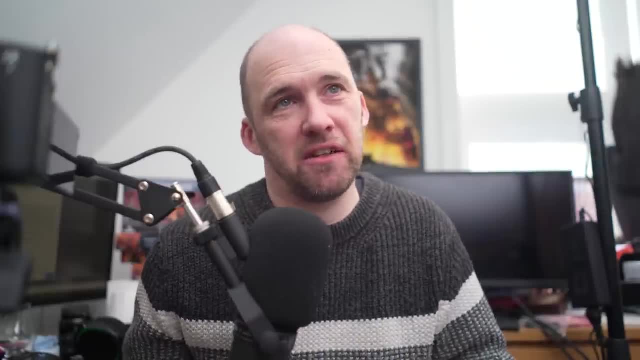 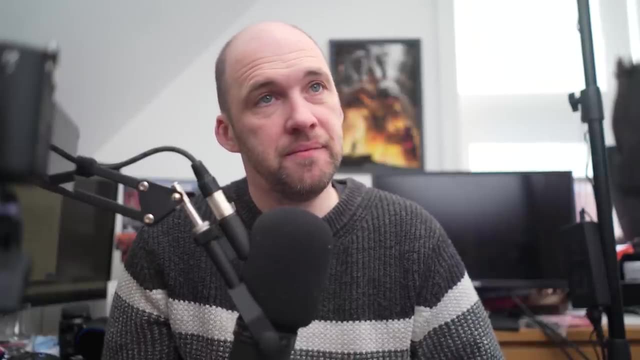 and stuff like that. um, and you can add details like the dagger. you don't have to stick it on if you don't want to. but yeah, and there's different places you can. yeah, for me, because I'm not a great painter of models, so it's again keeping it simpler, like that you've got. 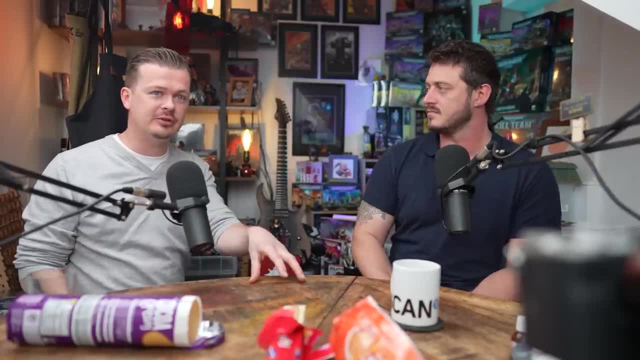 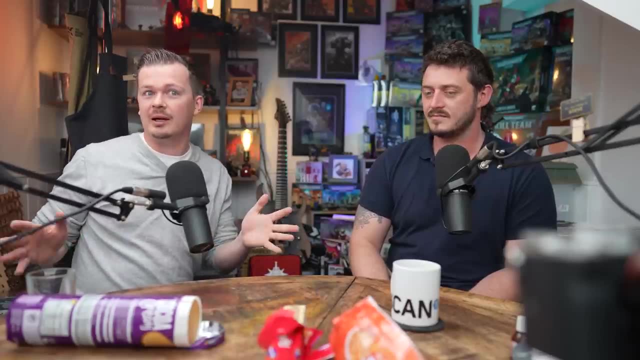 you've got, the more like the effector models. you're only going to have one or two of those. yeah, probably, so they can be more detailed. yeah, but if I'm fielding a load of troops- yeah, exactly, yeah, painting's not my bag necessarily- then obviously they're just, they're easier as well. 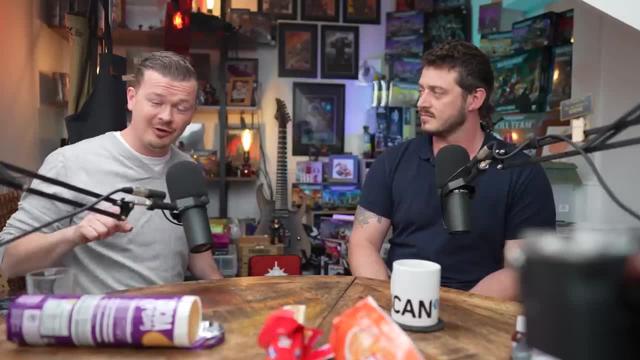 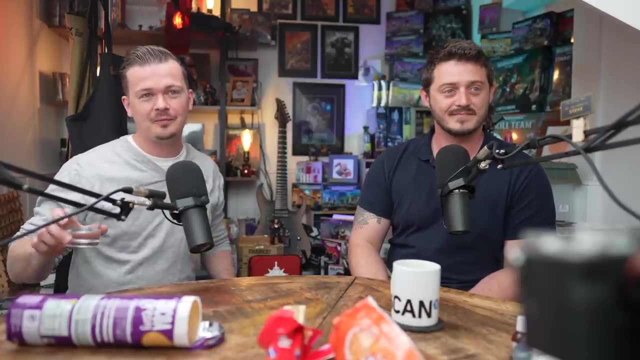 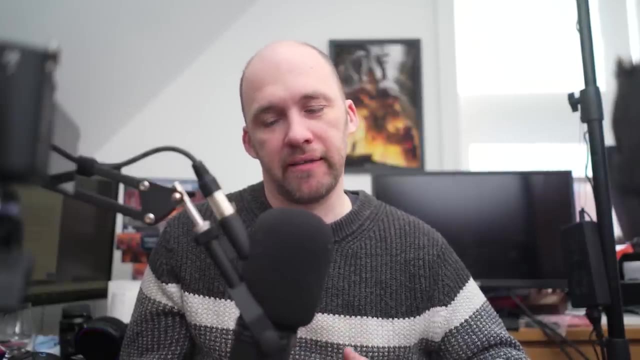 you don't want to have to paint if each one's so detailed and you feel like you have to get every single everything yeah in there. yeah, it's too much, too much for me, yeah, no, I mean, I think that that's a good thing to to push, really, because I wouldn't say it's like a floor of workshop, but that they. 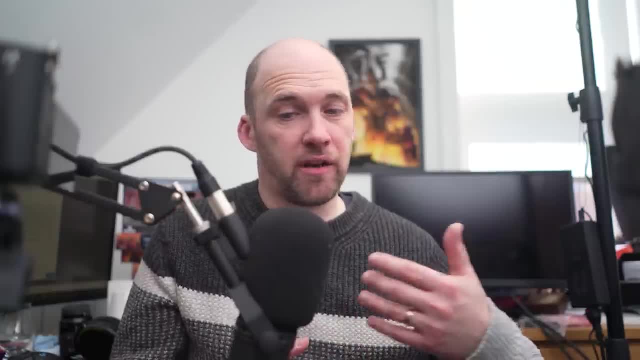 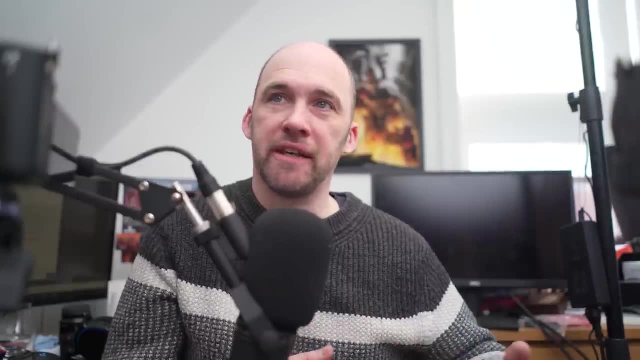 games, which has over the years, increased the detail of models, which is great for like painters and absolutely exhibition paint stuff like. but when, like someone like me who wants to like get loads of stuff painted, it becomes more of a hindrance than help. yeah, and it's extra time. 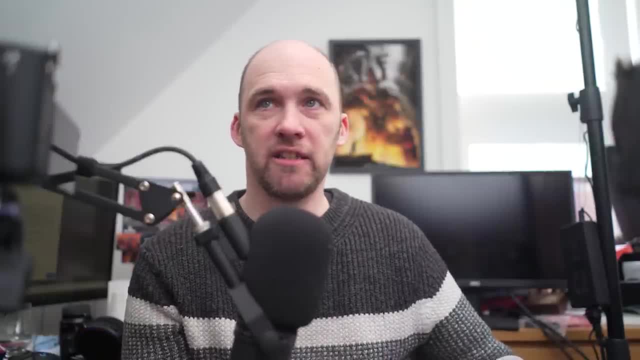 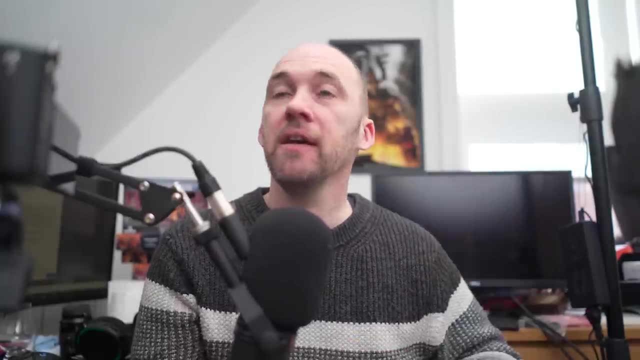 invested, whereas, like here, I could just like spray up white on like 10 figures. uh, do a wash, do a dry brush and then get some. I can put my effort into like a bit of markings. you've got time then to customize, yeah. yeah, I don't have to be working around belts and pouches and purity seals. 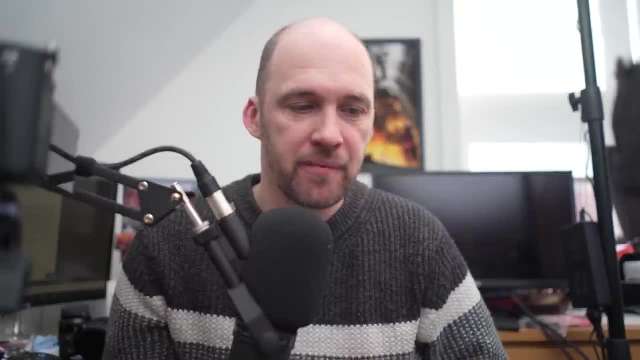 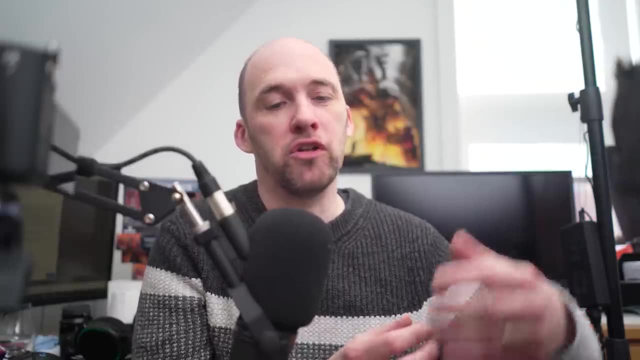 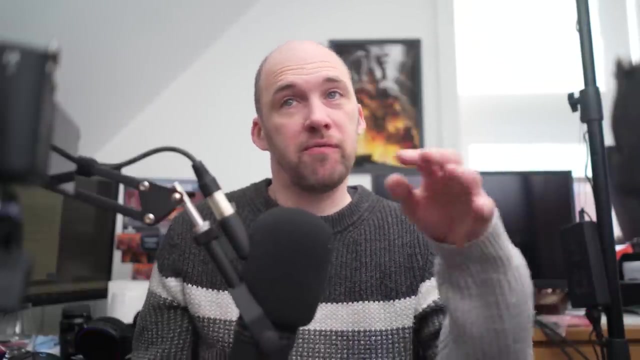 and like all sorts of trinkets and trophies and stuff. um. so for me it was like just seeing those was was great the level of of what you could do to it, even though it's like not as detailed as some other stuff out there. um, so I think that's a really, really good move. I've yet to paint some. 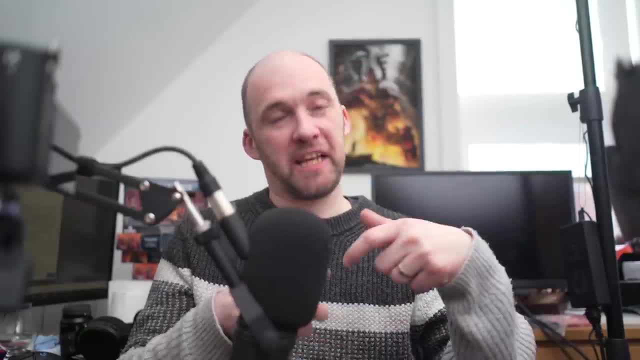 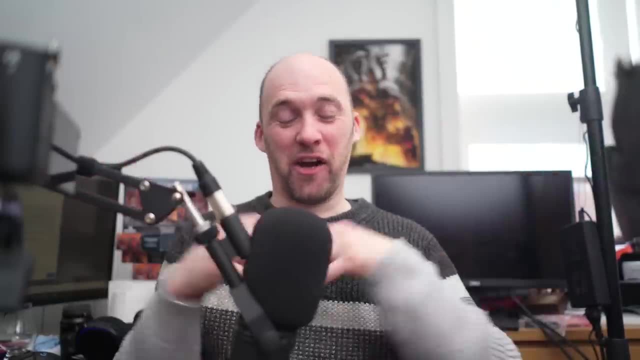 greys, I was saying to Pat, before you guys turned up, I'd sprayed someone my sticky bit on Mike and he dropped off and like one smashed or not at all. I can't, I can't like, because he's like broken in bits. I'm like I could try and do it. uh, I might use them as a corpse or just like bits of blown up. 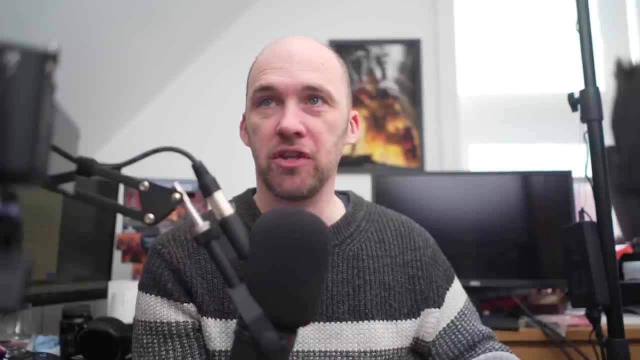 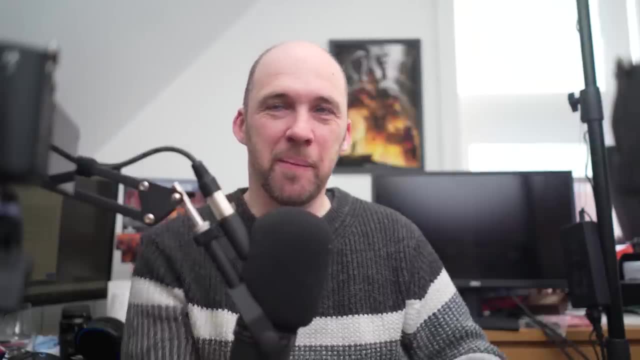 yeah, why not? um, but I really like the idea of like the greys versus humans. you've got these two factions, uh, in in the set, which is the greys versus humans, so you've got, like that, that Roswell connection, which is, yeah, um, you know, the greatest traditional looking aliens. yeah, the greatest thing. 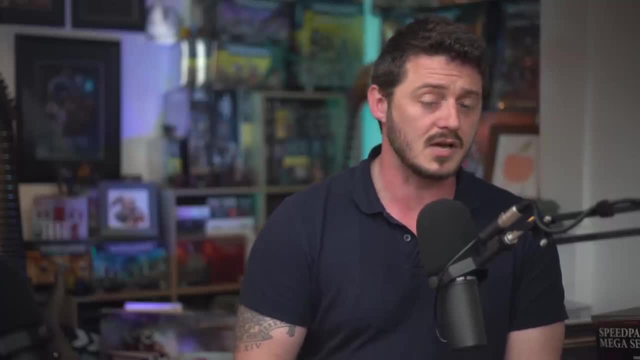 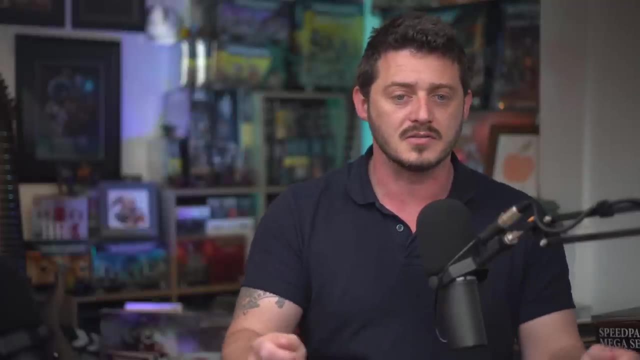 you mentioned, we've got the greys and the humans in the set. uh, yeah, the set that we sent you, um, but which is what you got? the four factions that are available aren't the factions that you you can get? you can choose one like two of the four. yeah, um, you could even choose both of the same faction. 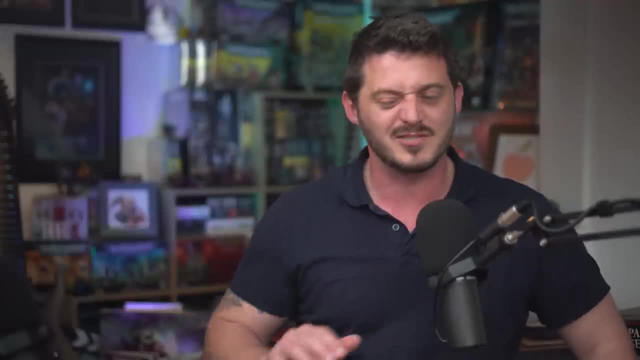 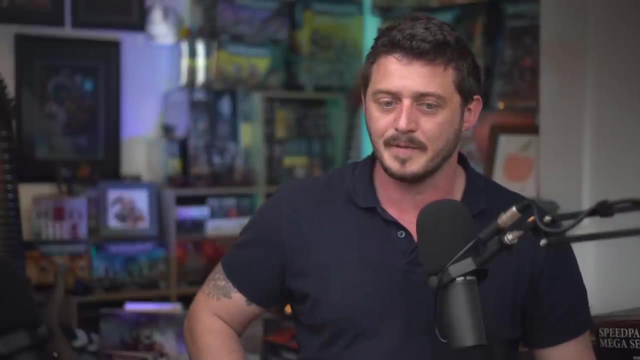 if you just want double up on the human forces because you don't really like the other three, you can do that as well. so you get like two tanks and things like that. that's absolutely fine, and that was another thing we spoke about. it's just like so many style boxes out. there is everyone. 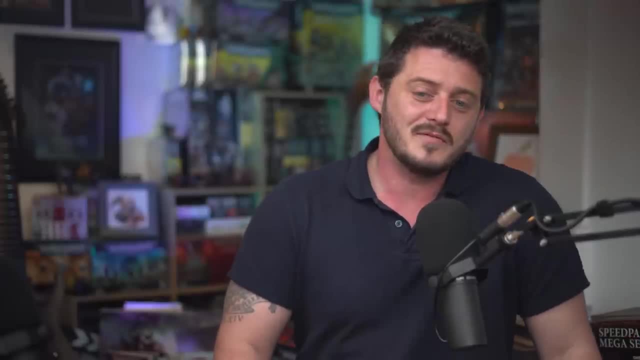 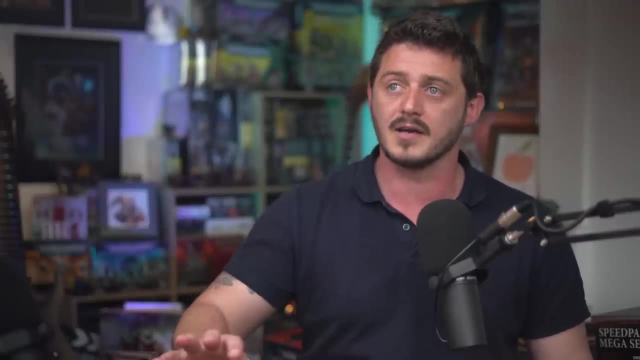 gets them. everyone's got exactly the same. yeah, yeah, yeah, it's just like: well, what if you've got all the comments? it's like, oh, especially. uh. last year at tabletop gaming live one guy went: I absolutely love the haraka. um, I've got too many humans in power armor and I was just like that's. 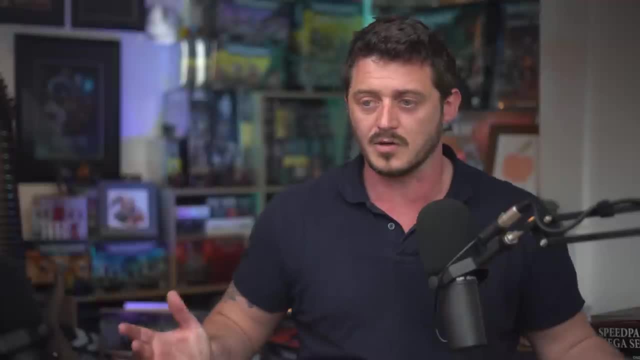 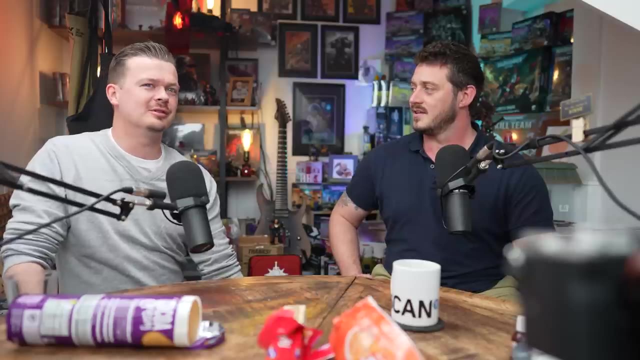 a fair point. man like I don't. I'm not going to take offense to that, because we all have lots of humans in power. yeah, yeah, yeah, um, you choose. yeah, it doesn't matter. I still think most people will go for humans versus grades. yeah, yeah, yeah, yeah, yeah, we've done, it's the whole. it's the whole. 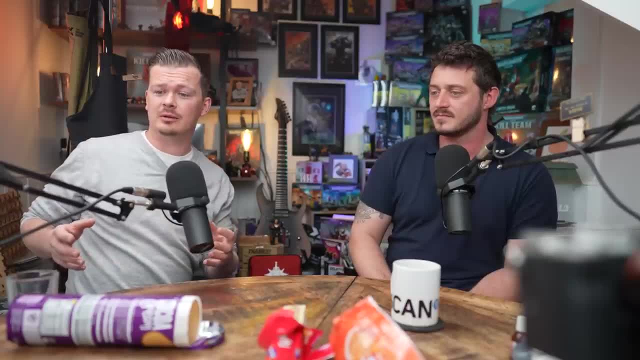 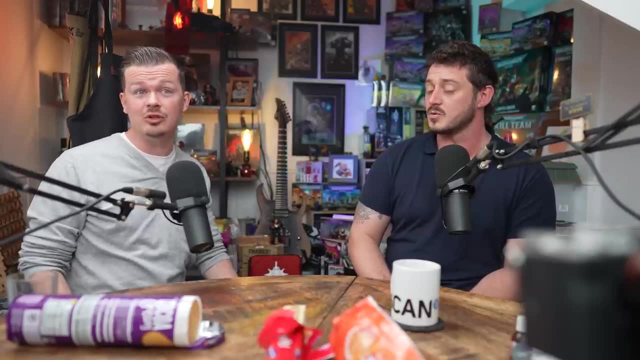 thing not to try and copy stuff. obviously, when you create something like that you don't want to, yeah suddenly realize, oh, it's exactly like that, yeah, yeah. and when we went online to find gray alien models, you can't, yeah, really. yeah, there's very cartoony ones, yeah, like ray gun and stuff, but 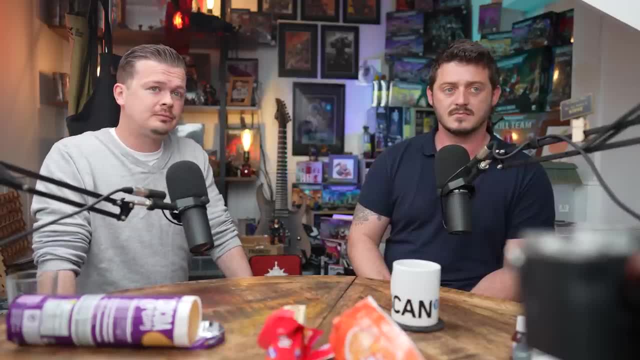 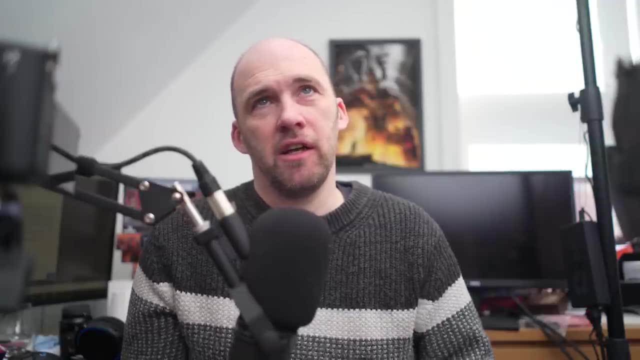 there's. there's really wasn't I mean the only uh models out there for x-com, or like a couple of human operatives that you get in the board game. yes, they did do a board, yeah, yeah. so it's like app-based, it's like you get like the original. well, I'll say the original, the x-com one, not x-com too. 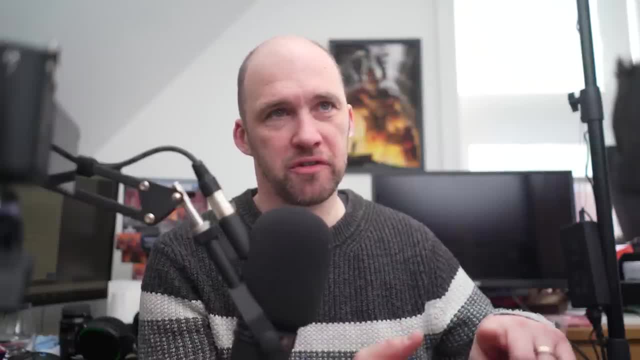 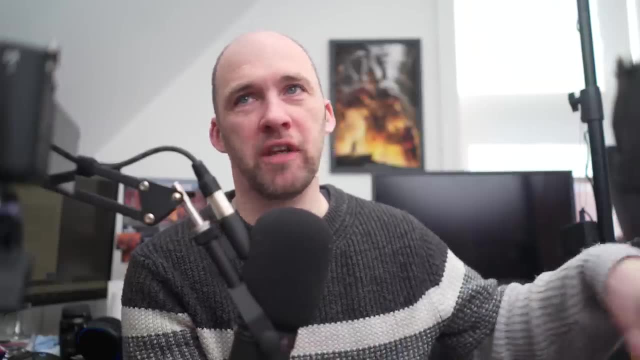 well, in the last 10 years, um, you have like an assault, a support heavy, and then something else, and they just like did each one of those four times so you could like use them on the board games, stuff like that. so they're the only things really that exist. are some human Troopers that. 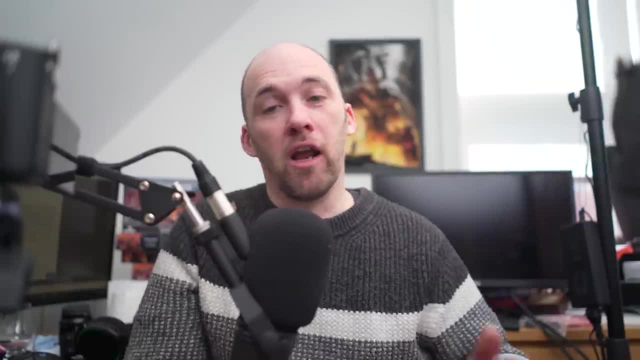 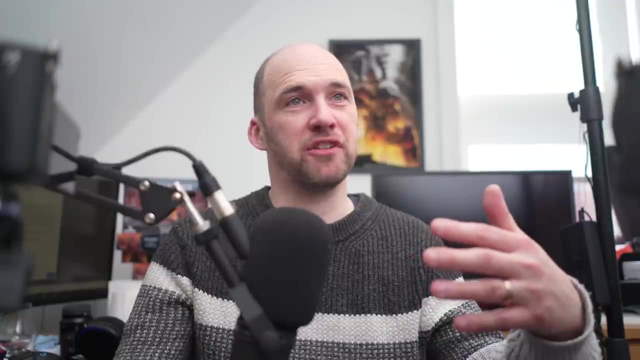 look nothing like your guys and stuff which is fine, which it kind of works. what I like as well is: and then I was going to um get to which I paint these guys on on Instagram. and then I read through, the factions went: oh, they've all got their own generated colors. ah, made up my own. oh, 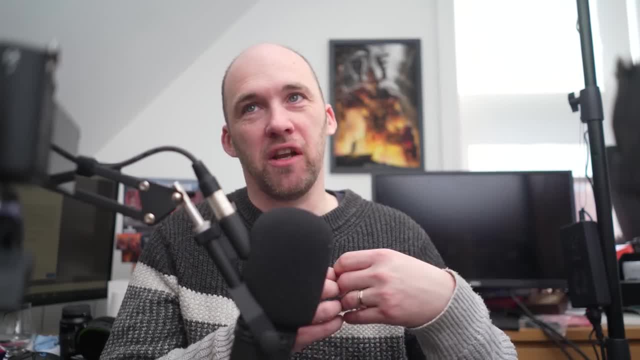 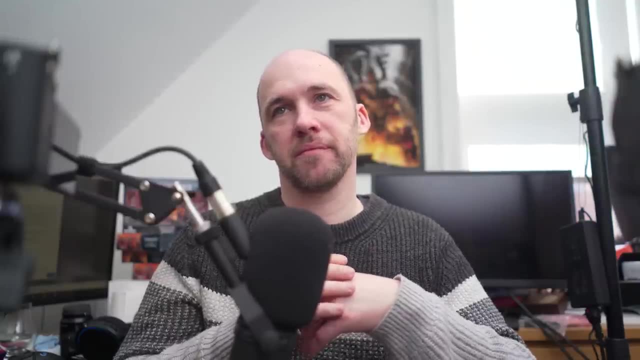 no, but then you know you could have like different factions or shoot off factions or different like color schemes from this this. yeah, so the way of the way, or well, because we did have quite a lot of chats over like how we're gonna, we don't want to do it too heavily because we don't want to lock. 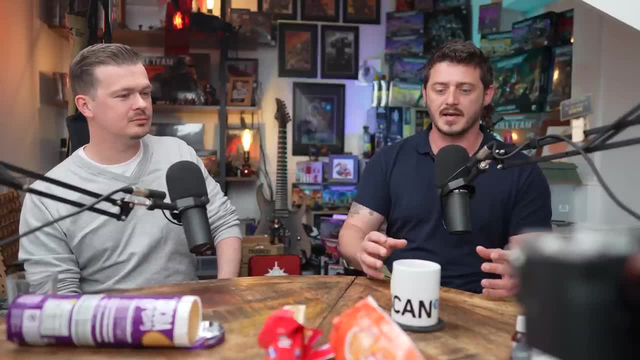 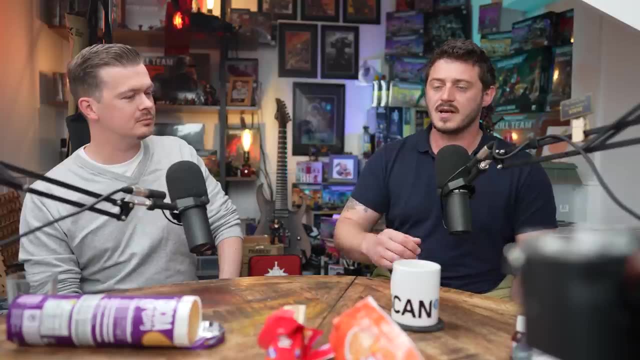 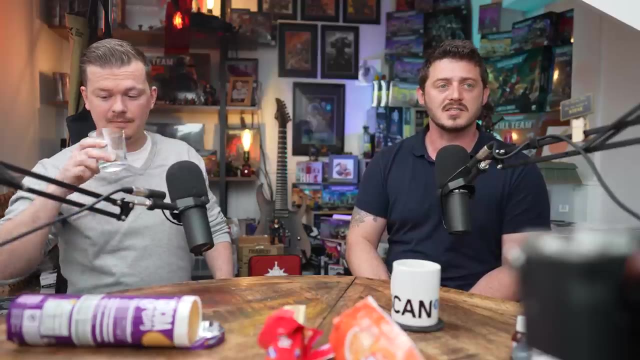 people into color schemes. um, so like 40k has had the main chapters that then splintered off during the second founding and then third and fourth. yeah, um, we kind of did the reverse, where um Earth got into a little bit of a sticky situation. everyone fell out. uh, resources became. 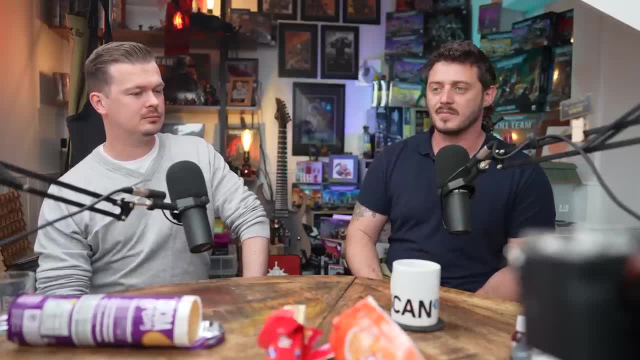 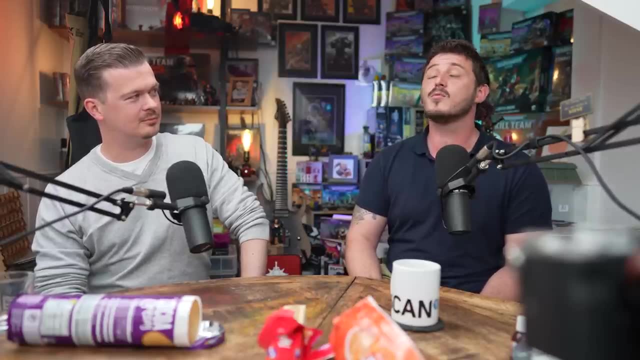 while they dwindled and people got a bit hoardy like um, I mean, a great example of that is just go back a couple of years into the old toilet roll scenario. yeah, yeah, it's just like no people would never do that people 100 do. that sounds like it's happening again, yeah, so I thought brilliant that. 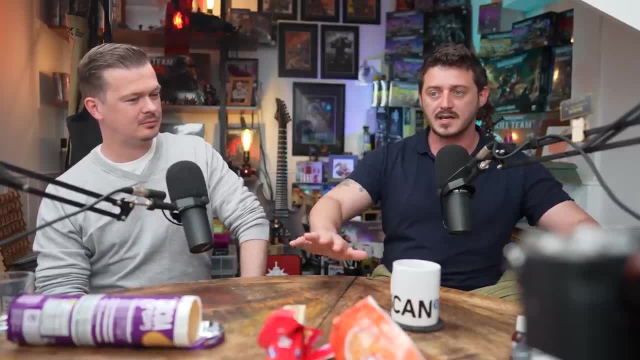 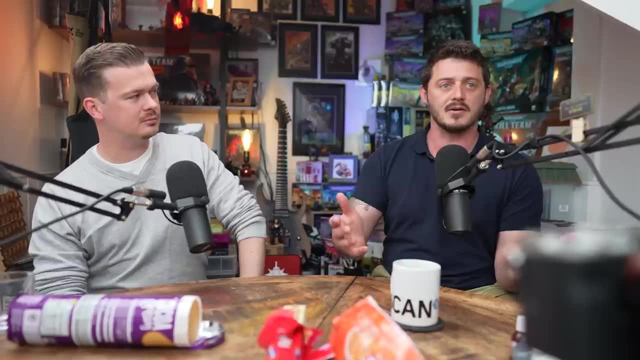 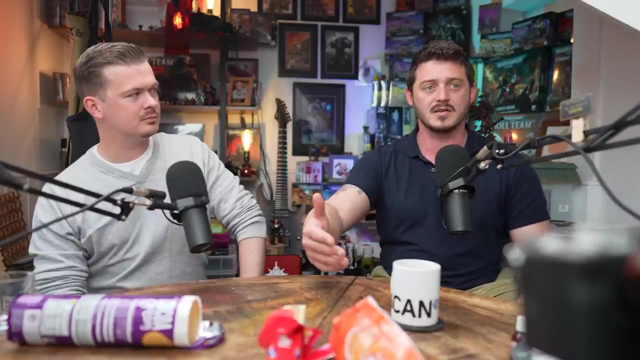 that then locks people off into groups and eventually, if that stays around, people are going to have territories again. reform country borders are going to break down and government's going to break down and eventually what you end up getting is just like tribalistic gangs in certain areas, given a certain amount of time, um, they're going to end up having colors. yeah, they're going. 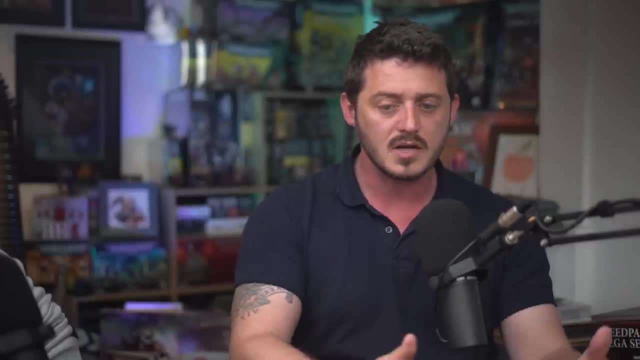 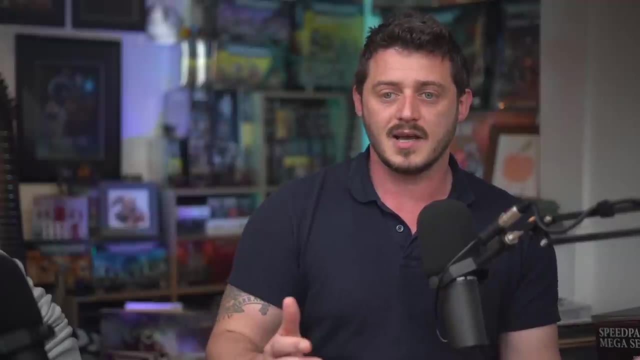 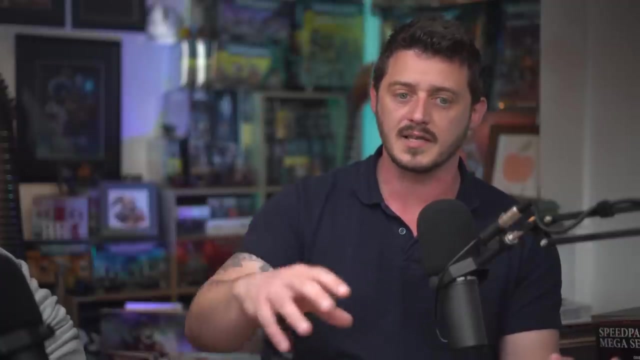 to end up having like all the same military gear, because they'll steal it off each other. so everyone's kind of equipped in the same way, just different ideas, different- um well again- colors, um, pros, cons to them, and then then we get attacked by greys and there's a reason why they then attack us in the law, obviously like the old. 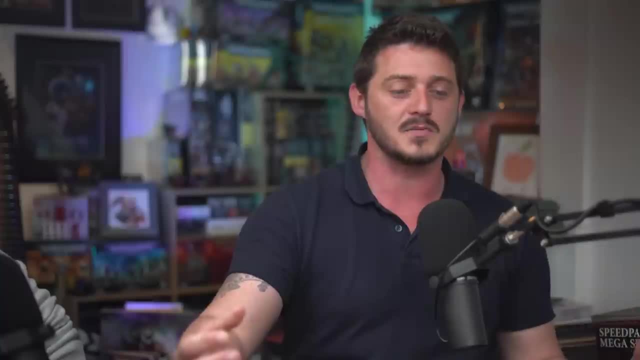 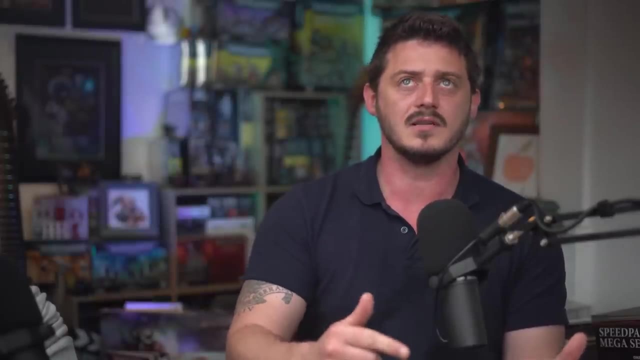 Independence Day everybody joins to defeat the aliens and that's when they form larger, the, the main factions, yeah, but you can do color schemes from them, because they're gonna still have ties back to their old tribes and gangs and things like that. so you can have, you can have a main color. 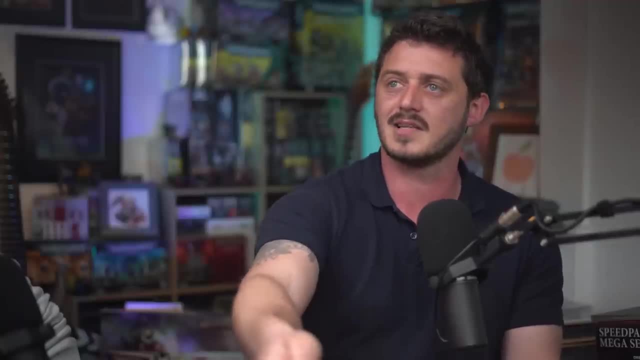 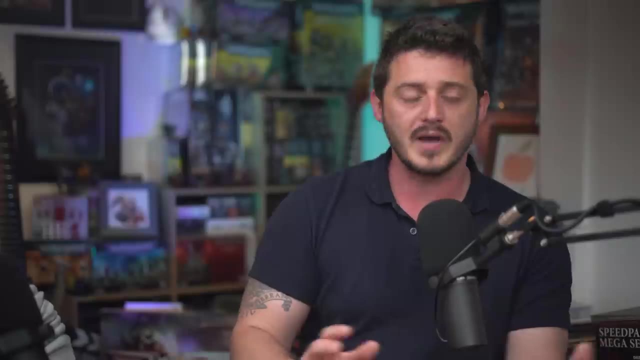 with a different arm, because that's a little bit of tying back to their previous. you can do anything you want with it. yeah, um, because we haven't really got any faction specific rules yet. we've got ways to implement them in the future. we've got tons of ideas for the future, um, but we just want to get the game out there. yeah, get it. 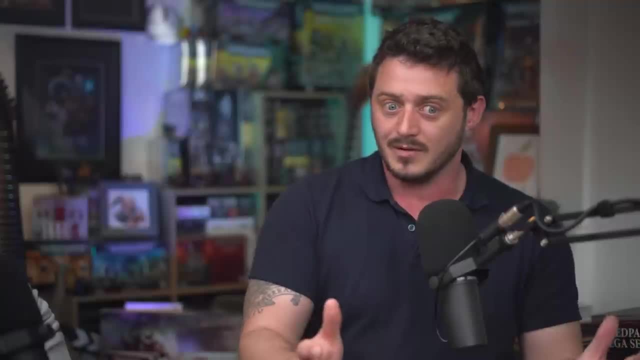 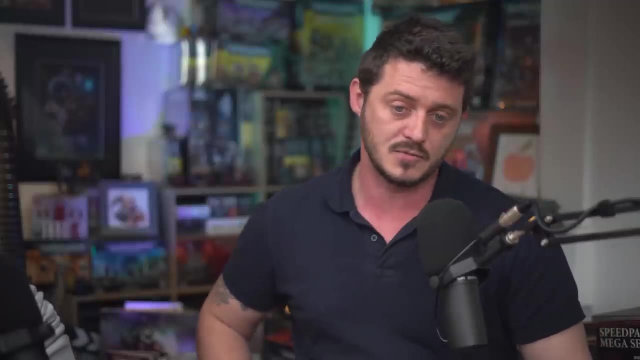 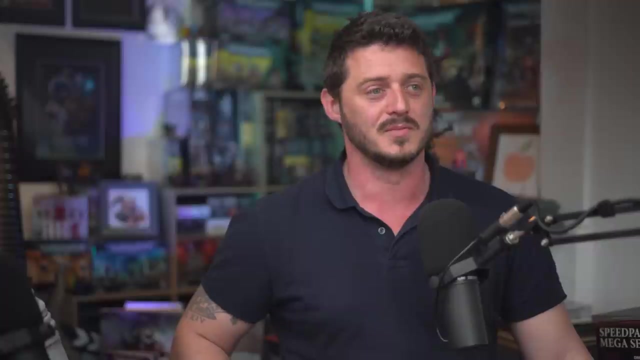 settled, maybe release another faction, uh, because we've got more, so many more ideas, yeah, um, and go from there. so, colors wise, it just paint them however you want to paint them, and I'm I've been loving seeing all the different color schemes. it's amazing to see what people are posted and stuff um. 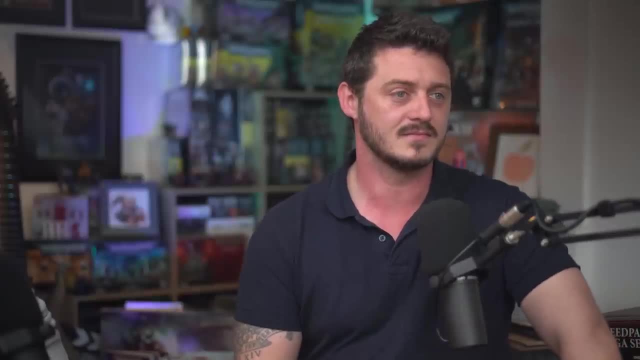 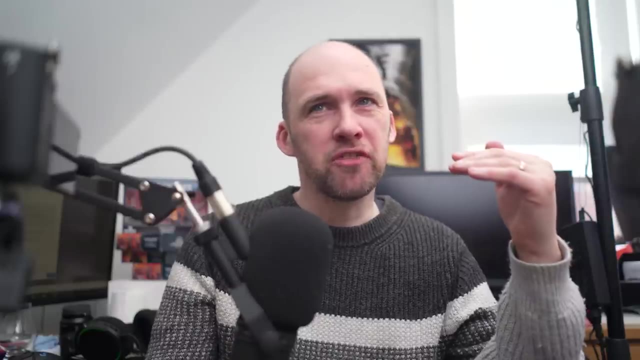 once I've realized that you've got like a bit of background for each of the factions, I was like, oh, I'm gonna there's like symbols so that, like you know, they've got the- uh, I'm gonna get this wrong, so you know, correct me. there's the American continent: United Consonants of America. yeah, 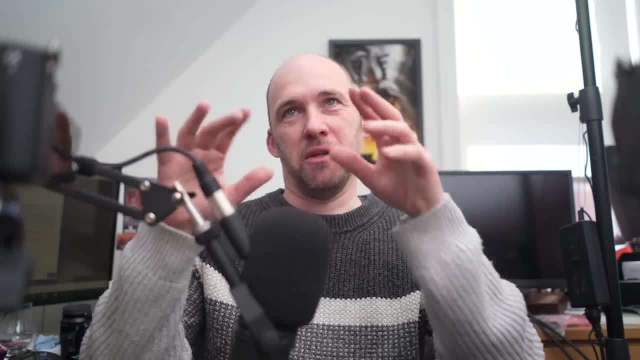 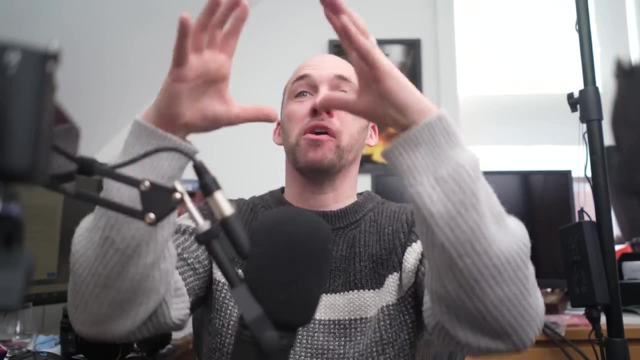 United Consonants and there's. there's what I would probably refer to you. you have to tell me the name, but it's pretty much like China, top of Russia, Central Nations, yeah, yeah. so I was like, oh, that's cool. so you got like you've made your own sort of yeah, this was this in in our world, or the album. 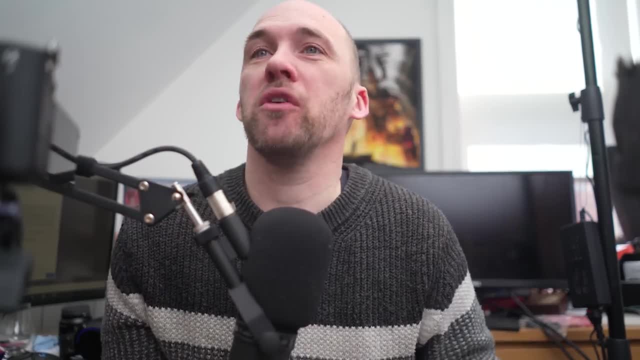 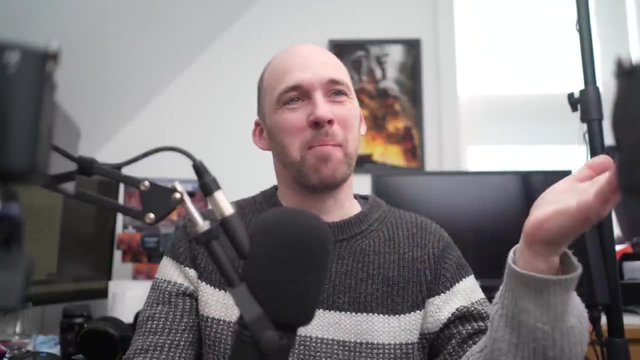 or a bunch of other um countries with it as well. so it's become its own own thing, which I really like. and you look through and you've got a bit of background to me, you've got a bit of colors and there's just one called the darkness. is that based on the pop group? no, it wasn't. oh, because I want to. 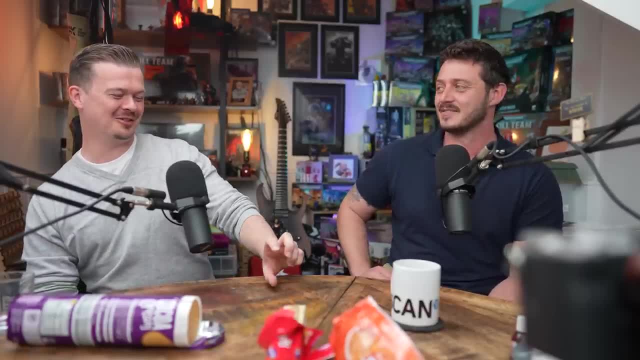 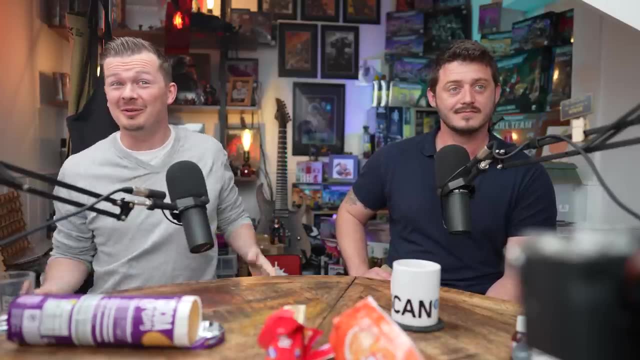 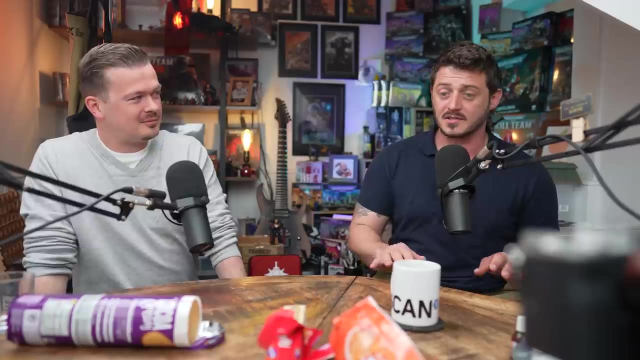 go. it should have been. yeah, just have like. Justin Hawkins is like a custom. yeah, yeah, um no, we just thought it was a cool name. yeah, and the description was like: top secret, top secret. yeah, they all wear black. yeah, yeah, certain sub-factions are still black, but this is matte black. that's a little bit. 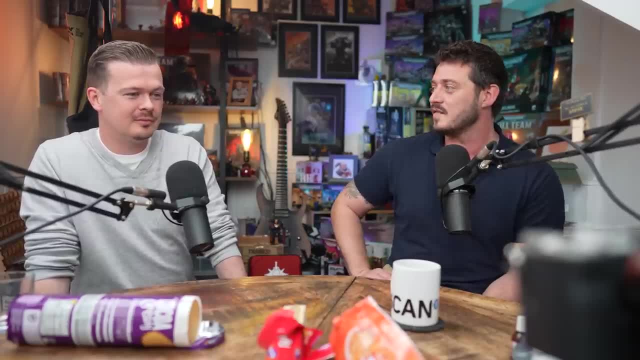 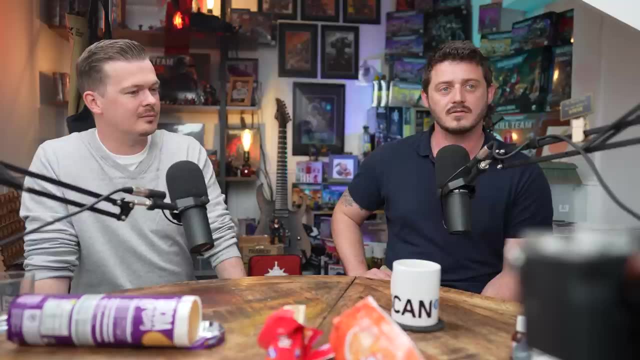 of gloss black. yeah, yeah, that's a bit of both. yeah, and it's our favorites. um, the al-kabulin Empire, um, I think we found years ago that there was an old term for African continent and we thought to reunite the continent under one banner, so to speak. it's, it rolls off the. 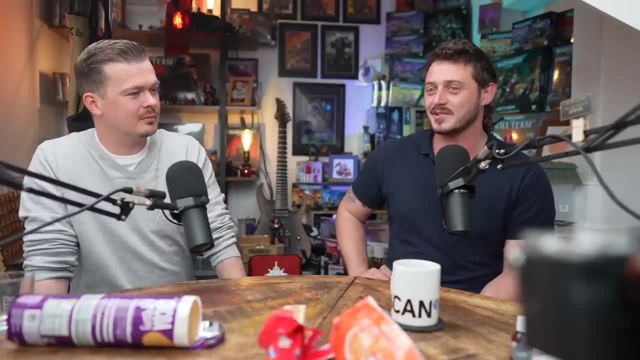 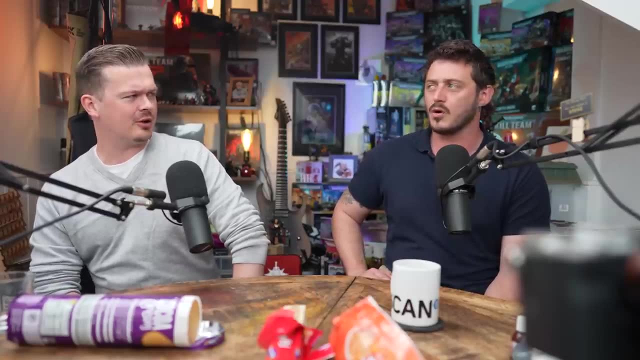 tongue really nicely. yeah, yeah and um, every step of the way. we're always. we're always thinking, oh, that'll be a great rule if we have the leopard print ones. no, yeah, and every time remember because it's so- yeah, I think- spread across the world. we're starting with 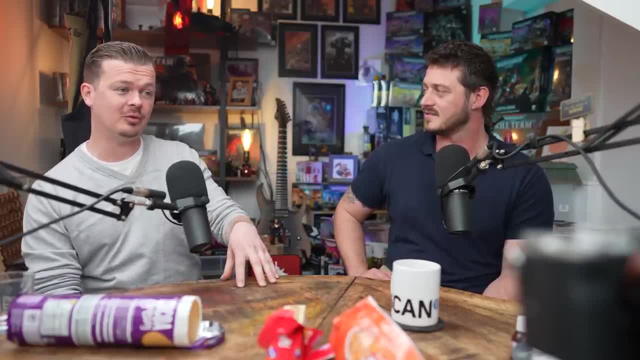 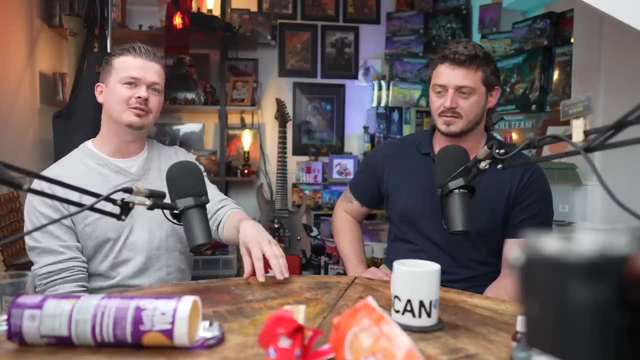 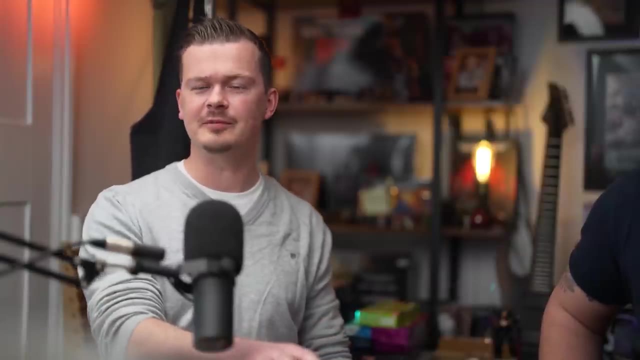 four uh forces, but over the five that we'll have, um, I think there's 63 different factions we've got so far, so we've come up with different. yeah, and I say for the humans, they've each got their own symbol. and then, yes, yeah, they've got their own. um quotes phrase, motto, I think, but it's in Esperanto. 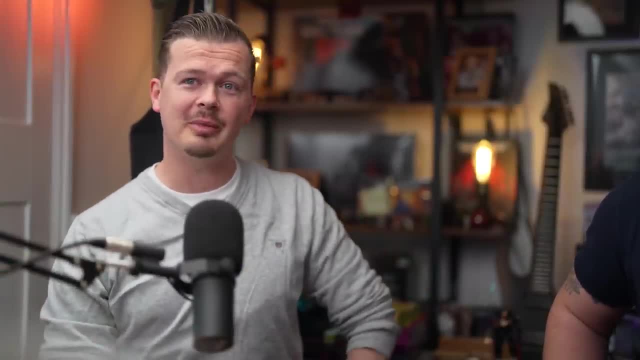 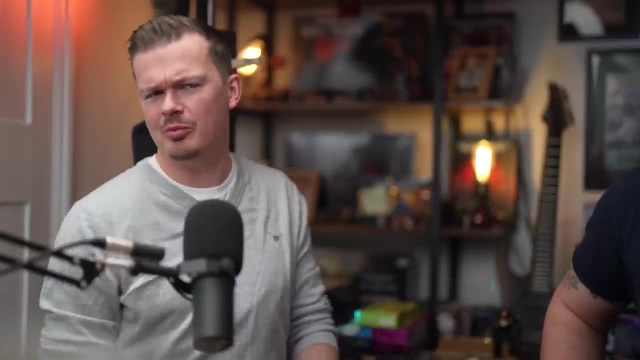 because obviously in in our books, as as the world's come back together, we've formed this global language. uh, we tried to come up with one and we thought, well, they've already tried it with Esperanto- which is: yeah, that makes sense, yeah, nice, um, so your humans come with like these cool domed helmets and stuff like that. 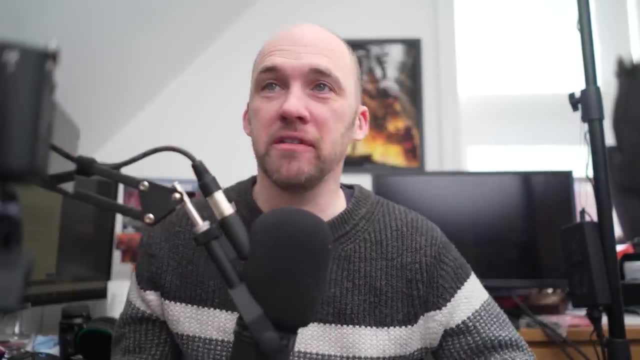 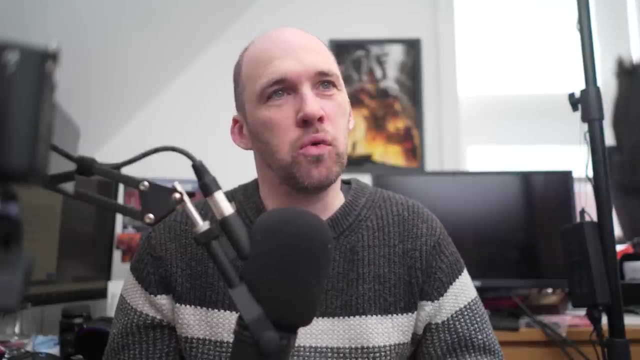 um down that? I mean, I'm not at all suggesting anyone should do this, but down the line, are you looking like doing like different sorts of um upgrade sets for like different weapons and helmets and stuff? hundred percent? yeah, you've got loads of ideas for different. well, because of the 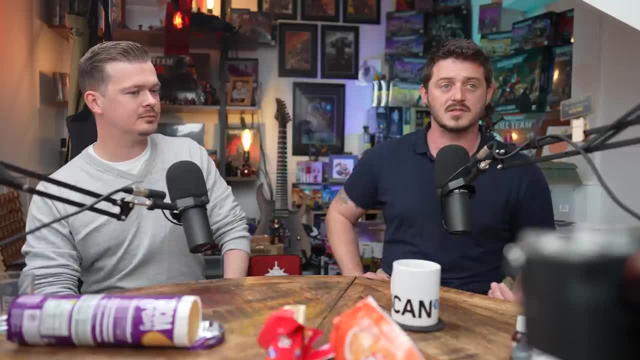 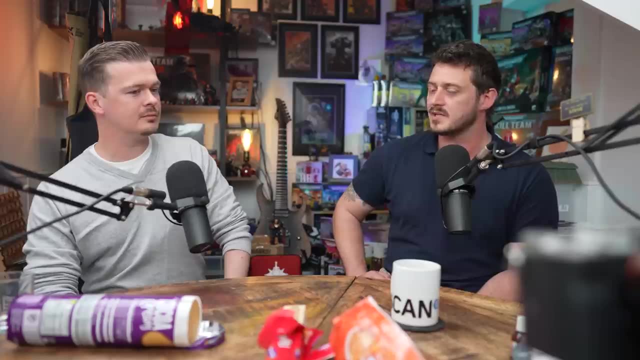 yeah, factions across the human force, um, and as I've just explained about having different backgrounds and everything, we just want to try and piece together quite a bit from all the world, mix match some of them and bring them together, yeah, yeah. so yeah, there'll be faction specific ones and then 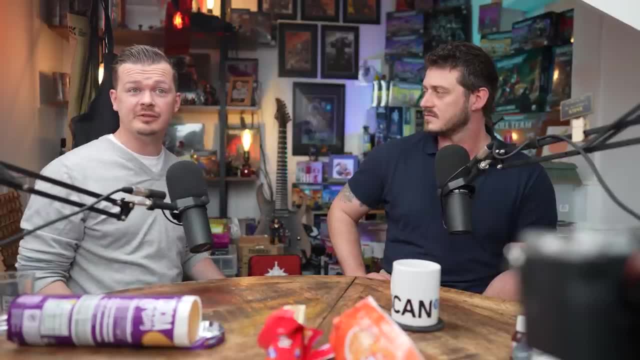 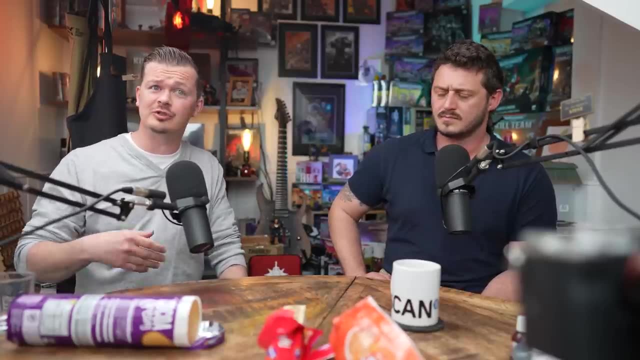 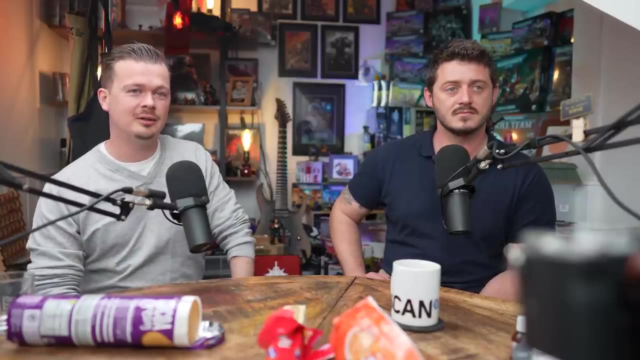 they'll just be general ones, because some people like painting heads and faces. yeah, yeah, yeah, and, quite frankly, even if they, even if we didn't, there were so many decent companies online producing, or yeah, people have been. yeah, I was looking at uh, trying to get like mine, Jeff, and uh, Pat's head 3D. 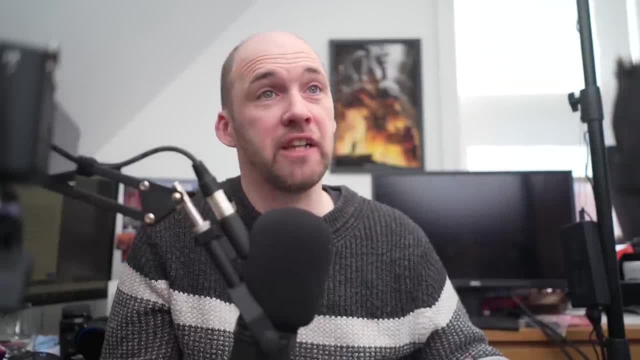 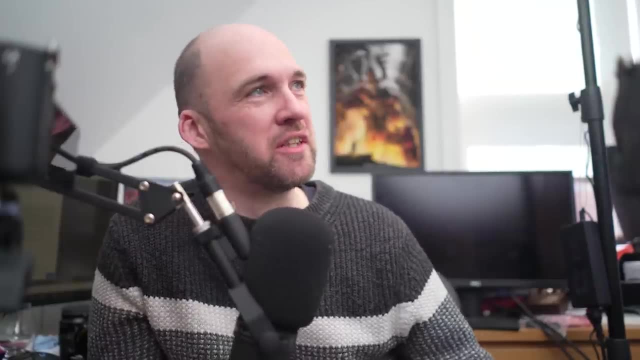 printers, a guy who ran knots. we've got to get the stars to align because he's like: I want to scan your faces, oh yeah, because you've got those things now. yeah. yeah, he could only do weekends, but Jeff can't, and then the weekend he wanted to do we were all like busy and stuff like that, so I need to. 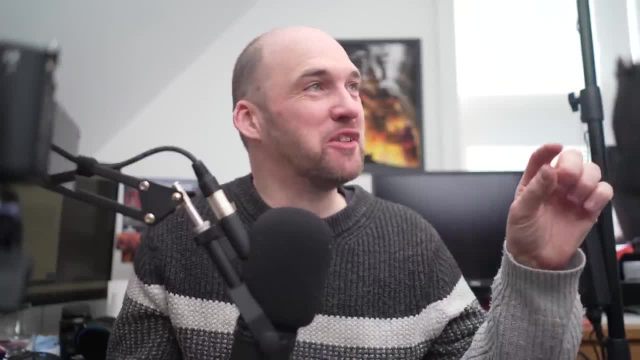 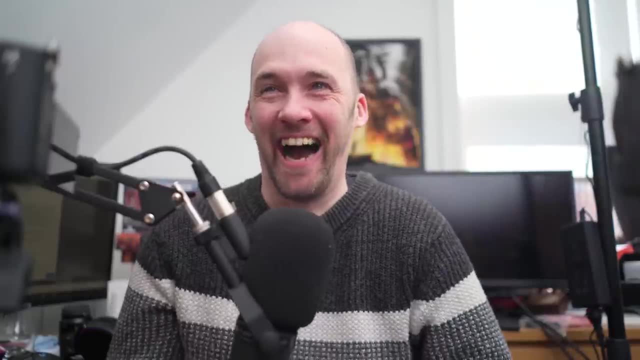 catch back up with him. but I'll just be great. just have different scales of our heads that we can just, like you know, all sorts of different models, like I want to do some Napoleon X. let's stick my head on something. just have your face on a warlord Titan, yeah. 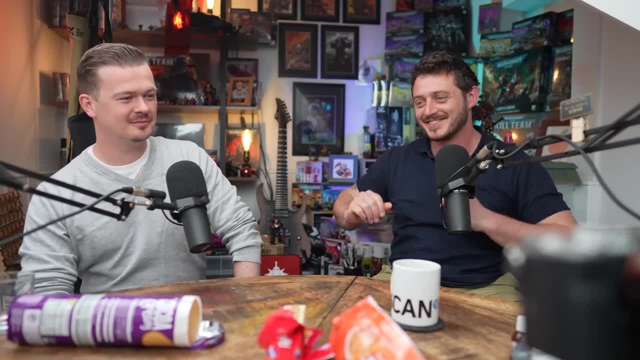 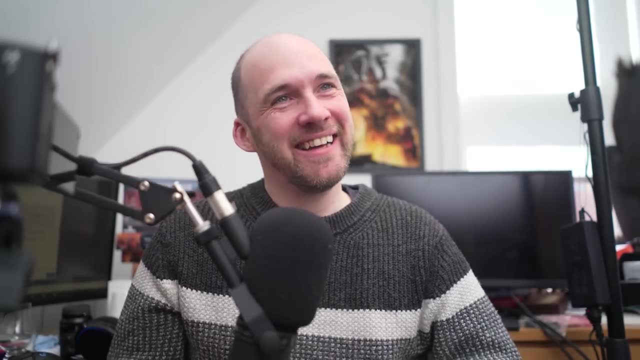 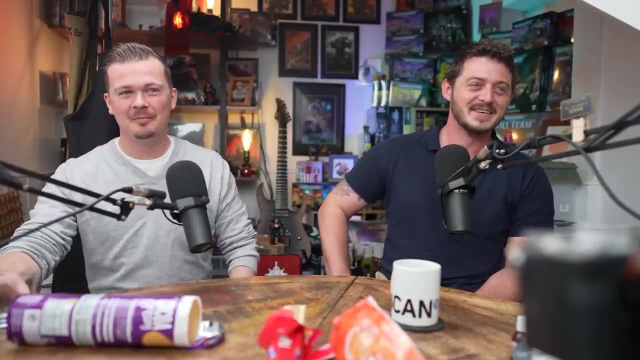 oh, I could just get cardboard and make it out toilet roll, just walk around on the tabletop, do it. so, yeah, you have to wear that, to choke on that. yeah, yeah, yeah, boom. so so you've come up with this background. you caught the law. um, how did you find doing the? 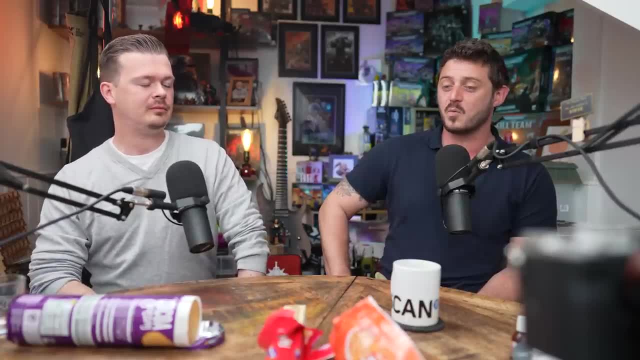 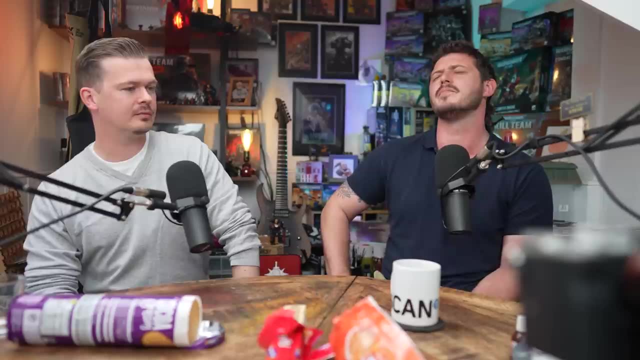 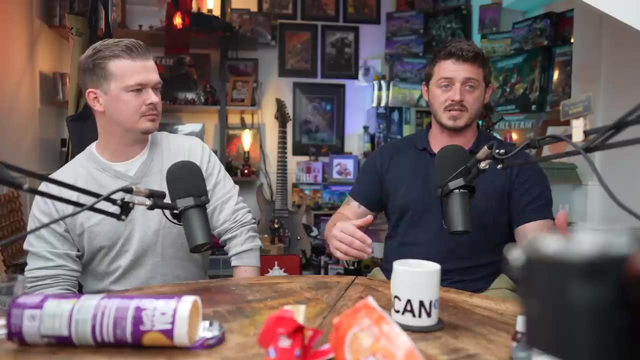 game mechanic. well, we, there was one thing that, as soon as we had it, the rest of the game, everything just followed through, and it was the impact, uh, the um, engagement grid, okay, which originally we just called it the grid. yeah, yeah, um, and it was the 20 by 20.. yeah, um, how to hit your? 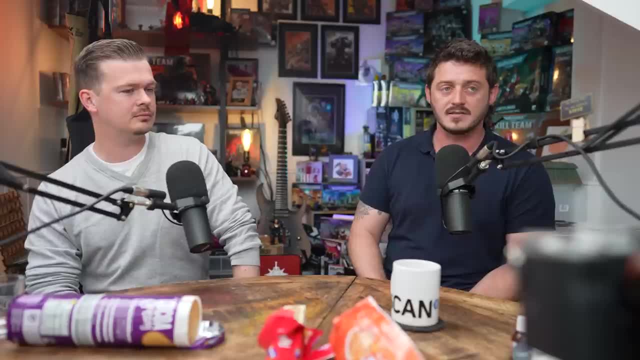 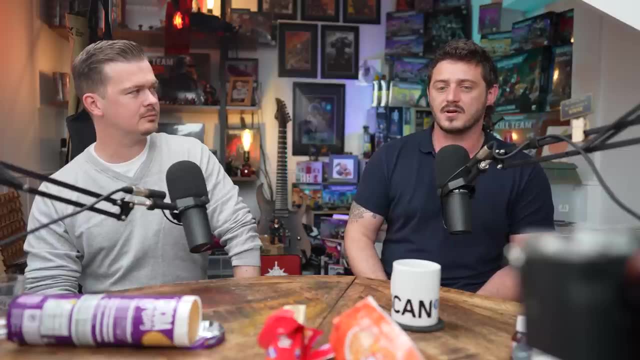 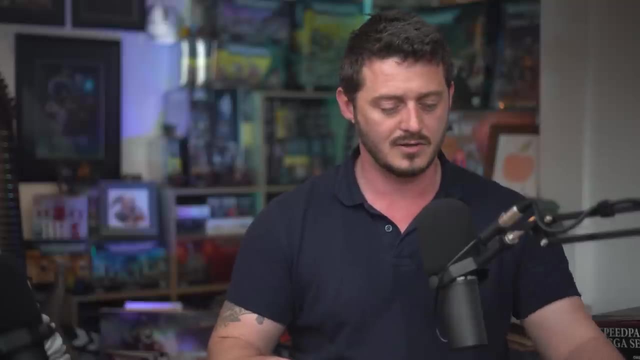 opponents and everything from there, all the characters, um sort of like intelligence records or their stats, the movement, how to hit, combat, ballistic, everything. we use that grid to try and find how outrageous something would be like. if we need good armor, how, using the baseline of what we've got, what would it need to be to be like a decent armor? that's good armor, that's good armor. 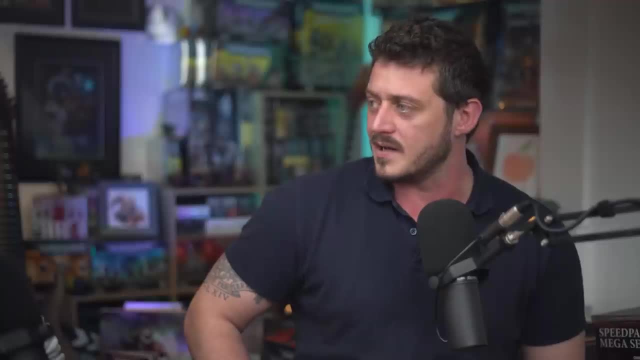 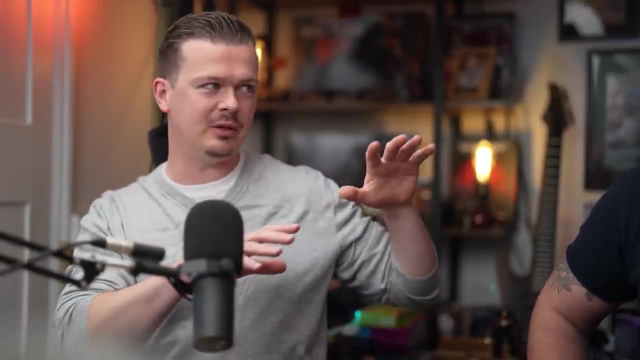 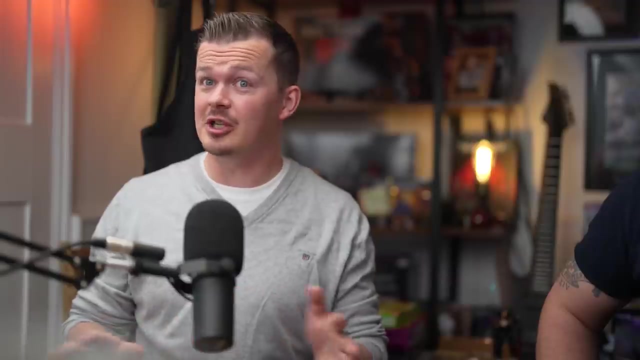 stat: yeah, and everything seemed to fall in place. we, I think what helps us a lot is we had, um, we had the sort of juxtaposition between will being familiar with a lot of tabletop games- yes, yes, and rule sets- and me basically having zero knowledge. yeah, a little bit some idea of 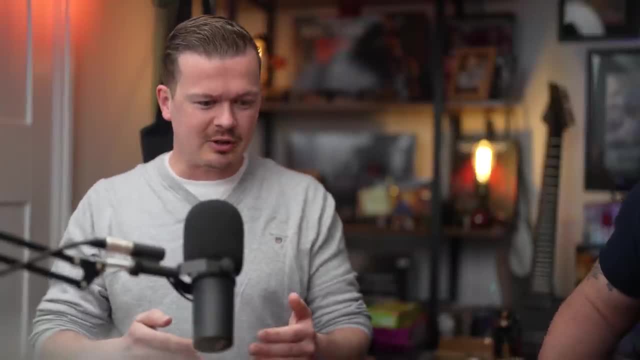 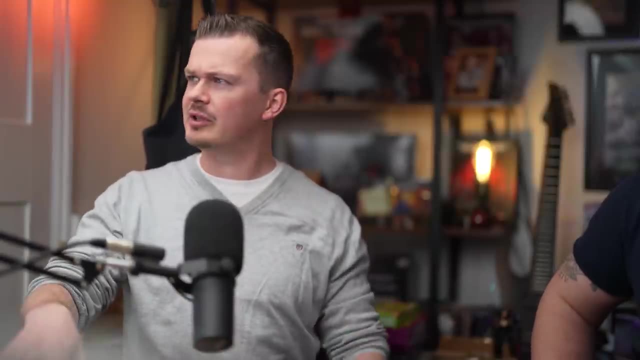 how bits and pieces work. so there's when we were coming across. yeah, it's like: oh, so now we need to talk about movement. yeah, this is what other systems have done. it's like: well, that okay, well, that sounds good, or that bit, why would you do it? like that doesn't make sense. yeah, so putting. 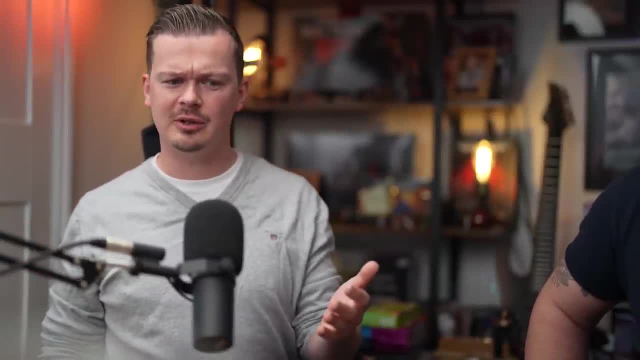 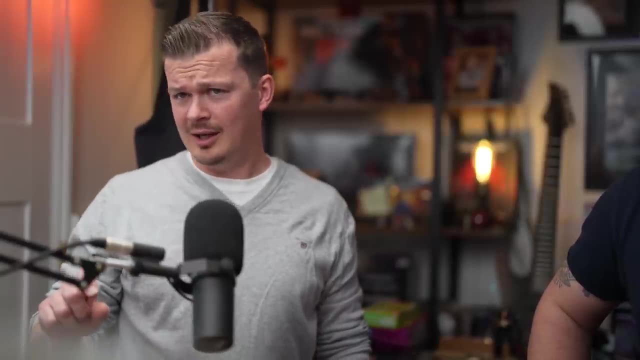 those two ideas together, because sometimes it's just: oh, that's just the way it's done and someone goes: well, that doesn't make sense. yeah, suddenly you realize, oh, there probably is a better way of doing that. like I never understood a d6 for everything. um, yeah, I'm not picking on them. no, no. 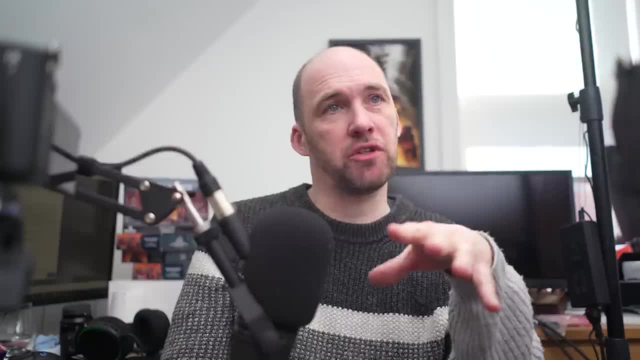 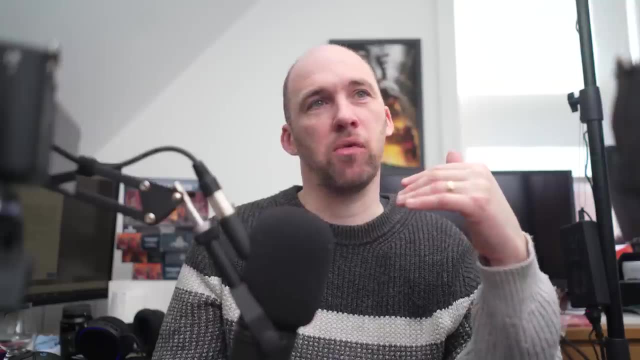 I mean, I'm so used to these six and I've only recently a lot of people. we had a guy called James Hewitt on it was a games. yeah, yeah, watch that one. yeah, on on a lot of the comments. so workshop games should be d10 and I was like I've never even considered, like the difference between 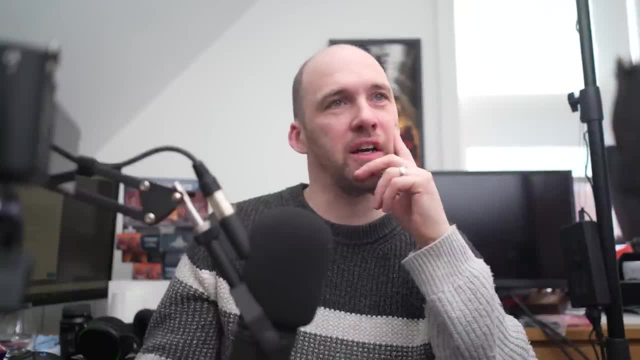 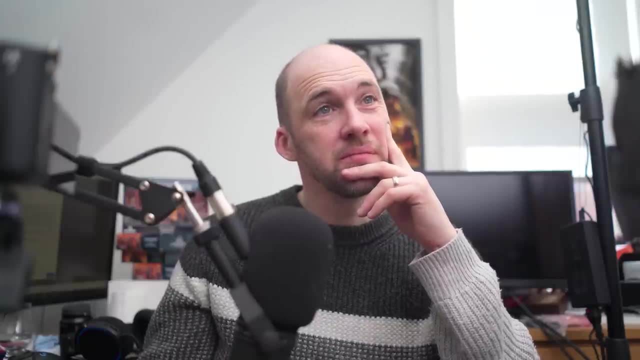 moving from d6 to d10. so that's like so much if you've got something tiny up going up against like a pain blade. yeah, you just got six. I mean it was. we jumped even further. I mean we've obviously gone d20. yeah, yeah, yeah, because then you've got that full. what's better than 10.? but then it gives. 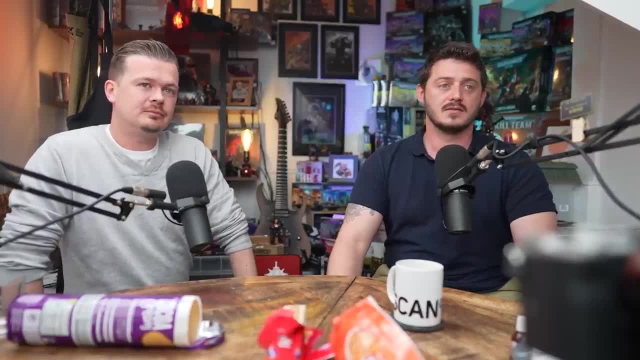 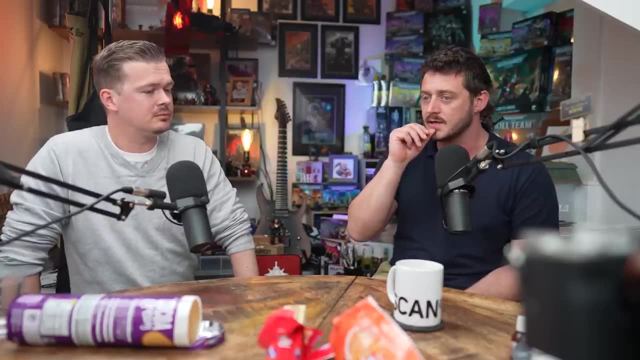 you more scope right to fit more stuff into it. so, yeah, which makes a lot of sense really, because I never really made that connection because I'm so used to d6 rule system. well, I was, yeah, I had a lot of times, and there's there's loads and loads of times where, as Alex just said, weird he'd sit down. 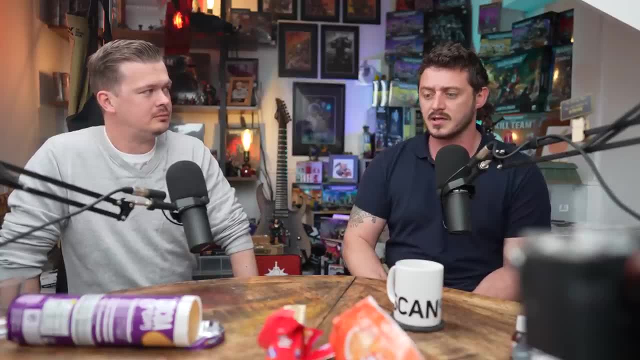 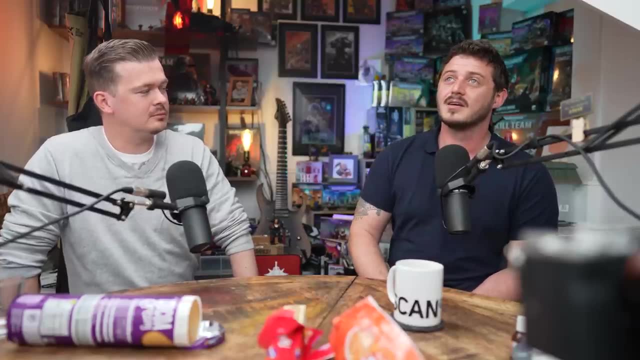 okay, how does so? how are we going to do this? oh, don't need to explain it, everybody knows how to do that. it's like, no, but they don't. yeah, it's like they're doing like what, if they've never played a tabletop game. oh yeah, good point. it's just like, oh yeah, yeah, they don't know how to do that and 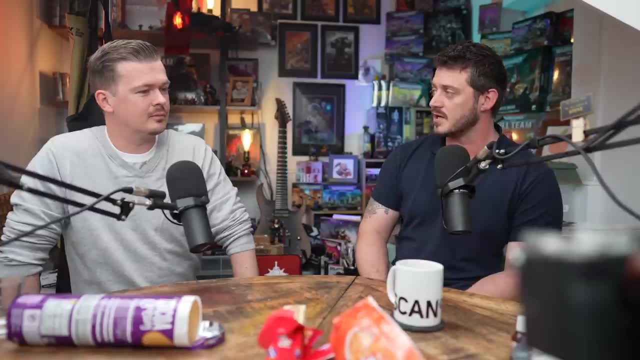 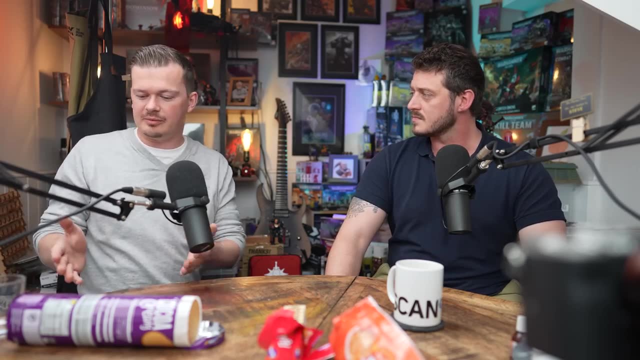 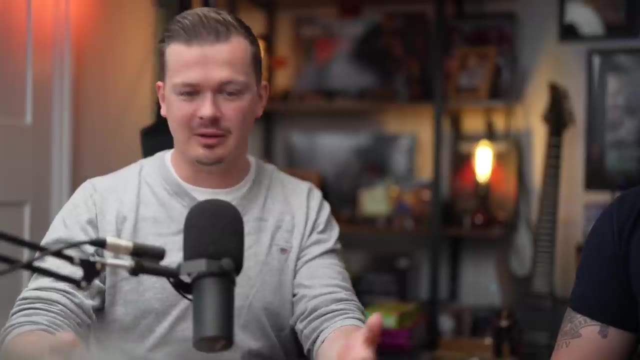 it's. yeah, a lot of the rules actually were aided by yourself not really knowing or not being familiar with lots of different rule sets. there's certain things in in rule sets which it has to be that way. yeah, you can try and make things as realistic as you like. yeah, it's still a game you've still got. yeah, you can't have just 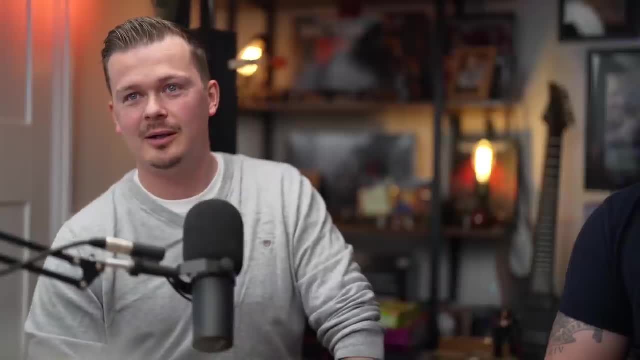 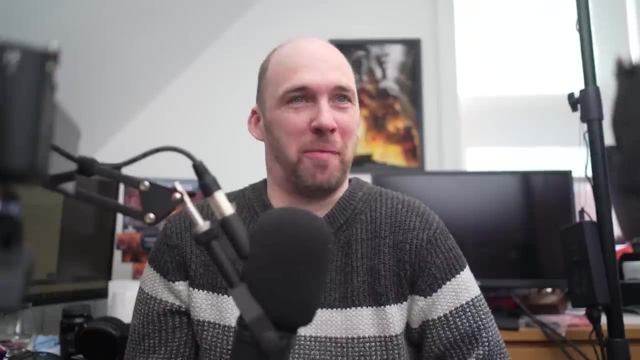 reams and reams of rules. yeah, I mean I've played those games and sometimes it is just like a lot of head scratching, hours of like running through rules and just like, did we play anything? no, we didn't. we just looked at a book for about. so, yeah, I could appreciate that. um, I mean, I've, I've had an. 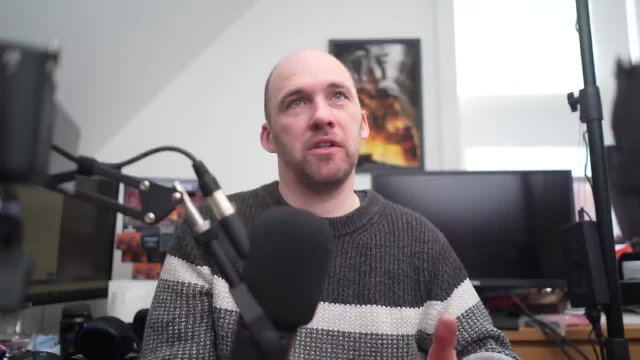 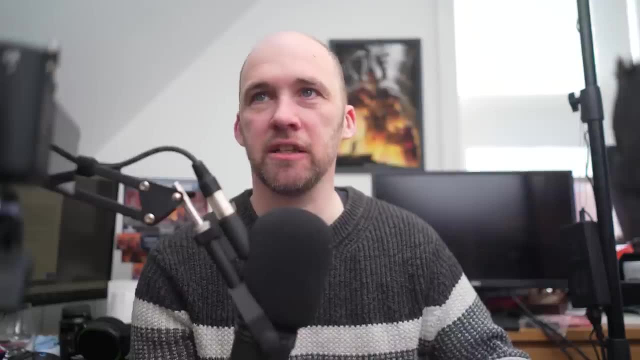 experience with, like, creating rules and stuff like that. I don't know exactly the pitfalls, because you and James talked about this on when we had him on. like you know, you have these things you really love and stuff and then you refer to it as killing your darlings and these things you're. 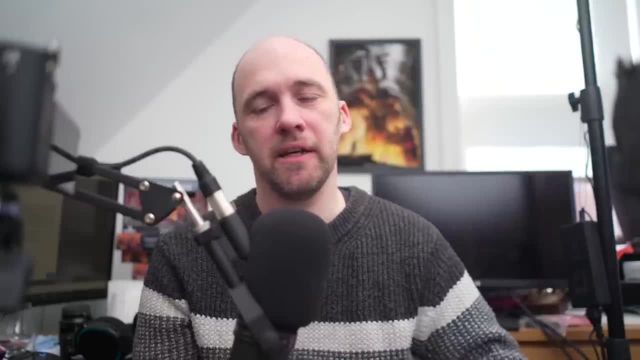 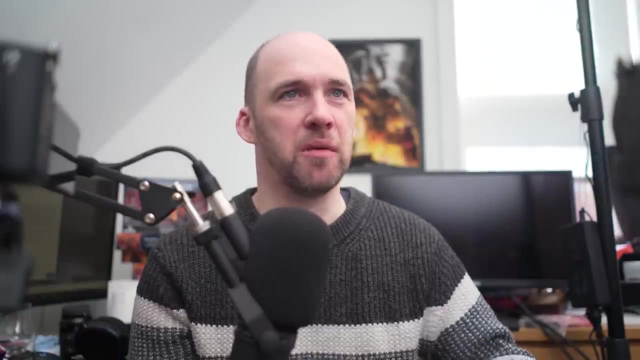 really passionate about that. you have to like: no, it's not working, it's actually holding me back. um, but yeah, just making sure that always at the forefront of your mind. like, imagine you've never played a game in your life, the, the terminology or because workshop did this with one of the. I 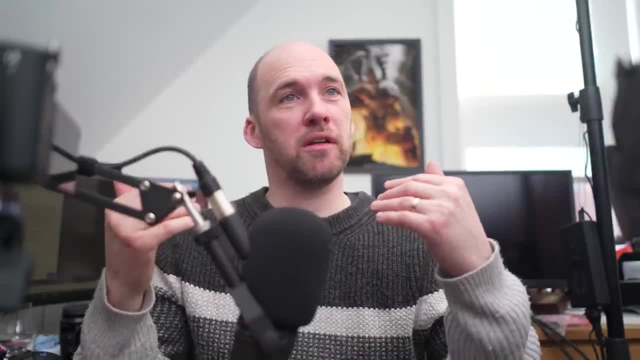 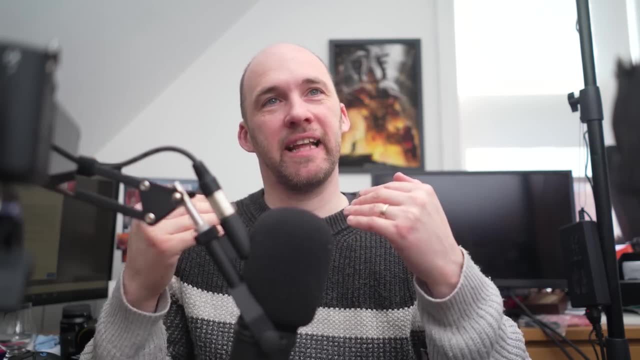 many people was so used to the panic rule in the rule book. no one explained any point in the rule book this, this got caught before it went, obviously to nice. at no point in that rule book did it tell you how to take a panic check. no, it was flagged up by a couple of people. that's what I was talking. 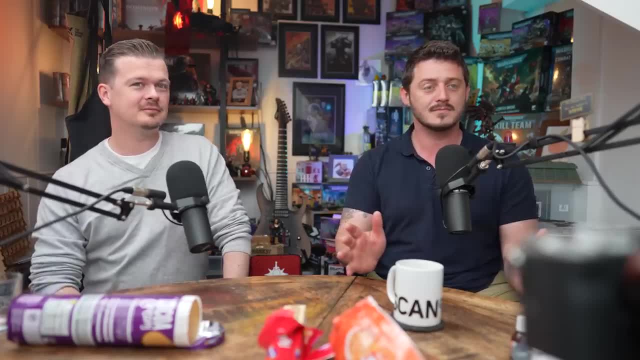 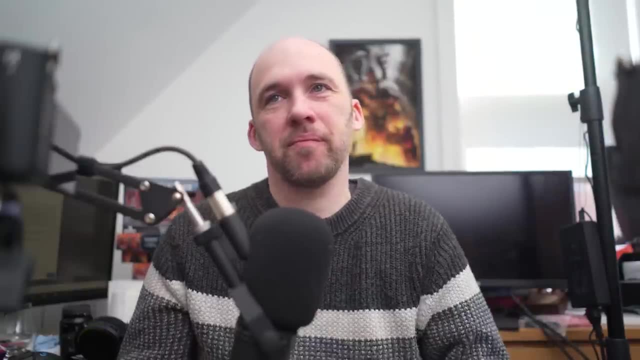 that's what I mentioned, like: oh, people just know how to do that. yeah, yeah, because you talk about like terror and fear and like or psychology, but no point did it tell you how to take the test. well, that was another one. actually you just mentioned you used terror and fear and like psychological. 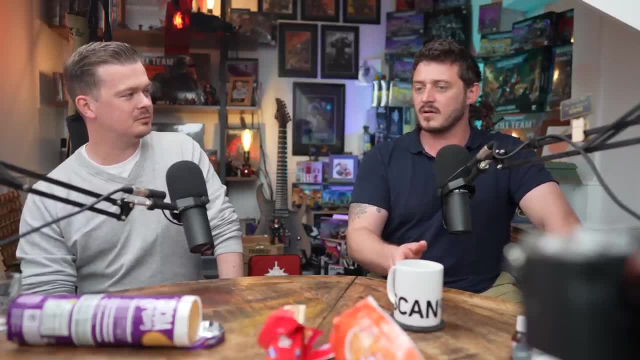 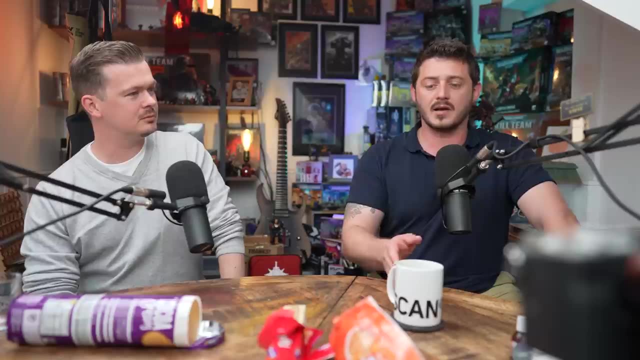 like Warfare, whatever. the one thing I found in the past as well. that was quite confusing to me when I was, when I really started, when it would go through and be like: oh, if it takes damage, remove it from the table, or if it takes damage, it's killed. oh, or it's killed outright or it's died. 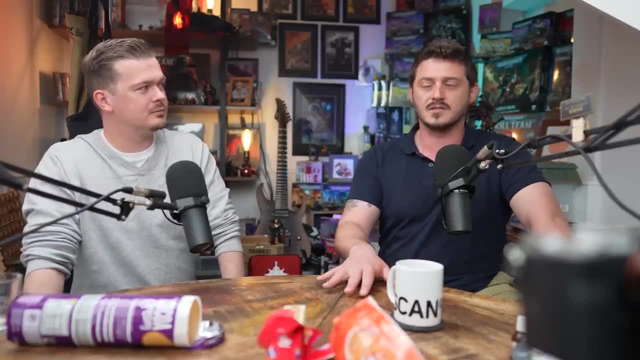 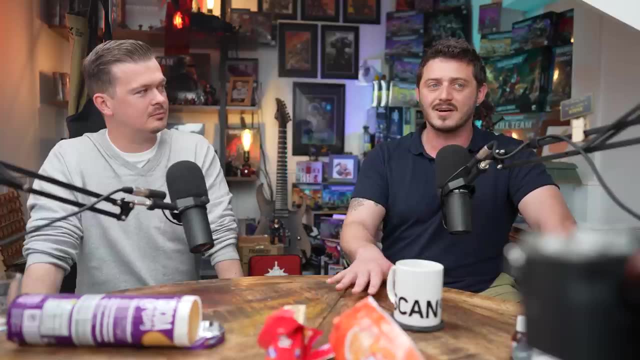 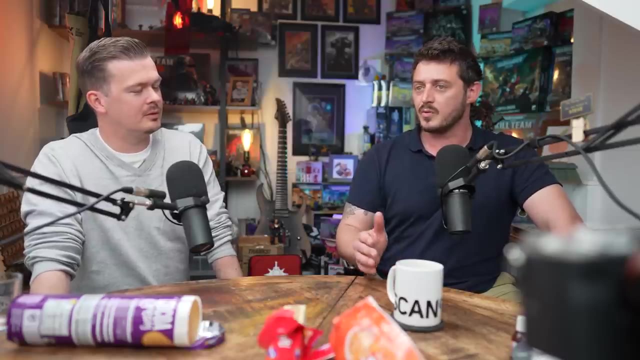 and it's like they've used loads of different words there, like: does died mean the same thing as removing from the table? yeah, or does being obliterated mean the same as died? yeah, and it's like, uh, and then obviously, yeah, they do, but actually that's not clear, so we have used the. 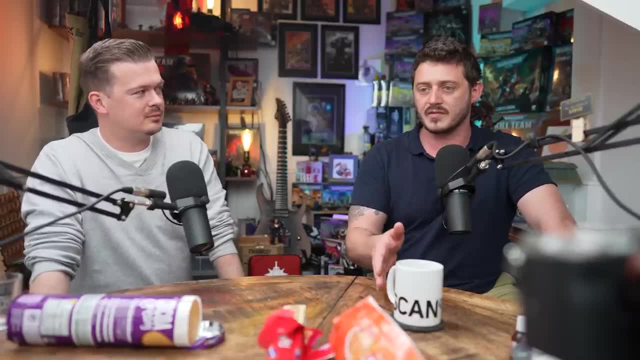 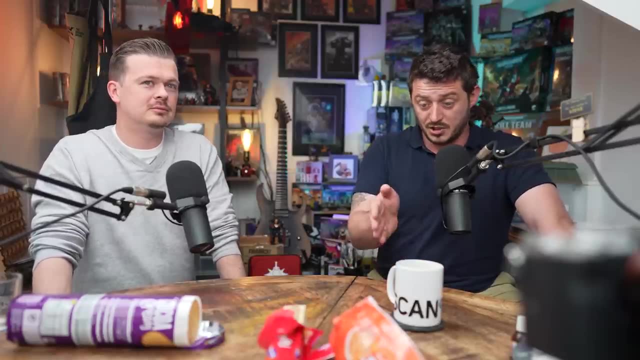 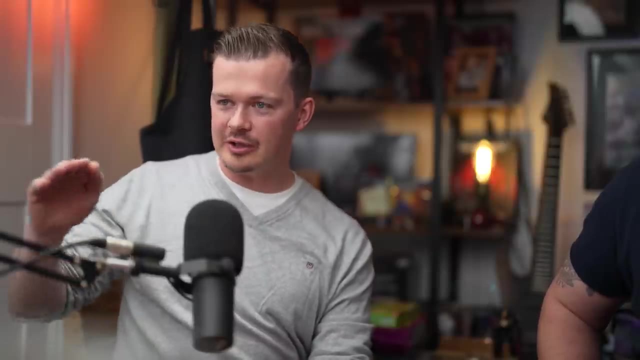 same terminology all the way through: yeah. so every stage we've referred to something as like: well dying, yeah, it's like there's no obliteration, there's no like: yeah, mortal wound, it's just died, it's died. yeah, you know what we're talking about. as simplistic as our rules are the rules as you. 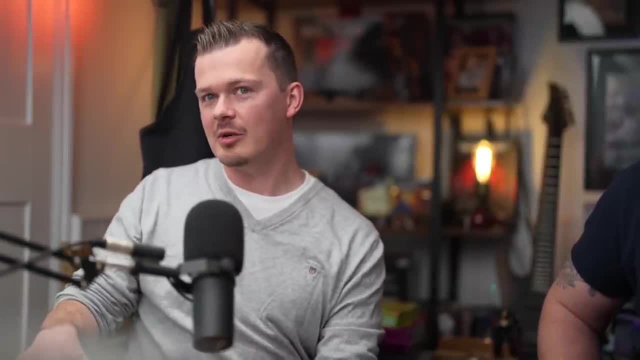 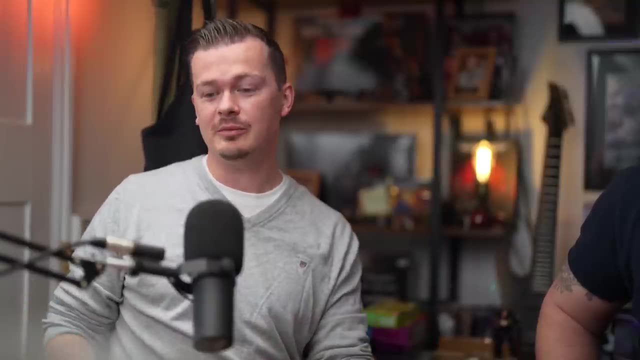 read them it might seem quite wordy. yeah, but we've, we've written it, so there's no ambiguity. yeah, yeah, and there's. there's set phrases, so set words we use are capitalized. yeah and yeah, you'll probably see as you go through. just so, there's no, you read it and you, you know what it means. yeah, yeah, there's. 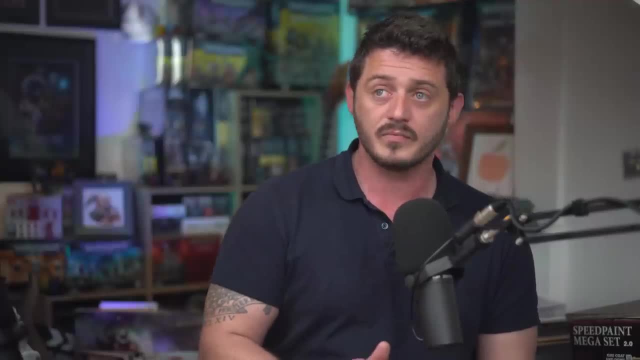 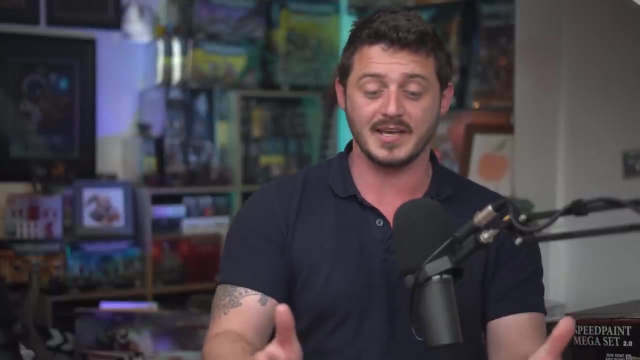 nothing which is annoying, because in person explaining to someone one of the simplest rules in the world- try is two minutes, okay. writing that in a really simplistic format is like two pages is going to be a nuts rule like- oh, this is insane- when actually the attachment rule, like in our game. 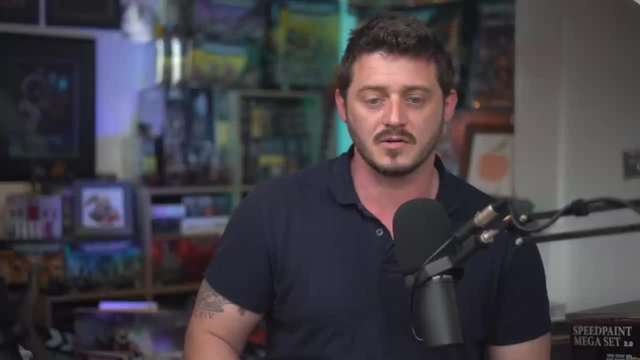 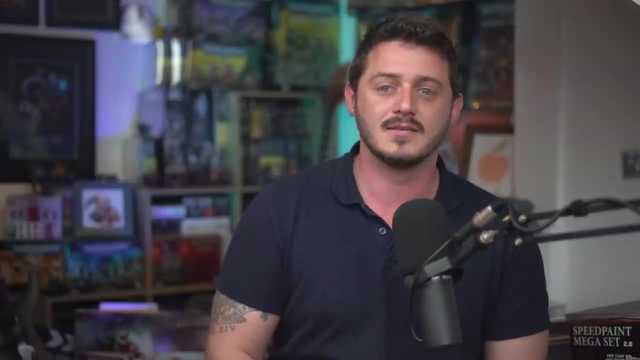 just means that if they're more than two inches apart, they're just two different groups. yeah, and that's all it is. if they're not and they, they share a same type, they're one group. oh, I'll get that. you write that down. yeah, you write it to explain it. so it's not ambiguous, it's horrendous. 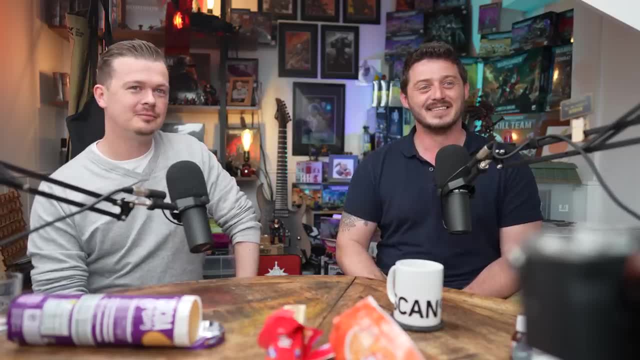 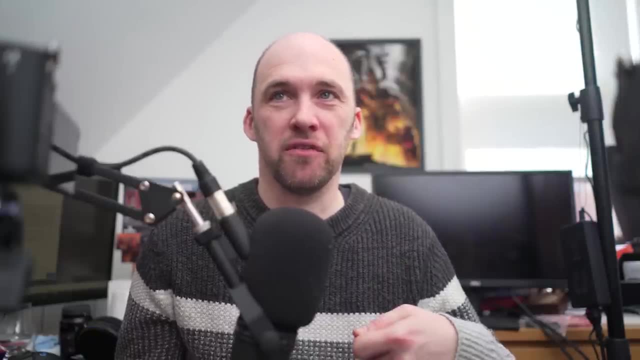 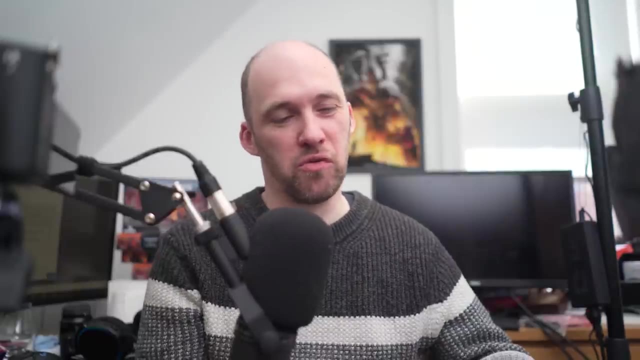 simple technique but putting that into words for people to understand is so difficult and has to be explained in such a way that there's no sort of like room forever of people like removing too much paint or not removing enough and yeah, how it should look on the model. it's just like so for something. 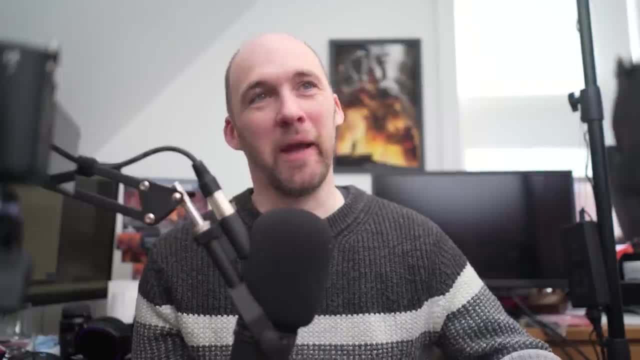 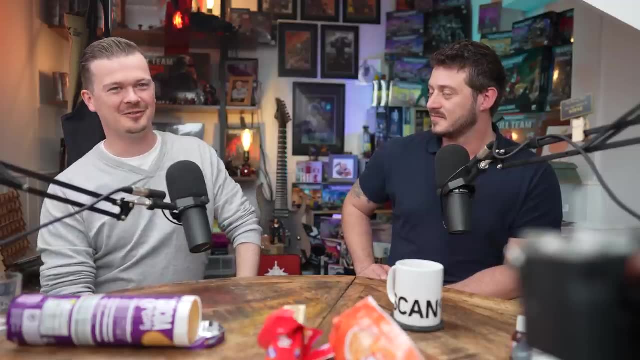 if you sat next to someone and showed them, they'd be like, oh, that's dead simple in words, it's like really hard, yeah. so, yeah, totally get that. yeah, that took us. yeah, it took us a long time to get that together, right, so we've talked a lot about, um, well, I guess, the miniatures and and and some. 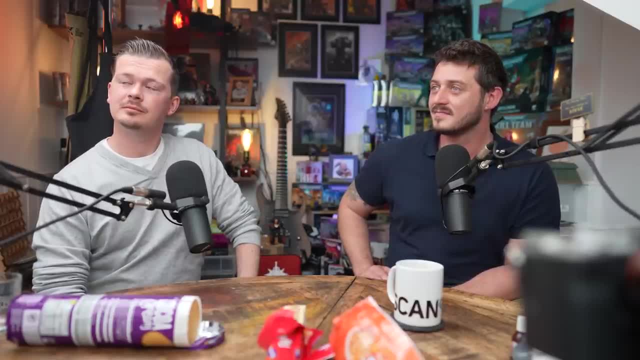 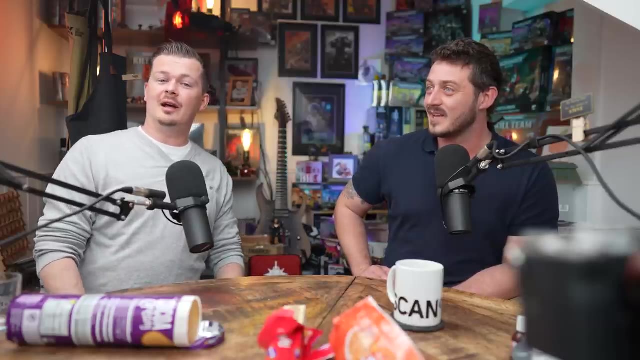 of the rules. what fascinates me is is how you get from taking it out of your minds onto paper into the finished product that that goes on Kickstarter. so I guess, getting all the cards, printing all the miniatures, designing them, did you do that yourselves? we, who you see here, is just: is everything war and terror? is there's? no, there's. 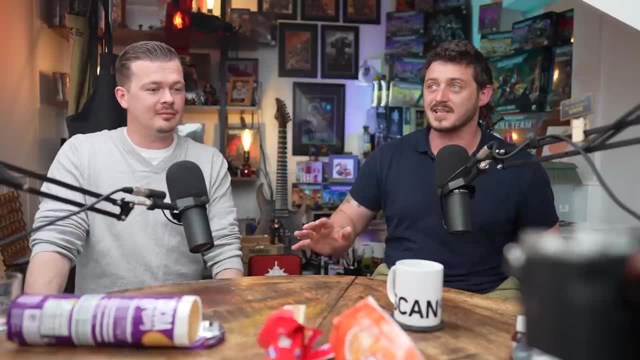 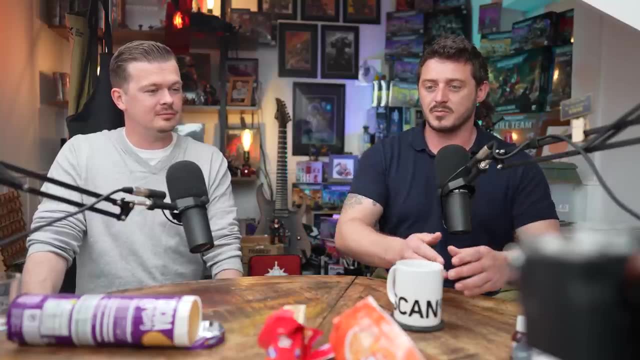 no extra people, yeah, it's just other than a couple of mates to help play test sometimes. yeah, yeah, um, just because sometimes, if we play test too much between us, we might think, oh, we'll rule like this and we'll write it like this. and actually because we're now getting so used to it. 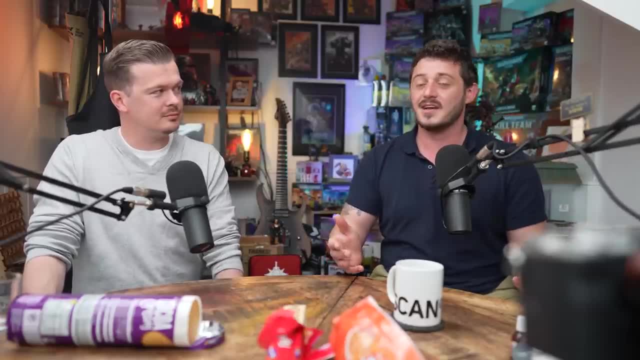 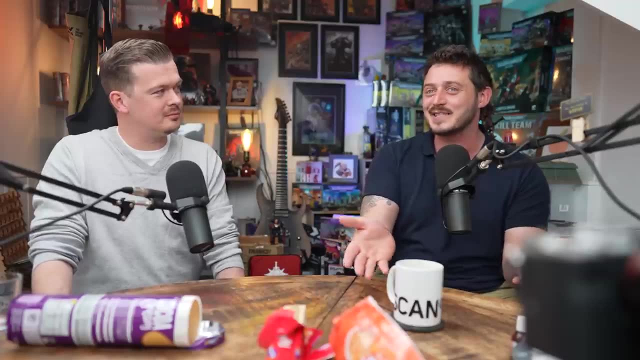 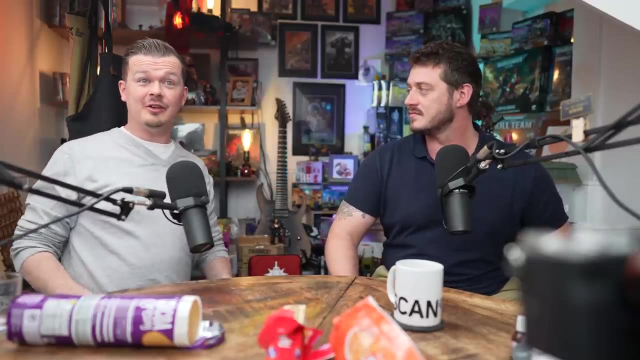 that we might miss. yeah, yeah, yeah, oh. we just know what that means. let's bring in some fresh eyes. let's like grab my mate, Jason, and be like, do this. it's like read this, how does this read? it's like go be our guinea pig, but no, yeah, it's just us. it started from, it started for nothing. we had the. 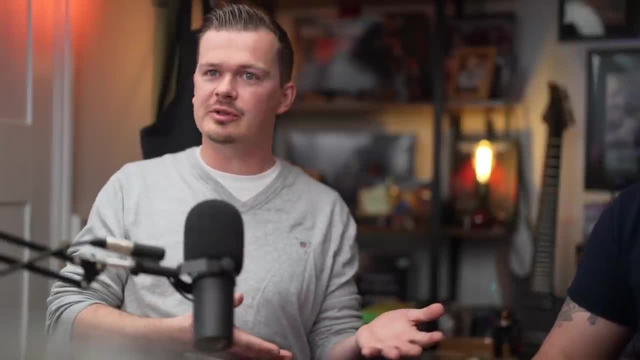 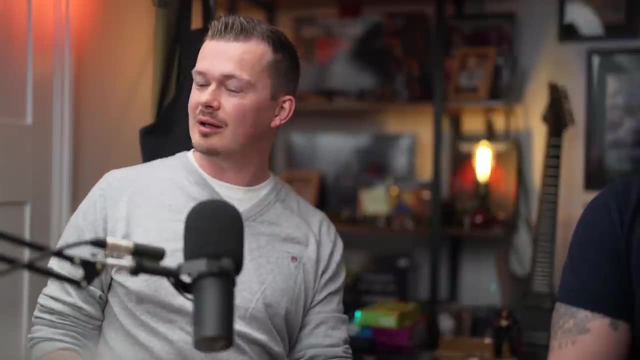 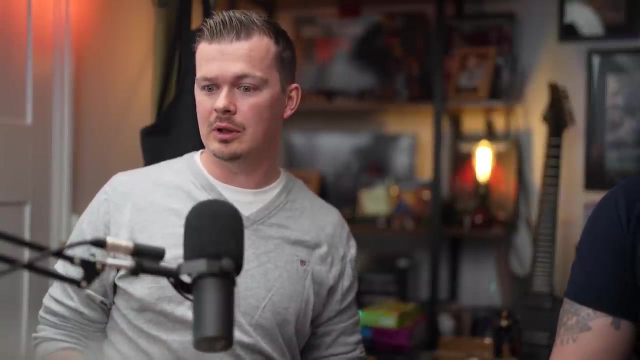 idea. uh, I met Will through work and then knew that he was into model and it just it came up to use you. just you'd assume you needed yeah, um, because obviously what we've got a, we've either got hand sculpts or we've got 3D model these. so, um, what looks like we're going to learn how to 3D. 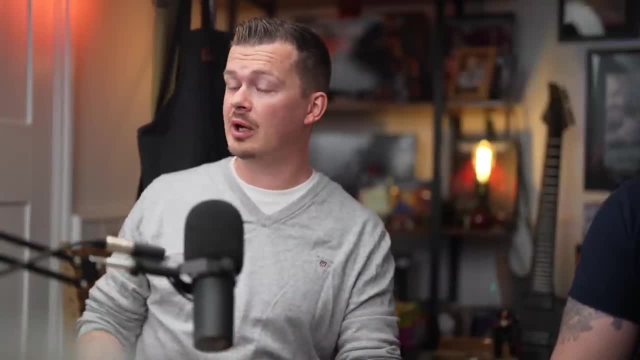 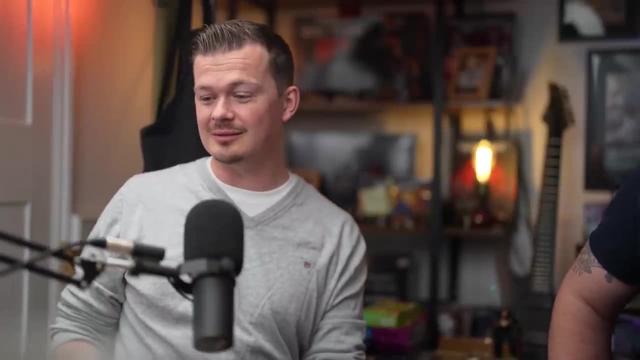 model. so you go online, then you find a software like blender, which is, yeah, open source, yeah, and there's a steep learning curve. yeah, but you, you find, yeah, you find your way through it. and then did you like make a donut? that's the famous tutorial. no, I never have done. no, this I, I haven't. 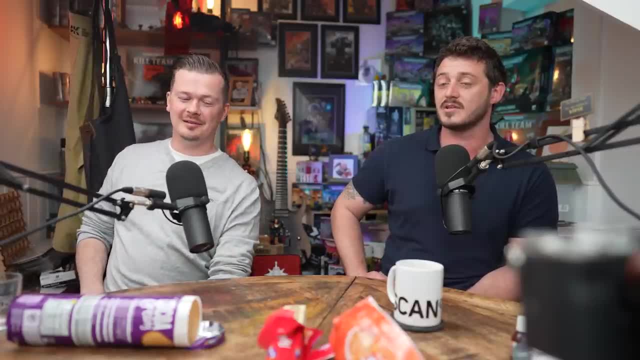 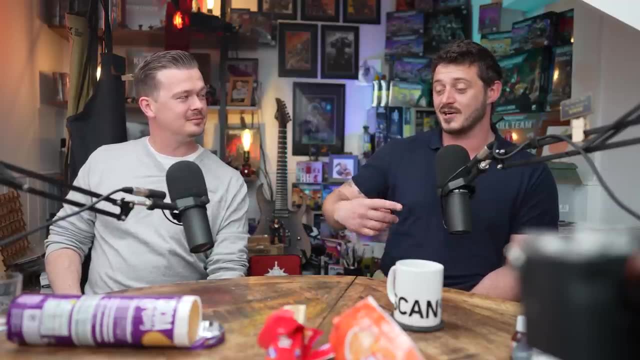 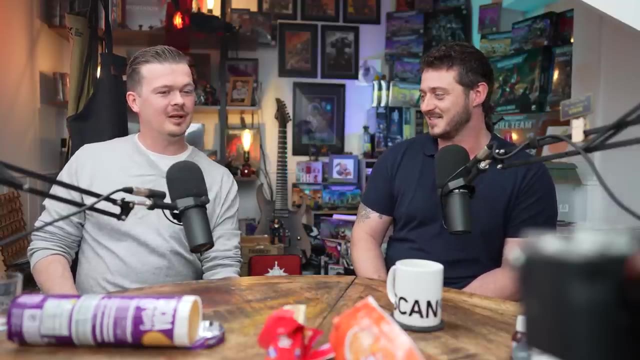 I, I just I just watched a lot of five minute tutorials on. this is how to connect two vertices together. this is how to Union two shapes. this is how- and eventually, over time, it just this is how you decimate a model without losing like detail, and it's like that's where I've been going wrong. yeah, I haven't, but I know. 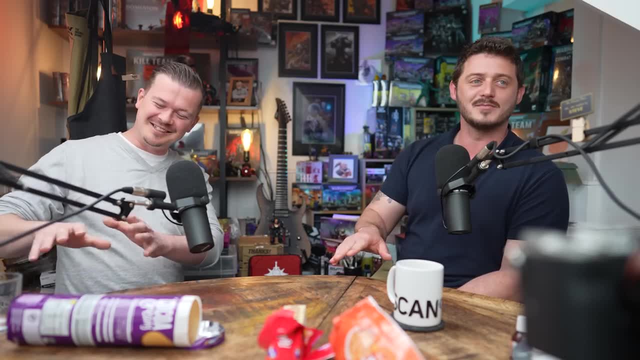 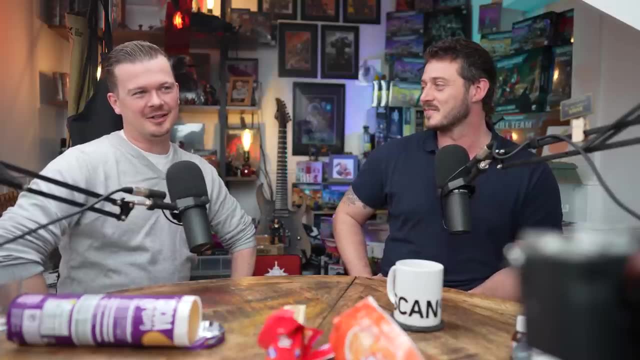 the exact video. yeah, everyone knows that. don't that glaze? yeah, yeah, if you type in how to and blender: yeah, here's a donut. yeah, yeah, what we might have to do. I don't know if we want it popped into the to the video or anything. I'll send you some shots of the first, because you've 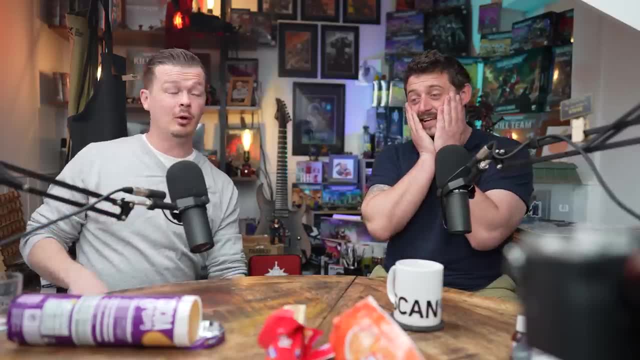 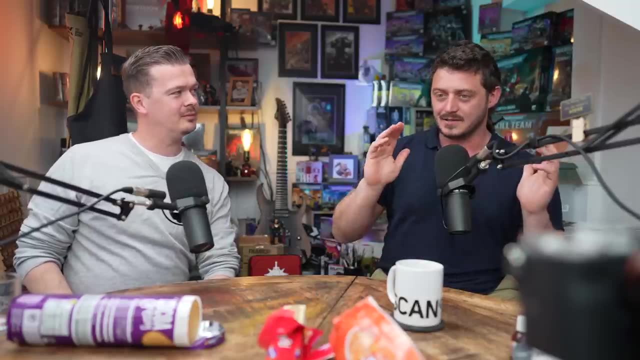 seen the Marines- yeah, the first one I ever came- horrendous, it's horrendous. we were happy with it. we were, we were willing to roll with it. we were like: this is the best thing ever. let's go, yeah, let's not. so what changed your mind then? what was it that made you just going to go? 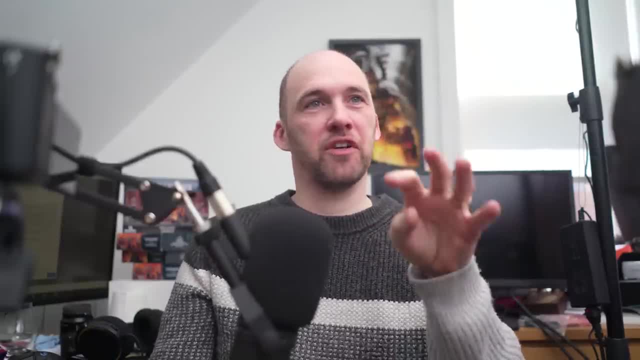 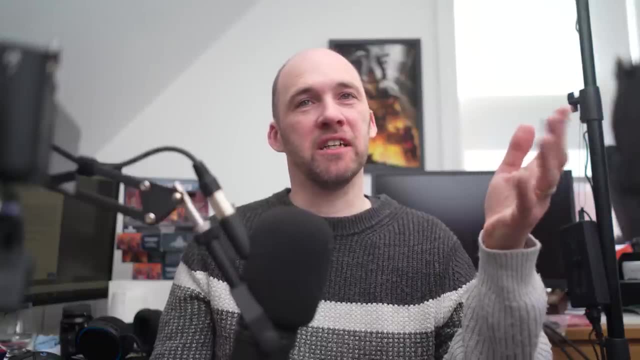 because I've done this, where I've, like I've, I've done a paint job or I've done a conversion. I've gone to work. I've come back the next day it's looked at my desk and what a pile of dog poop- I think it was shoulder pads it was. yeah, I mean, we had shoulder pads. so, yeah, we came up with that. 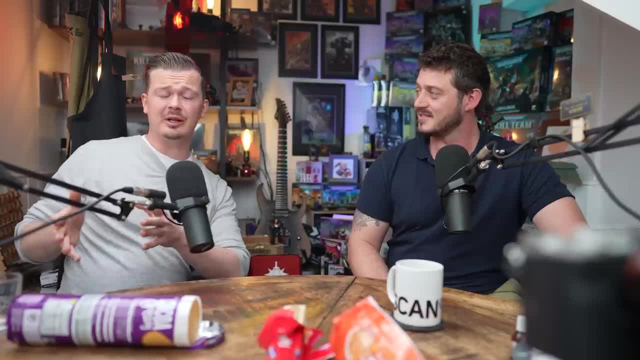 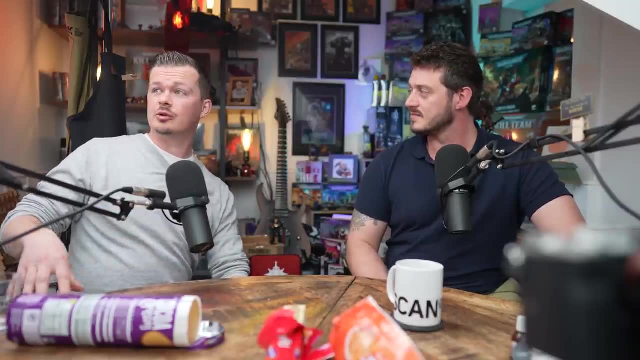 as a basic idea. and then I thought, well, because sometimes when you're focusing on one thing- yeah, it's tedious so often you've got two or three different models on the go, so you can- just you can- chop and change. so I thought, oh well, we'll do a different, we'll do a different model, it's. 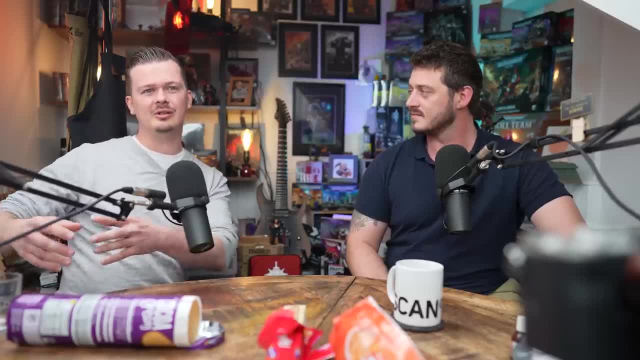 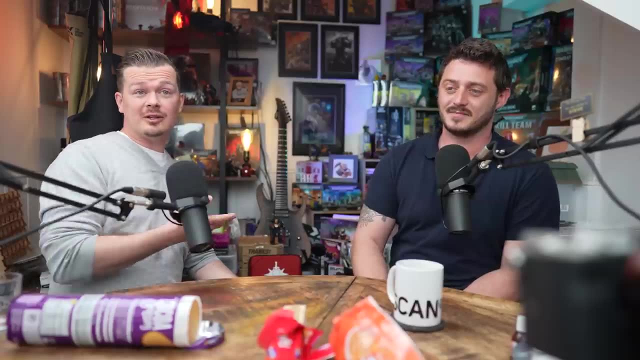 going to have a slightly different armor. and then, in discovering how you'd- oh, I want it to look like that, and then you watch a video and you think, oh, that looks great. oh, that'd be something that's so much better than the like our bogster, because, like I'm going to keep arcing back, but a space. 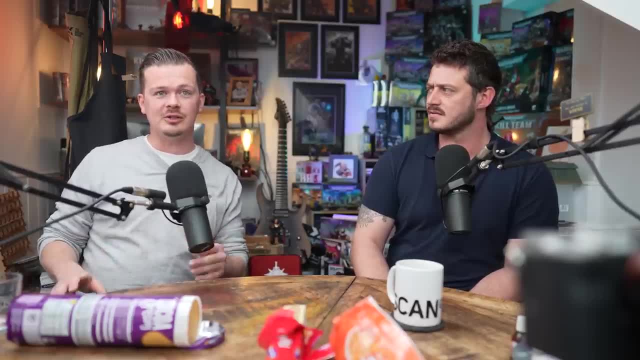 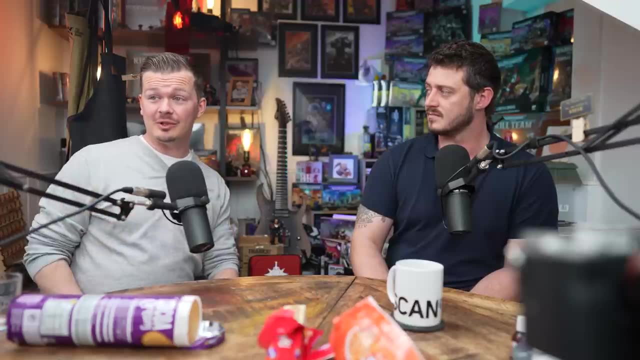 marine is and always will be iconic. yeah, yeah, yeah, it's designed so we knew that, even though it's a basic troop, it has to be. yeah, yeah. so yeah, I mean, don't I mean that the design, you see, there was probably our. I mean that that shape was pretty much the second one that we- yeah, it was actually. 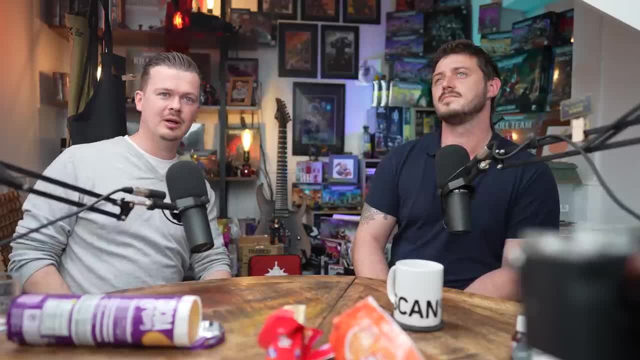 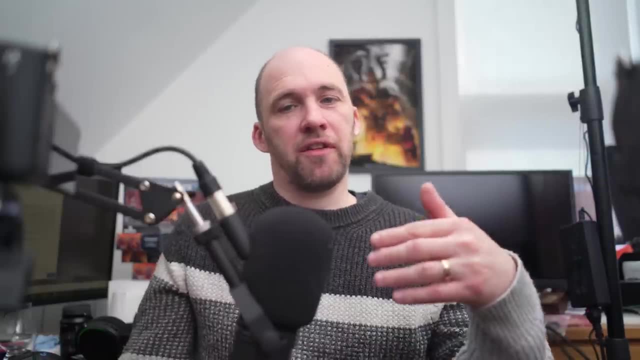 yeah. so I mean we're quite lucky. that's not to say there's been other models where we've- yeah, I've- tried 20 different designs and they've been so from being in an arts background- because I was at college and union did lots of art- one of the things you 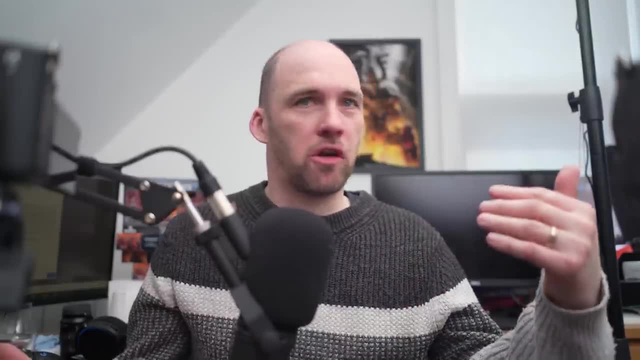 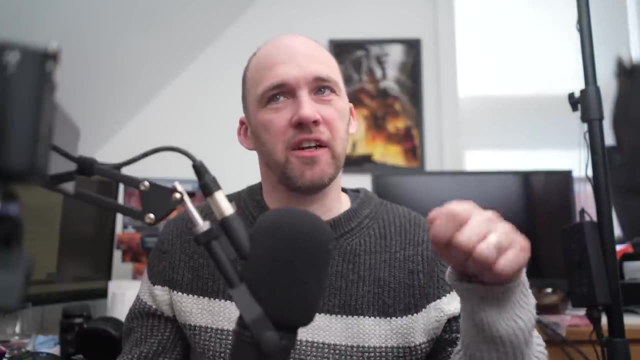 always push to do. is you like right what you want to do? we're doing the concept in today. we're going to concept, like I don't know, a start, a body work for a car or something like that. you sit there and you sketch the best car design you can think of, but what you're encouraged to do is do 20. 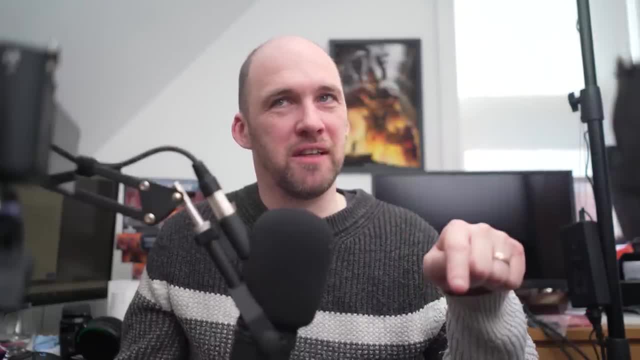 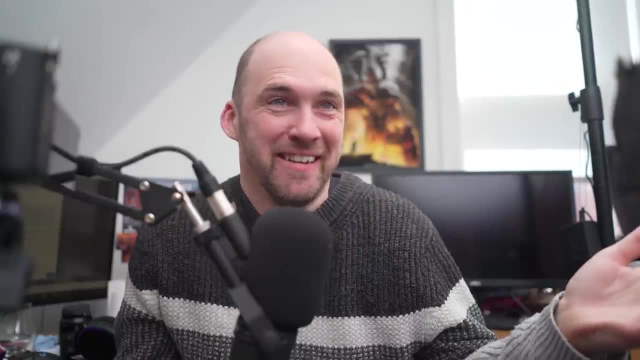 so, even though you're like hooked on the first one, you have to like still do 20 more just in case there's a better one or a more refined one. and it might just be the first one you did was fine, yeah, and obviously the second one you did was the one you settled on. 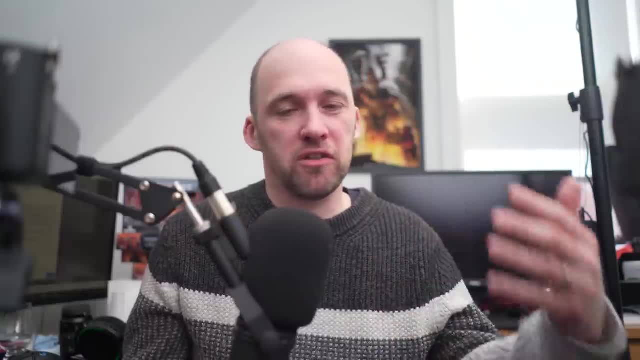 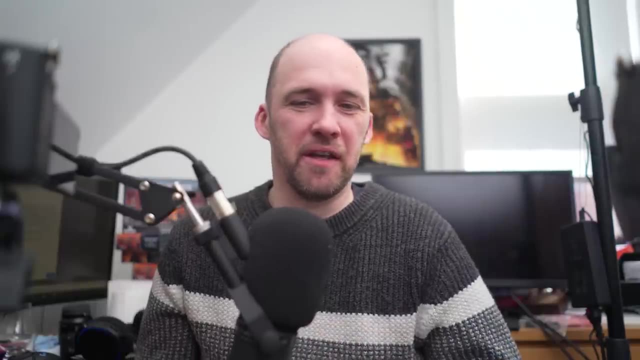 but I always remember that from like college was like when I was like doing stuff for work or like colour schemes, like for arm and stuff, I'd always like do five or six more just in case I'd find like a better sort of like well, style or where I position the colour and stuff. but if you know you 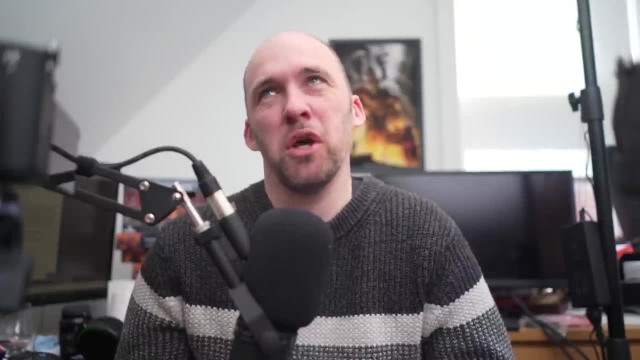 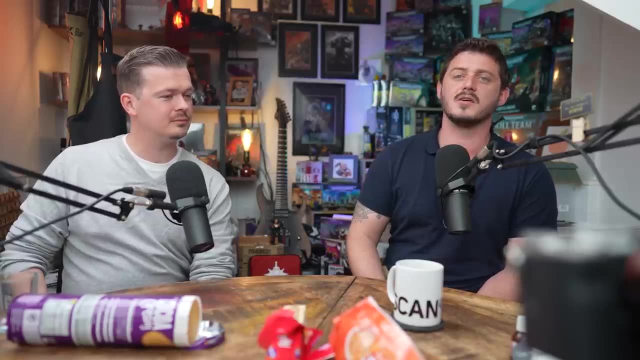 know, don't you? it's like the style you're just like. this is fine, I'll do it for for the teacher. I'd find a spare 20 minutes at work and we'd be struggling on something and an idea would come into my head. it's the old: always keep a notepad by the side of your bed, kind of thing, just in case you. 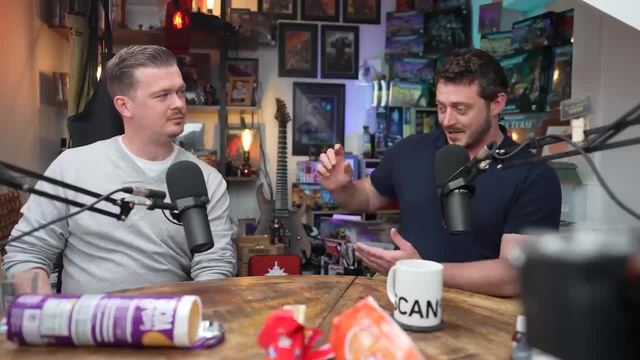 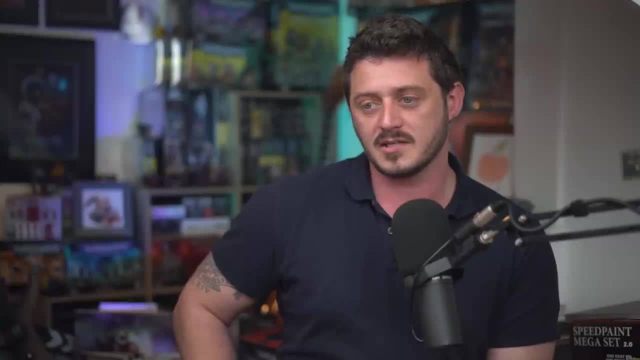 you wake up in a hot sweat and you're like i've dreamt of the idea and you just go straight back to bed. um, yeah, i'd find a spare 20 minutes and alex would have messaged me going. i just can't get this. this leg armor, these legs. i've looked at the legs for too long today and it's just like: oh, 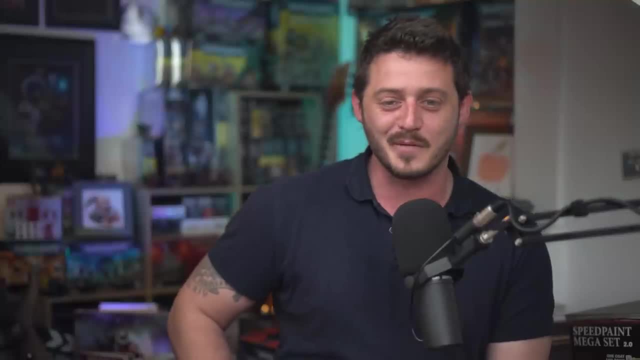 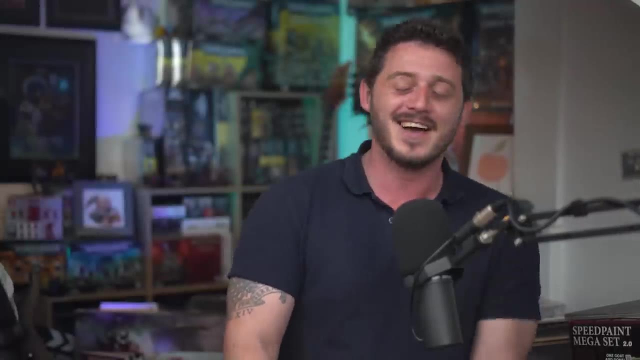 a human butt, just like what do i do for butt padding? like, how do we make their bums look? it's like what? yeah, it still looks like it's wearing a nappy. we need to try and address this. so i just get a piece of paper and a pen and i just sketch a shape. um, because i'm not the best, but i'm okay. 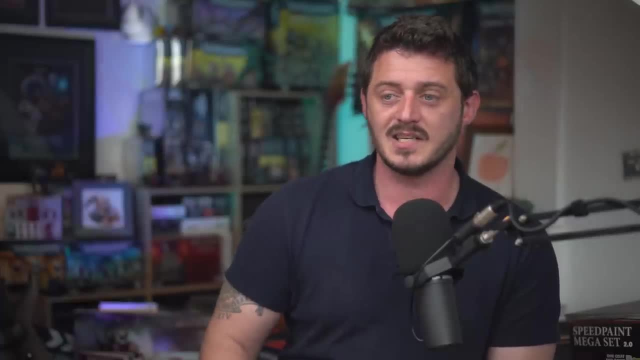 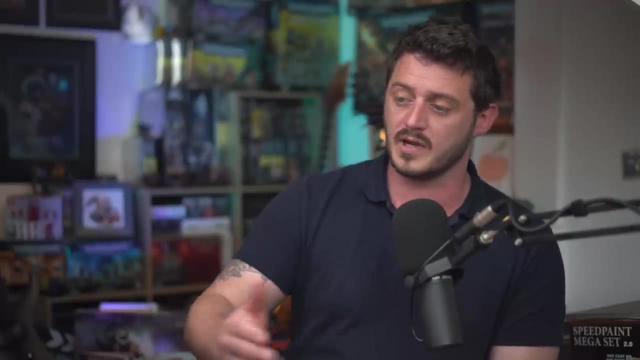 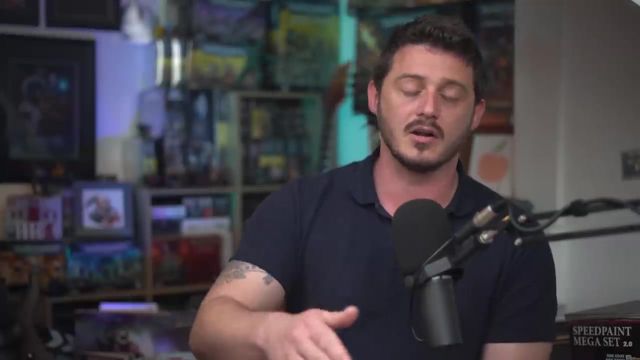 putting some shapes together and i'll just take a picture, send it to alex and he'd be like: uh, uh, oh, actually, yeah, yeah, and sometimes what he'd come back with would be nothing like what i sketched, but it's that. but the shape might be like: okay, i've got an idea now and that would help, and a 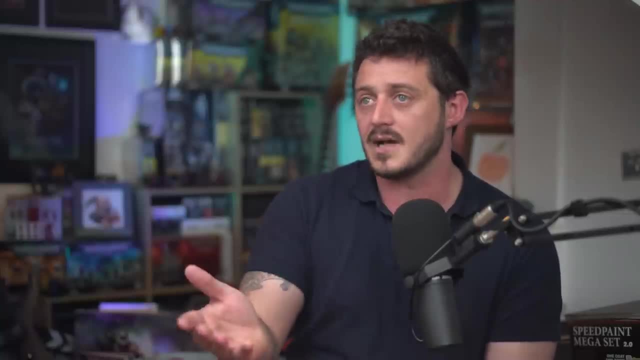 lot of time. it's just again working through it. yeah, like, yeah. so, as you ask, like, how where do we start? i had no idea. you, you chat to me seven, eight years ago and tell me i was able to design a model on blender, like 3d, model it and then print it and actually have it as a physical thing. i'd. 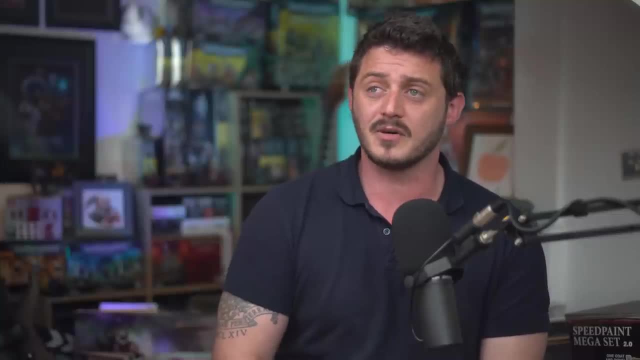 laugh. i just i'd be like: there's no way, i'm, that's not me. i haven't got any qualifications, i've got. no, i just i wouldn't. where do i start with that? yeah, and and even then, like alex came to work one day and opened up his laptop and he threw some shapes together on this wacky program that he 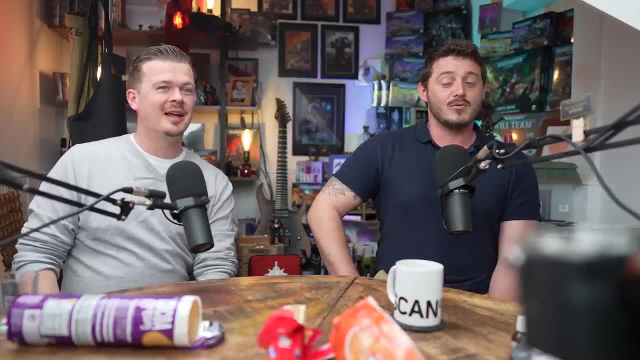 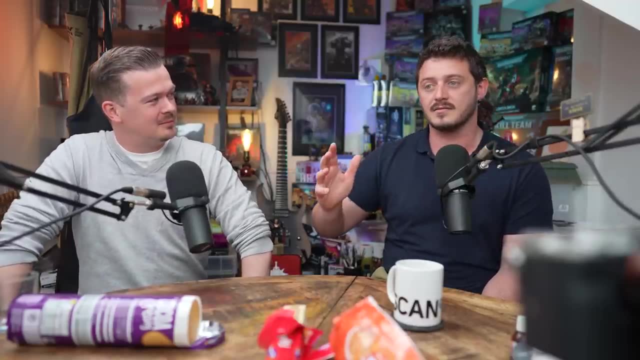 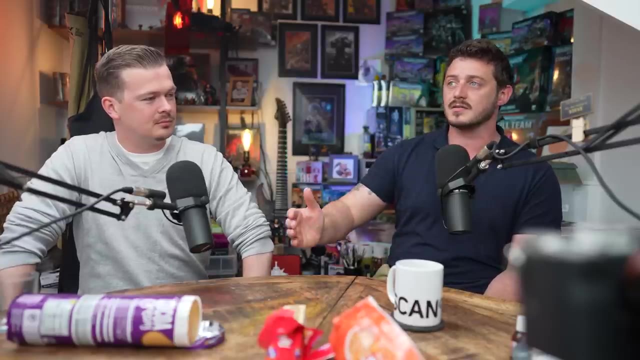 got for free. i just imagine you two dancing at work throwing some wacky shapes. i couldn't believe it and even then, knowing that alex hadn't had a background in 3d modeling, even then my brain was just like, oh, i'd never be able to do that. and it took me months to get over, like 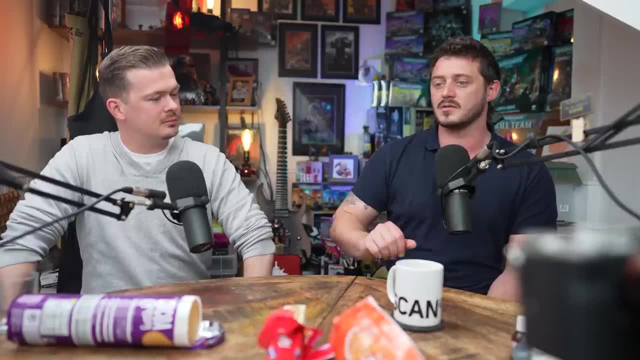 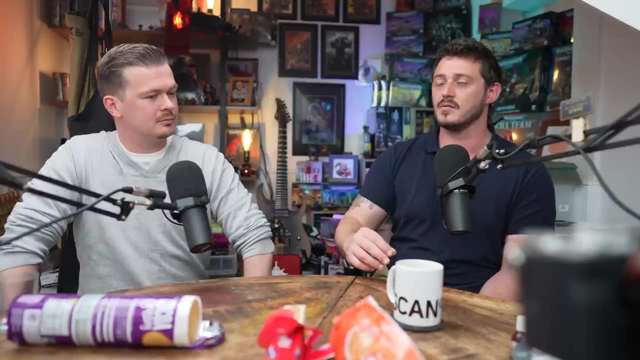 to get to the point of seeing something alex had worked on and being like i- i think i can change that- so i forced myself to download it, get the file, how to play and thought, oh no, i can do this, yeah. and then i was like, oh my god, i can't do this. 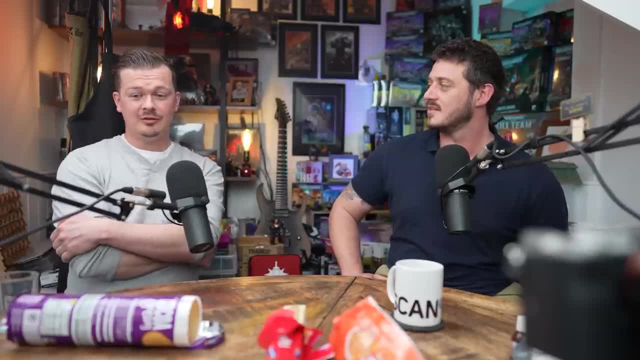 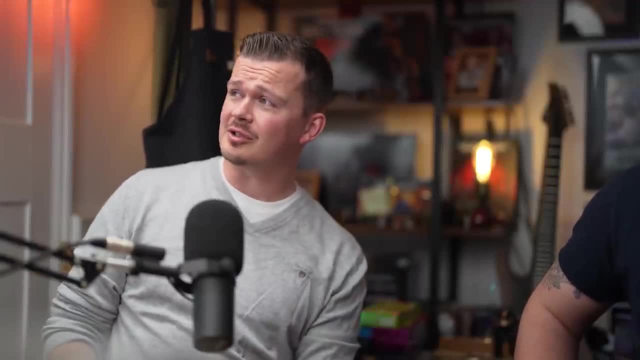 absolutely i can do this and it just went from there. yeah, the great, the greatest thing is just just start doing it. yeah, like if you want to say to anyone that wants to do it, just start. the internet's such a wonderful tool. yeah, i mean we use. yeah, so we use blender for the. 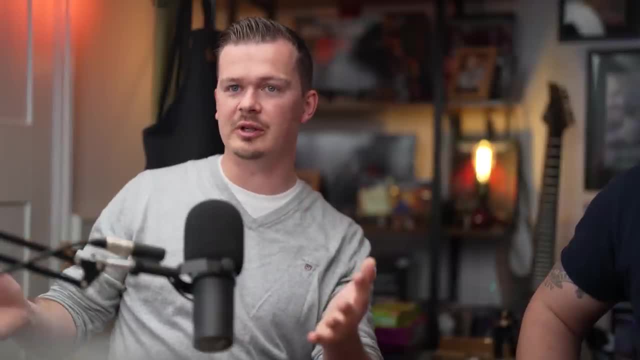 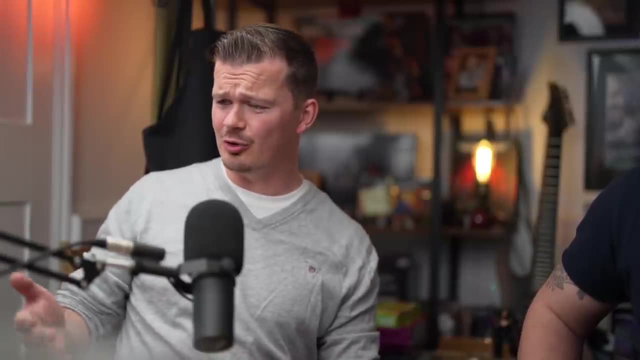 modeling: um, obviously, we've built this world on the website, which, again, is just done through wix, so there's no html coding. all the graphic designs, um, i use a unfortunately named program called gimp, which is: yeah, basically. yeah, he's an open. i wanted to know you were going to bring that. 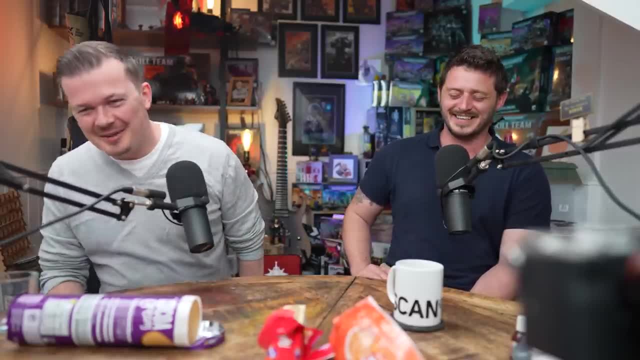 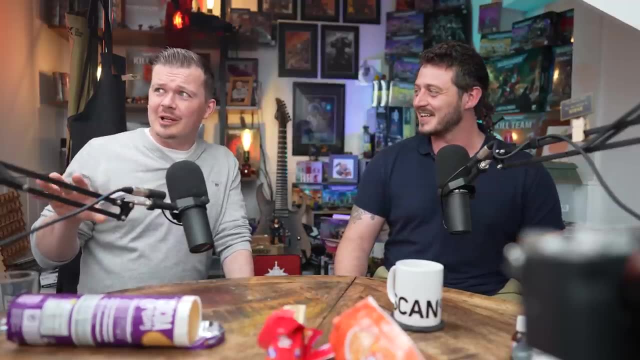 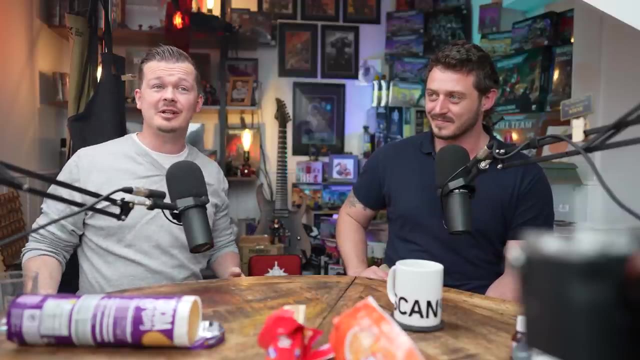 i didn't just want to lay the word out there randomly with no content. i i am familiar with gimp, yeah, aren't we all? but just before that comment gets, before that comment gets lost, that's an open source photoshop. yeah, for people that don't know, um, so again, all this stuff's. 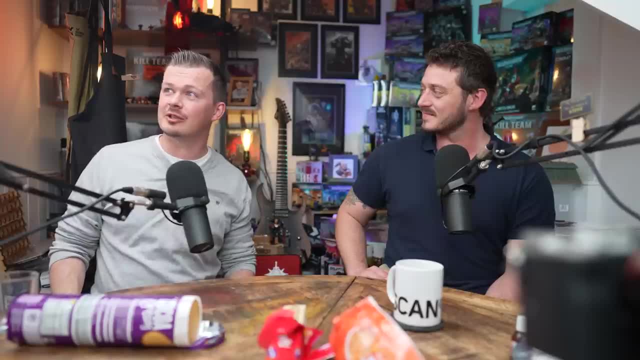 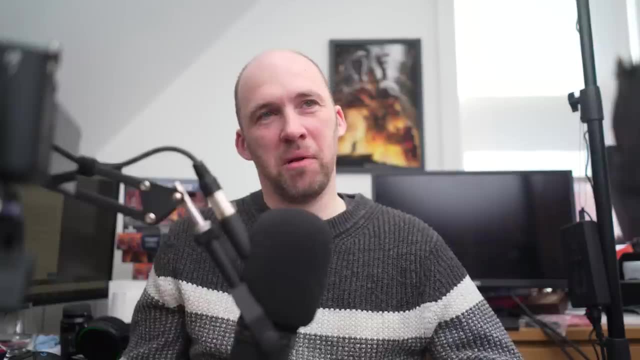 available out there for free and and then it's really it's on yourself. but again, you've got youtube and there's- yeah, there's nothing you can't learn to do, yeah, from youtube. can you tell me when you're in the office, just please? at one point did one of you say: bring out the game. 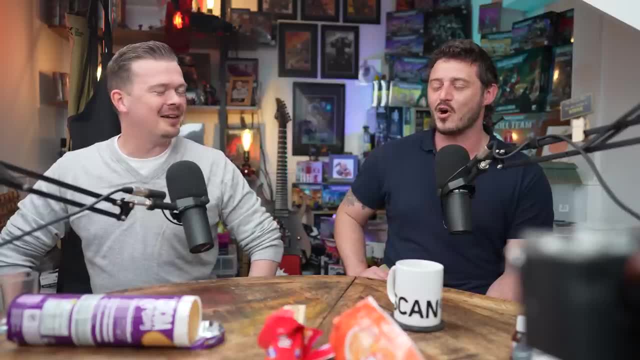 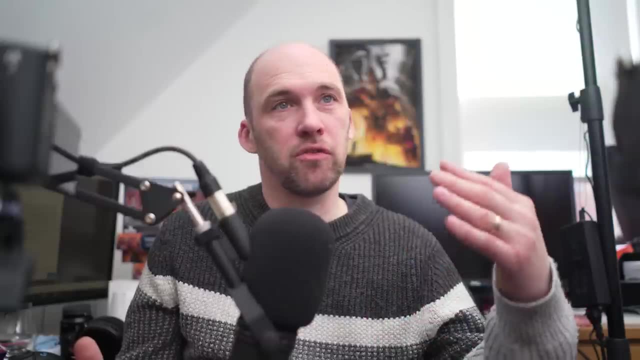 did anyone at any point say that i think we've got it on it? yeah sure you gotta do it. uh, so i mean, i've looked at the website. i really like it. um, i love your shots of all the different factions and all the different units and stuff and you've got like little army shots of like the stuff that. 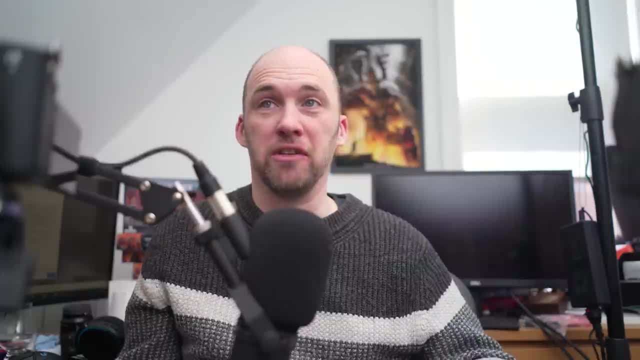 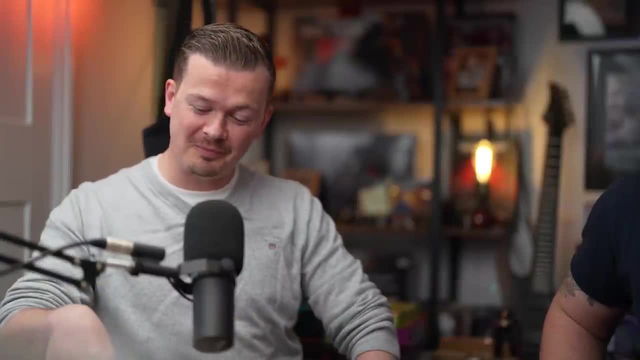 comes in the box with the humans. the tank's amazing. i'm not built with a tank yet i need to get on and do it. i looked at the tank saving you for the end. we've had- yeah, we've had had- a lot of love for the tank. again, coming back to something you said earlier: um, things that people 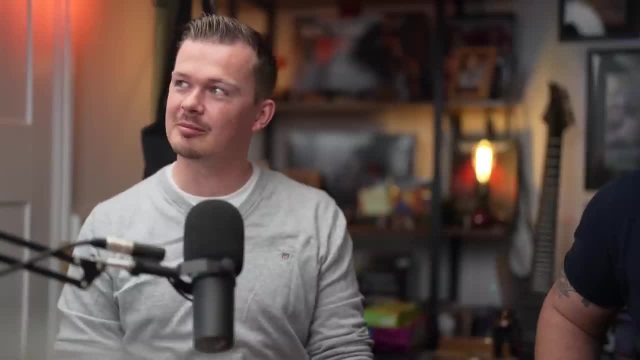 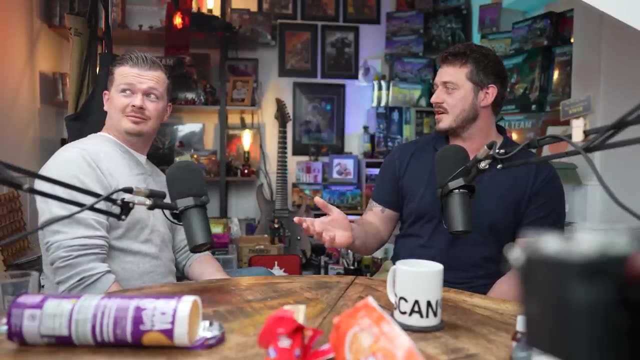 said it looks like we've got because you've got the scorpion uh tank from from hayley's. yeah, because it's like got the four like quarter tracks. yeah, you've got the mammoth tank, there's another one. yeah, as soon as you add four tracks, though, it immediately looks like everything else. 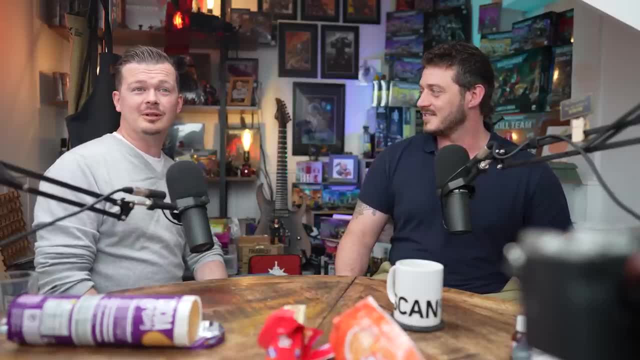 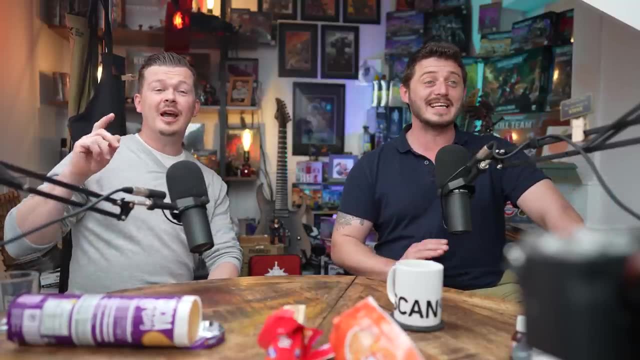 with four tracks, yeah, yeah, you know. the best one, though, was the um. some say it looked like the tank from thundercats. it's been a long time. you might have to immediately google that. the front of it's basically like a cat lying down. yeah, the front two tracks are the arms and it's 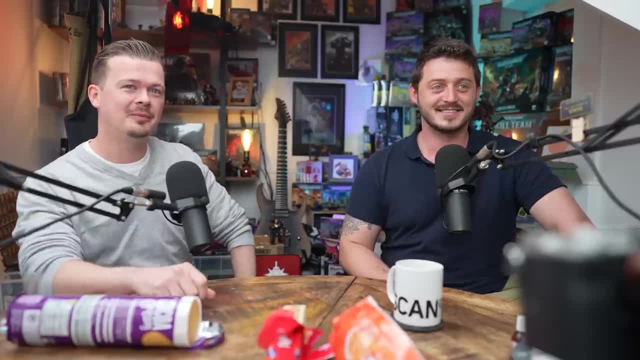 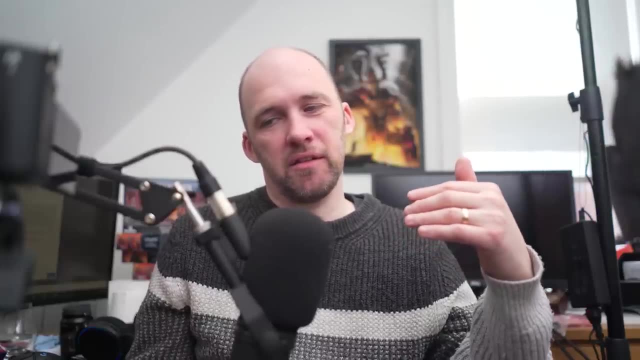 got the head, so not exactly like: yeah, i can see where. yeah, but then it's like anything we said on uh- that, i think, was when we're talking to barb, or one of the recent chats we were doing- it's like there comes a point where there is no sort of super brand new design, because it's only 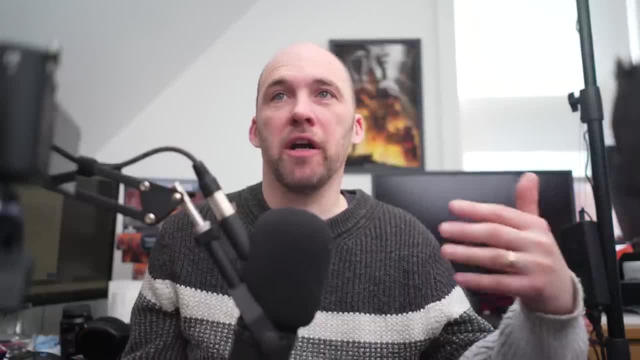 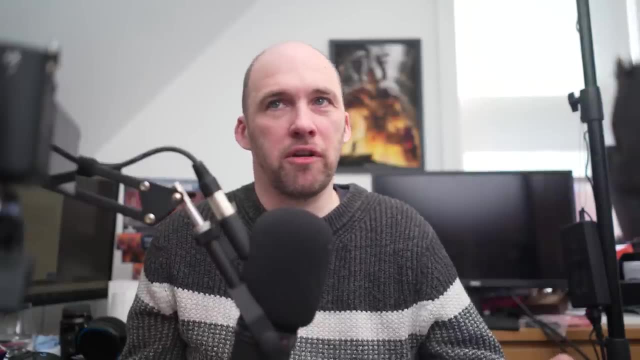 so much that you can, and a lot of things are inspired by other things and then tweaked and changed. um, you know like 40k, for instance, that you know a lot of like the human element are just like napoleonics thrown into the future. yeah, we're given laser guns and just made splendid. 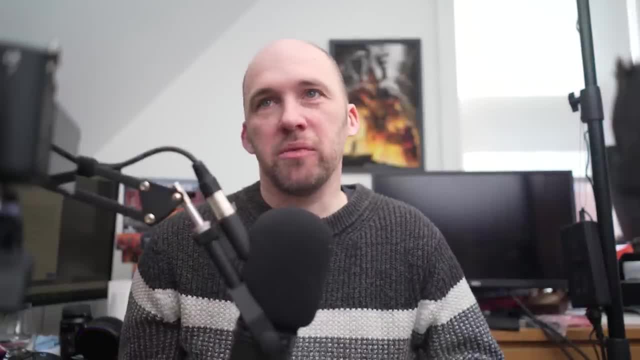 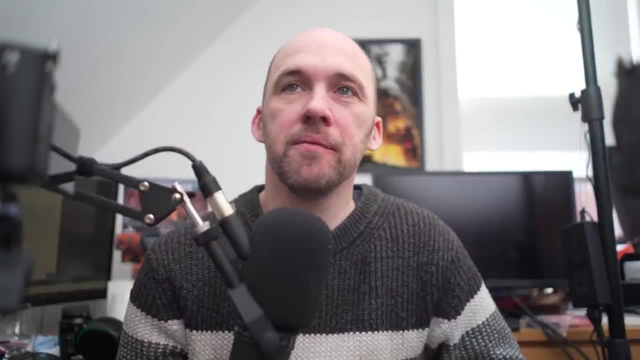 outfits slightly tweaked. but you know, trying to make something super alien, you need to be alien to be able to make something. yeah, there's a couple of things that i've always. well, there's one aspect to designing the greys that we knew from the start and it was a little bit about us. 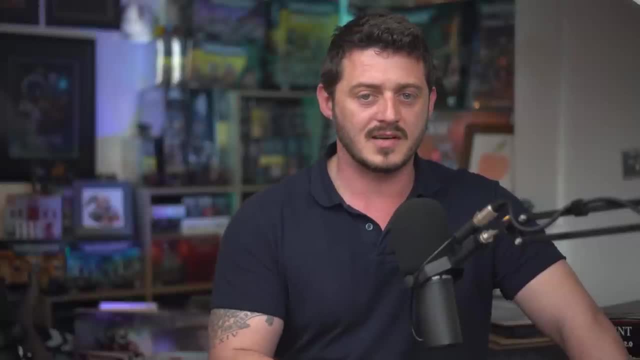 knowing a lot about sci-fi. but before i get onto that, one thing i found really funny is i love going through all these like: oh, it looks like this reference. yeah, yeah, i've never played x-con- i never. it wasn't until people started bringing it up i was like let's start looking into this. 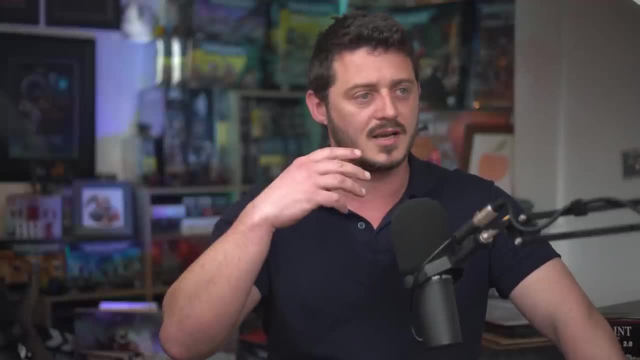 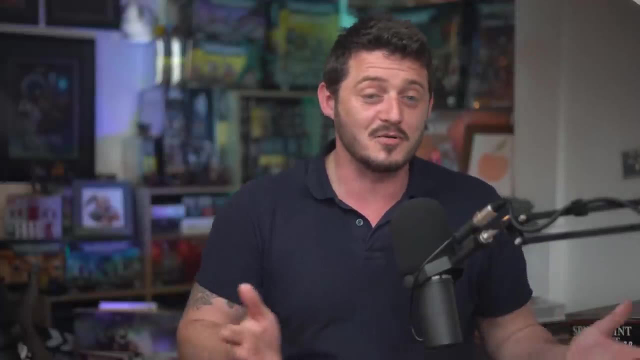 um, same as the? um, the human visor. um, i even had a friend bring it up, uh, that it looks like. was it destiny? yeah, yeah, yeah, never played destiny, yeah, same. so i, i didn't know. it's like it does really look like that. no idea, because we had a we wanted. 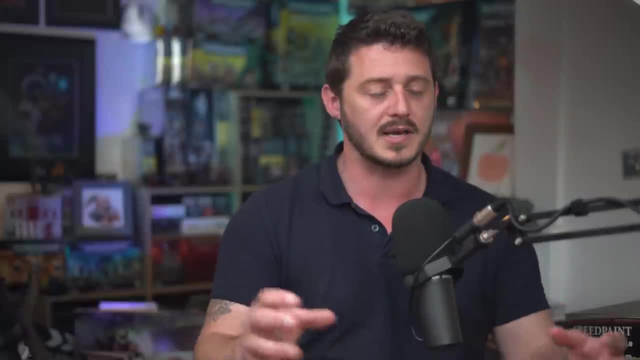 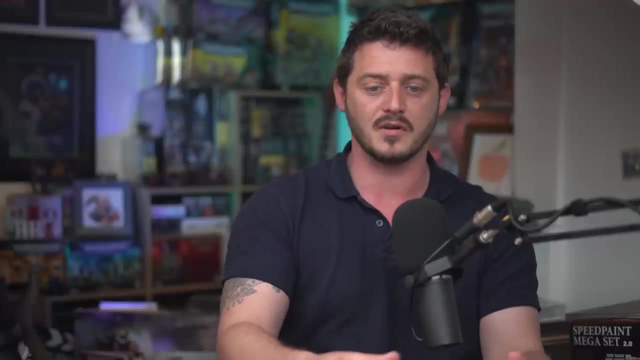 to make the greys look different. but we always wanted- we wanted to tie back to that roswell. we wanted sci-fi based in reality kind of thing. so and the roswell style gray was a great one to go for because it was like everything we could do for them. it's kind of already written, yeah, and 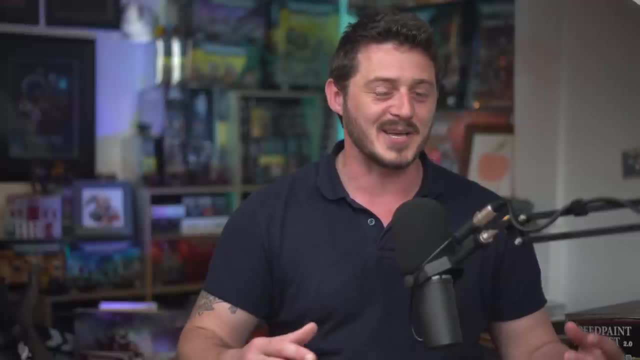 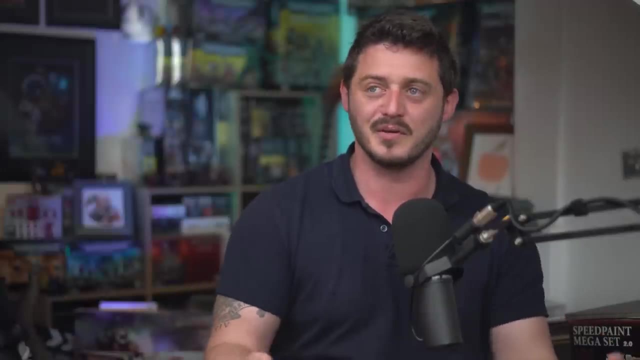 we could borrow from the conspiracy theories and everything about it. there's their, their um, their vocals or their speech works through vibrations, which is great, because you put sand on a film and put a vibration into it, it makes a shape. yes, right, yeah, yeah. yeah, we haven't put it on the website yet, but we have created a language for the group. yeah. 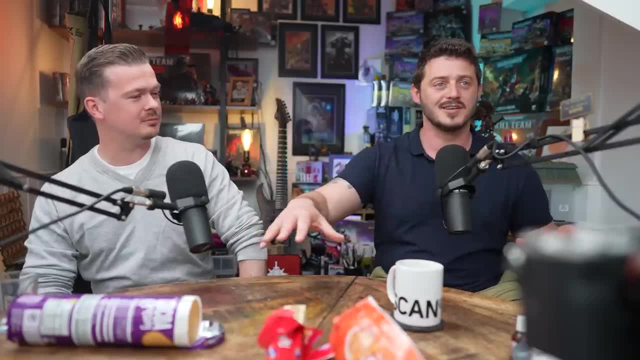 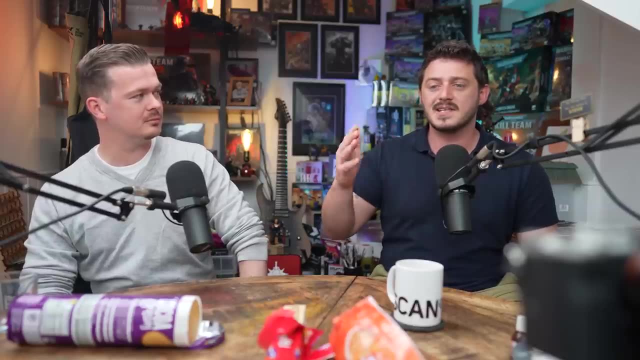 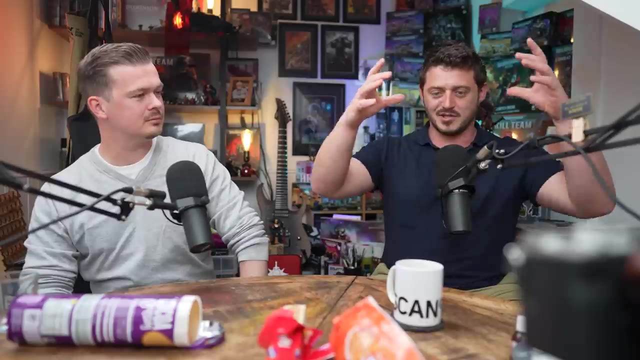 that's what crop circles are. yeah, that's their vibration language, which is really cool. why not? yeah, um, i had a. i wanted them to look sickly or like weird to the human eye. yeah, So we're quite a chubby species. I suppose We're very cylindrical. 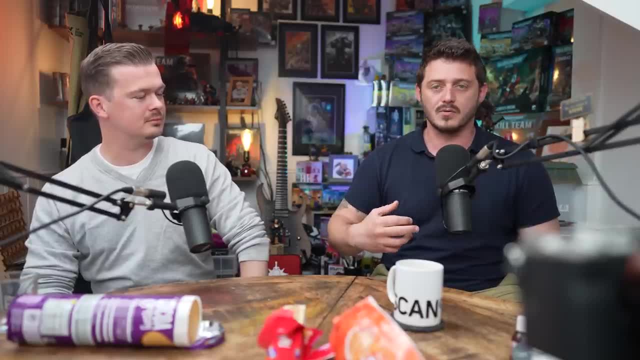 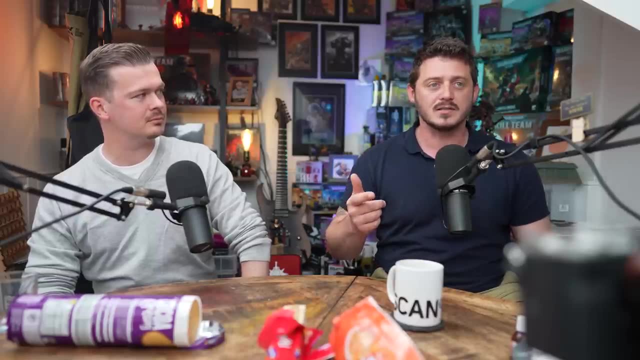 And I thought the one thing that's really weird is just anemic, Just like real no organ type thing, And my brain went to an old game called Legacy of Kain's Soul Reaver. I don't know if you've ever played it or heard of it. 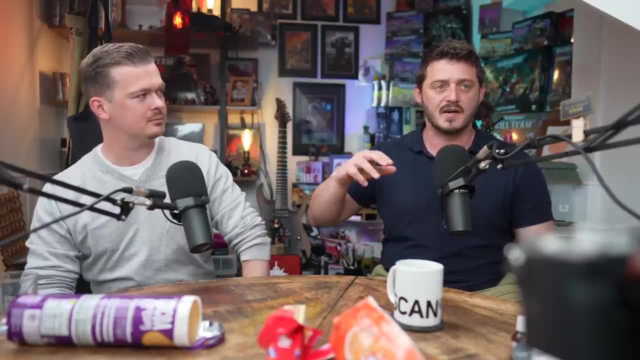 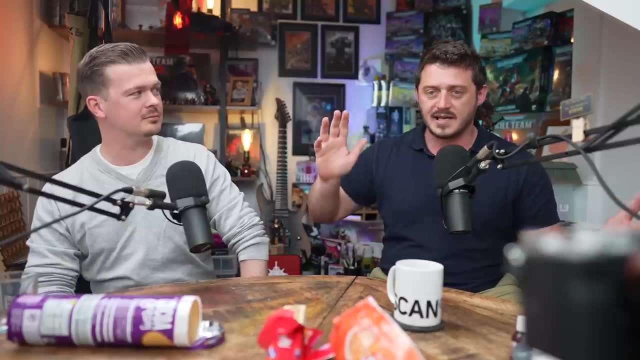 You play as this main character called Raziel, and he's a blue-skinned vampire. Yes, I have. Yeah, crikey, this is quite an old game. Yeah, but he was like thrown in water and it's acid to them and it's all in the lore. 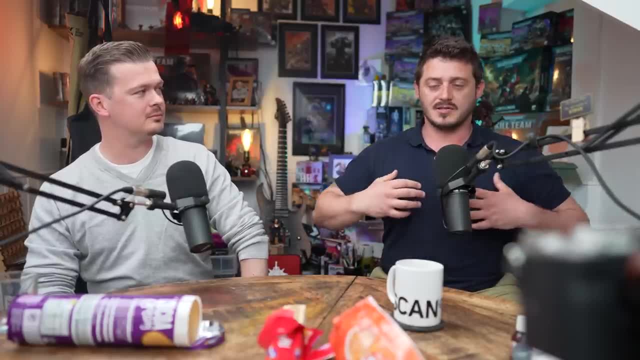 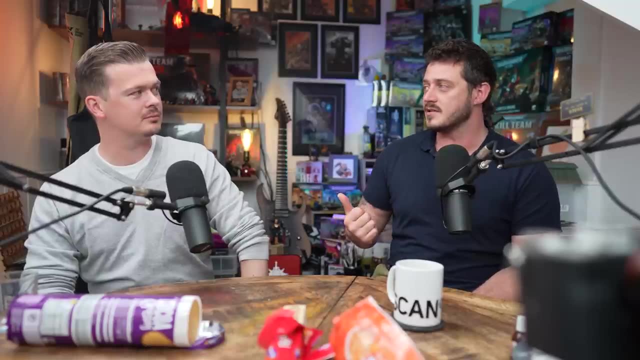 But it ends up like scarring away all of his organs and he's got his rib cage and his spine, Oh God, And it looks great And I was like that's a good shape. Alex had never heard of it, So I showed him a picture and, yeah, he's got the big hips and little teeny midriff. 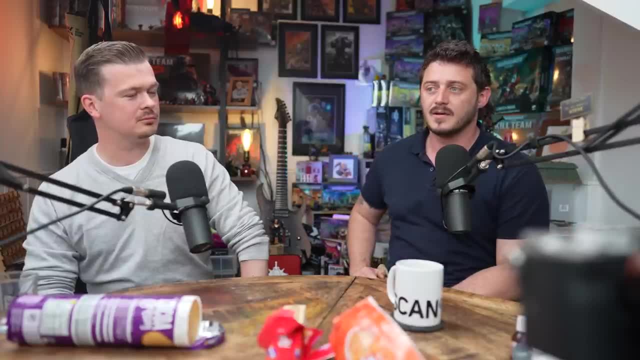 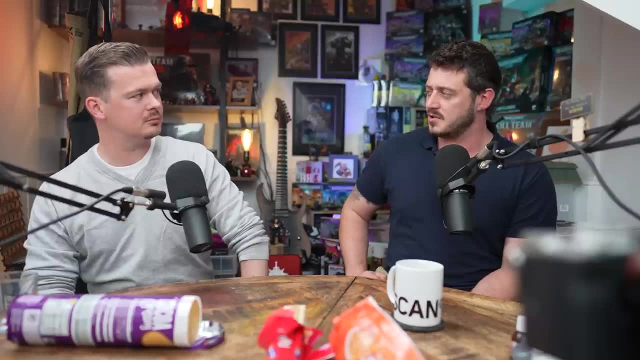 And then you've got the ribs and it worked. It worked to make them look sickly and skinny and just non-human. And then the one thing that I think it was you that came up with the idea about the spine. Yeah, Everything's got one spine. 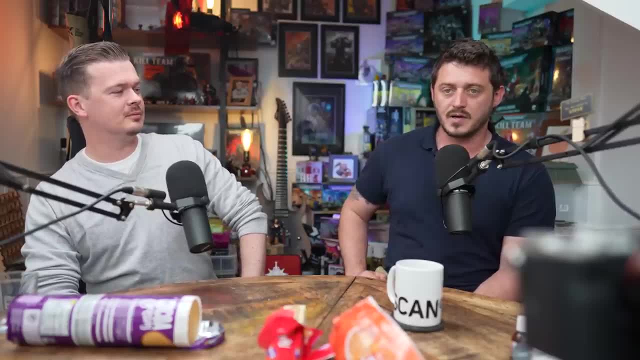 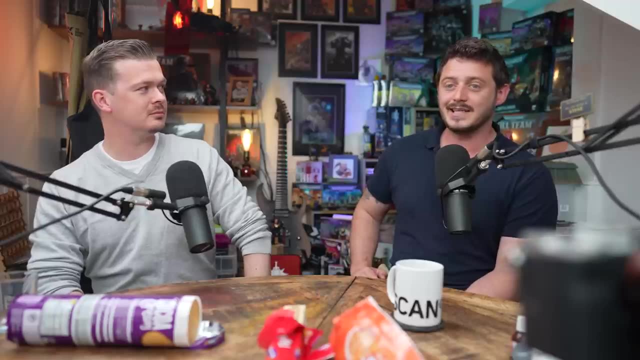 Yeah, everything in sci-fi, no matter how alien they are, they've only got one spinal cord Interesting. So our greys have got two. Nice Yeah, Why not? Yeah, It's the one teeny, weeny difference which is just, and it highlights in paint. 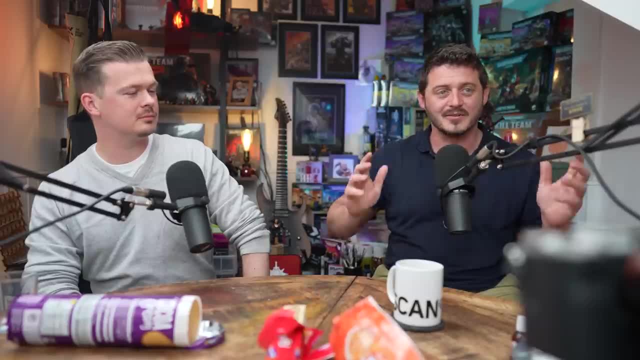 Very nice, Yeah, Because you've got this nice highlighted bit going down and yeah, Oh, that's really cool, Yeah. So I thought, why not? And then they've got two ridges going up the head because of the double spine. 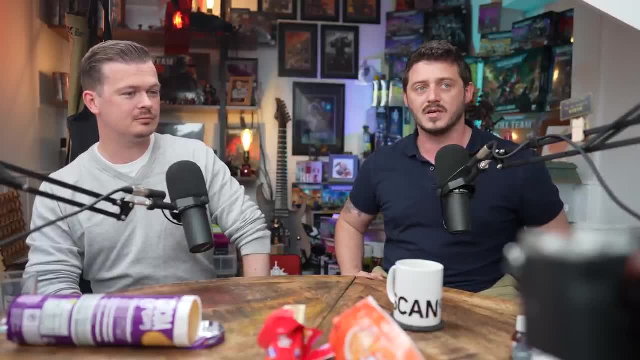 Yeah, Yeah, It just worked. It really changed up the back of the model as well, Cause obviously It's great having the front of the model when you're painting it, but when you're playing with them, yeah, you see in the back, you're seeing the back. 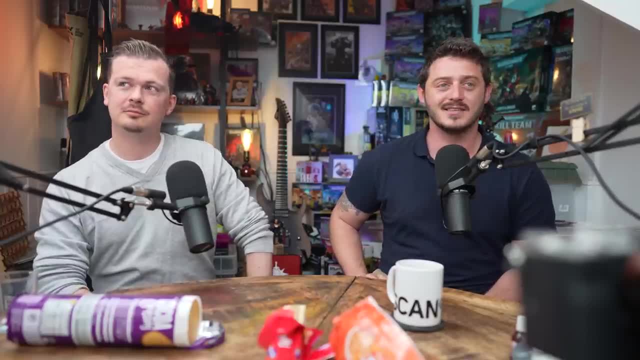 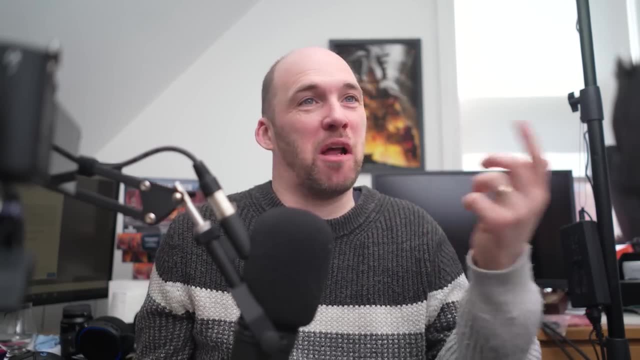 So, yeah, it was a great addition to that. Yeah, Oh, that's amazing. So one thing I'm going to do with the stuff that when I get all painted, obviously I've got like two colors, three color schemes. now that, um, I've just like a bit of a just. 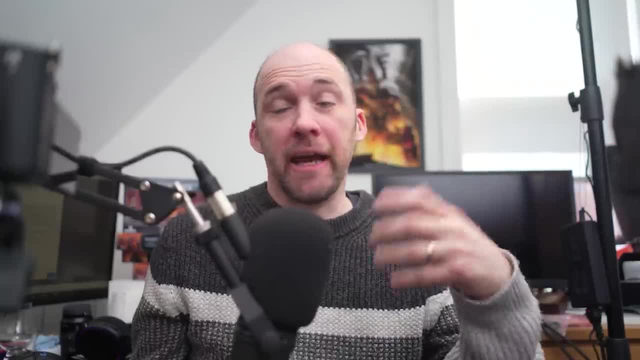 like me playing around, So I'll probably get some more at some point. but, um, in XCOM, one of the things that I always quite liked when you you have like this when you play the normal game. I like modern stuff. 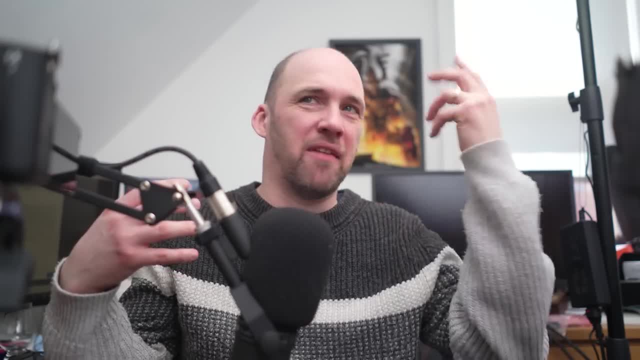 There's a lot of moderators out there that just like do free content and like give you berries and different heads, Yeah, Styles, and different like armor. Oh, there's this really cool armor from this film. I'm going to stick that as a model. 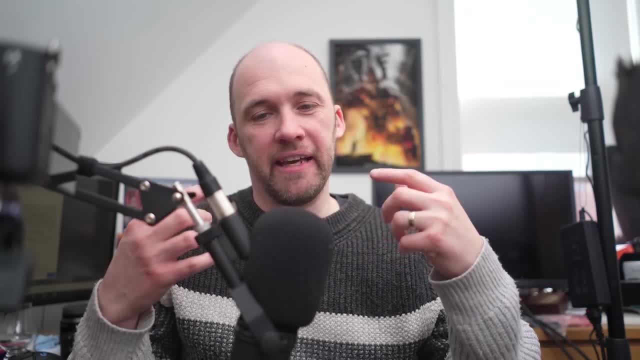 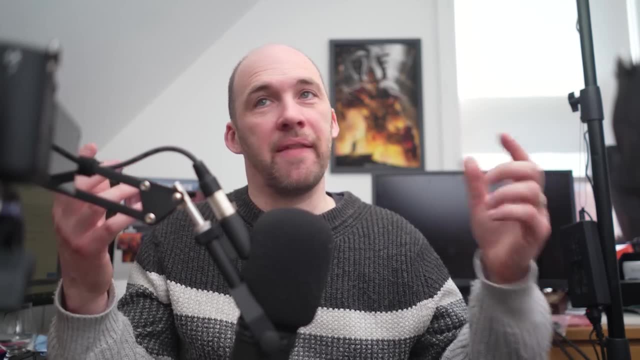 So you could do that with XCOM. but one of the things I really liked- and it's still there- is no matter what when you, when you hire recruits, they come from a nation and their flag and their name is that you can change the flag and the name if you want to. 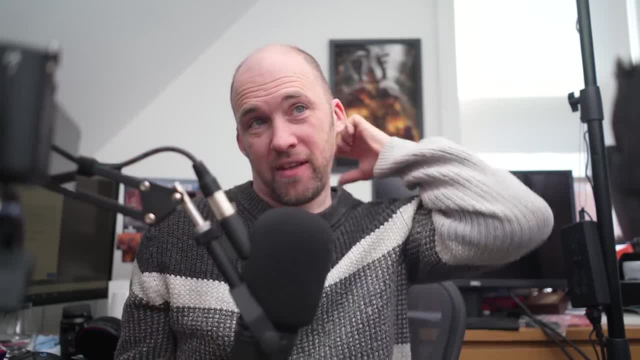 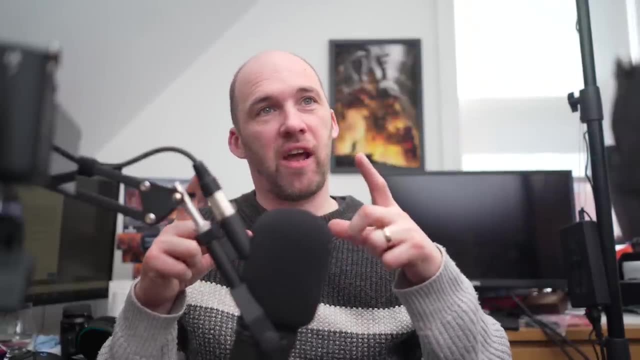 customize your own, but it goes. they have like a little stick a bit on the back of the- oh, you did that on the uh, yeah, I did that The United States. So I printed out ages ago a load of different like nation flags to that. 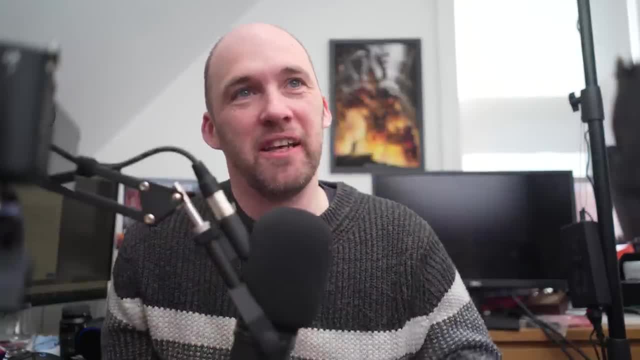 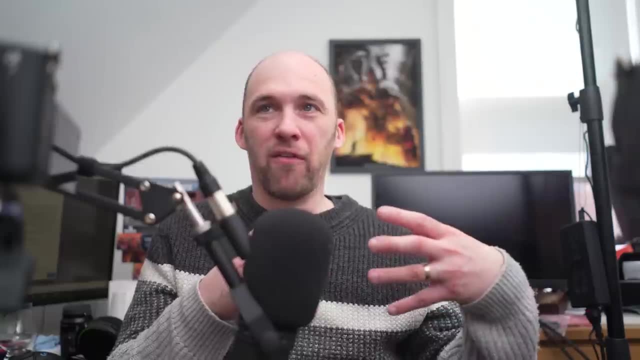 scale. That was just going to cut like different ones out and have, like, you know, this guy from Canada, this guy from India, this guy from Nigeria and stuff like that. So just have like a mishmash of like it's the same outfit. 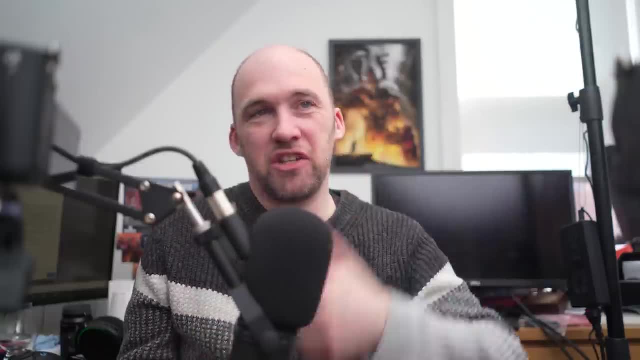 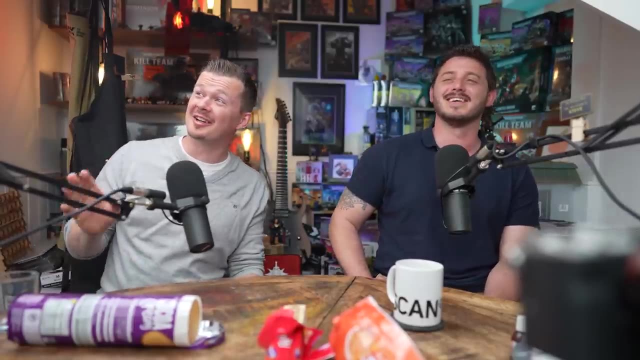 It's the same uniform but they've all got different, like uh, yeah, we might have to, yeah, we might have to steal that. There's, uh, that's how you find inspiration. Just folks, people and nickel. 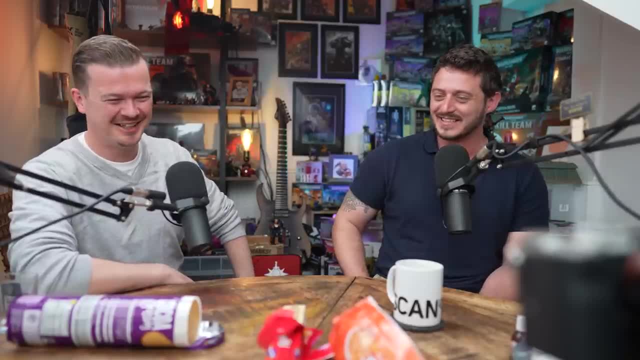 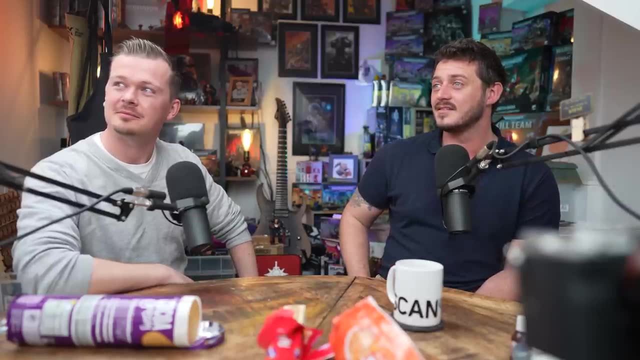 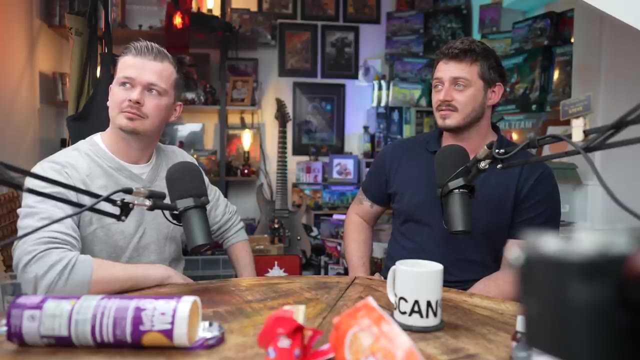 Then you shoot. Go wonderful, Um. so I want to put myself in in the shoes of someone that might want to make my own game. Yeah, Um and we. you talked about your inspirations from the law learning, blender and all that sort of stuff. 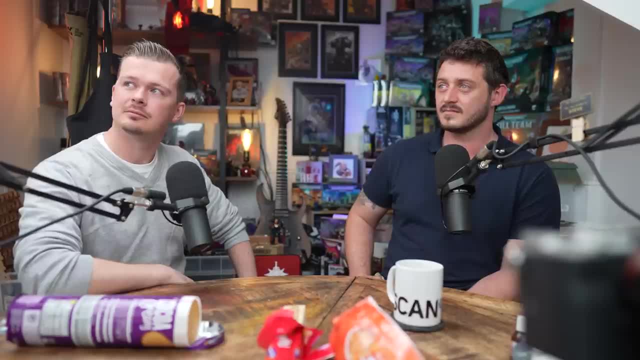 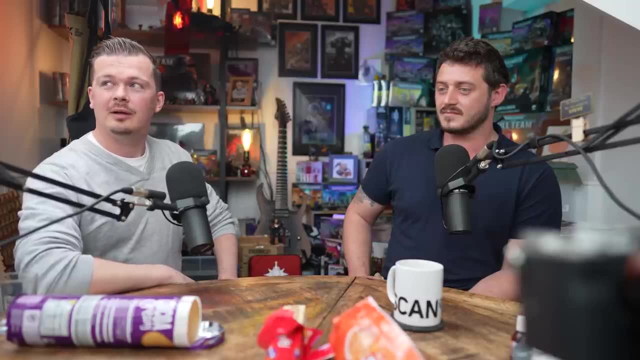 How did you then take that and turn it into a finished product that you can then sell, Like, where did the cards, the dice, how do you make models on mass and that kind of thing? Yeah, So I mean, obviously we haven't had to pay them on it. 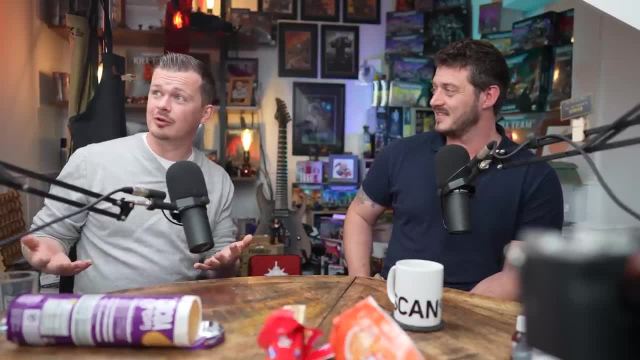 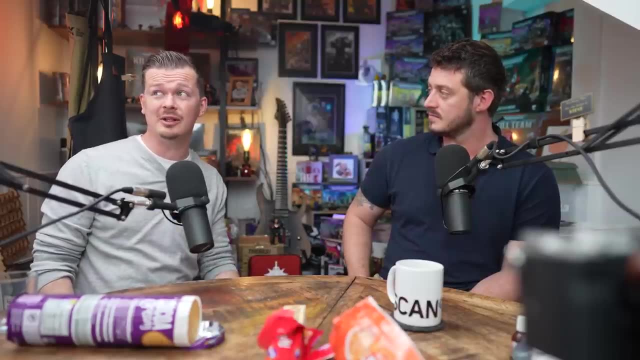 On mass yet? Um, obviously, once you go down the route of 3d modeling, you then find out that you can 3d print them. Yeah, Uh. so then you get your hands on, cause there's very decent 3d printers. 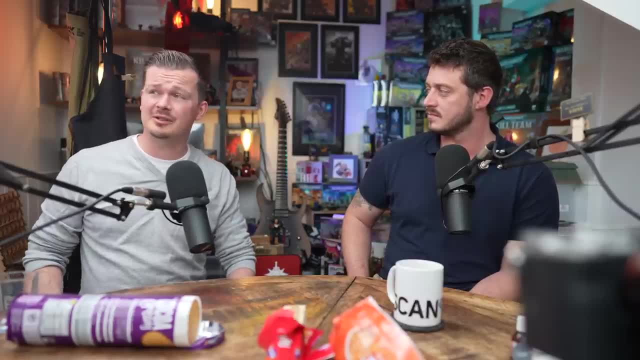 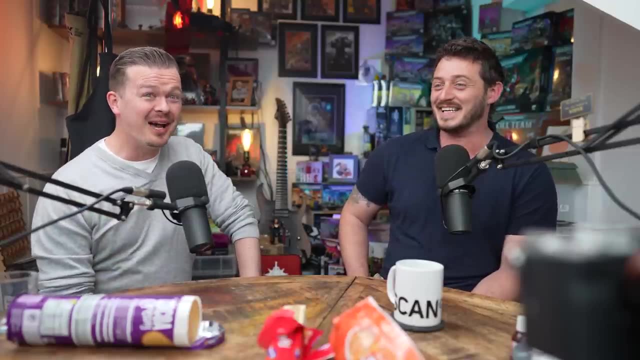 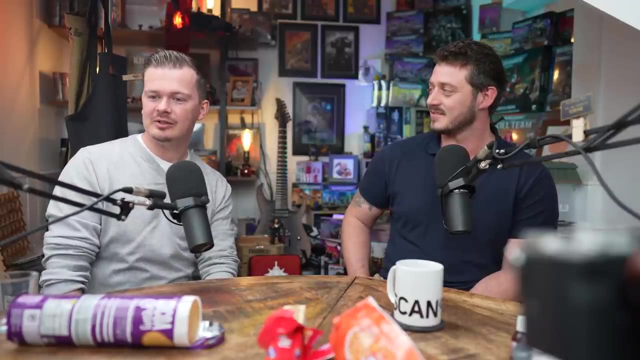 Yeah, Very reasonable, reasonable price. Um, I mean, that's, that's probably going to be the future of most things replicated, right? Well, exactly, heading in the right direction. Um, so, yeah, you look at that. and then things like the cards and the dice. 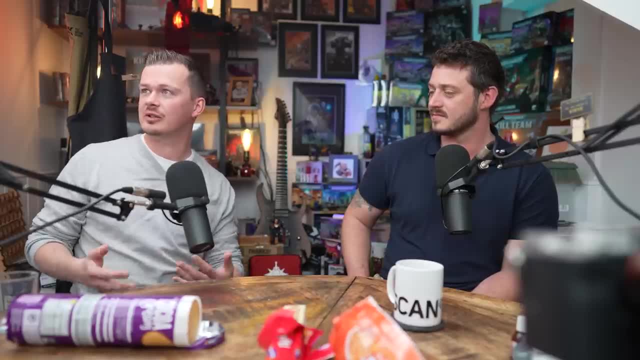 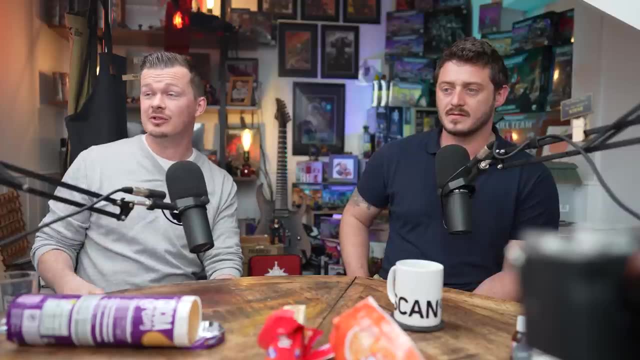 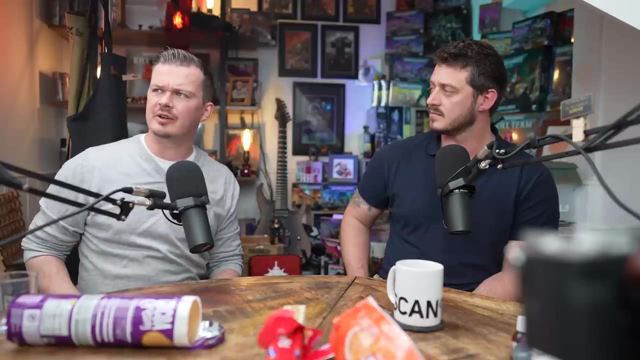 You just, you just have to look and find companies like that. Obviously, the graphic design we did ourselves. that's not to say that you can't outsource, but I would encourage anyone to say: you can do it yourself. Yeah, You just, it might take you a bit of time and a bit of a bit of work, but then, yeah, you find companies when we've kept it. we've seen a lot of Kickstarter that bad problems with cause. obviously, there's horrendous issues with China now in terms of getting stuff over and additional costs and people waiting. 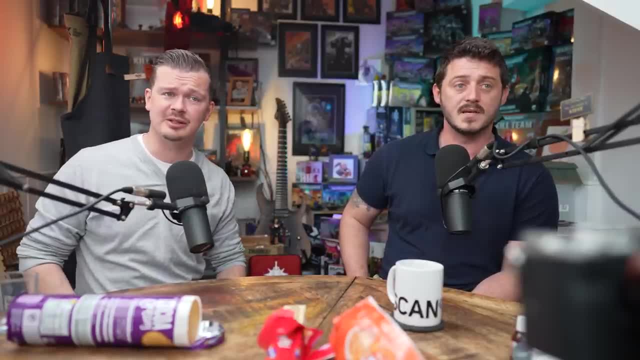 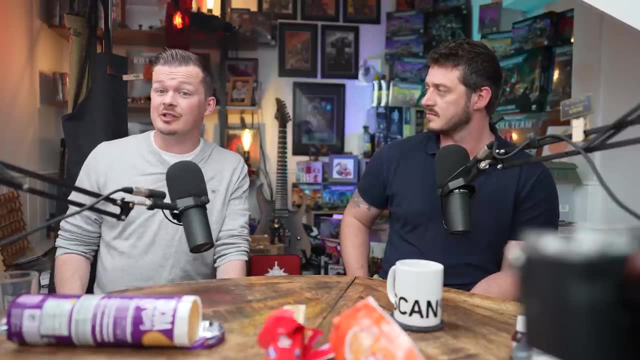 I know people that are waiting three, four years for things. They're back. Yeah, it's really insane. We're using UK companies for everything. Oh great, Um, so yeah, things like that. obviously, if you've got big enough, you can buy the machines that make things. 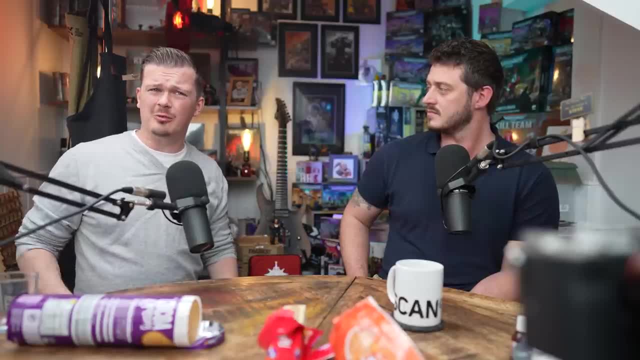 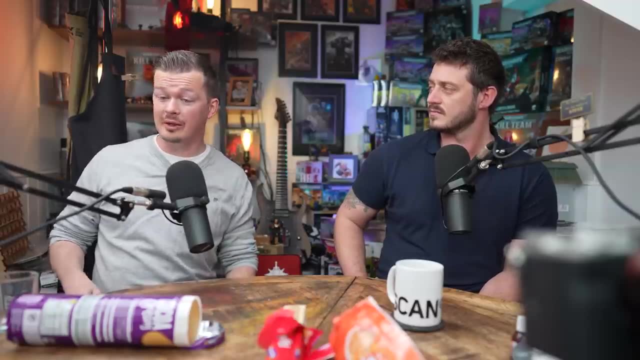 But to start with, yeah, there's a company, I think they're in a place called March, which I think is Norfolk way. Um, yeah, Ivory graphics, or shout out to them. So yeah they're, they're printing our cards. 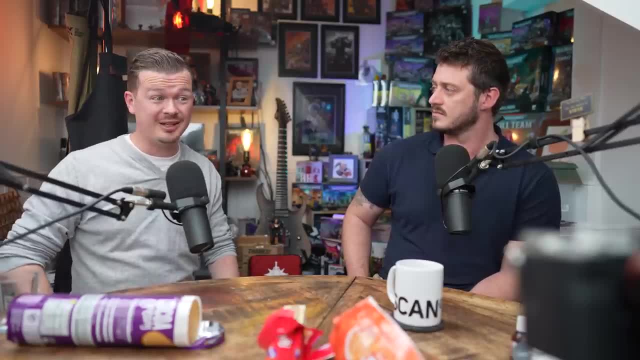 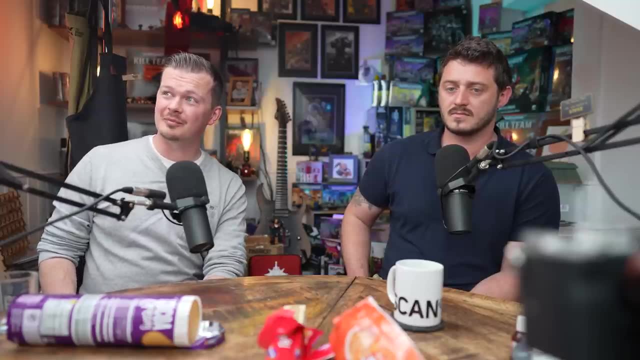 Oh, amazing, Yeah, Yeah, So you could, yeah, you can do things like that. It just yeah, Oh, it's back to yeah, Teaching yourself how to do Yeah, A multitude of different things that you know. so if you already entered one of these things, you already had probably a jump ahead of where we were when we started. 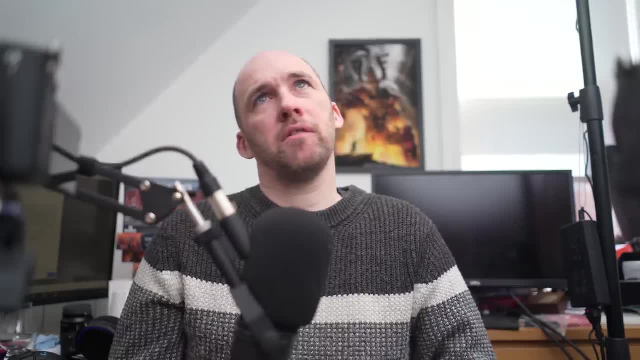 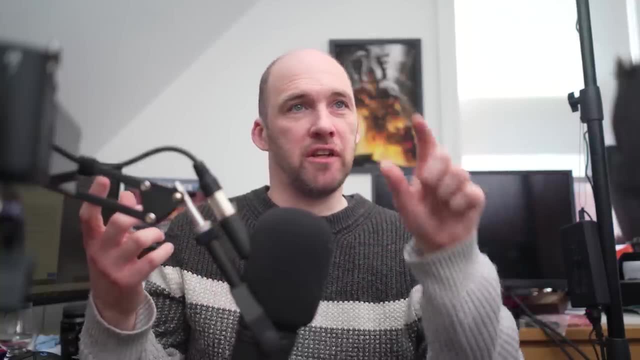 Yeah, So would you say. um, like from an artist point of view, there's a lot of really nice visual, uh geometric, shapes that you've done for, like the different factions, like you know, all the different logos and stuff, like the grays, the humans and stuff. 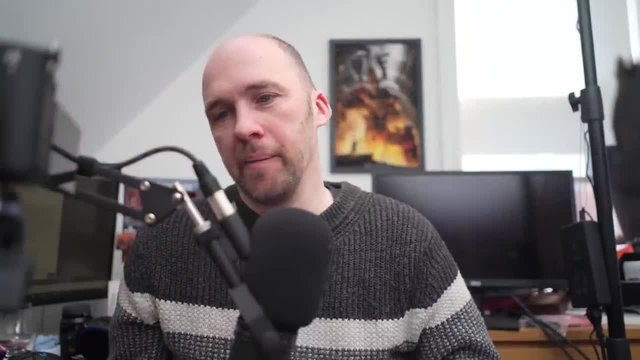 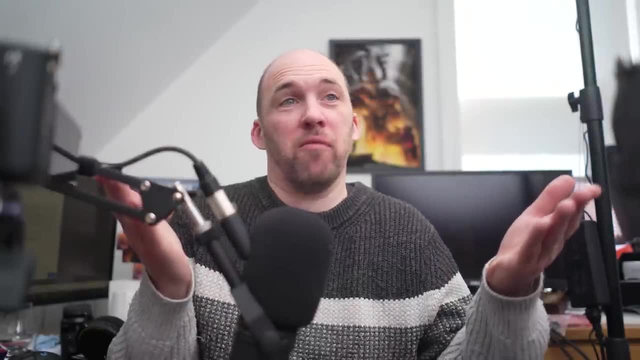 And obviously the way you've presented the war on terror website. um, is that something you've learned or is that just something that you all had? Cause you've both got very different backgrounds right? Cause it'll be interesting Just to talk about, like, where you both came from from a hobby point of view and, uh, how you met and uh make yourself like a dating site. 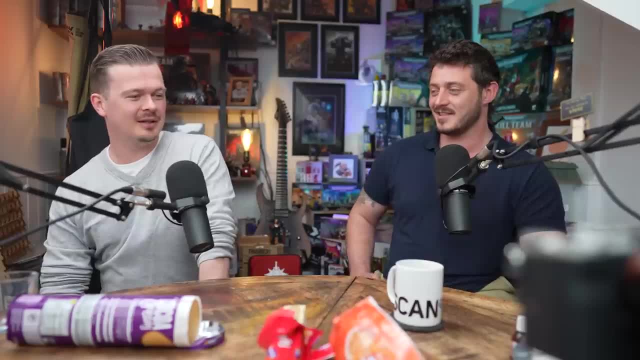 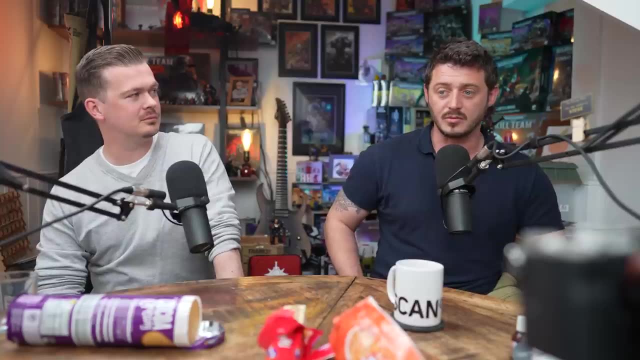 Really. Well, yeah, yeah, The, the geometric faction shapes. Well, I'm just going to put it out there. Like anyone looking at making their own game, like humans are the hardest thing in the world because of the uncanny Valley. 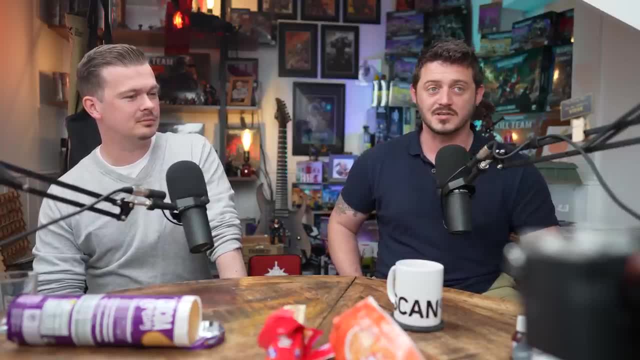 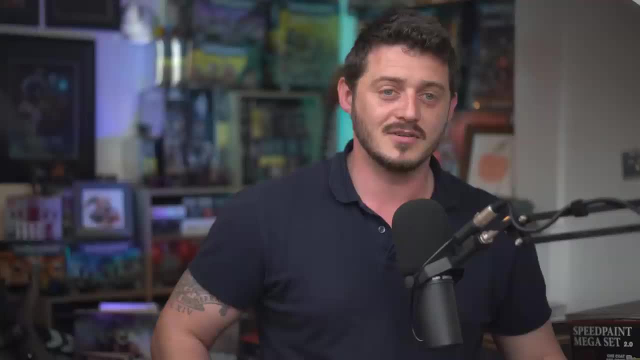 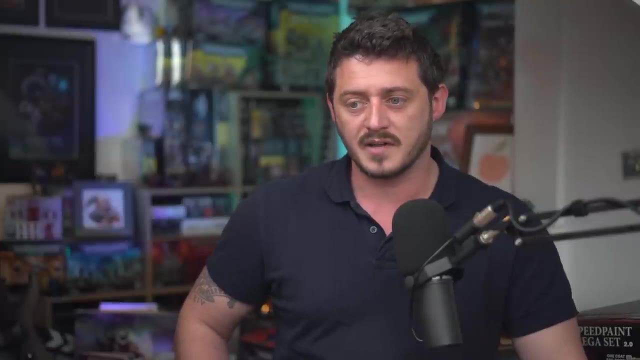 I despise modeling humans, any changing position, to make a nice like I don't know, different. Well, yeah, Different position model. It's the worst thing in the world, Because if something's wrong, your eyes are immediately going to go to it and you know, and yeah, and even even the faction symbols, the main five faction symbols that we have. uh, so the humans- gray talus, watcher and Haraka, the other four were they pretty, they came pretty easy. 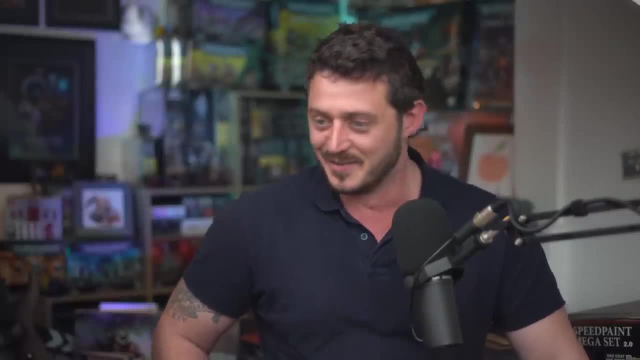 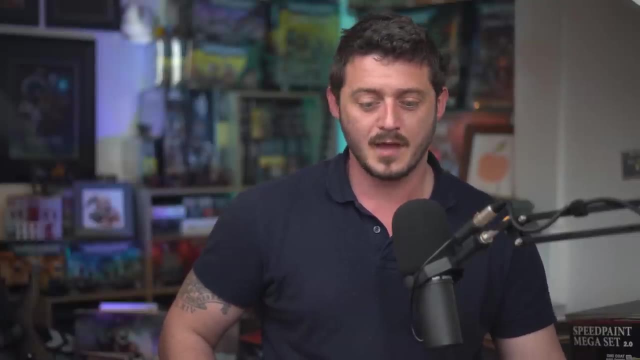 What? there is no unified human symbol. We went through loads of different designs and just ideas, and until we just came up with one and we were like: yep, let's just roll with it. Yeah, And now I can't picture them without that. 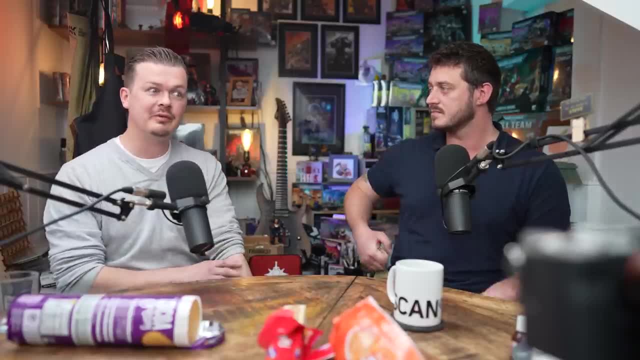 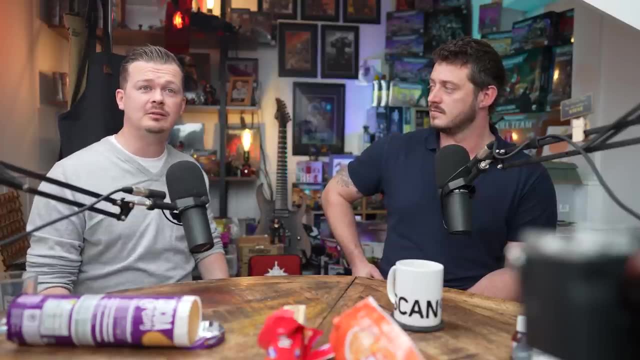 Yeah, Yeah, And the affection was. there's still quite a lot of uh information that we haven't quite a time to get onto. the because all of the faction logos and symbols, they do have a meaning. Yeah They. they arc back from, be it where it is in in the world or or something about them. 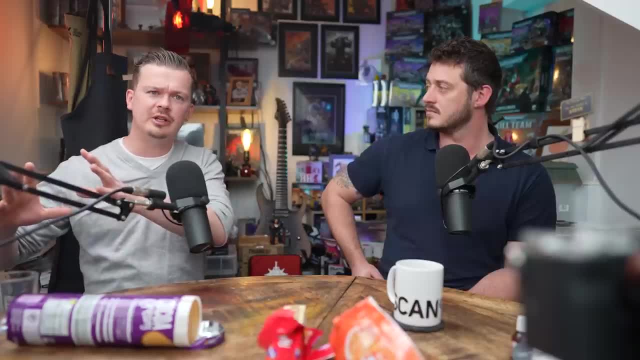 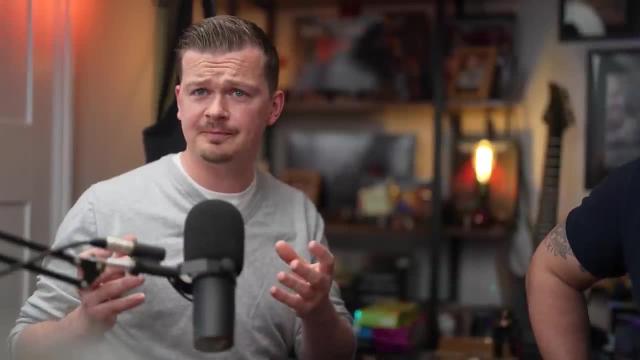 Like you mentioned, the um, uh, the United, no, the central nations. Um, their sign is sort of a circle with a bit of the top, and it's a stylized uh Uroboros, Uh, oh, which is the snake eating its own. 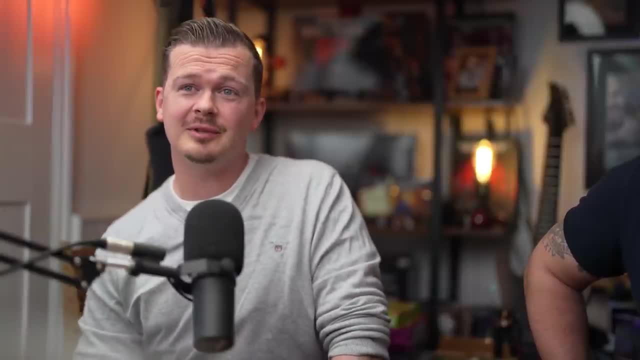 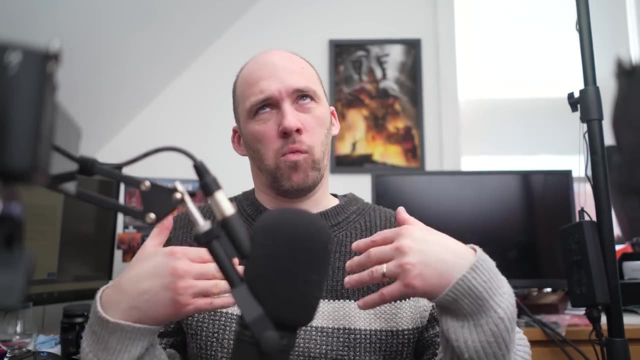 Yeah, yeah, yeah, yeah, yeah. So, yeah, everything, Yeah, We, we thought, tried to think about everything. Yeah, Yeah, Cause I was lit, That was going to be the one. I asked cause I did. uh. uh, I did get them white time with red markings, but on the circle, but the front I kind of tried to mimic that. 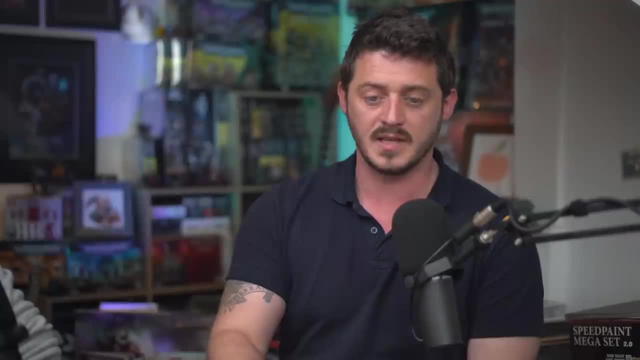 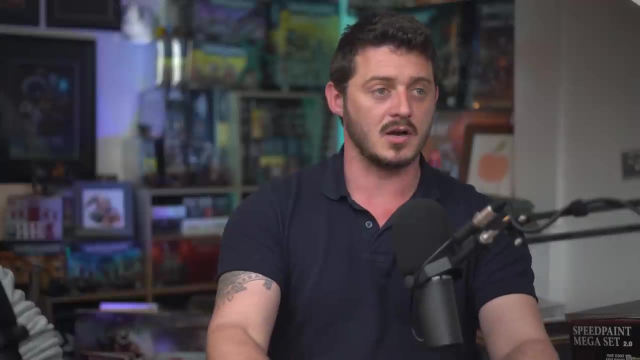 Yeah, I just cause there's a. there's a heavily detailed one of that. It was: um, instead of a snake eating its own tail, it's a snake going round and facing a dragon. Oh, um, and they're kind of snarling at each other. 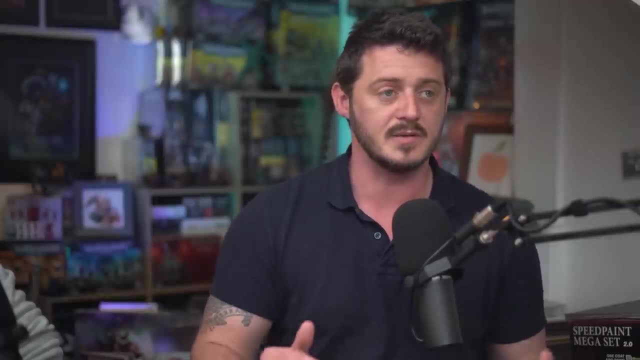 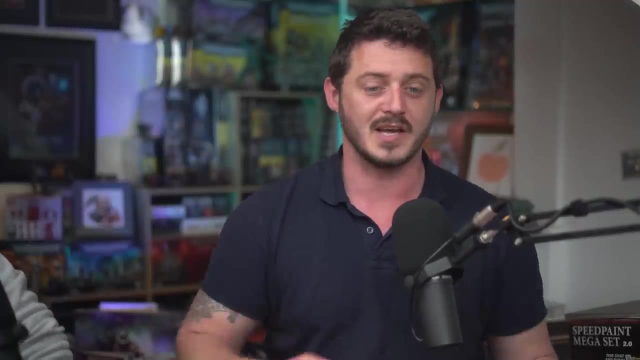 So I drew that one heavily detailed And Alex was like no simpler, Yeah, So I drew a real simple version. He was like simpler. So I went and I think I got. the fourth one was just that shape. It sounds like my university course. 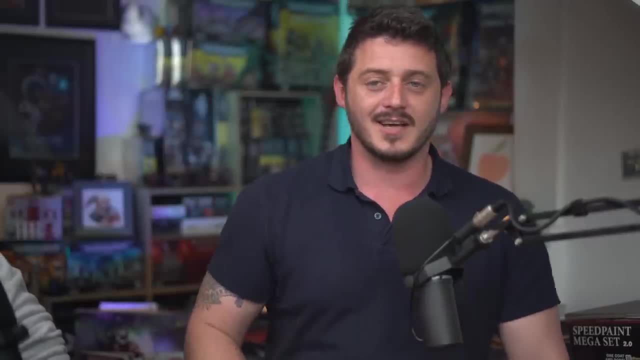 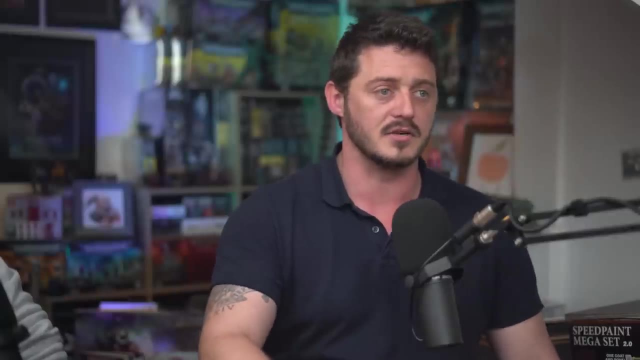 Right, Yeah, Um, so he was like brilliant, Um, so I was like cool, And that's that's how it came up with that sort of circular shape with the break in the middle, Um, but there's that, there's the detailed version of it. 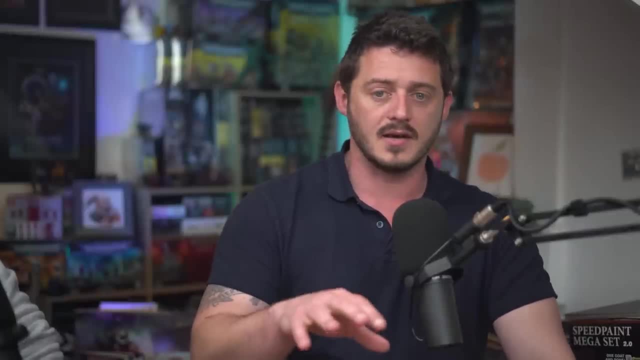 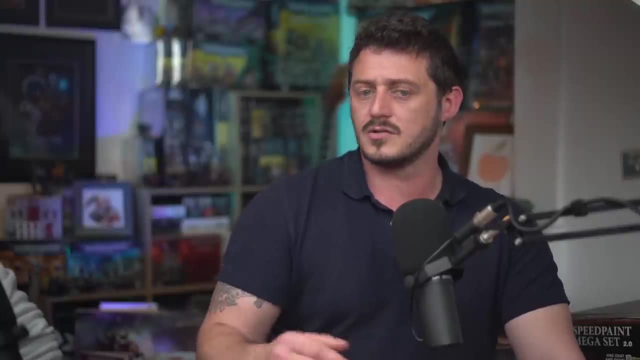 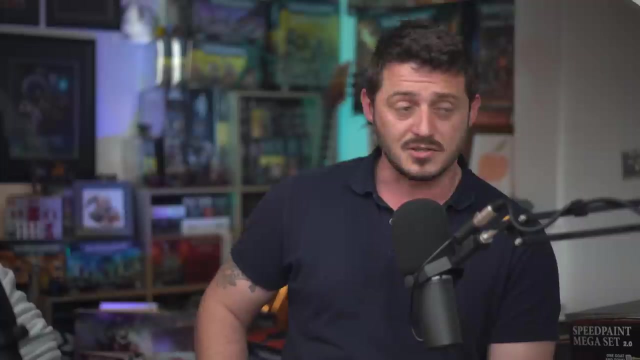 So, yeah, every single one of them has either a a symbol from, like language or mythology. that basis that, yeah, is based on The factions, strengths or direction that they want. It was good fun, Actually. We learned tons about different mythologies and history and loads. 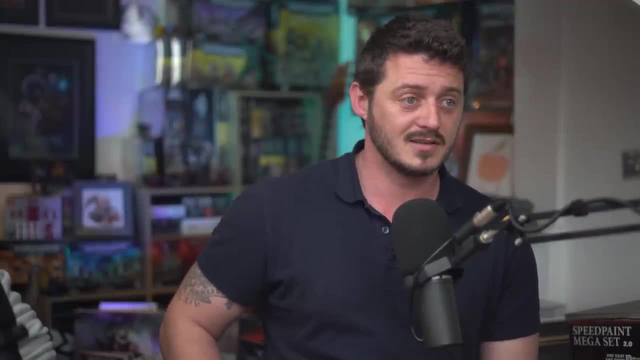 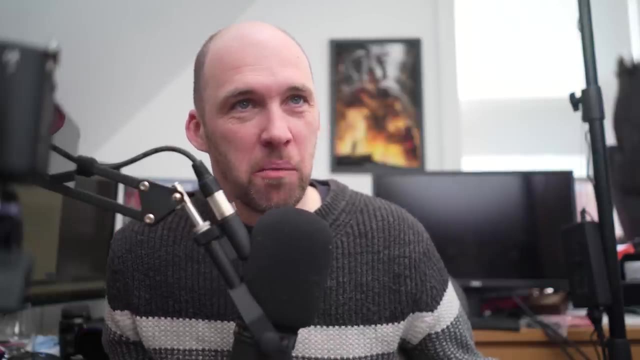 It's awesome, Yeah, Really really good fun. So I'm going to ask a quick question just for our viewers, Cause Mike, right, All these guys. So, Alex, yes, your background, brief description of who you are, what you've come from and how you both met. 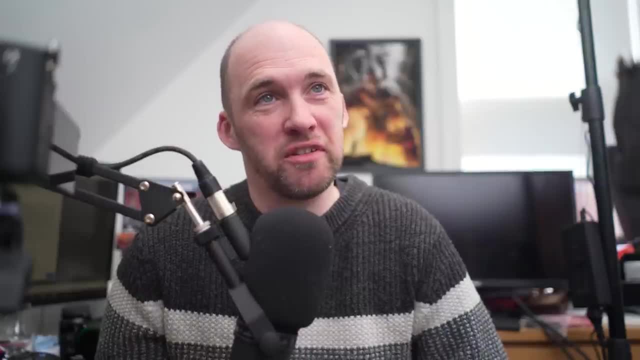 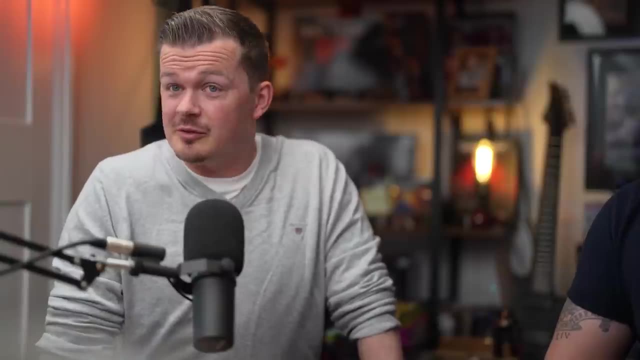 And then we'll go on to you. Well, cause you know, cause you both combined forces at some point, Absolutely Yes, My, my background- but not quite as exciting, as you will find out, Wills is: um, I've just been a chef, for I heard the chefs- a seal just chucking that out there. 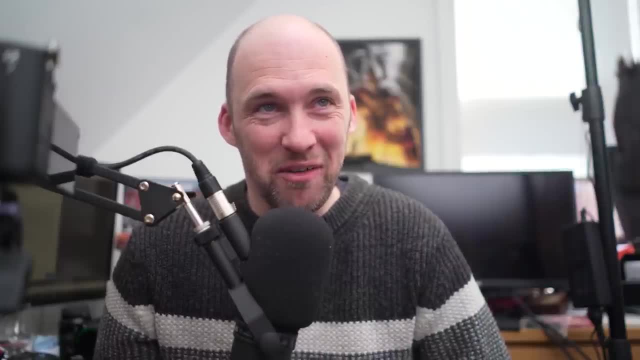 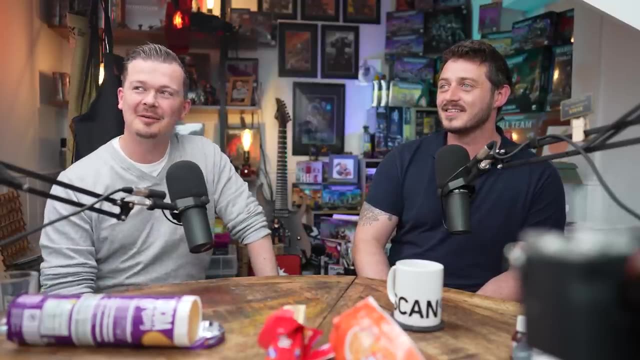 Chef's a seal. Yeah, Have you never seen under siege? Oh no, Am I showing my age? I've seen. that was that was. it's well, under siege is the only watchable. Steven cigar is a Navy ceiling. He's a chef. 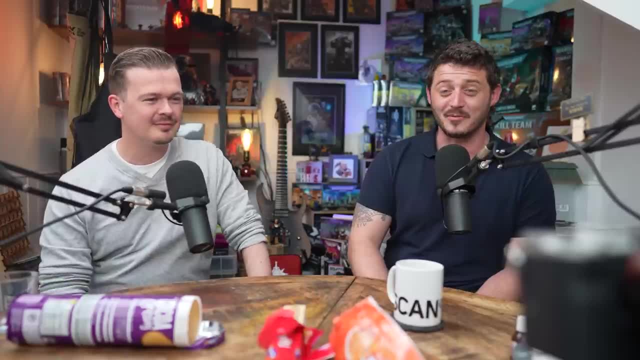 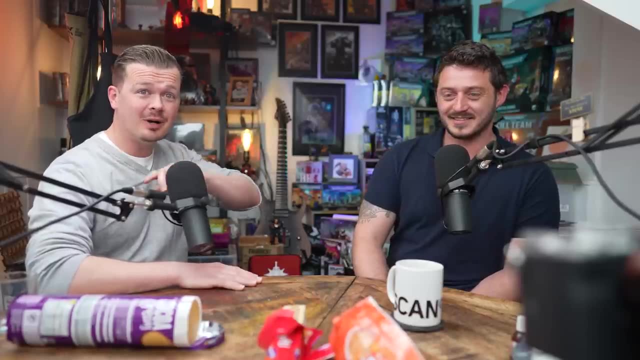 So I've seen. I've seen on the stage. Go watch it now. That sounds amazing. So I thought I'm normally pretty good at film quotes. fun, If we were in a bar not far from here last night and I missed another blazing film. the guy looked to me like well, if you're not, I mean I'm the same. 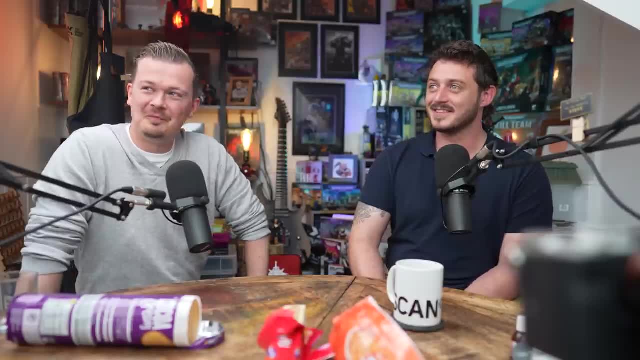 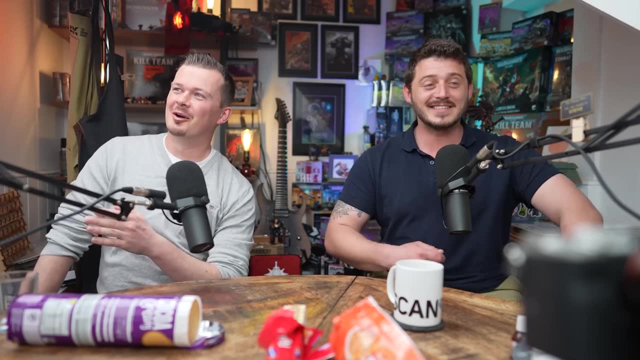 No, I have. sometimes I'm just like I have no idea what just happened. to be to be fair, The way he said that I was like chef is I went down the seal route initially. I mean it does laugh like that, but I'm not going to lie. 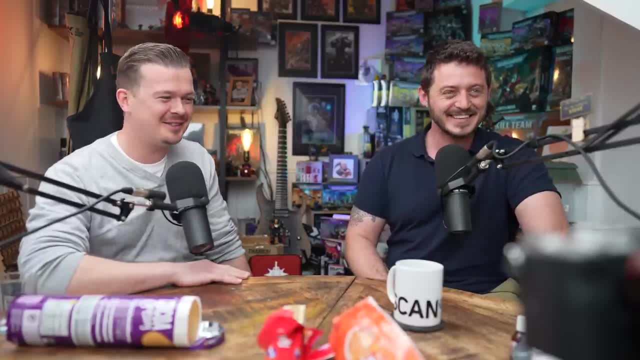 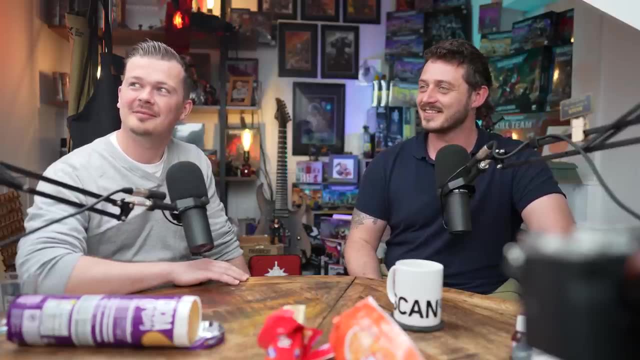 Yeah, I was just balancing. I was like, oh, is there some like weird, weird language about being a seal and you're a chef? Sorry, Did I ruin it All right? No, So you're a chef. Yes, 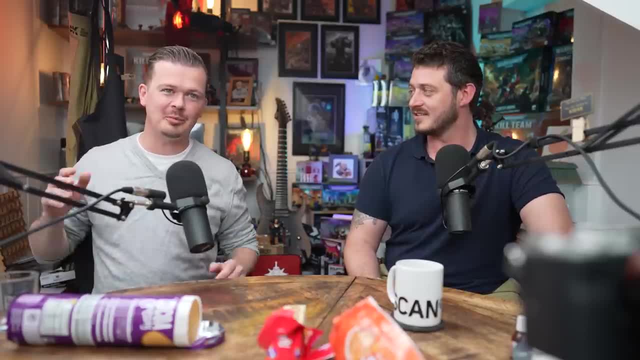 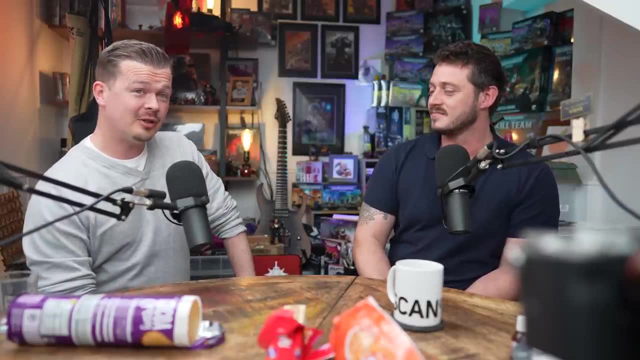 Well, I'll do for next time We'd meet yours, I'll put on some weight, slick my hair back And I'll become a master, Yeah, And then I will come back and that's: yeah, Yeah, Um, no, just a chef. really fell into it when I was a teenager, part-time, and then never fell out of it. 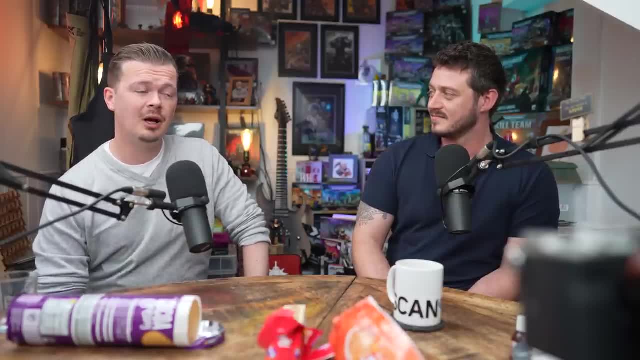 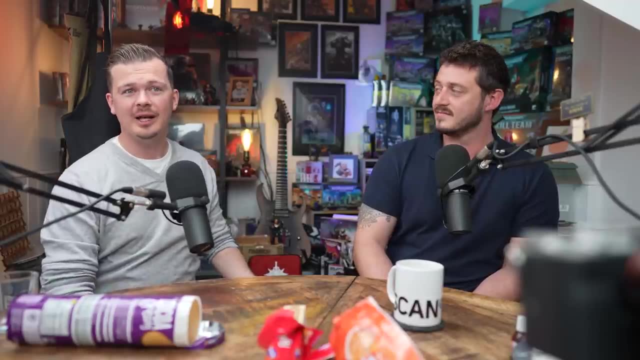 Really left school and and favorite dish To cook? Uh, it's gotta be something with venison. Oh, I think, Yeah, Well, yeah, Anything, really, That venison is probably the best mate. What was it about venison? 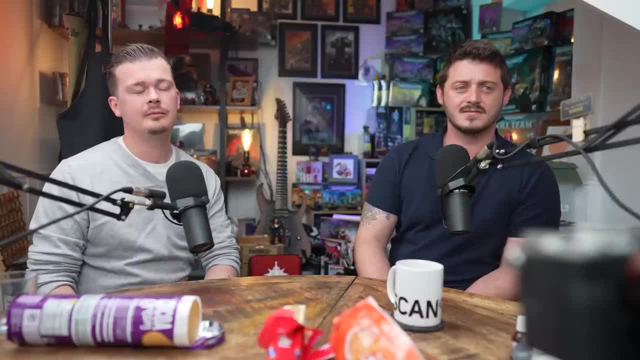 Cause I've had a venison burger a few times ago, Cause I used to go to reenactments and they used to have like a venison uh big stand And I was just like I've never tried it before. 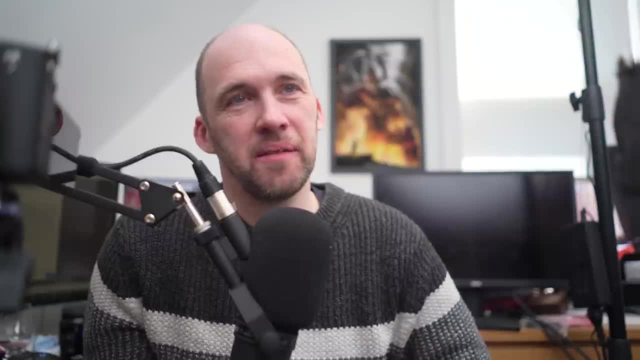 And I had a venison boo and I was just like I want this every time. Yeah, It's just. yeah. I mean certain cuts. obviously it's a slightly gamey and meat. Best thing is going to be the loin. 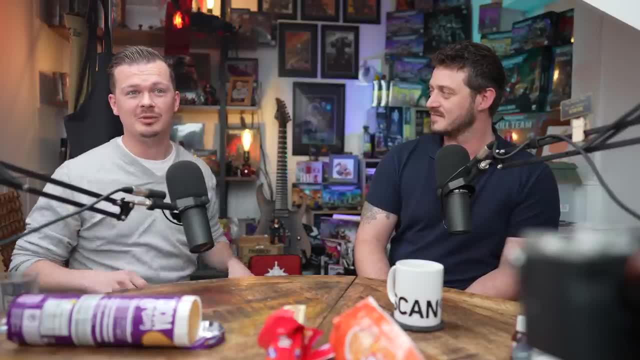 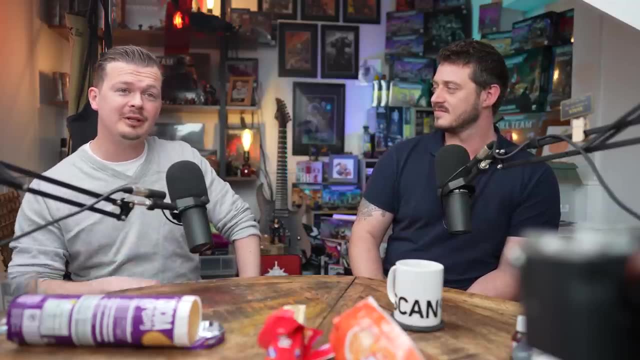 If you enjoy a decent fillet steak, then you're you're never going to have any. Is it more the taste or just like what you can do with it that you prefer? Um, what you can do, I mean it's pretty with a lot of the cuts of meat. it's pretty, pretty similar to what. 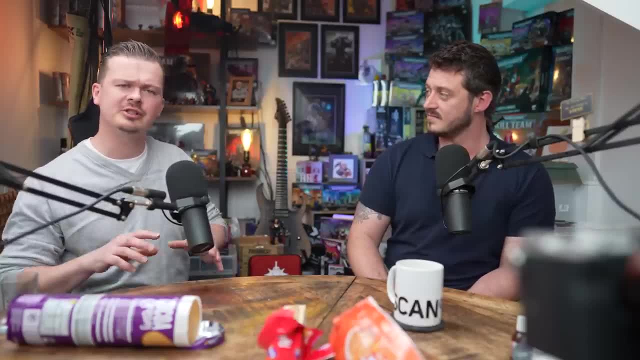 you do with a cut from a, from a cow, really, um, depending, although obviously it's a lot leaner. So, yeah, Um, it's just a tastier meat. Yeah, Just a far, yeah, Far taster. 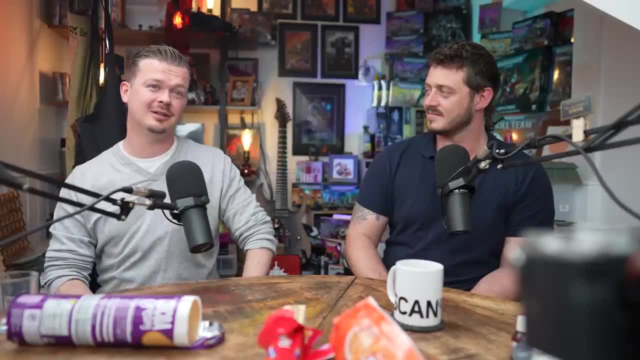 Got into fish a lot more. I'll take my kids fishing a lot now. Oh cool, Yeah, My daughter caught sea bass- The other. she'll be very proud that I'm mentioning Uh. so yeah, Felted that the other. 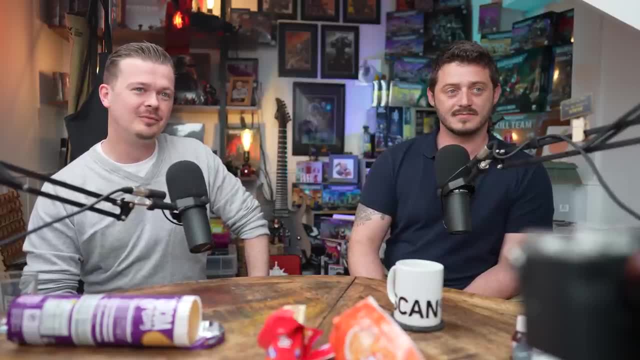 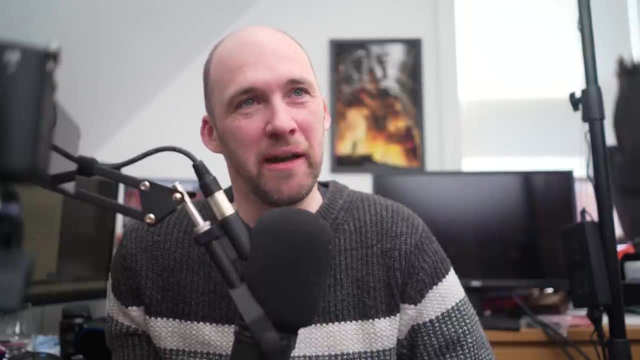 And so, yeah, I remember that I worked at a trout farm for a time and would bring up back the odd rainbow or brown trout and I just have to watch my mom just like gut it and then squeeze all the poo out And I was like there's a lot more to cooking a fish than I realized. 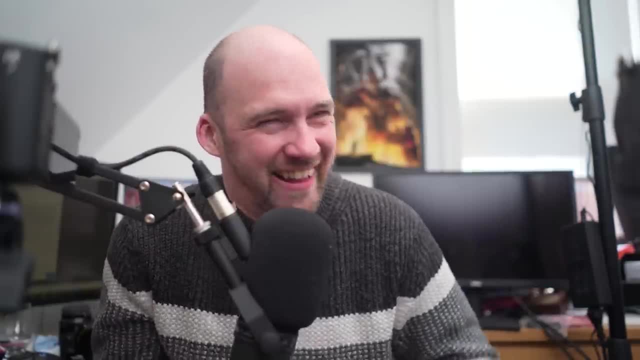 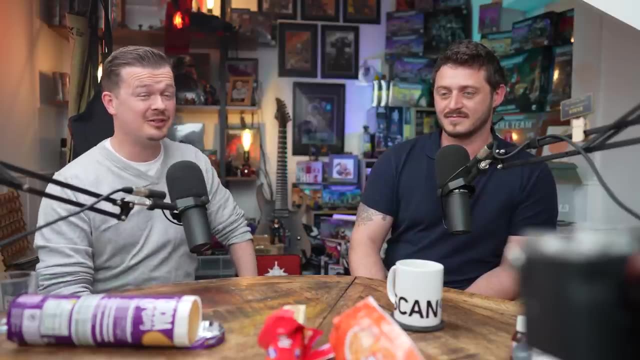 Just there, just squeezing all this stuff out, I was like oh, oh, Yeah, At some point I mean, yeah, She didn't want to watch as I dispatched the fish. Yeah, Yeah, Yeah, But no yeah. 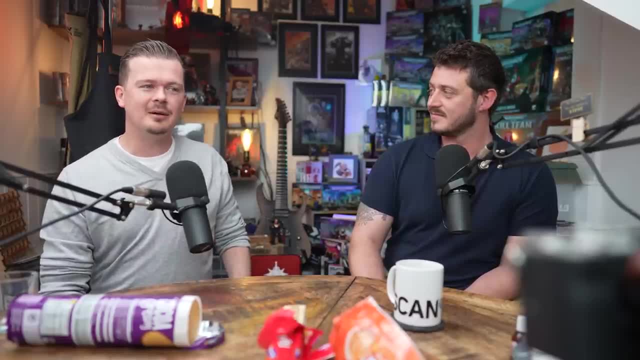 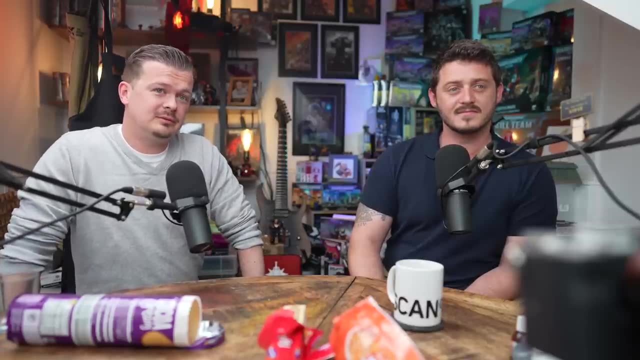 She was, yeah, She was quite proud of that. So how did I get into that? Um, oh, you said yeah, Yeah, Yeah. So so you're currently still, You're still a chef and, uh, uh, you, are you working in the same place together? 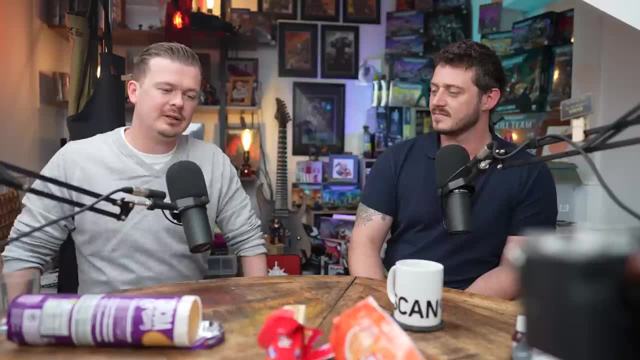 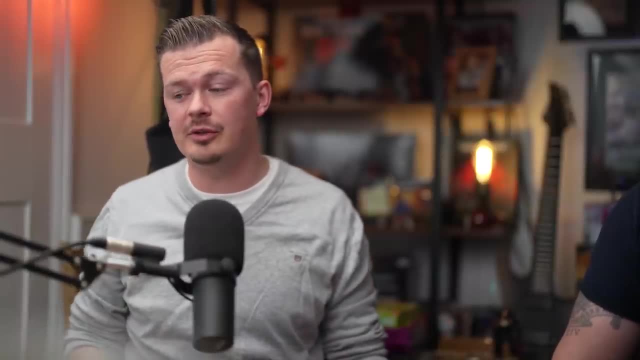 Is that right? No, we, um, I uh yeah. So, having two young kids, uh decided it was easier to uh basically go freelance Uh, so I work with a couple of agencies and just they can put you anywhere. 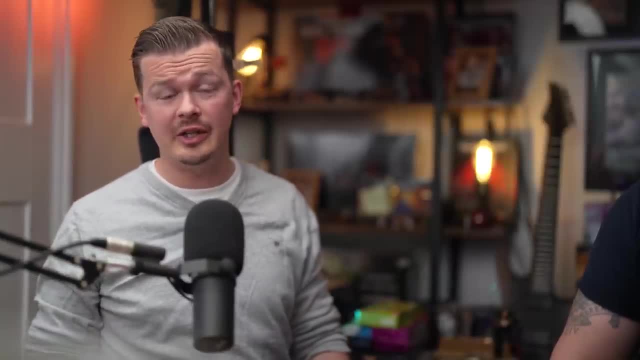 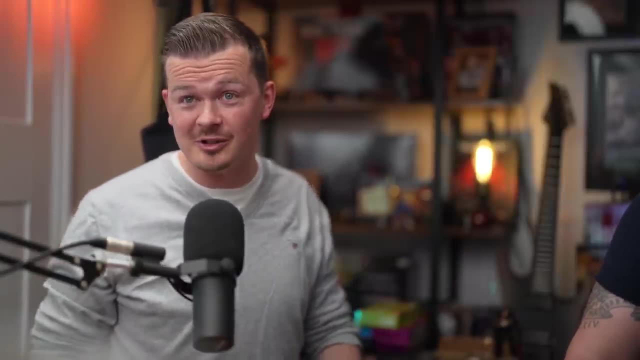 Um restaurants, pubs, schools, uh, and then zoos. Yeah, Uh, there's a. there's a zoo down, uh, near where we work, Um Portland zoo. I'll shout them out: It's a nice place. 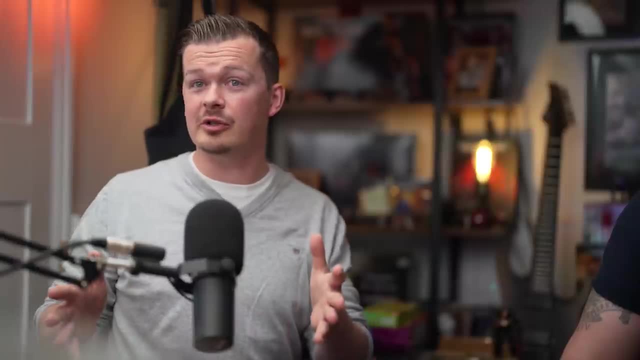 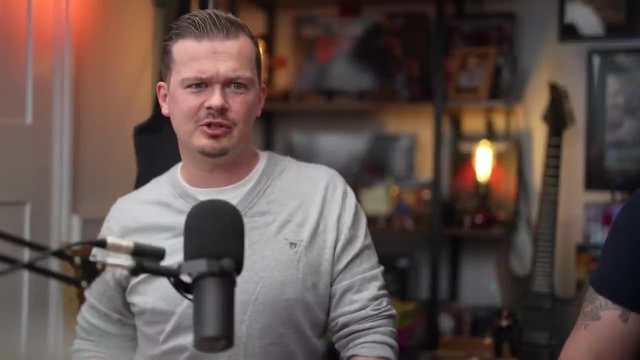 Uh, and they've got accommodation there, Um, and one of them's a, a cottage sleeps up to eight people, and you get a private chef that cooks your dinner and cooks your breakfast, Oh wow, Uh. so I got put there for two weeks, which ended up being about four years. 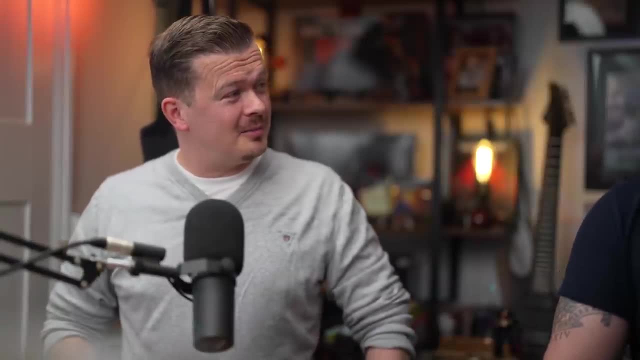 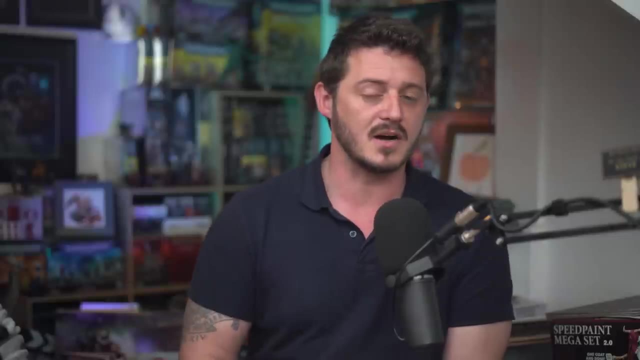 And is that how you met Will? Yeah, Yeah, Cause as part of that, um, my job at the moment is zoo ranger, So not a keeper directly, but the education part of the park. So we do dabble with the animals, like in winter comes a bit quieter. 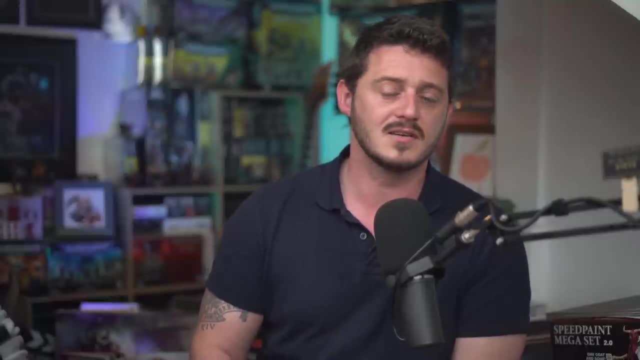 Uh, the sections need help. Then I've helped out on all the sections, Uh, which is good fun. Rhinos are the absolute greatest animals to work with. They're cute, They're cuddly, They're gentle, They squeak when they're in a good mood. but, um, part of my role is taking people. 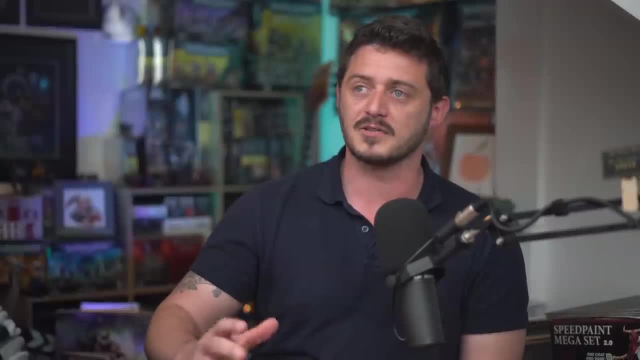 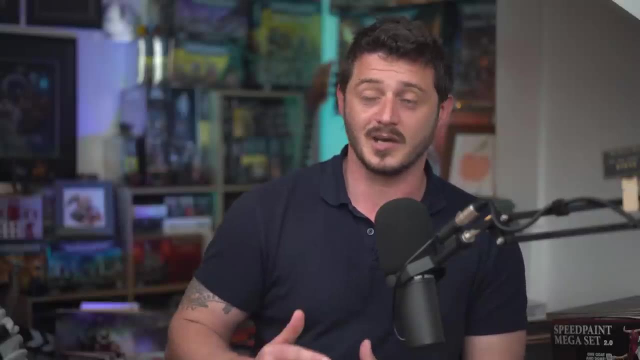 on sort of like private bespoke safaris on a small Land Rover up to group of 10. And basically for a couple of hours I just chat absolute nonsense about animals And uh, it's shutting me up. That's the trick. 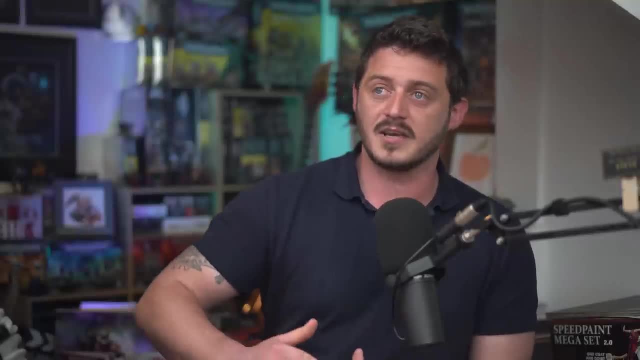 Um, part of the cottage experience is you check in, you get a safari, or part of the safari up to the cottage, Um uh, we then with you hosting for the evening, carrying on um while the chef cooks, And a lot of the time you just leave the guests to chill out in the cottage and relax. 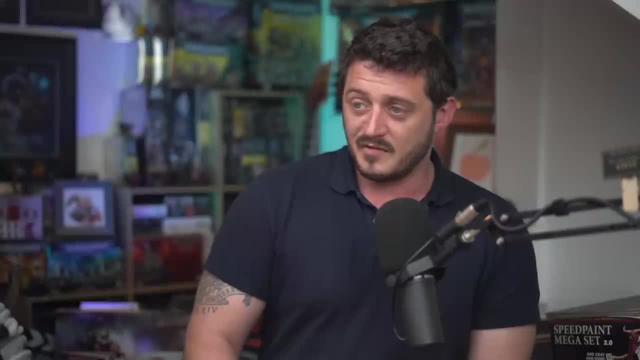 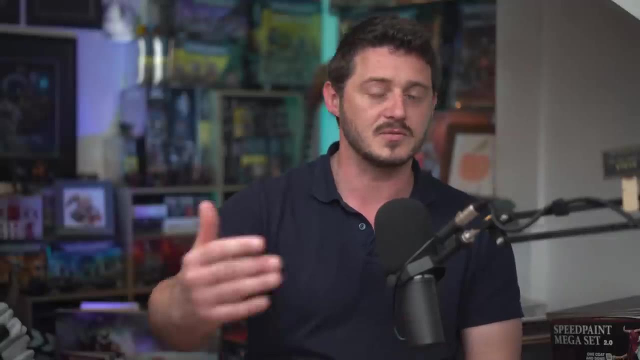 And we ended up having a laugh, chatting about random movies and inventing games in the kitchen, Um, and then in the morning I'm back chef in the morning, and then they get a safari out and that's when they check out, Um, and that's ended how we ended up, sort of working together. 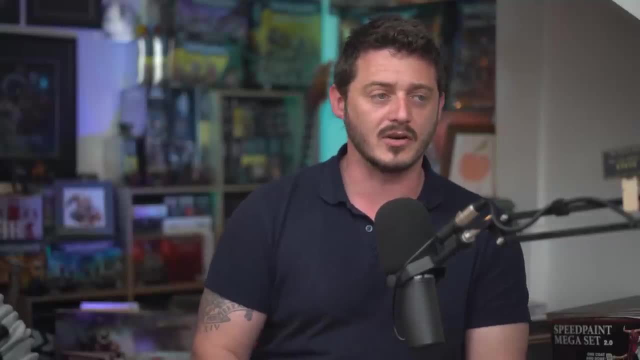 Um, but yeah, before, uh, before I've been, I've been a nine year old. I've been a nine years now, uh, which is absolutely amazing. Uh, it's just, it's flown by by um, but before that I was Marines, uh, for sort of. 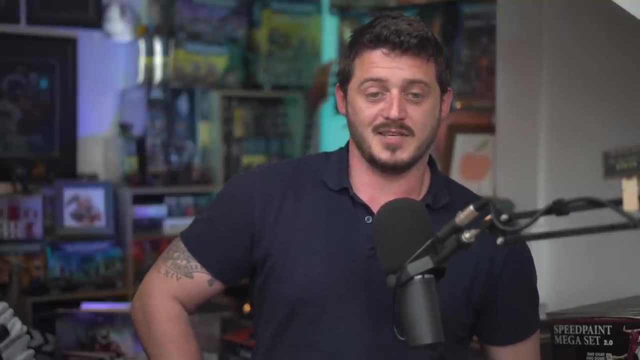 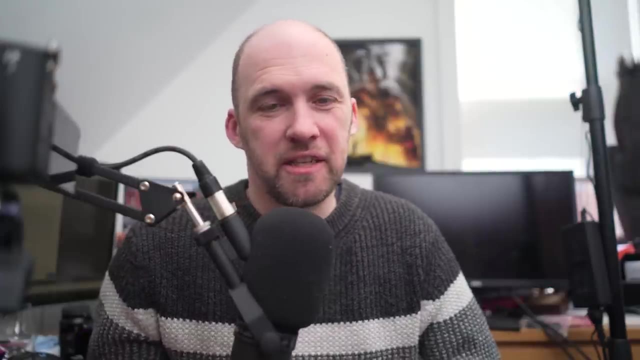 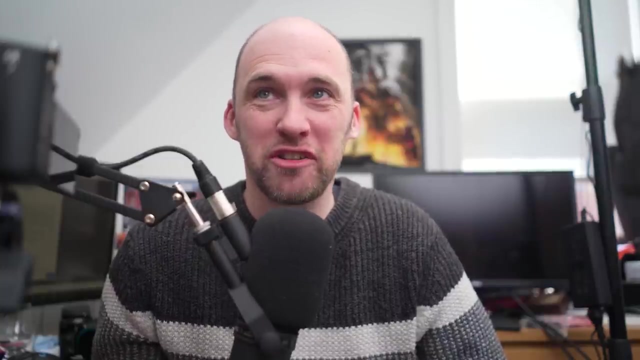 four, four years, And before that I was a. I was a young lad- I mean, Jeff would obviously appreciate that- And I was in cadets. uh, probably a lot of our viewers, being a Marine isn't easy. It's not like yeah, but it's such a hard the the the recruitment side of it. 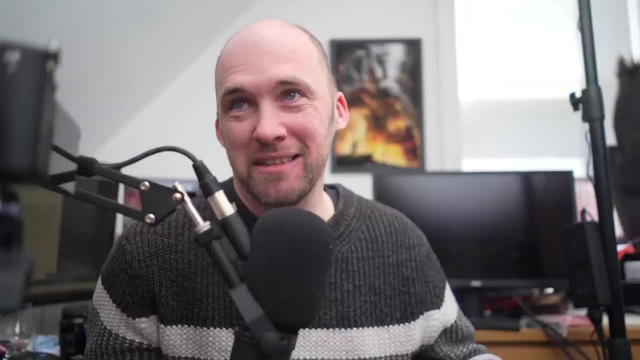 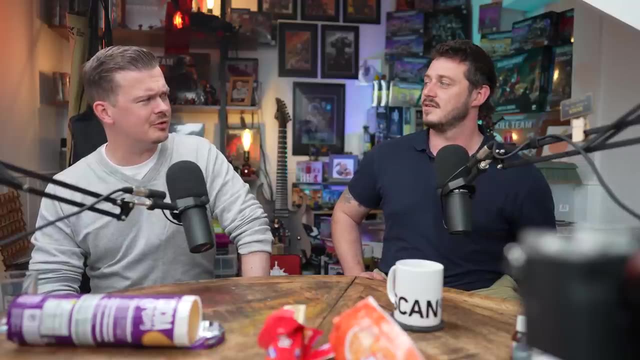 Uh yeah, it says a lot about a human to be able to just get selected. Yeah. So yeah, Cracking job. You tend to. obviously your brain forgets all the bad stuff. So I look back. I mean it was because of stories you've told me. it sounds pretty. 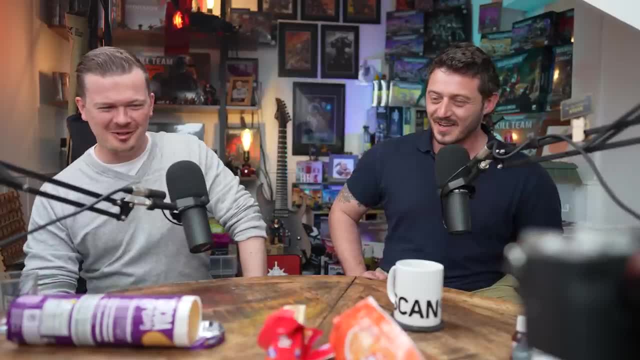 easy the times you were having on the ship. So every time I'd call home from some random country, I'd be drunk and I'd be like, oh, mom, I'm in Albania. It's like, oh, I'm in Djibouti. 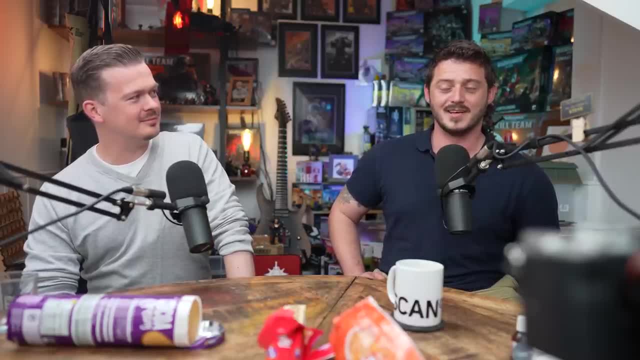 She's like, oh, I'm in California. It's like I'm having a great time, but the brain forgets the bad stuff, Yeah. So I look back, my, my little cousins Just passed out of Marine training um October, November, and it's like: 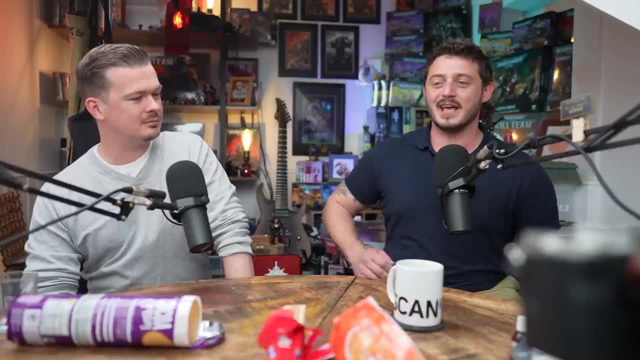 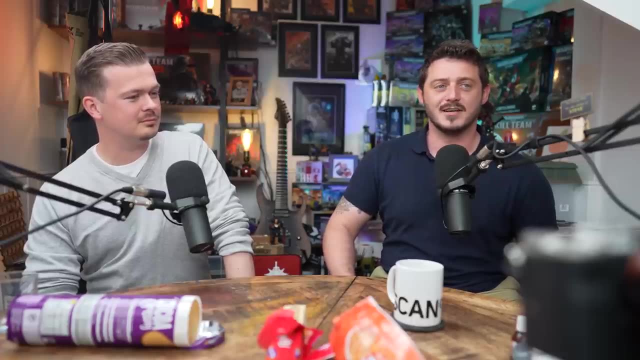 I'm proud older cousin kind of thing, And, um, yeah, I was hearing all his like nightmare stories fresh. I'm like, oh, I do remember it, like that I had a great time and it's just like: no, no, I probably didn't. 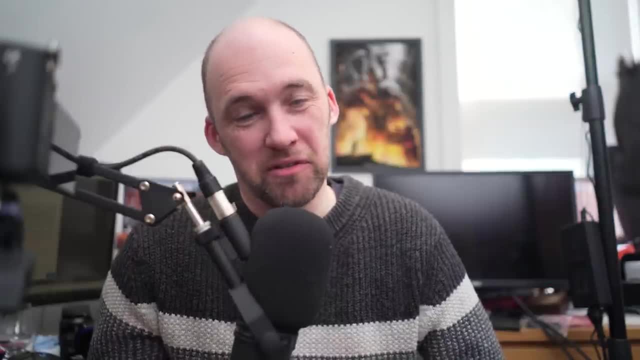 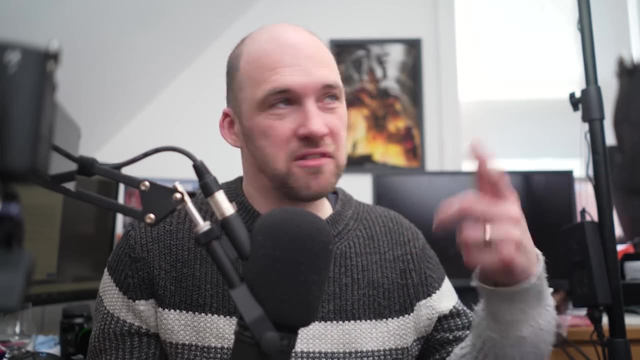 It's just. I remember watching a documentary It was. I can't remember what the ship was now, but it was just Royal Navy ship. Yeah, It was a TV crew there. I think it was like BBC kind of documentary And like one of the officers had just taken, the TV crew ran. 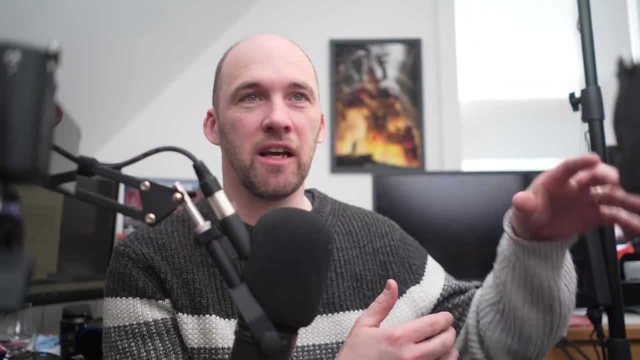 There's like a bit of the front of the Ship where there was like I think they had like some games going on and they had like a load of like um plants just all bushed up just to add a bit of greenery. 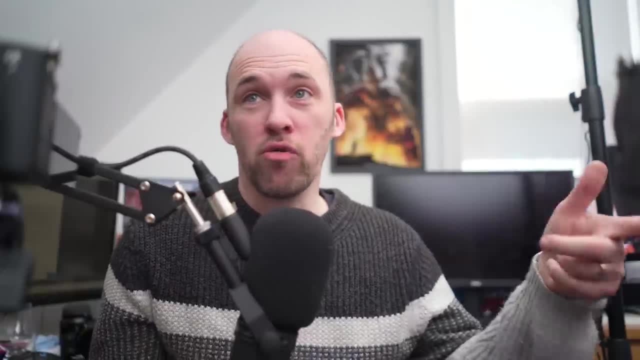 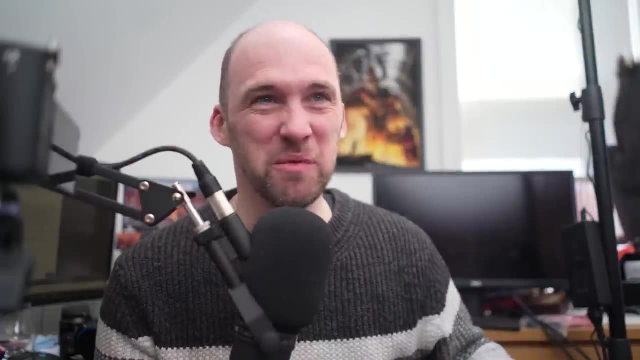 to the ship. It's just gray, Yeah, And it was just like walking around going. oh, this is where the Marines train. I don't know if you can see them right now, but they're probably in there somewhere and it's carried on a couple of it's like they're all losers. 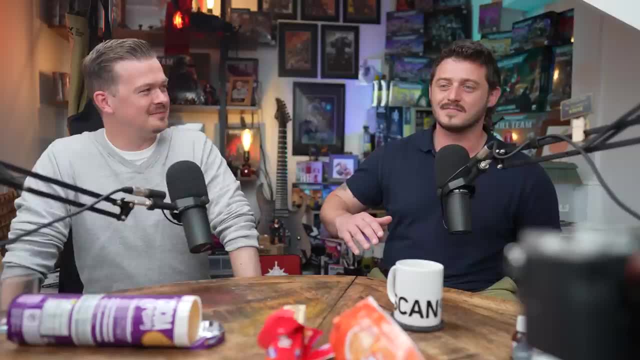 We don't get on with them, We just leave them here. When I was on ship, they just shoved us on a real low level And they were just like, yeah, they just leave them alone. Yeah, It's just leave them to do their own thing. 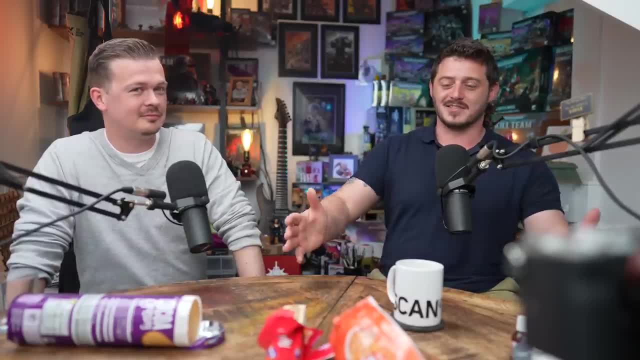 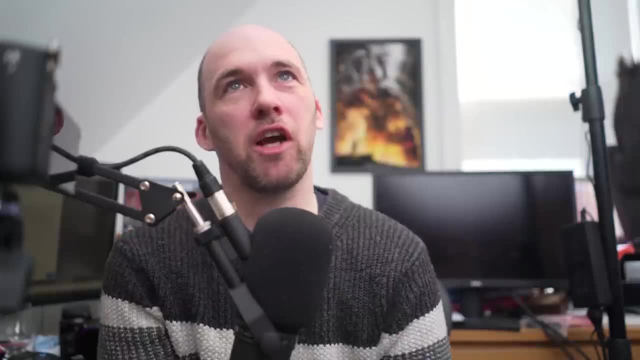 Just let them they'll, they'll entertain themselves. It's just like having a load of toddlers and shuffling them a load of toys and be like they'll keep themselves busy for about a day or two, And it's like, I suppose, as well from that point of view, like a ship Marines. 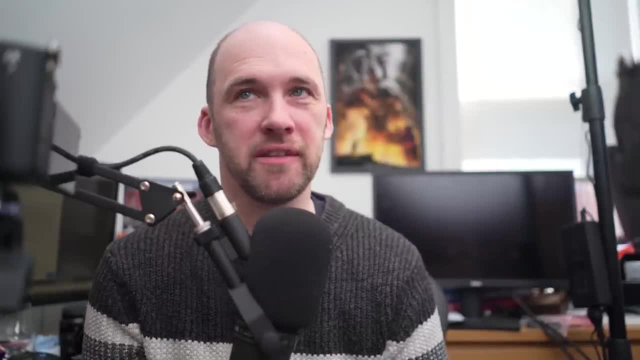 when you watch a lot of sci-fi, you have ships and, like enterprise, they end up having the. the makers don't they, Which are, like you know, the, the armed element of, like the, the Starfleet crew and stuff like that. 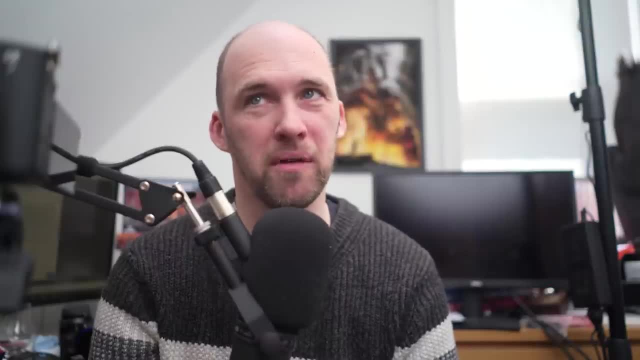 So when it comes to like doing your, your sci-fi kind of stuff, you're like I know, I know about this, I know what from a, even though it's naval on the sea, it's a very similar, it's um. 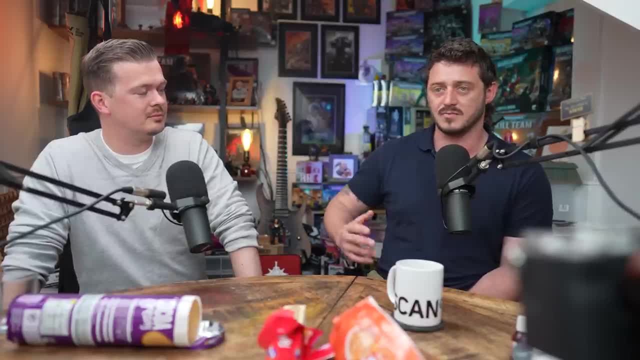 having a force Is Background has helped um designing the models, making sure, like the kneeling position- there's lots of kneeling positions It's to take, especially when you're firing a rifle, but some of them just aren't comfy and they don't. they don't work. 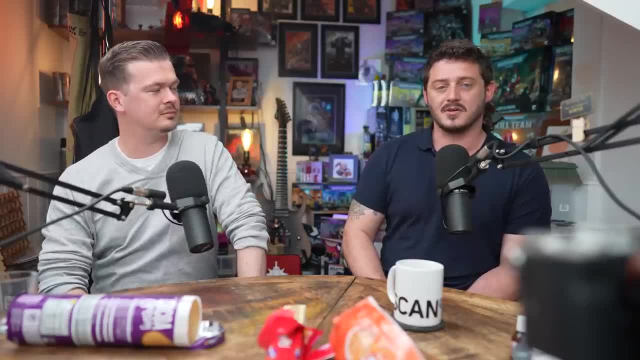 You see some models taking a knee and it's like that's not a good firing position. Yeah, That's, that's not going to help you at all. You might as well just stand up. Do you know? my my favorite fine position I've ever seen? 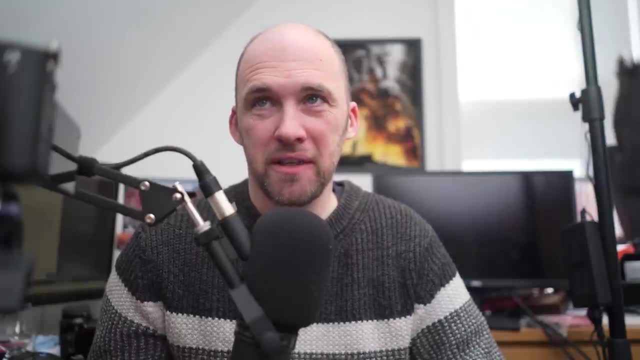 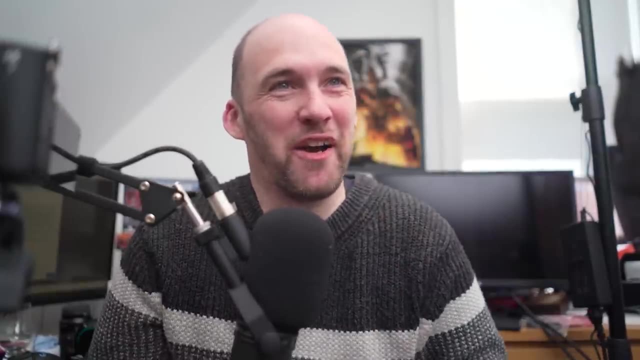 It's really old school. It's like: do you know much about Napoleon X? Yeah, So British rifleman used to do a thing where they're just like lay back and then cross their legs, Yeah, And then just steady on the, on the, on the. it's like chilling, enjoying the. 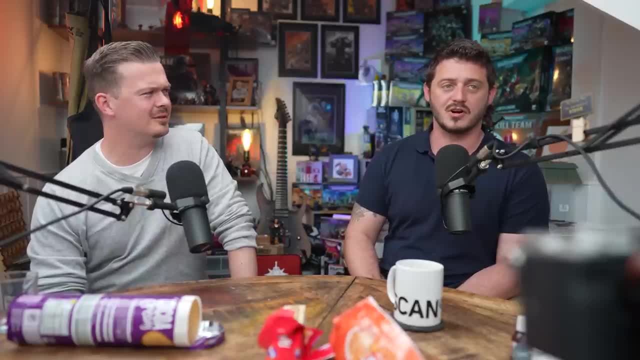 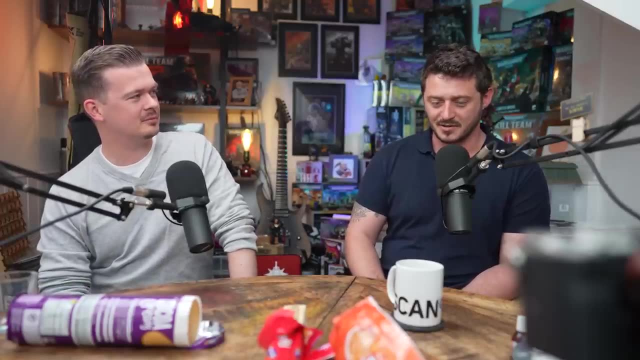 holiday poking away at some. it's: it's a great way of just makeshift tripod. Yeah, it makes perfect sense. Yeah, it really does. Um, one of my favorites was: you just sit down and you, you kind of like you do. 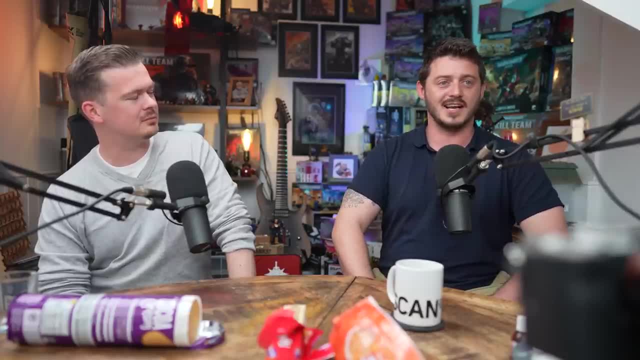 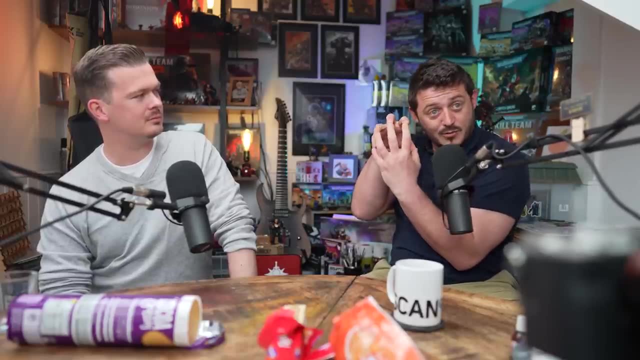 you bring your feet in, you do the stretch, uh, to stretch the inside of your legs. You just do that and you pop your elbows in and you hug it nice and tight and you're just this little, Contained little ball. It's so comfy. 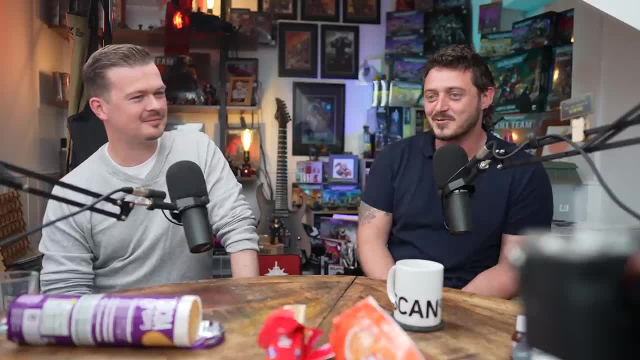 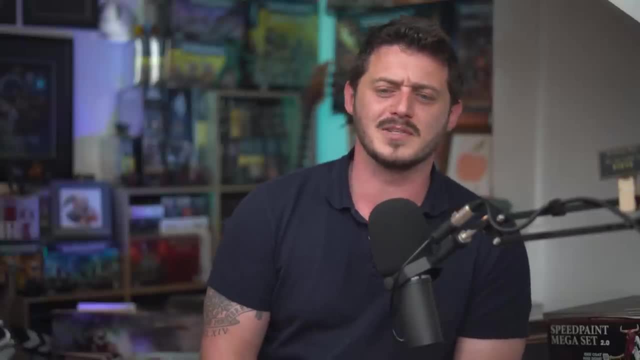 It's just so comfy sitting on a hill and just like so comfy right now. It was always a good one, Um, but no, it's things like that always work. Uh, it's good fun, Um. people always thought: well, I left the Marines, I think Feb 2014, and I 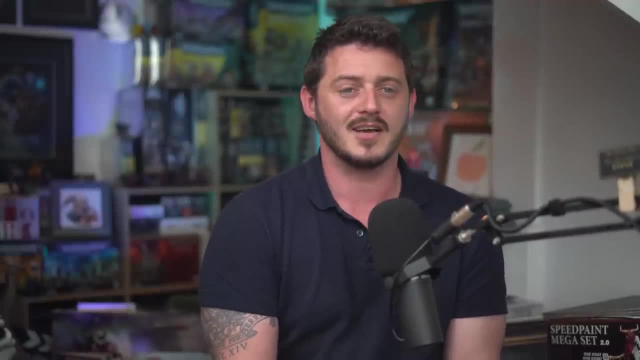 literally started at the zoo March 2014.. Oh, wow, Um, I started in the gift shop. Yeah, Uh, yeah. I started right from the bottom cause I was like there's no way I'm going to jump straight in, but I'll give myself a five year plan. 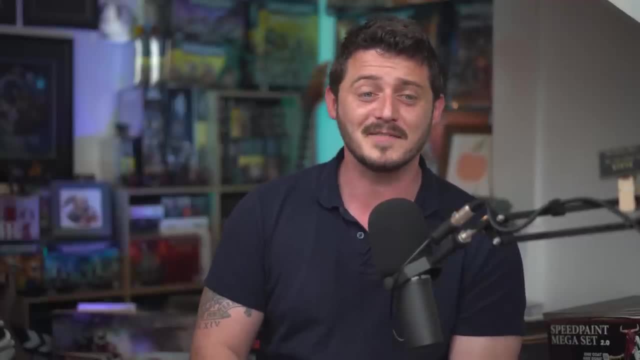 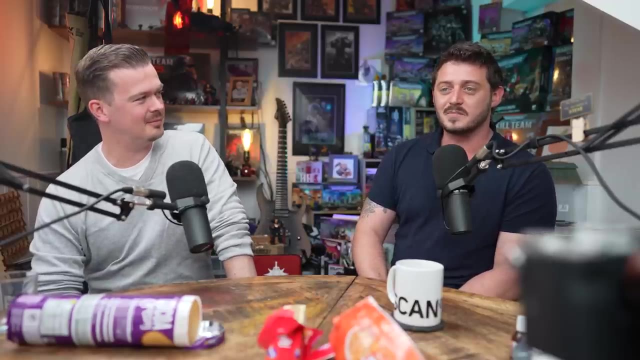 And There's one thing: the Marines- and, well, military in general- give you hits, the gift of the gab Jeff to everyone. We've got Jeff. So, yeah, exactly, You know it. and uh, yeah, start chatting to people like come rain or shine. 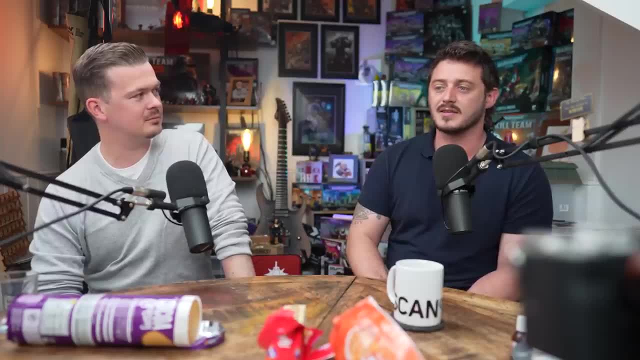 I started like volunteering, helping people out even during the rain, and they couldn't work me hard enough. There was no way. it's like you've been here a lot. He, you're not tired, I'm all right, All right. 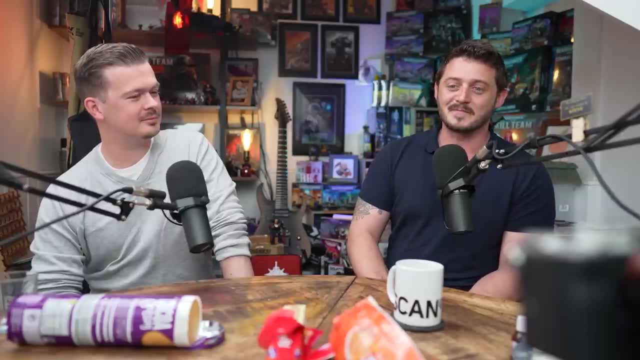 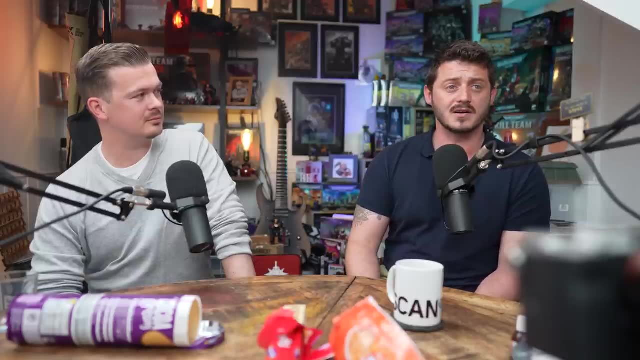 Yeah, I'm fine. That was still fit back then, Cause I just come out, Um. and then he ended up getting me into chatting with some nice people and eventually, a few months later, I've got one of the speaking jobs in the park. 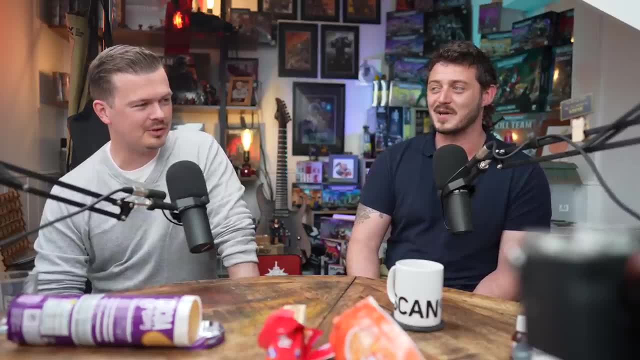 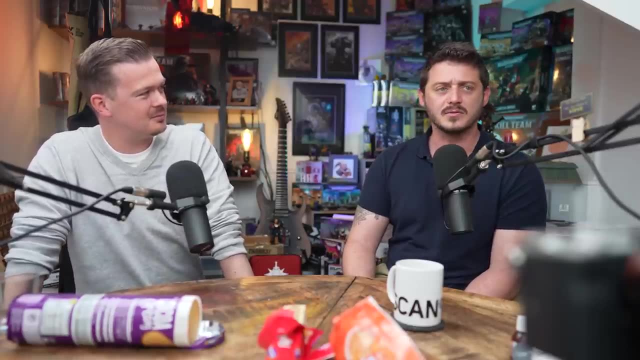 Um, I'm a very loud person, naturally, So, speaking to a lot of people, the speaking job suits you better. And uh, yeah, it just worked out from there, and people are Marines to animals, It's a bit of a jumps. 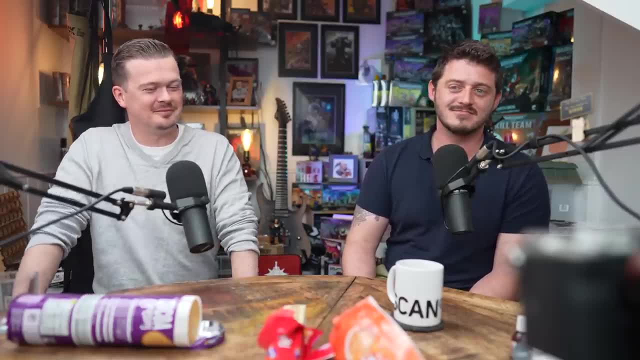 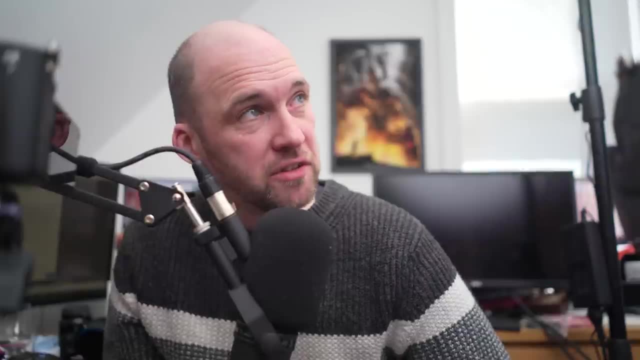 And I'm kind of like gorillas anyway, Aren't they glad you said that. happy gorillas. How are we doing for a percentage on battery? I know you've checked a few times, Oh uh, no, Yeah, we're fine. 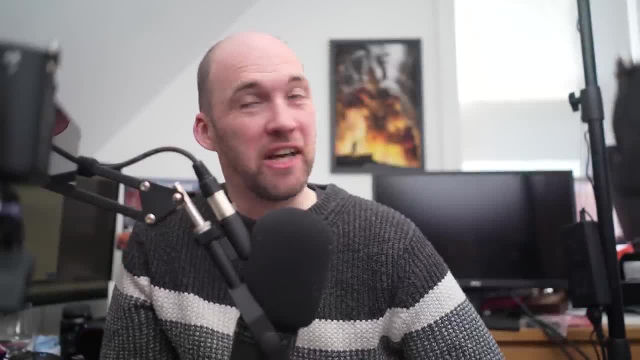 Oh, that's good. Do you want to go to some page on questions? I do. How's yeah? Cause I know he's been egging. I can see: Oh yeah, Wicked, We've got. I've got a few. we, we asked, we asked our patrons. 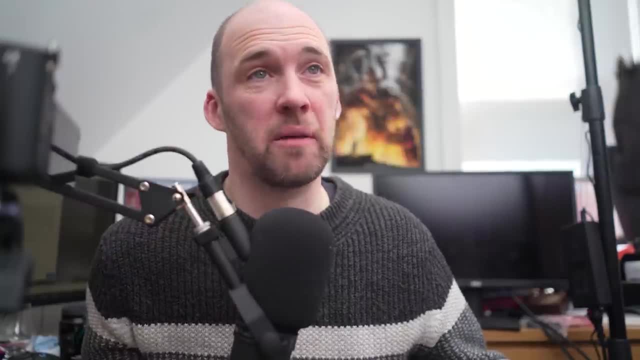 We always like to give them the opportunity to to check nice. Some of it might be the same kind of stuff we've covered. Well, it's good. Yeah, Cause I saw the one where someone asked a question about mashed potatoes and I 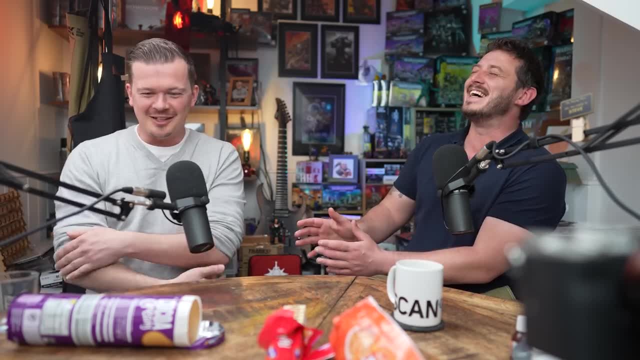 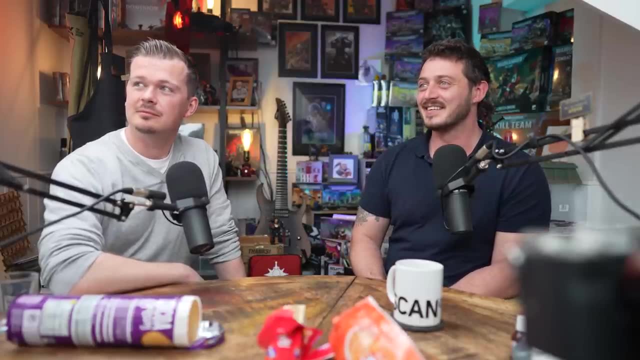 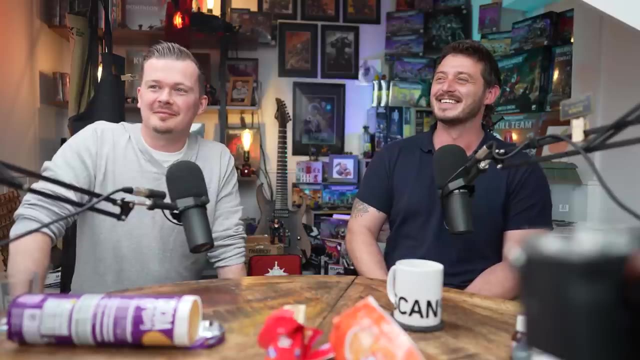 think it was. yeah, I mean we might even get them. I mean, to be fair, most of these are actually um, seem, seem quite sensible. Oh, fantastic, That's, which is almost almost disappointing. Um so uh, someone has asked what considerations went into choosing resin. 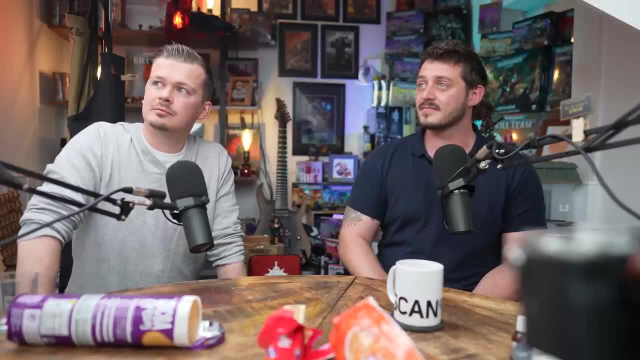 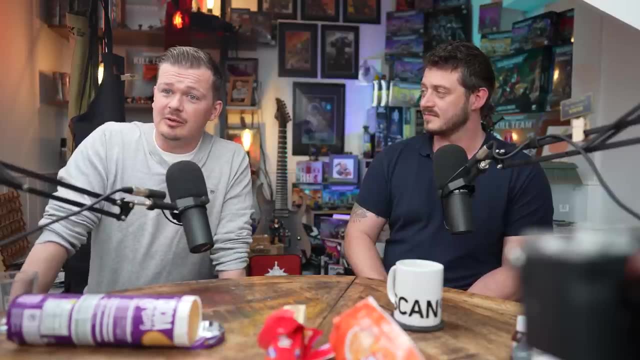 uh, for the miniature material. Uh, did you look at any any different, any different options? We we've looked at lots of options. The main reason why it's resin at the moment is because the way we're doing it is obviously we've designed that and we're we're 3d printing them ourselves. 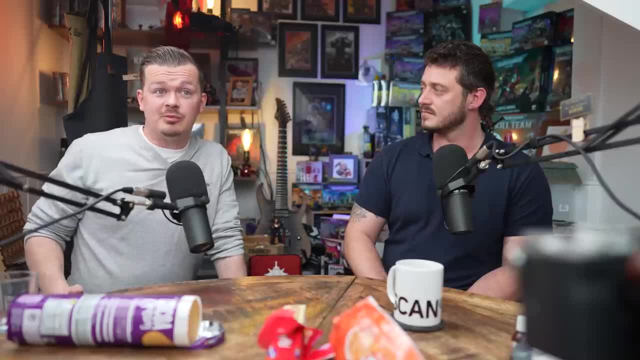 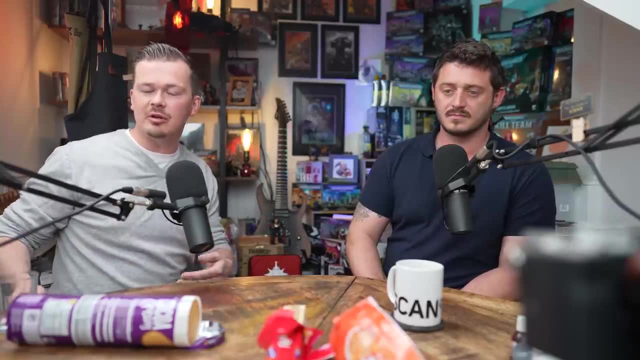 Yeah, Um, obviously moving forward, that's probably going to be the best bet, Um if the Kickstarter is wildly successful, or even if it's not, and as the business grows, um with the volume comes obviously different ways of doing it. 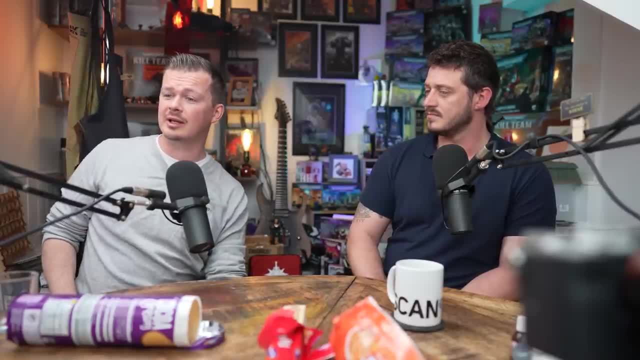 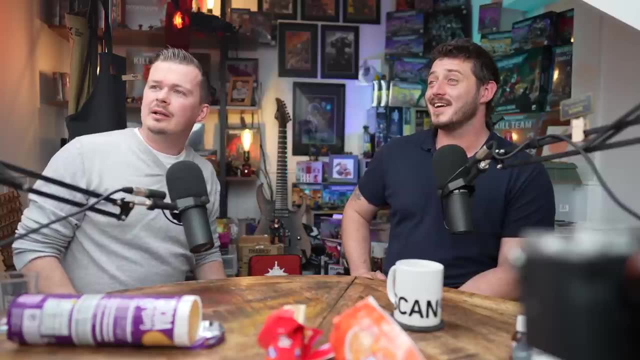 You can have a CO cast uh, which is again in plastic, but it's uh. people that don't know it's uh. there was a goober town video about it. Yeah Yeah Good, That's a good video as well. 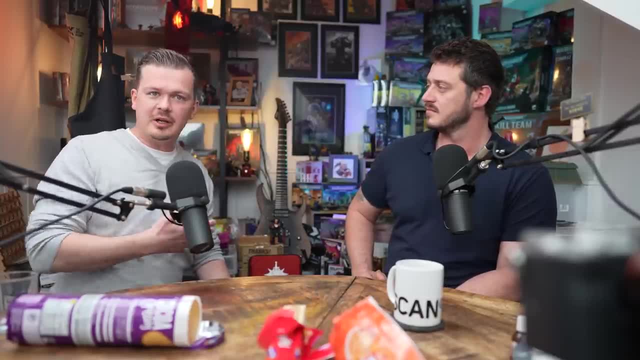 Maybe a year or two ago. Yeah, Cause generally it's because a lot of bigger companies you'll see plastic sprues what you're after and then you got to pay quite a lot to have those CNC machined aluminium. Yeah, 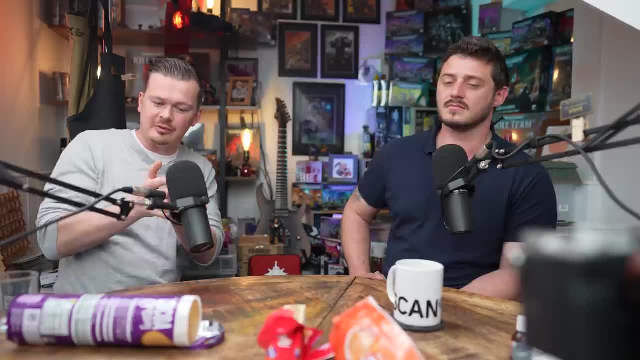 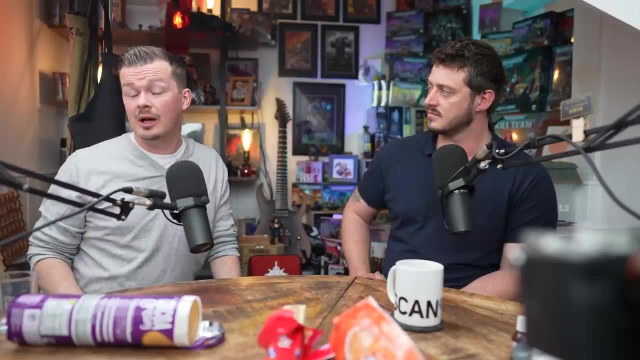 Blocks and then it gets injected in, But obviously you can't have any underhangs because the moles have to come away. But CO cast, it's hard rubber So it's a little bit more forgiving and accessible. for yeah, So we're not saying it will always be resin. 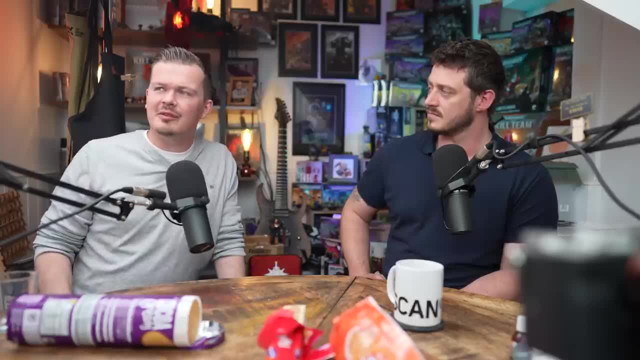 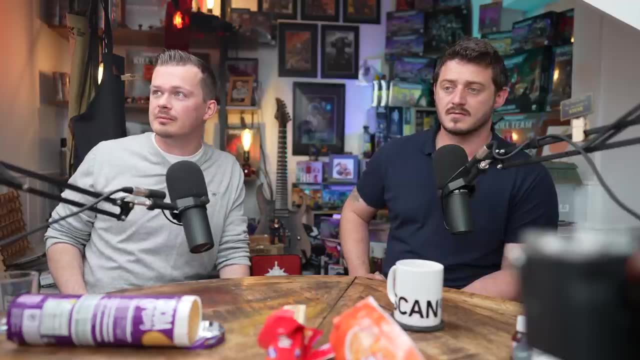 Um, resin gets a bad rap. I don't seem to have any issue with it at all. Um, far off. I have no issue with paints. nicely, Yeah, The. the quality of them was yes. Okay, You've got to use super glue instead of plastic. 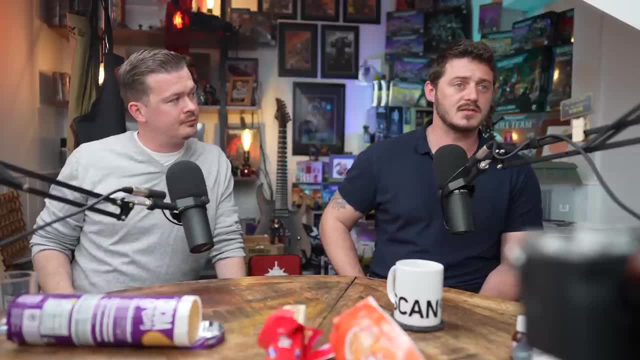 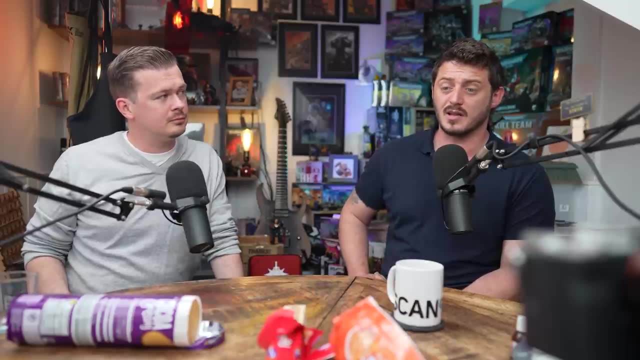 Glue: Yeah, yeah, yeah. Um yeah, Paints up nicely, As you just said. I've not had an issue with the paint Not sticking to it or anything else like that. Um, just I felt. I actually felt like the cheaper super glue I'll go, the nicer it sticks. 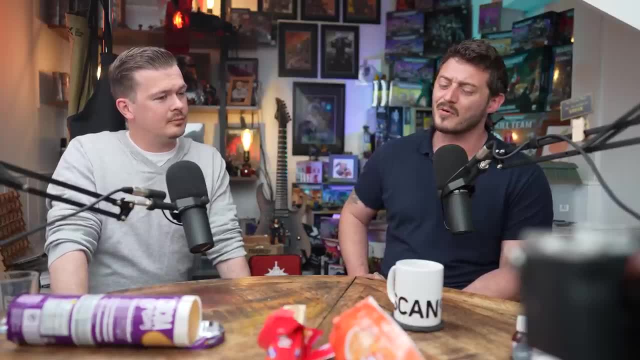 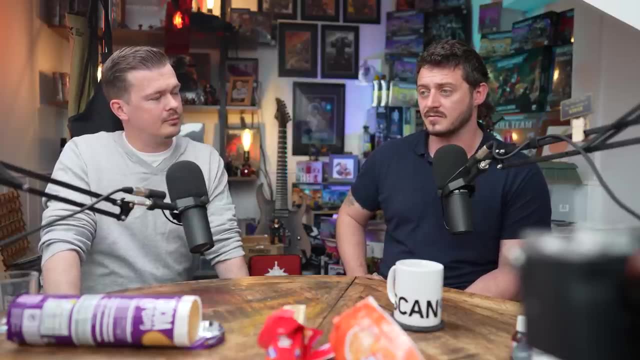 Yeah, Yeah, Yeah. I just don't, don't look into it too much, but different brands of resin and everything A lot of the time- Well, actually not a lot of time, but in general, again coming from a background of doing everything, 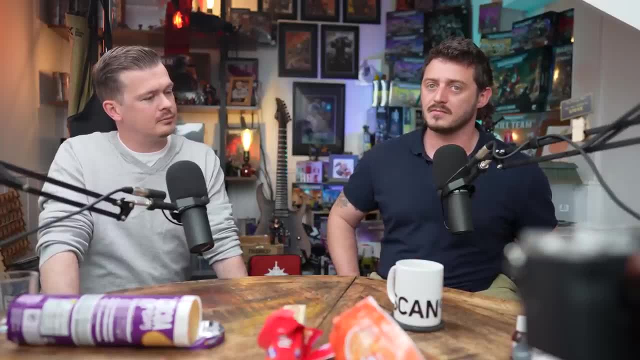 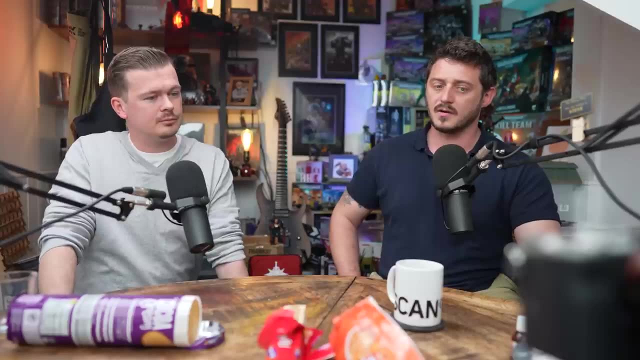 at once designing the game. uh, there's not been a lot of time to hone in and become masters of one specific skill. So, uh, we are like followers, Okay, Of a lot of 3d printing groups and everything where we do get a lot of like tips and tricks. 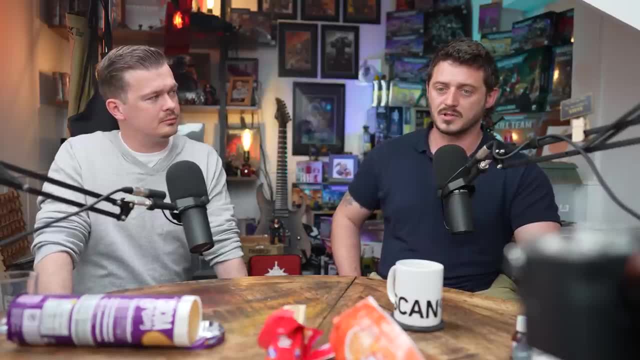 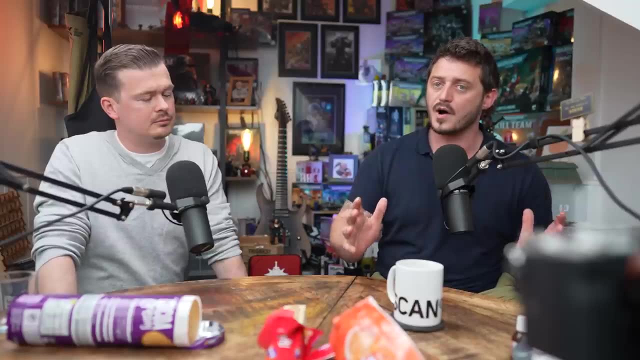 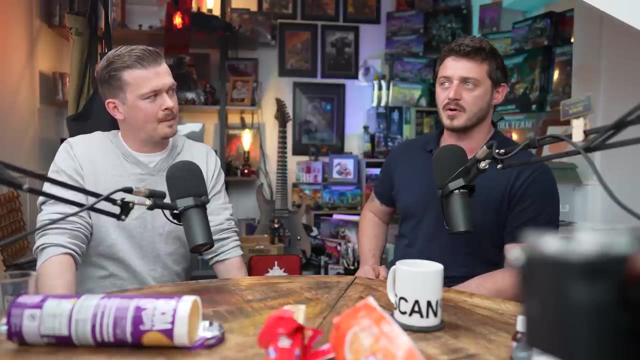 and things like this. But I haven't got all the time in the world to just hone in my, my, my resin brands and dialing, my settings and stuff, which is a shame because it probably could get far obviously perfected minis. but um, there, there is best of quality as I can make them at the 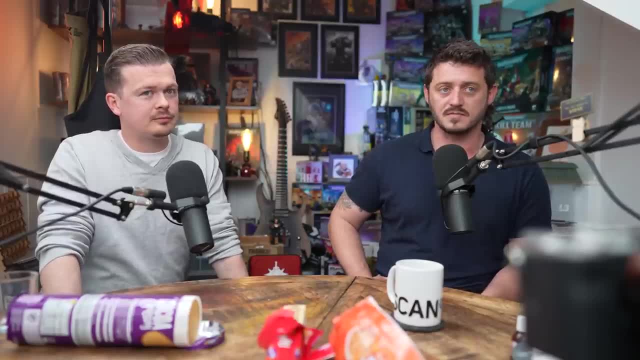 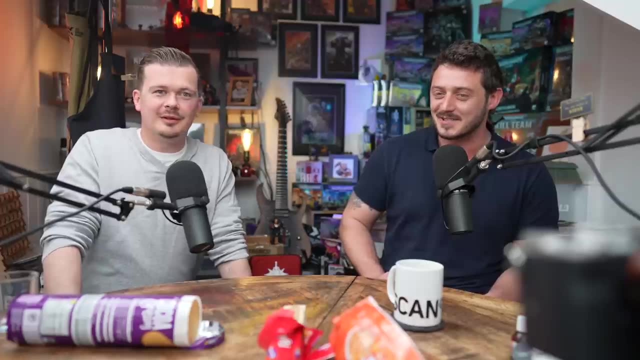 moment, Yeah, And I just use any cubic resin. I just found it. It's really straightforward and simple. I I'm happy with that And I'm a bit scared of chin. It's just like I don't want to check, just in case. what they might mean is because sometimes 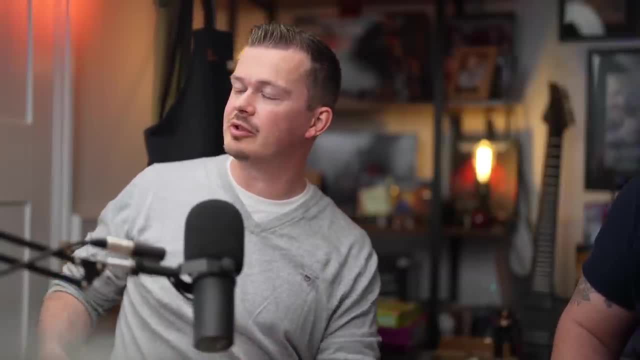 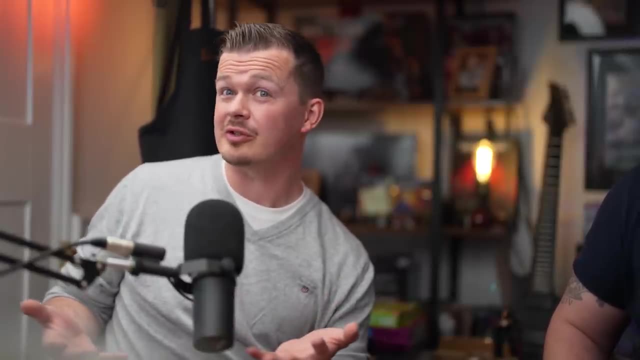 you get, or especially when you're at conventions and people are selling stuff they've- yeah, they might not have cleaned it, or that's quite a big and it's lots of videos online because obviously it's quite a toxic product you're working with during the process. but as long 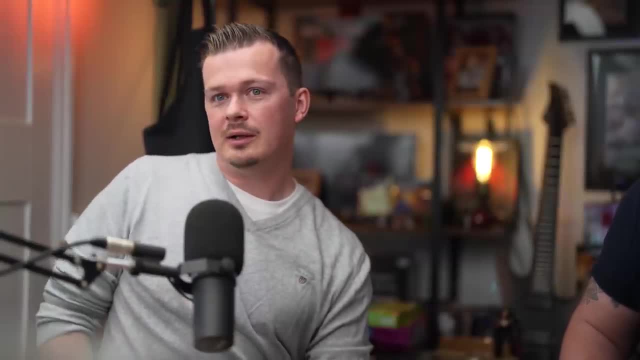 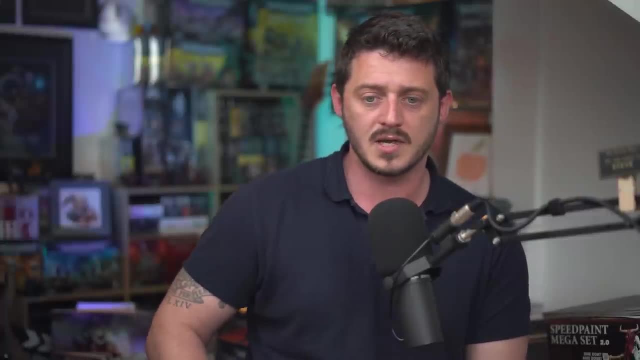 as it's, everything's cleaned and cured and we do, yeah, it's all. yeah. Last year at UKG, uh someone uh went to pick up One of our primary models- uh, just the Tesla Marine- and was like: uh, no, I've, I've bought. 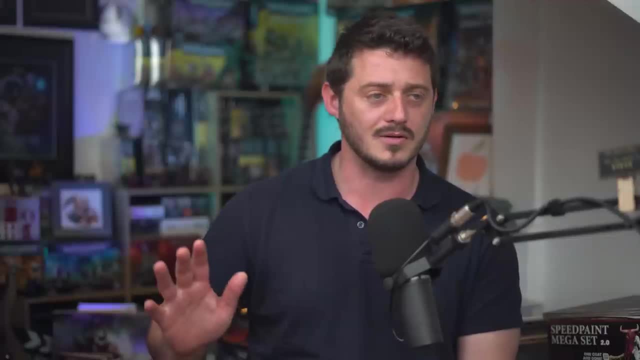 a resin mini before and it had all the supports on it and I was like: whoa, no, no, no, Like I've made sure I've sounded it down and taken all the supports off and it's just good to go. They were surprised. 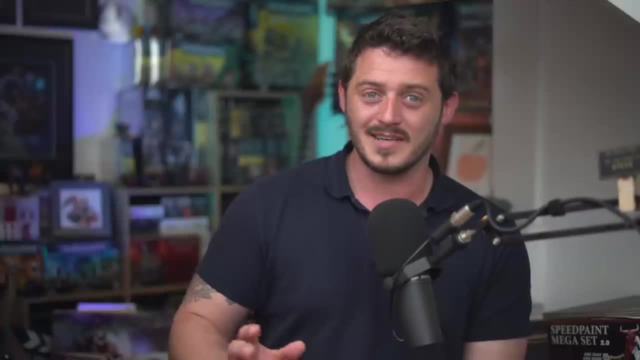 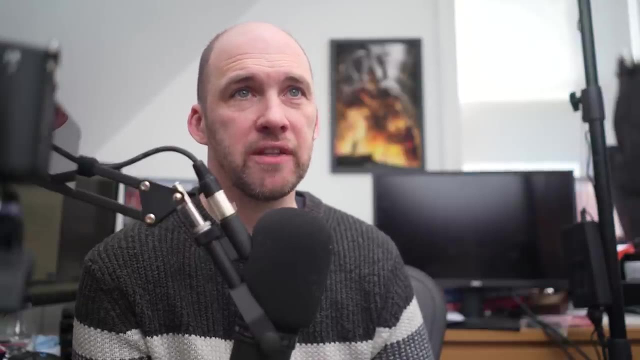 Yeah, I was like wait what People aren't doing that? Yeah, No way. This seems well. Yeah, I've got stuff with the supports on. That was weird. I was on the support, So a lot softer than the actual resin itself. 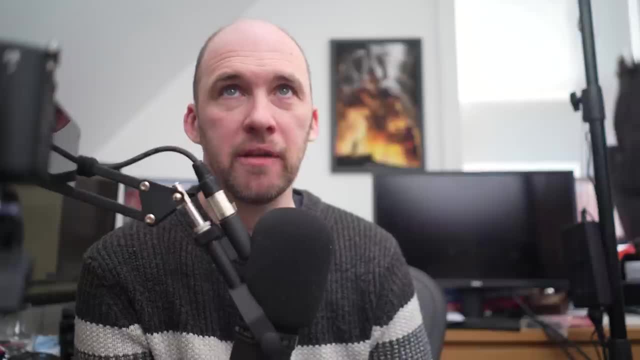 So you can just like pull it away and it's fine, But yeah, I get it, Yeah, And then you've got to start somewhere, Right? So our workshop started off with like frying pans, led point into like oh yeah, the molds. 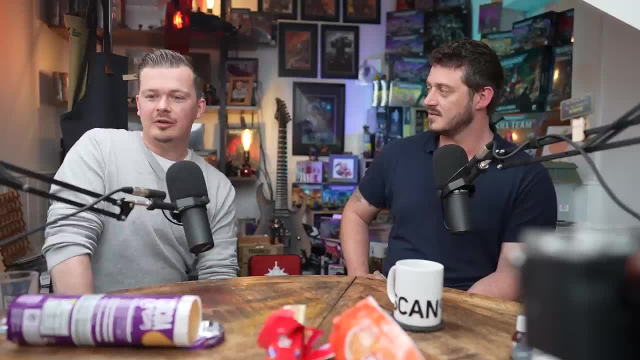 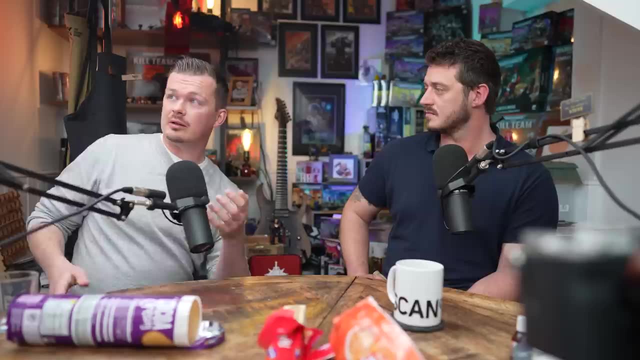 and look at what they make now. Oh yeah, Absolutely Yeah, Things, things will grow and evolve. Um yeah, I mean, if people are worried about cause, again that question might be in consideration of of creating anything like that. you have to um things. you don't learn until you're. 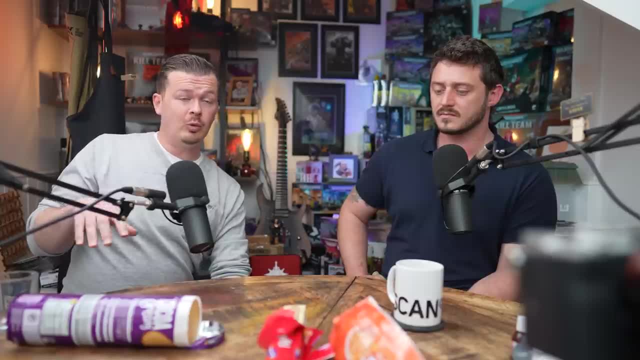 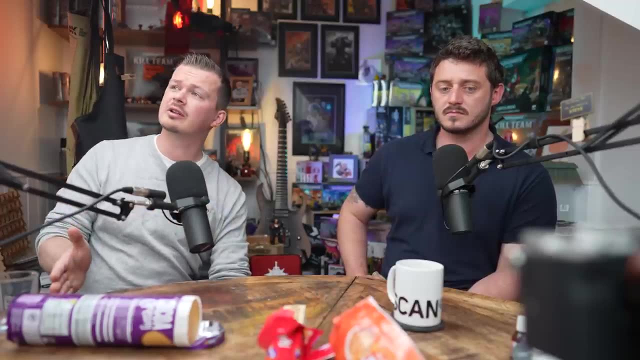 looking into it And I might not be a hundred percent correct on this, but we'd be putting for 14, plus in terms of age, the product, as I think quite a lot of others do. But if it's for anything below that, you have to get everything sent off to make sure it's. 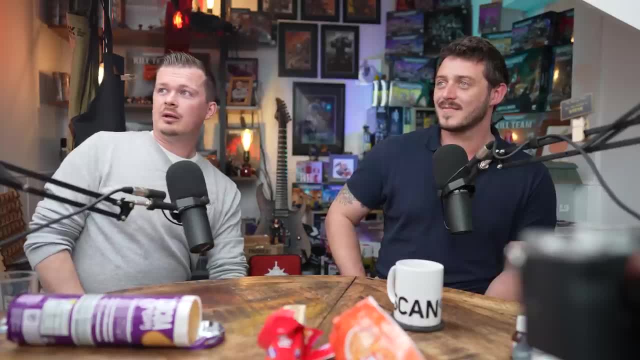 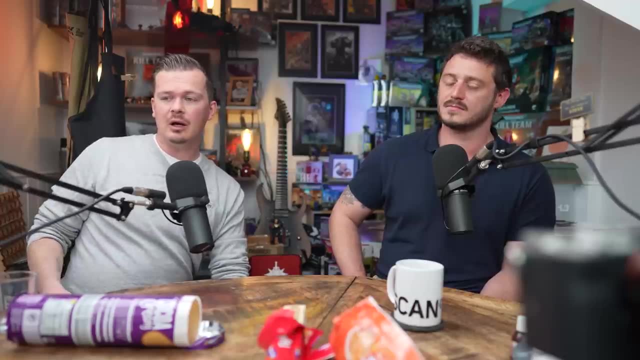 safe for kids. Oh, okay, In case they like: oh, this Tesla really tasty, small parts aside, like if you- yeah, if you're making a case, I think the plastic would probably be fine, as long as it couldn't fit down their 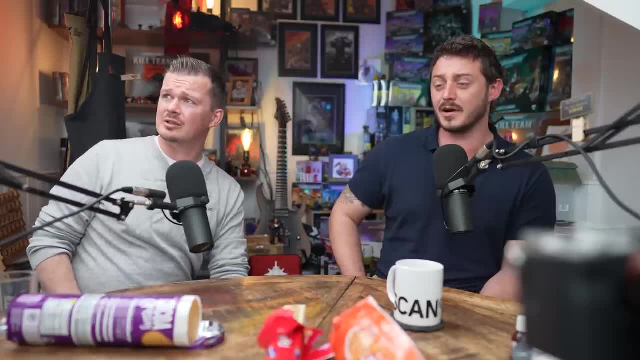 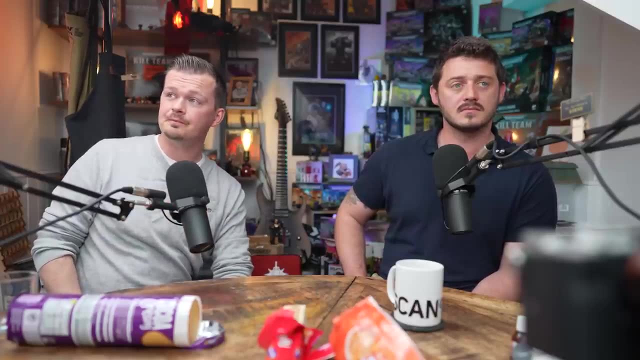 throat But uh, resin, I don't think you want to put that in your mouth. then different, different things to look at depending on what. but what we're designing for we, we think the residents find Yeah, I agree. 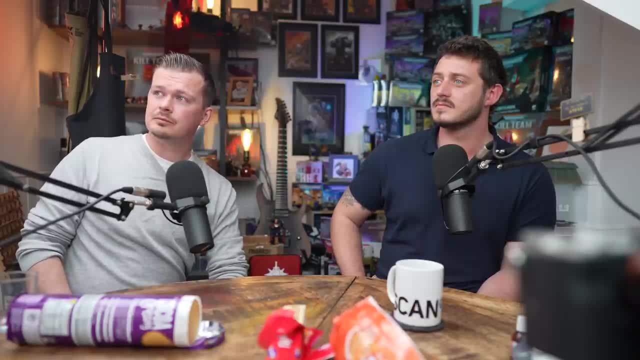 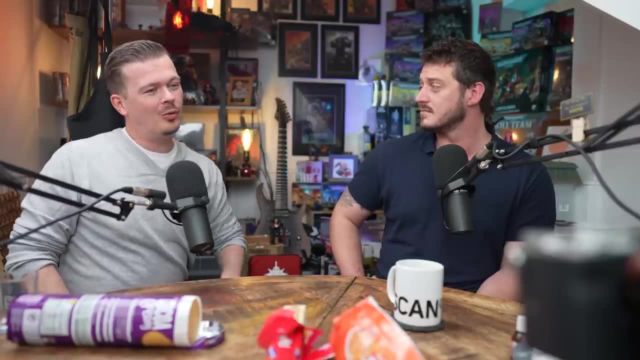 Brilliant, Yeah. Have you managed to sneak in any Easter eggs at all, or have you kept everything above board? The grays, most likely. There's things we've discussed that we haven't done yet. Things for the rule book, Yeah, Yeah. 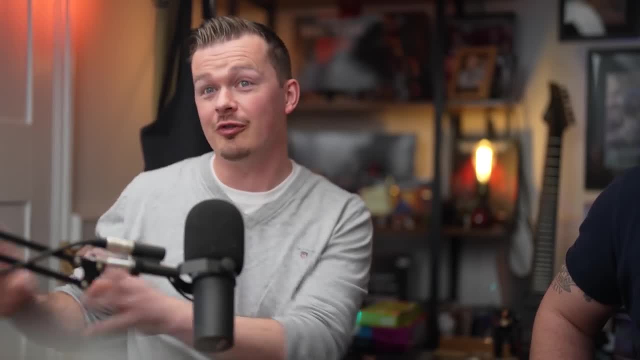 Um, which obviously is available on the Kickstarter, but because we're people like a book, so we're offering a book despite the fact that the rules are on online. Yeah, I feel like I want to say what it is, but not what we're going to do. 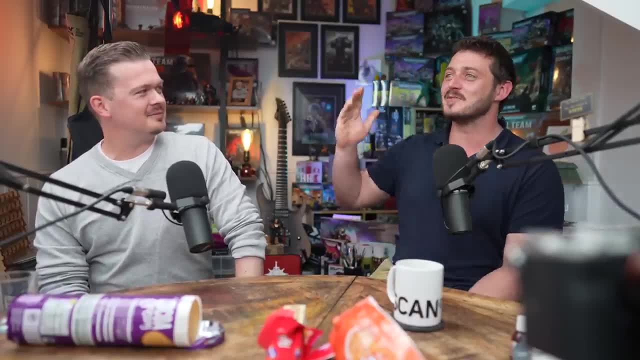 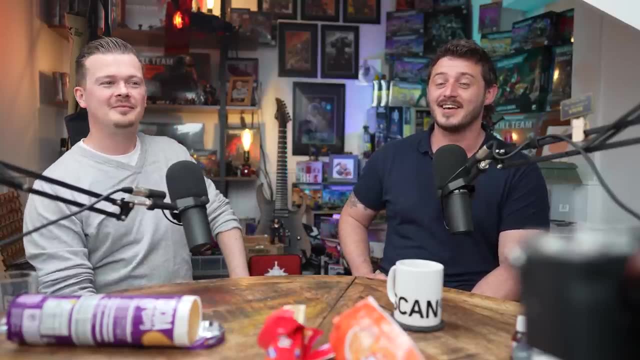 Or don't. then Keep it secret. Keep it secret. Keep it safe. Yeah, Keep it secret. Yeah, Um, yeah, Nothing. The answer is: buy it and find out. Yeah, Yeah, It's behind a paywall. 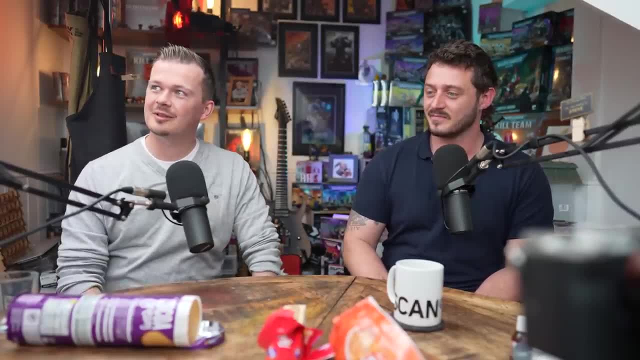 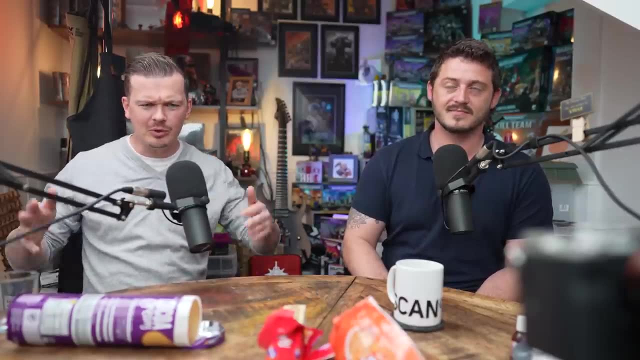 Nothing, Yeah, We're. I'm a huge fan of. I remember early days of YouTube. There was a lot of. it was finding the Easter eggs in movies and games and you end up going back and watching Titanic cause someone's told you there's a cow falling off at halfway. 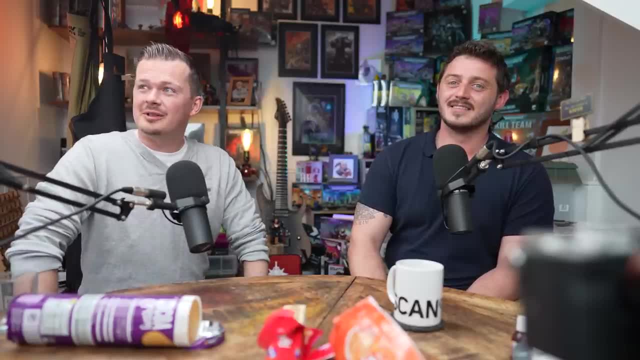 time It's there, Yeah, So we, we are putting bits and pieces in and there'll be lots. there'll be lots on the website, on the website, and there's certain certain things in the way we've named stuff as well, which, yeah. 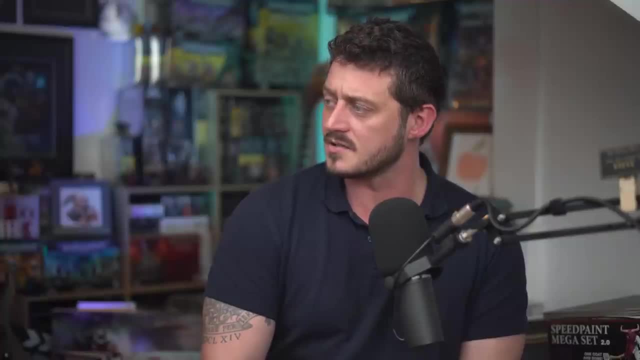 definitely the planets that you named and everything else, like in the star systems. if you go on, like the world's tab on the website, alex has come up with amazing graphics for like the star systems and everything. it's all linkable. you can click on them and we want to add in all: 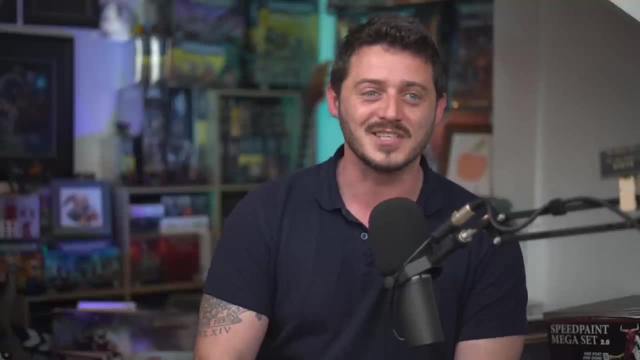 the information, even like how long it's. how long is it going to take you to walk to this random star from earth? oh, why not? why not? um? but a lot of the planets didn't have names. so, for example, in ursa minor and ursa major they're latin for bear big, bear little. yeah, yeah, um. so a few of the. 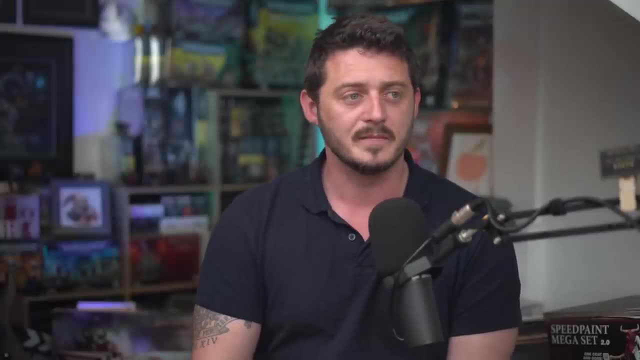 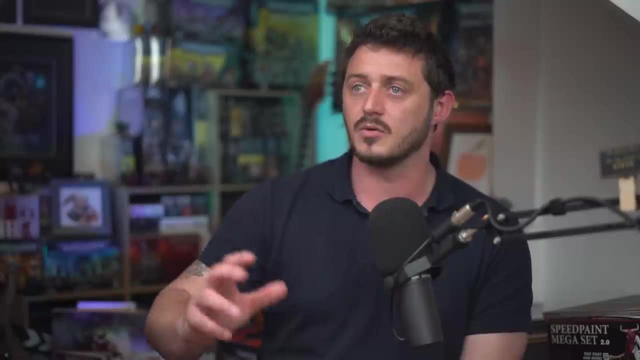 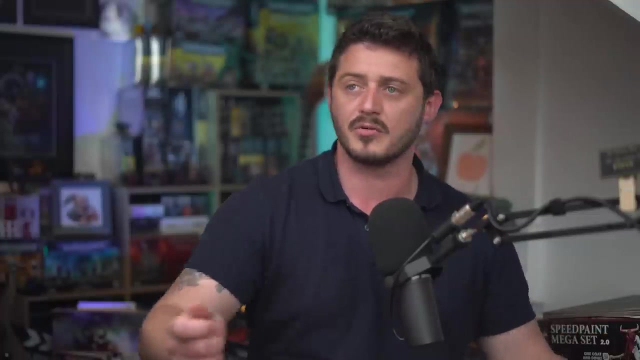 planets within those systems are just named after different bear species. nice, we thought it makes sense. and then there's uh draconis star system. so you found different languages or for uh, or different dragons through mythology and folklore, and then different parts of the dragons like claw, then separate parts from that. so that's cool. there's loads of stuff like that. we're, we're. 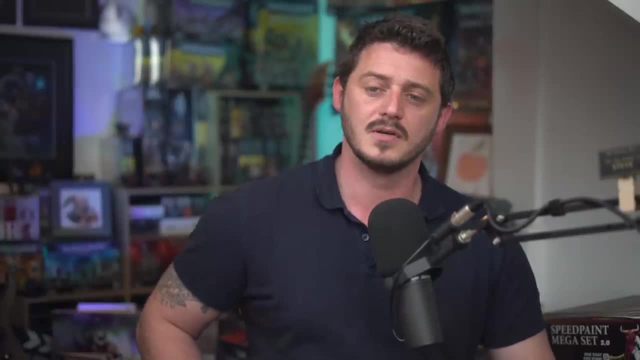 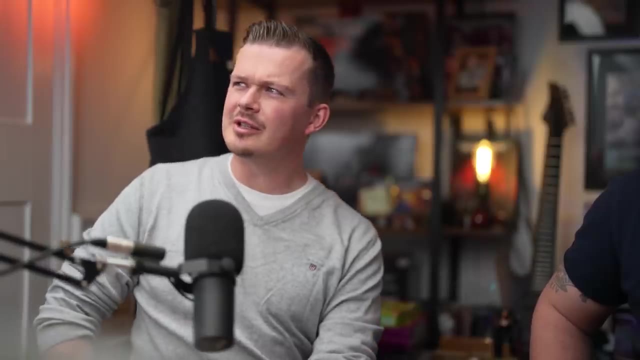 quite big in our into our etymology, um, so there's a lot of law or easter eggs- rather, they're not really easter eggs, they're surrounding names. it's nerdy easter eggs, yeah, yeah, like there's quite a lot of, because, yeah, again, we go into detail and a lot of this isn't on the website because it's. 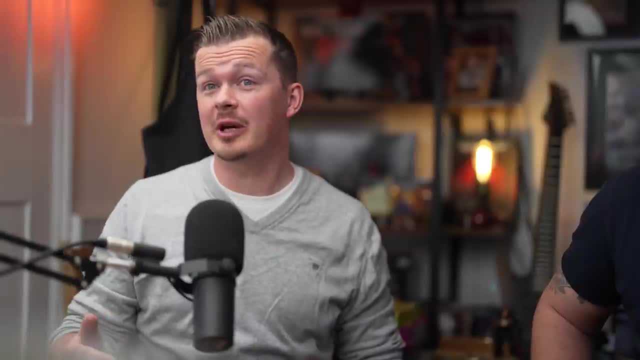 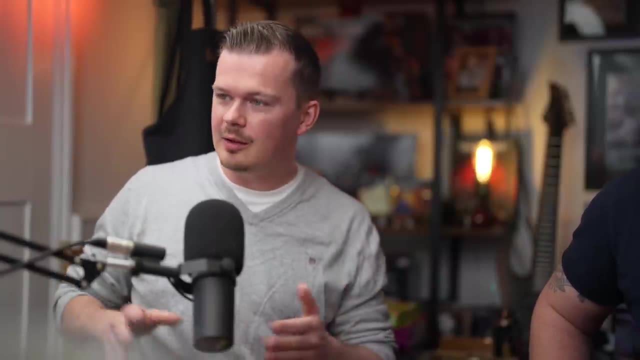 time frames, so more is being put, but we've made up scientific papers or pseudo-scientific papers to match the things and a lot of the scientists you might find their names are mismatched from characters in lots of- uh, sci-fi, yeah um, novels and films from way back. 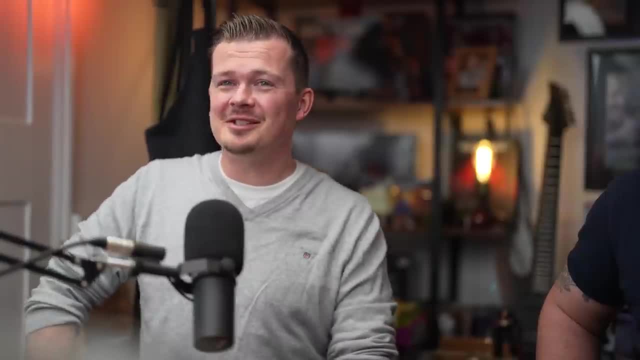 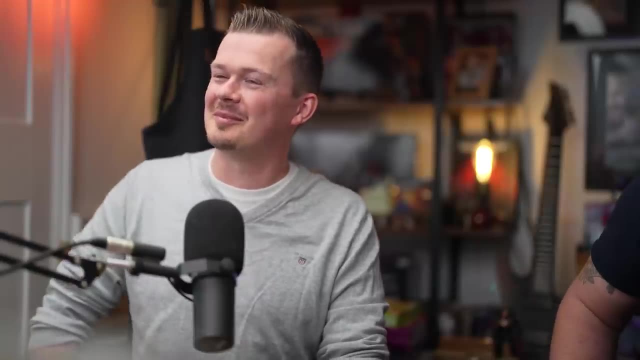 when so there's there's nerdy stuff to find, yeah, we're getting there, we're getting there. there's a little bit, yeah, they've all, but there's, yeah, there's a few bits, we're gonna a few bits, we were gonna hide- excellent. so, yeah, worth looking out. yeah, absolutely, because that's quite nice. 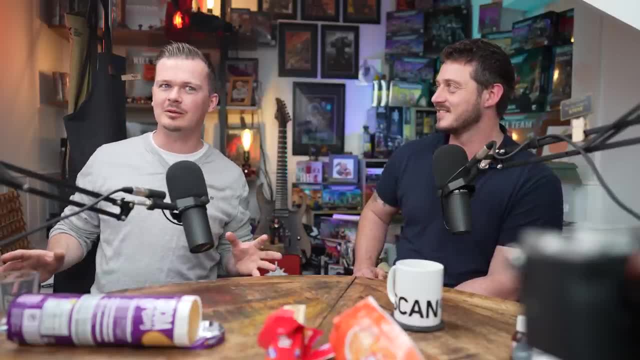 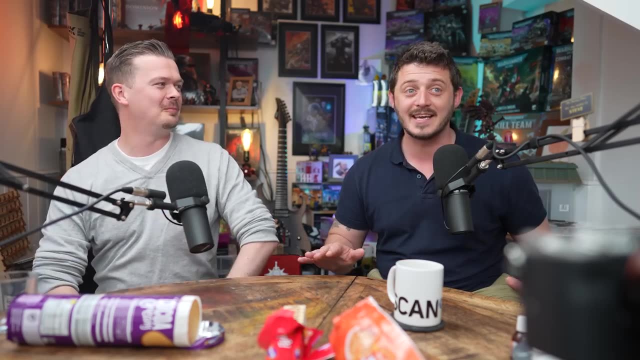 actually because you start to think: well, if you put it in and don't tell anyone, yeah, maybe no one will ever know. yeah, yeah, where you think that people are gonna start looking. so now, hopefully, at least this is when we don't put any in, yeah, and just look forward. yeah, i found one. 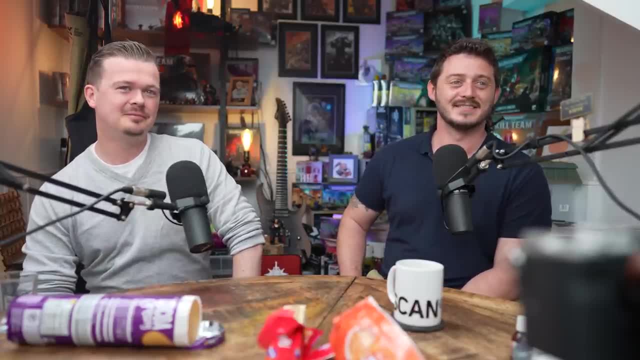 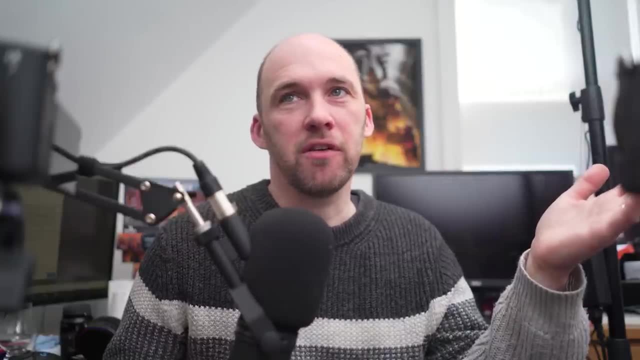 it's like: did you, that's the easter egg? there's nothing. i think fan of computer games, i really like like, uh, the elder scroll stuff and like oblivion and skyrim all have easter eggs from like movies and stuff. there was like: um, if you ever seen the film the goonies, yes, in oblivion. 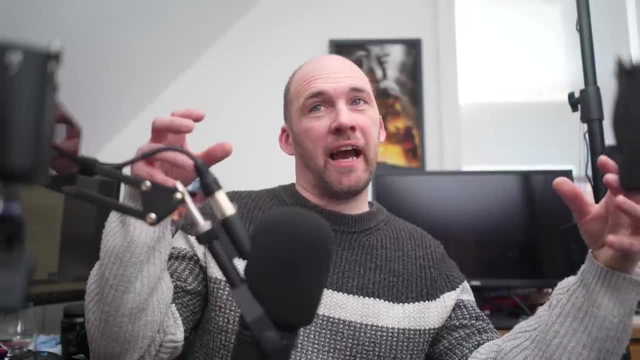 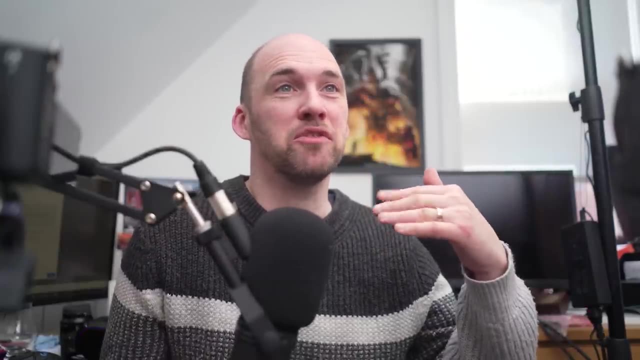 there's like a version of the goonish ship inside a cave. that's amazing and you can get like a cutlass, uh, like it's like a special magic weapon and stuff. but you have to. you wouldn't know it's there until someone had mentioned it and you have to like go on the internet and you have to like go. 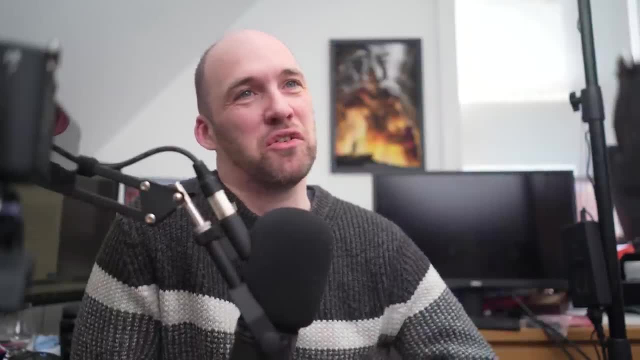 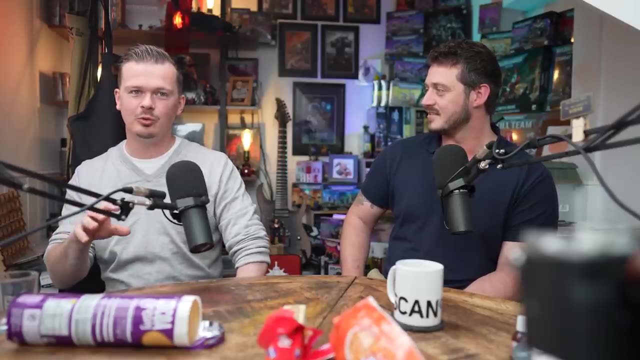 to that search. that's so cool: this cave and how you get down there. so there's all sorts of random stuff like that desperately trying. i can't remember any because, briefly in the car on the way here, one of the videos that popped up on like a facebook reel was all the star wars references. 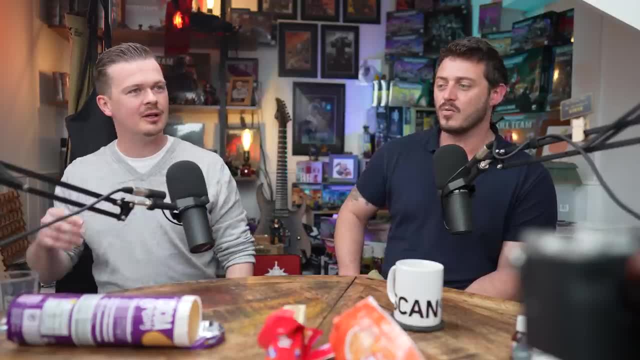 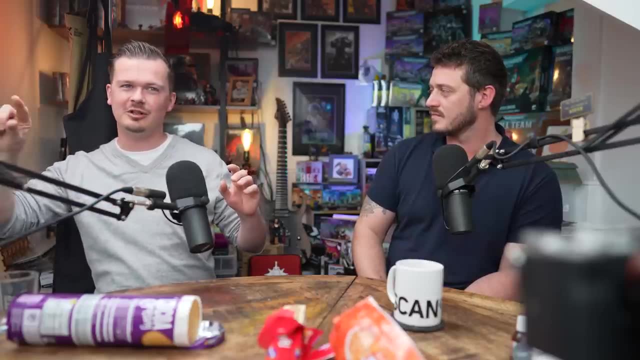 they made in video games. oh yeah, oh yes, yeah. well, no one of them tore through and went back in time to paris, and then then extra theater and it's got like in french: the return of the jedi and the day and stuff in it. well, there's, there's fun fantasy games always have a bigs and wedge. yeah, okay, yeah. 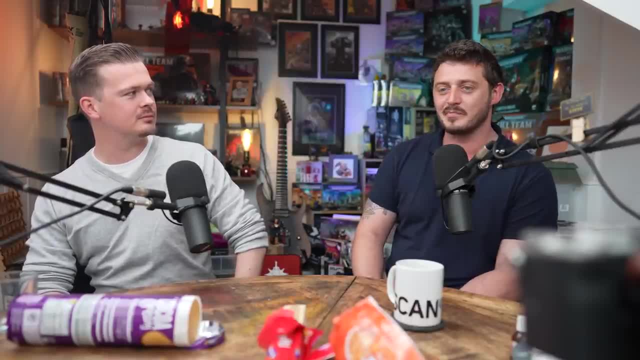 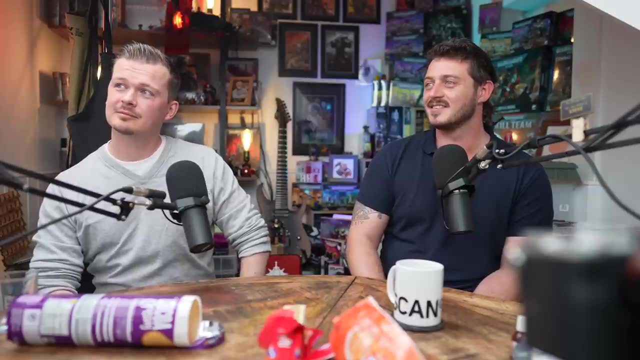 they were fans of final fantasy, the creators, and they just wanted to add in a bigs and wedge. yeah, yeah, why not? yeah, fantastic, okay. someone has asked- i think we talked about it a little bit with play testing- uh, how did you manage, uh, you uh, to balance the game? 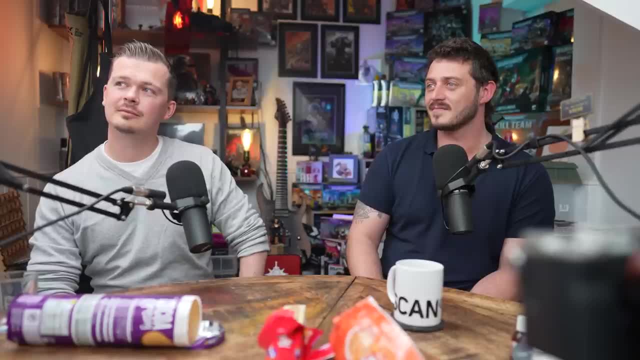 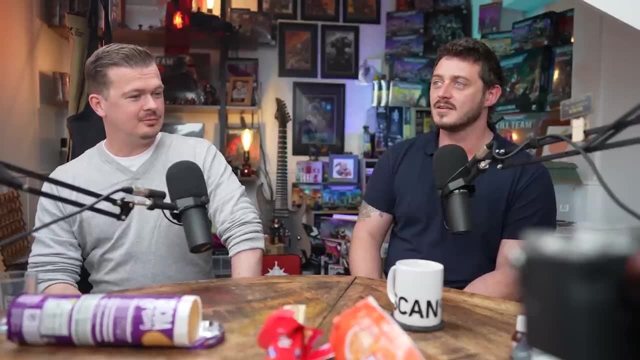 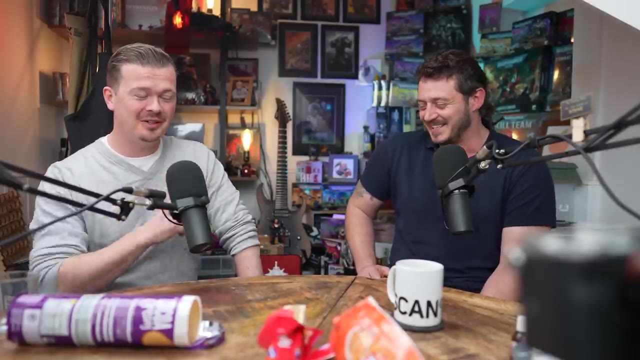 by play testing or did you take inspiration from existing games? well, we looked at a lot of existing games and thought none of them are balanced. so it doesn't matter. no, it's just it's. it's. it's worrying how accurate that is. yeah, is it? am i joking? 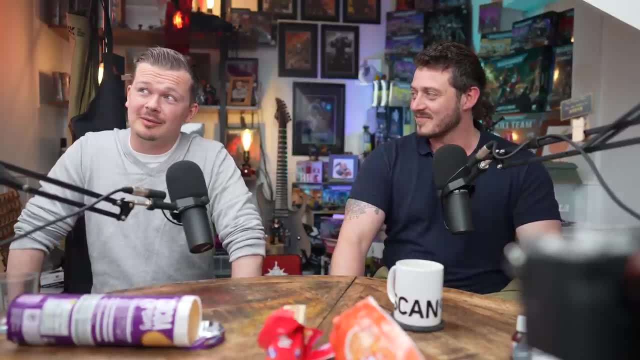 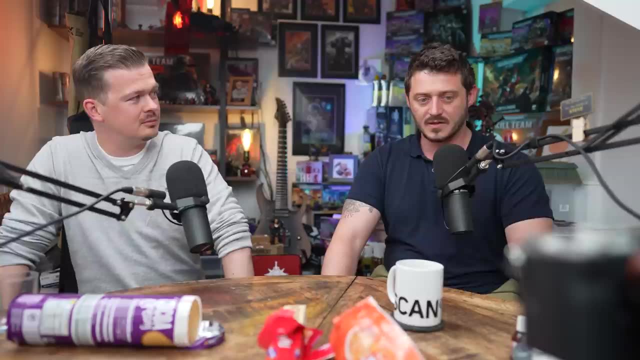 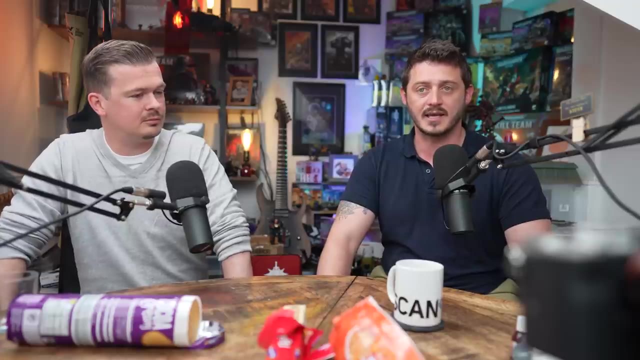 will's going to explain that, but that statement, that statement is truer than you think. yeah, yeah, it's um essentially balancing war on terror, as yeah started earlier i mentioned on the engagement grid, and we've designed a lot of the game surrounding that engagement grid, um, and we kind of followed all of the roles from there. 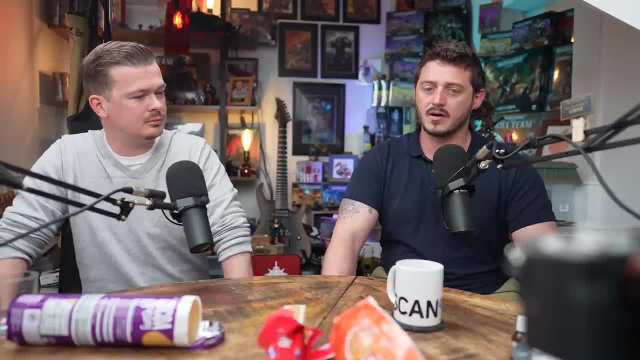 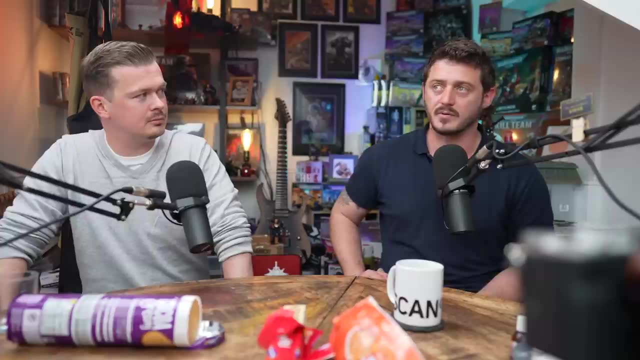 the point system for all the models. uh, we came up with a way of so like the battle value to to field them on on tabletop. uh, there was a way that we invented to equate the point system from there. um, and then by play testing, some of them have had to have tweaks and everything, something. 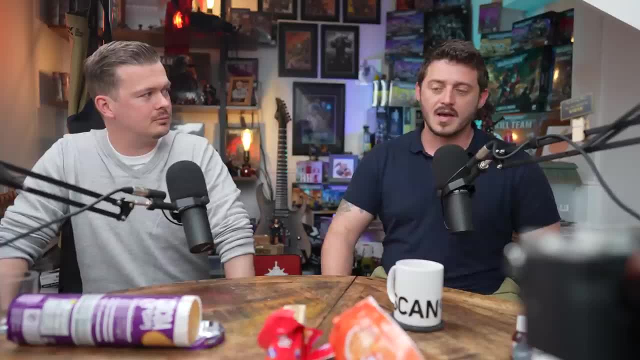 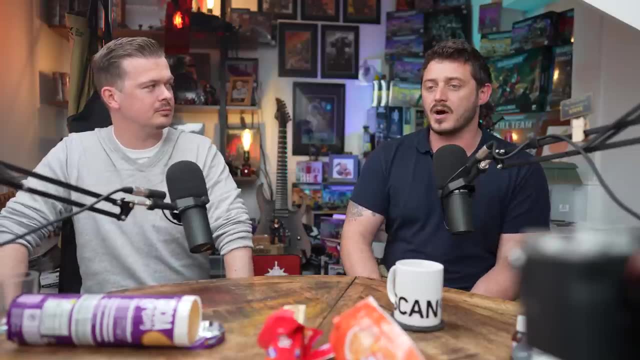 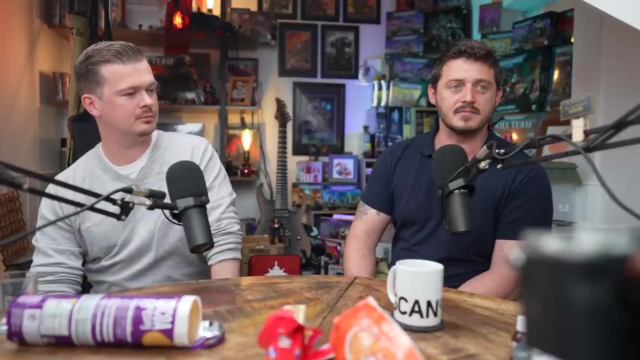 like that. one rule doesn't fit all, yeah, and so we've tweaked every bit from there. however, balancing war on terror in general, there's there's a that how i've been saying it is because i'm not the best at chess and probably alex's kids could steamroll me in chess, but that's probably one of. 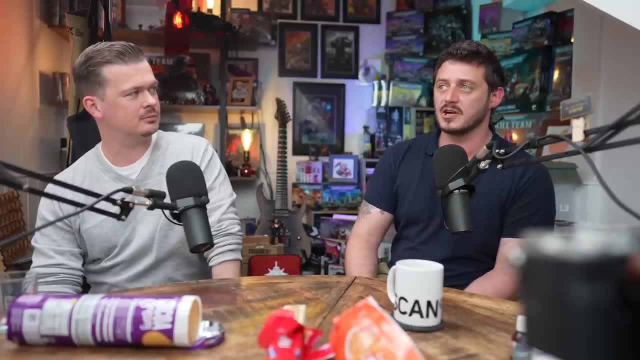 the most balanced games in the world? yeah, but it doesn't mean because i i'm absolutely terrible at it, that the game's unbalanced. yeah, yeah so because there's however many million tactics that you can move in chess. yeah, so war on terror? because we don't have a unit system. we don't really have any. 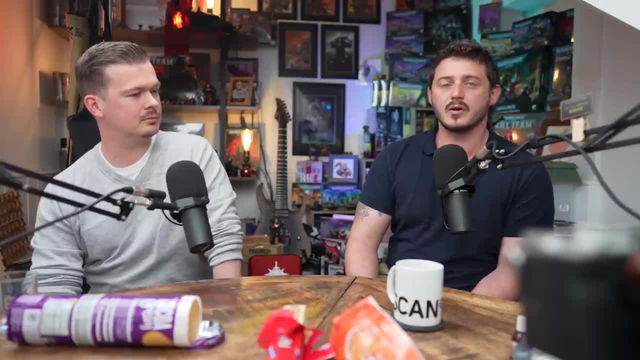 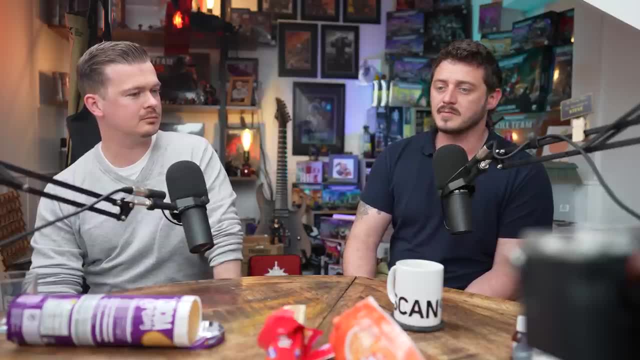 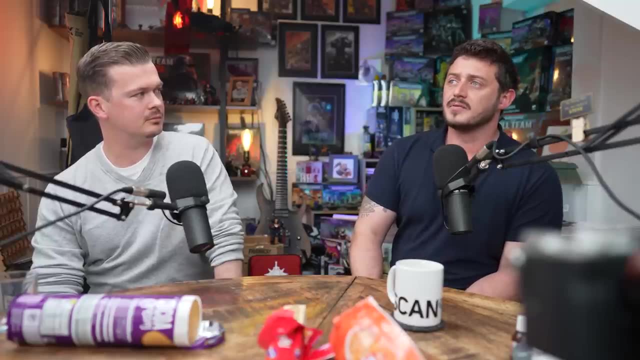 typically any way you want. so in the games that me and alex have played with the same armies- grays versus humans- there have been games where grays have just absolutely dominated the battlefield and it feels just like, oh, this is a bit unfair, do we need to change this? no, let's play it again. 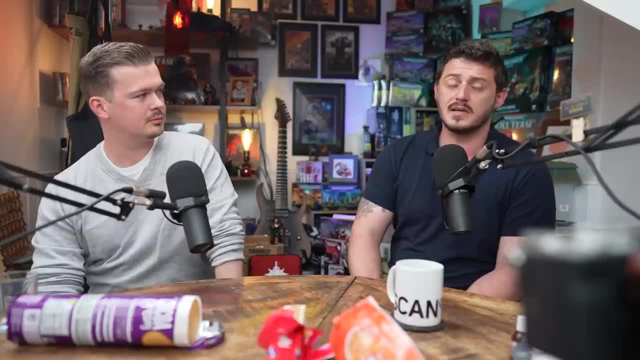 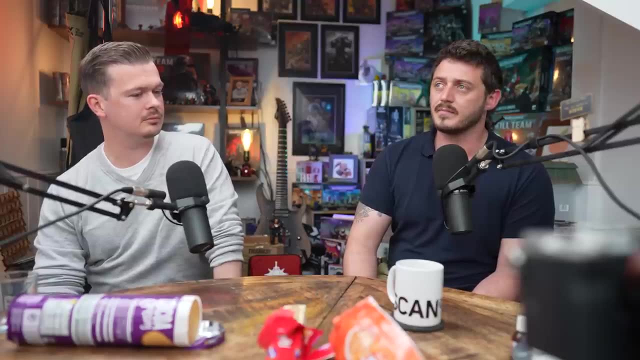 another couple of times and even the last other couple of times, it'll completely flip the script, not only because of the dice rolls, but maybe i ran larger groups, that turn, uh, that game. i ran larger attachments and it worked better to have more humans in a blob. 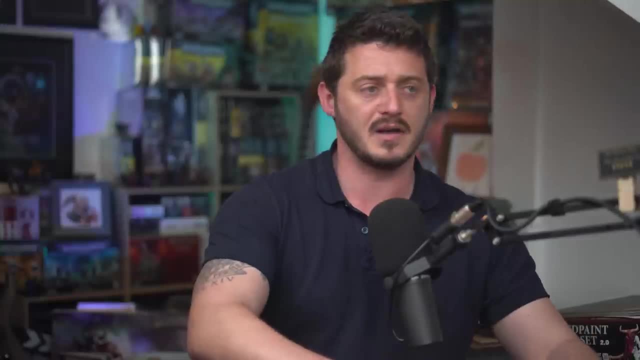 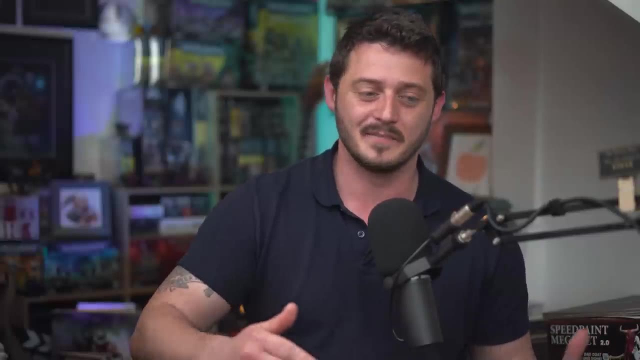 and spread them out into individual models. oh, maybe that works better for me and so, but then it'd flip again the next game because maybe he would then learn what tactic i was using. so balancing is very hard because you don't just have these. 10 models are x strong? yeah, it's like. 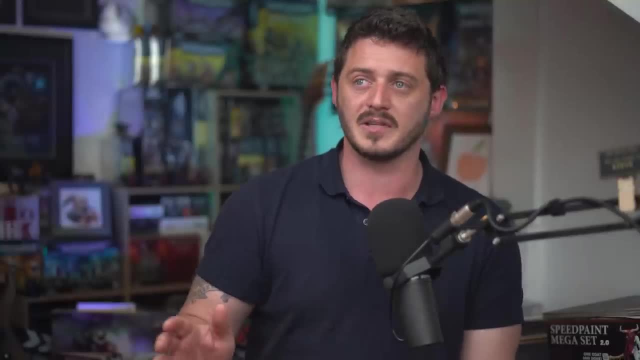 no, these 10 models could be 10 individual models and they're very weak by themselves, but then your opponent could separate all their models into georgia, individuals and great. now what do i do? because i can only kill one at a time. and i can only kill one at a time, because i can only kill one at a time, because i can only kill one at a time. 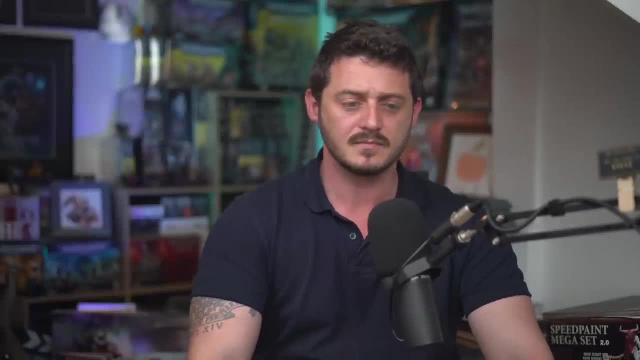 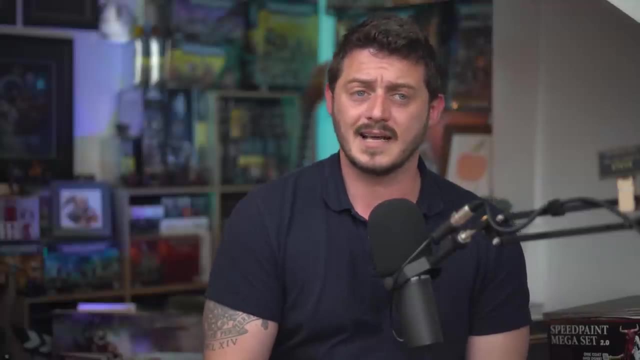 so balancing the game is very difficult. we don't have a unit roster, so there's no such thing as like: well, you must bring one hq and two troops or whatever. if you find out what your opponent's fielding- and he's bringing an all vehicle list and all tank lists- then bring completely anti-tank. 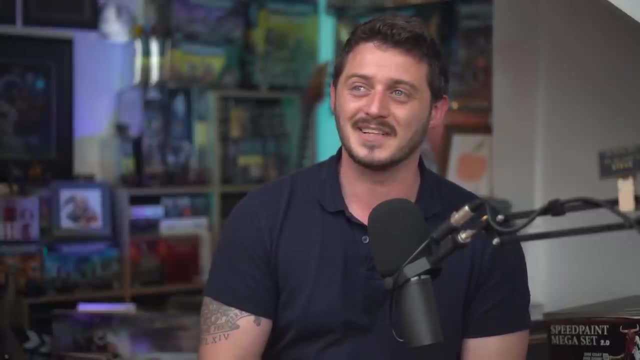 via um, infantry, uh, or models, and the game's going to seem very anti-ban like, very balanced. in one way, that's fine, because that's that's what you've done and that's what those models are designed to do, um, so you, it's up to you to design a balanced list. 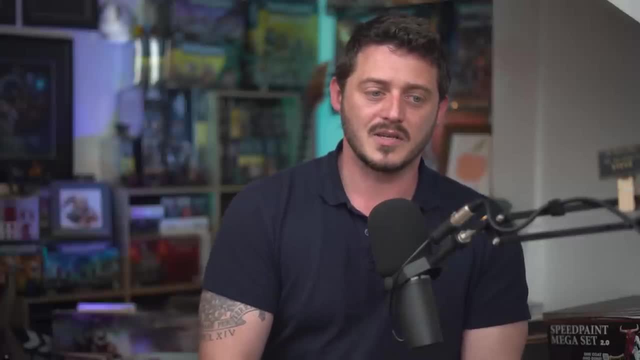 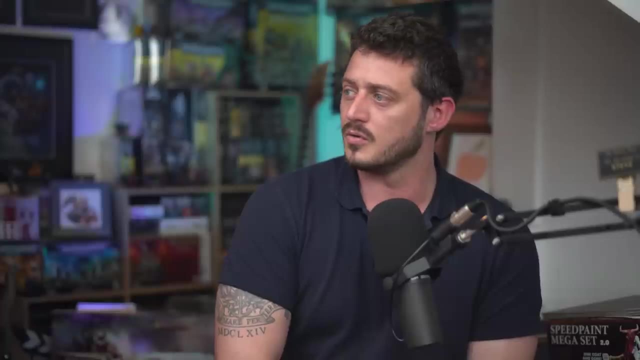 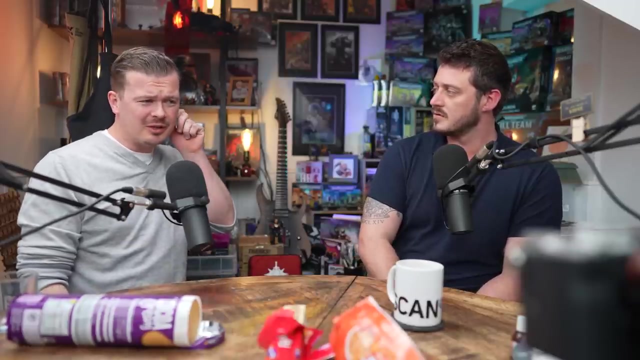 and field them and do the tactics that you want to play, which, in short, means that balancing is next to impossible. yeah, because it's all about what you do. it's balanced by the player's skill more than anything else. yeah, yeah, it's um. the game is simple. i can't remember the youtube video. 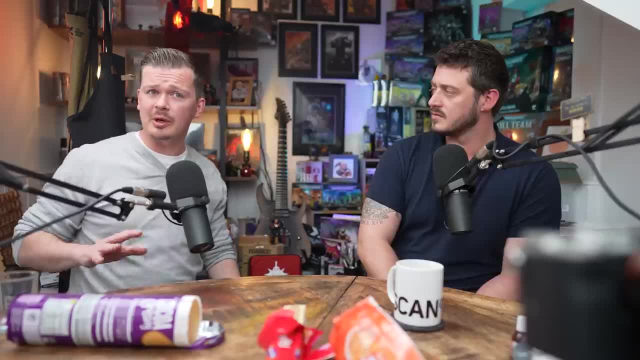 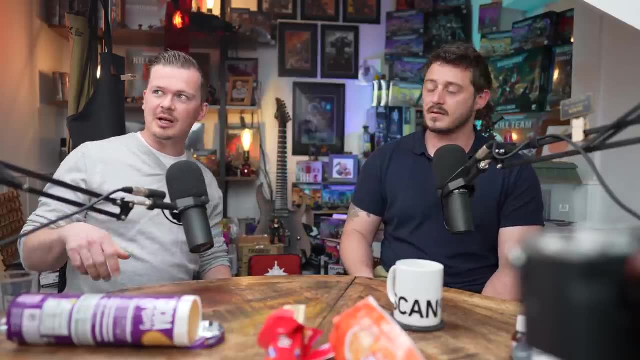 i watched it might have been a lecture at one of one of these conventions, but someone's talking about balancing games and they said them because even chess isn't balanced because someone goes first. yeah, yeah, very good point. yeah, yeah, i can't remember, but the most balanced game. 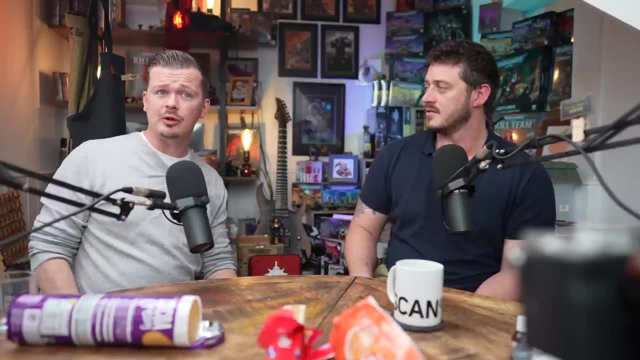 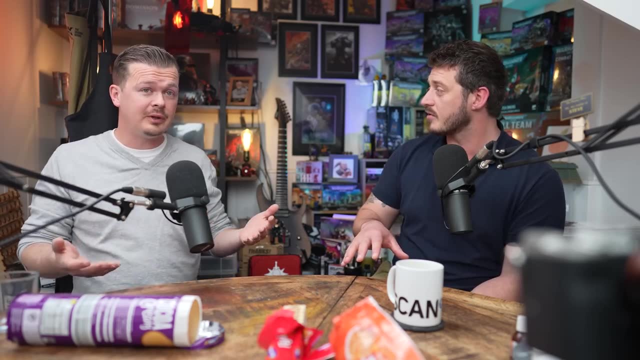 there ever is is rock paper scissors. yeah, it's also the worst, most tedious, boring game. let's not say that our game isn't balanced. we've done the best we can, but, but it is tedious and boring. no, but no because, because you can take anything you want in any. yeah, yeah, you might. 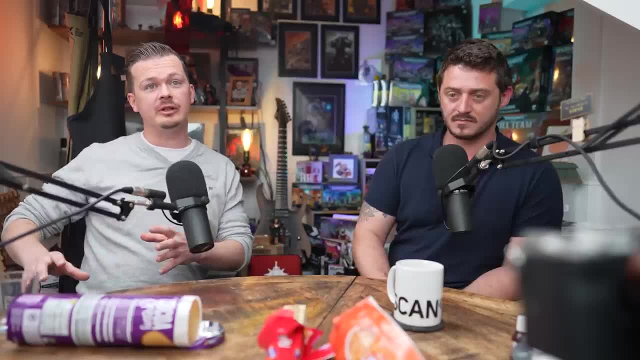 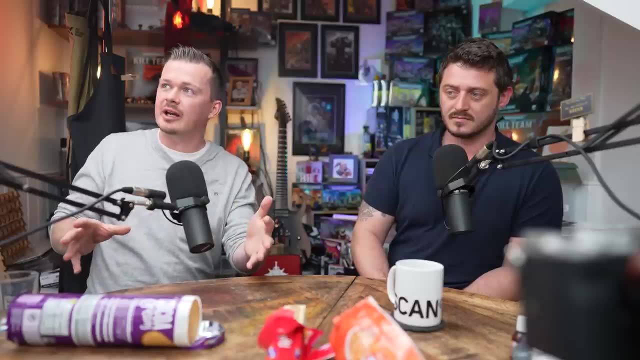 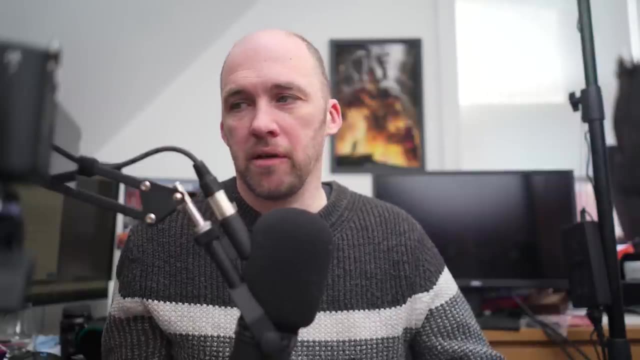 find they're knocking me off the table every single time. but if you take the right units and use the right tactics, yeah, suddenly you're not. yeah, you're balancing the game. yeah, by being better at it. yeah, another thing as well. i've had years of experience. we talked to a previous year about. 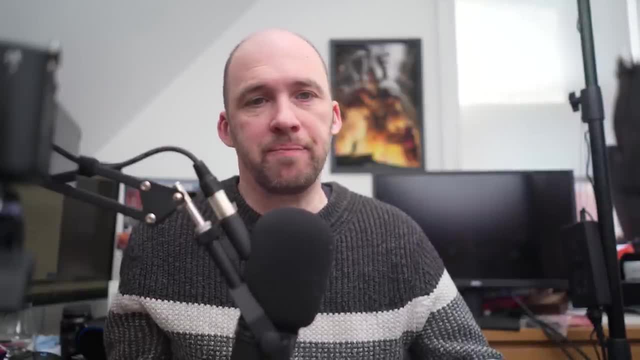 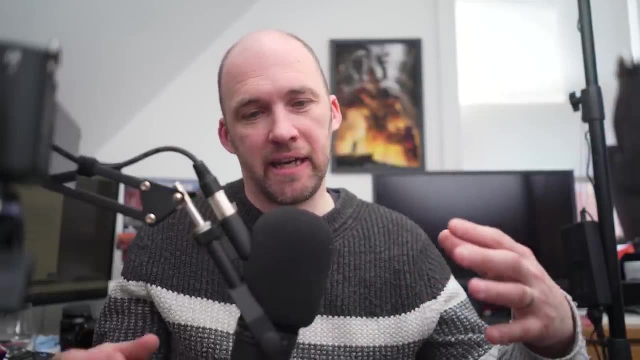 um, black powder and it's an impaler on a game and i've played games where, um, there was a guy head office- he was very tournament-based- a guy called greg um and he had he he'd like, literally when he wants to play he goes tournament mode. so i was like: join the game of black pound. it's like. 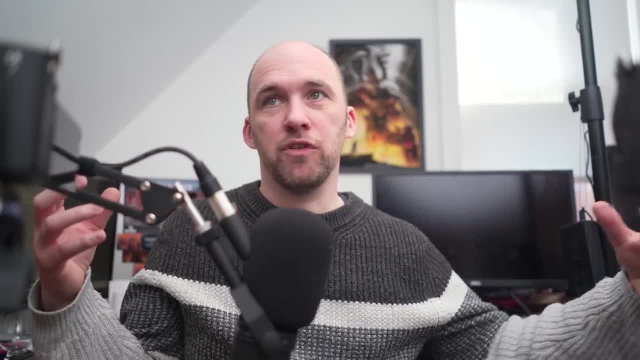 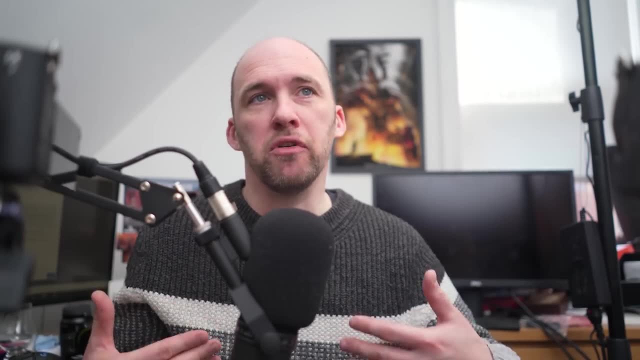 yeah, i'll have a game of black power. a couple of brigades of like infantry in one of cavalry, um, and in my infantry there's like a cannon in one of them. and he went: i've brought big battalions. if you do big battalions, so the normal size, you get small battalions which is like 12. no, not 12. 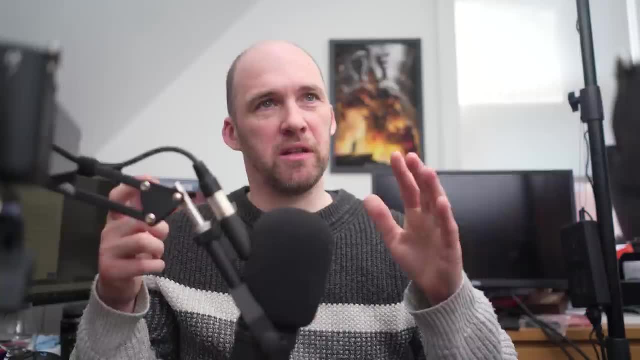 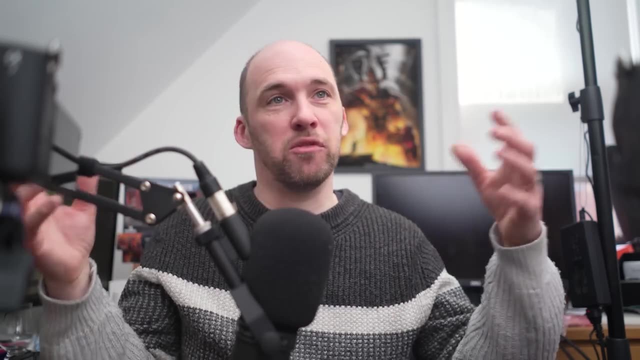 figures, like eight figures. medium size is like anything between like 18 to 36 or something like that. and then big battalions is 40 plus and he brought like loads of big battalions which gave him all these extra rules and everything was big battalions he had. i think he had two or three more. 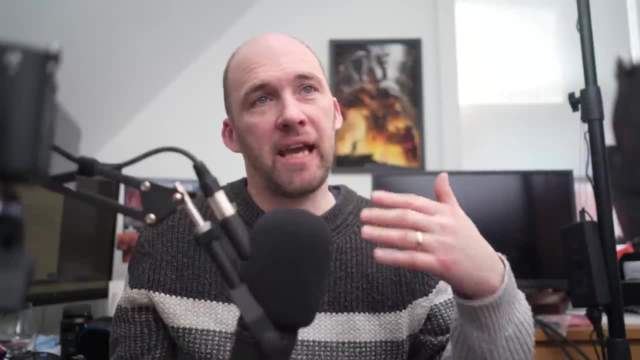 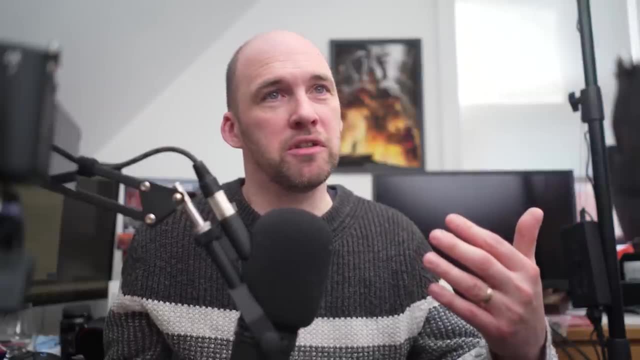 brigades more than me, so instead i'm like i'm outnumbered, but the game, just because of like the dice rolls and just the way we played, i lost, but not by that much, nice um, and it wasn't about the game balance, wasn't about he had more force, it was just about how he played. oh, so any warfare? 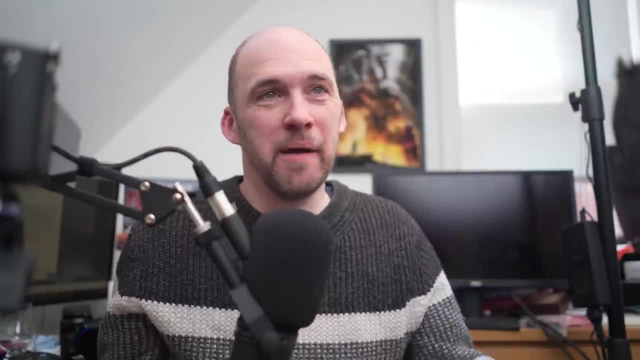 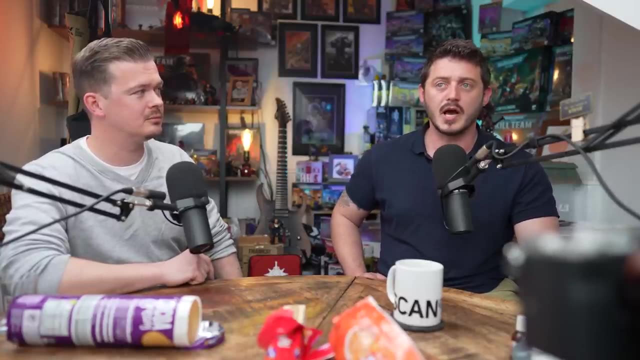 isn't balanced, right? no, there's no balance in war. no, never. um. so if the one thing you you want to make sure is it's going into real warfare, warfare, you want it as like as little balance as possible. you want to dominate over them to make sure you are safe. yeah, yeah, so actually. 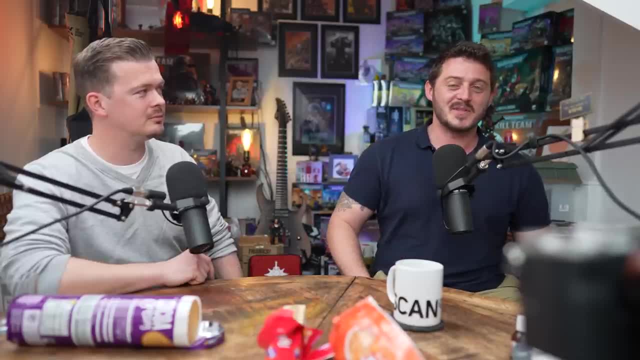 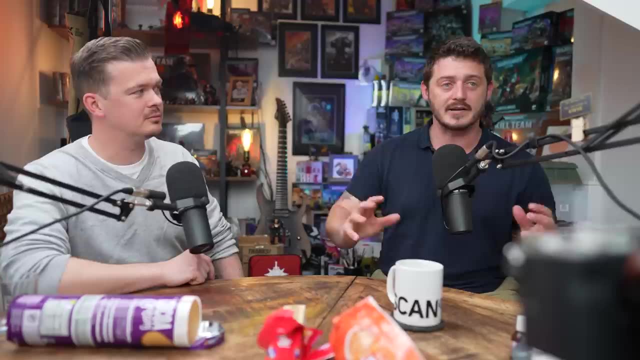 don't? you don't want to balance warfare? there's no fairness in war. yeah, yeah, um, speaking on uh coming back and seeming like you're starting on a losing edge. we have a weather system, or planetary weather system in the game uh, where you shuffle a deck, draw a card. 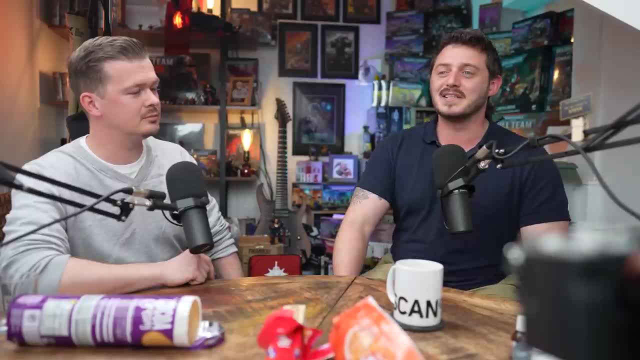 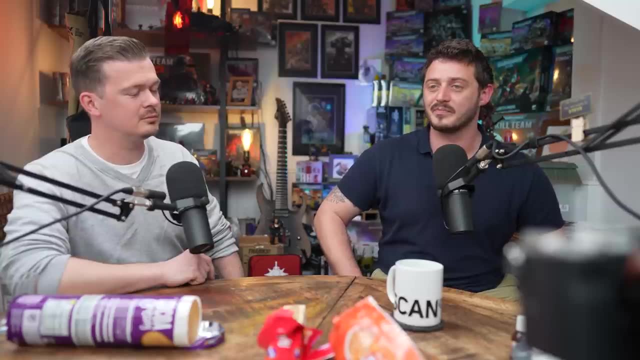 and random effects can happen. um, while playtesting one of the games, um- and my buddy actually mentions like: oh, do you want to? do you want to start again, because this is quite unfortunate- i drawed um sort of heavy lightning and, uh, you roll a scatter, die, and then you roll two dd's. 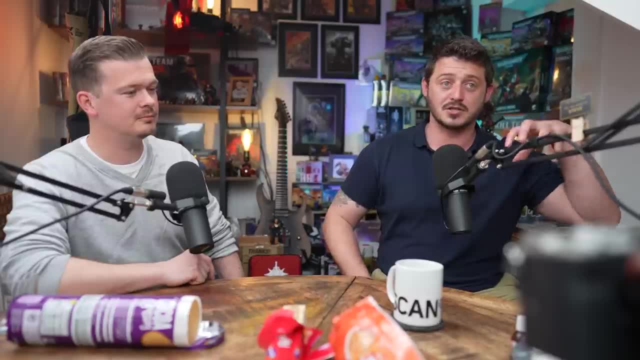 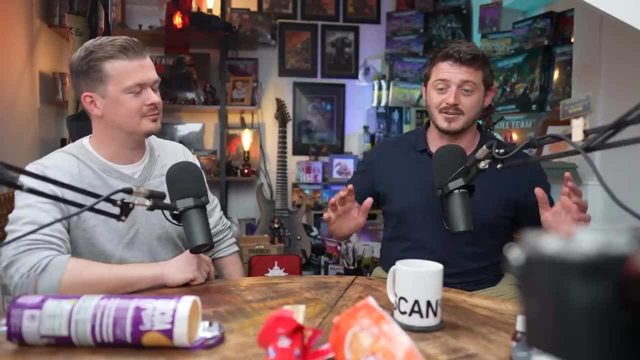 and find out where that lands on the board. yeah, and it just so happened to land straight over one of my attachments and i had to roll saving throws and i lost six guys straight off the bat. nobody had even moved, yeah, and i was like, well, that's great, i lost the game. but i'll tell you what i i. 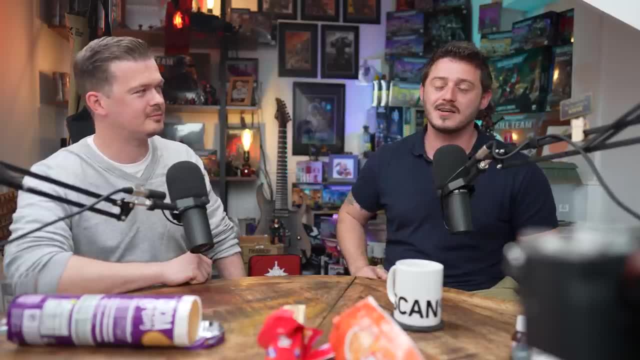 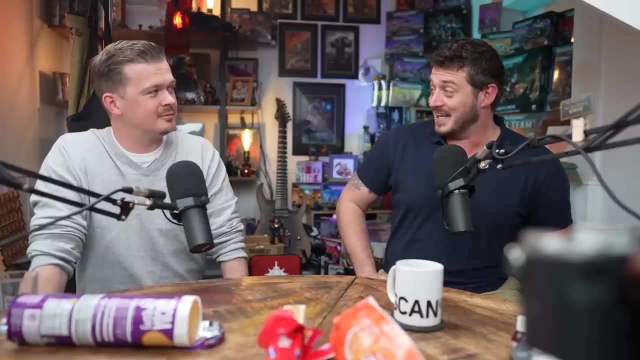 pulled it back and he's like, yeah, do you want to? do you want to start again? i was like, no, dems are the rules and that's the game, and you can't help lightning. and yeah, yeah, that's great, it was a good game. it was a good game. yeah, it's nice having that random effect as well. that could just like. 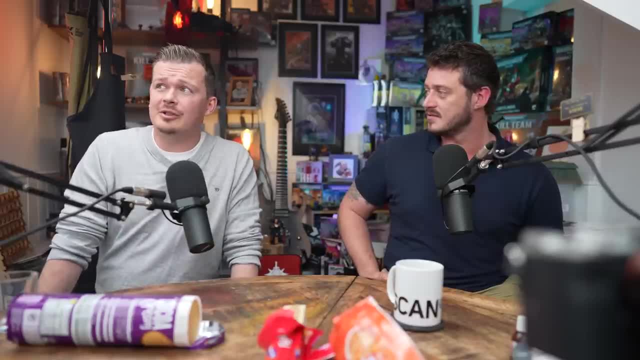 completely change it. that's great, it was a good game. it was a good game. it was a good game. it was- and that's weather? yeah, because at the end of the day as well, it's still it's a game. yeah, and it should be fun and things like that happening are fun. yeah, i mean, obviously some people are not. 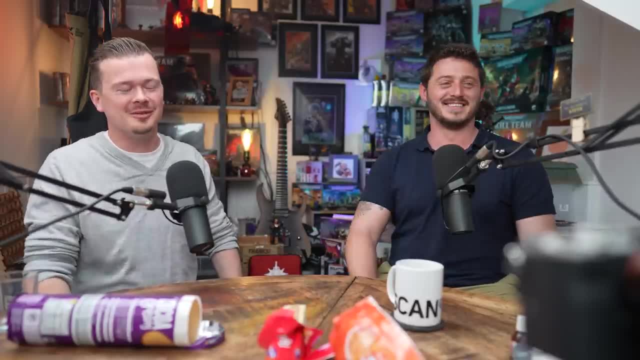 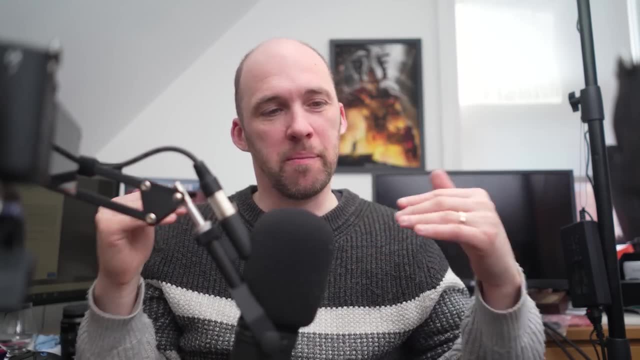 going to find that. yeah, but if they're going his tournament mode, then that's yeah, oh yeah. sorry i digress, but i had a game of war cry. i'm a big fan of war cry, simple skirmish game. yeah, you can like try. and there's a guy i work with called nick and nick ermston and he wants to do stormcast. 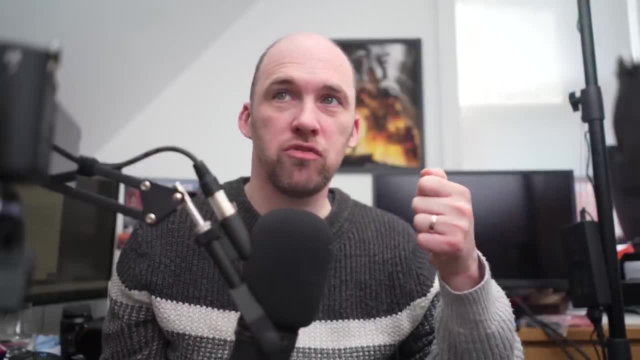 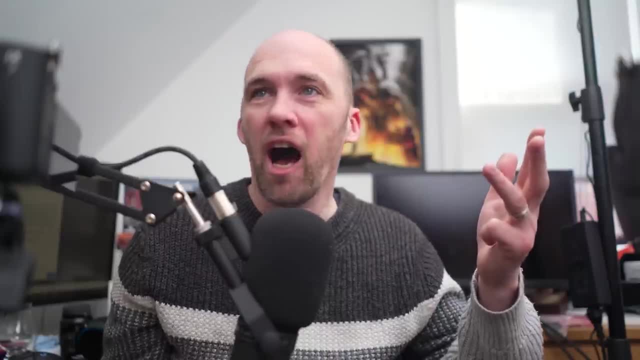 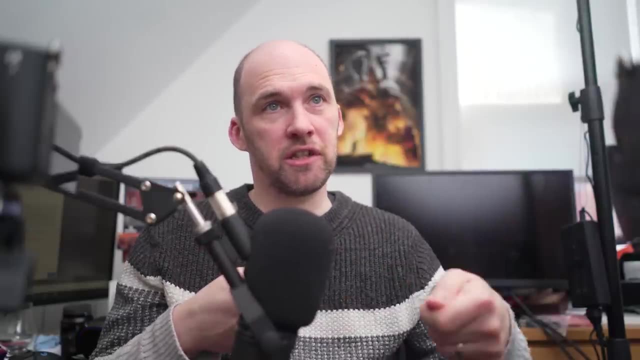 and they move faster than normal stormcast. i was like okay, so he's like i think i've broken the game. he was like cool, the great thing with war cry is you get like a deployment card, you get like a victory condition card, you get um and something called a twist. so you that this is. 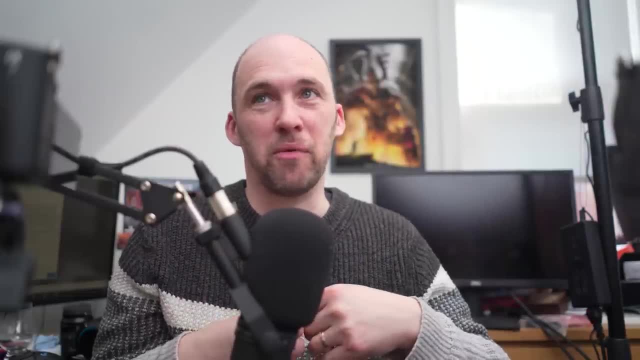 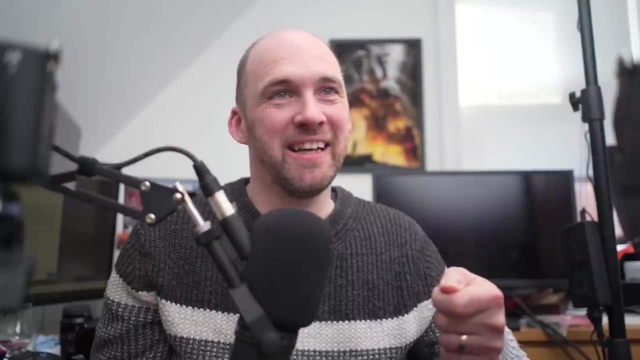 how you work out your scenario, and he was just like, yeah, i've got this, and i was like i'm gonna get cream cracker here, but give it a go instantly. the twist was you can't shoot anything more than like three inches away, so his ability of having all these bows was instantly lost. that's great. 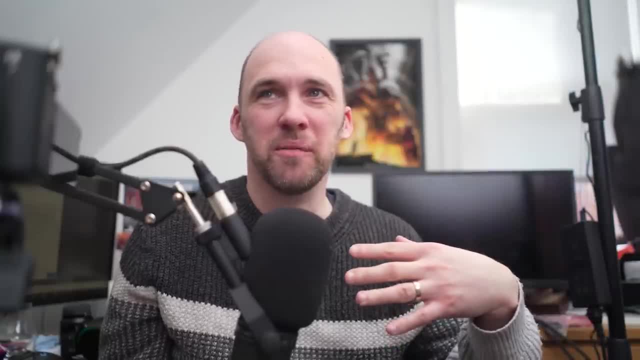 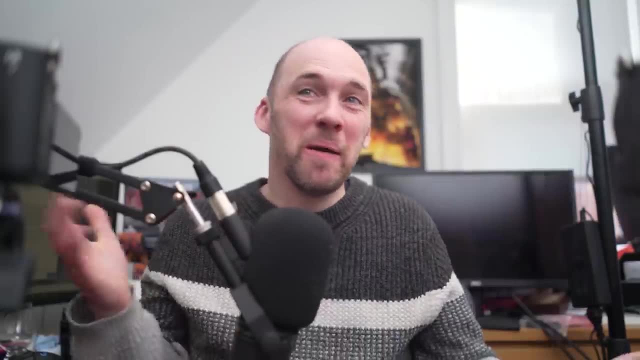 and yeah, he had like five guys at about 10 or 12, something like that, so i was able to get these objectives and stuff, like. so he's there just like great, oh, this game's rubbish, yeah. yeah, it's not balanced at all, but that that's. i mean, that that's the thing is like war cry is really good at like. 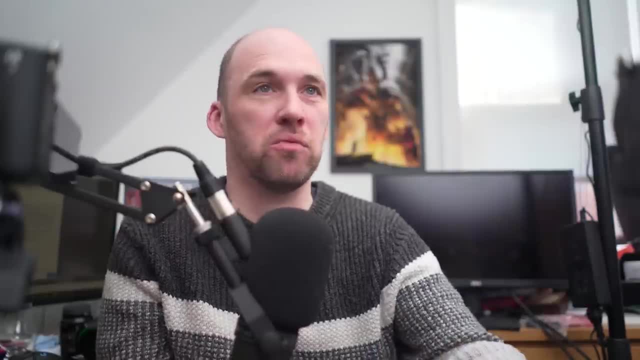 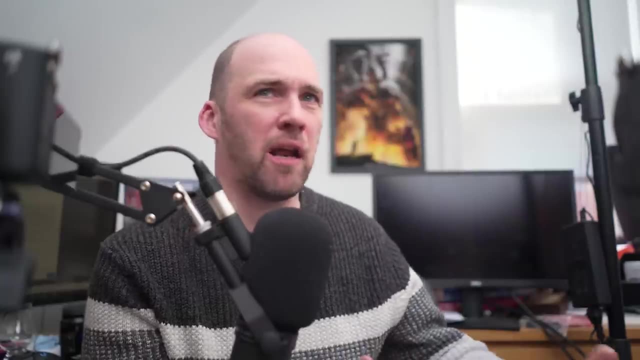 that's cool, regardless of whether you think you're gonna lose it. the twist will like, maybe throw it out a bit or make it really one-sided. you'll be like, oh, i'm definitely gonna lose this, but you, it's so quick pace you could play like three games in in a couple of hours, yeah. but 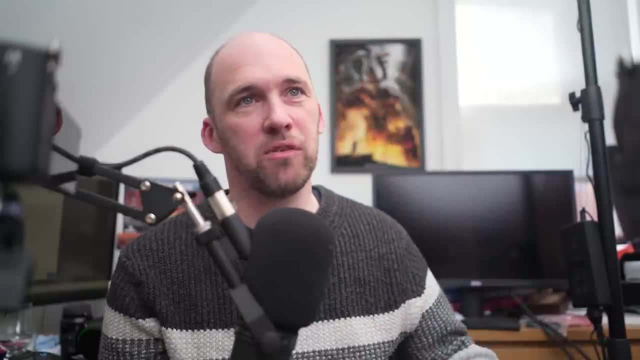 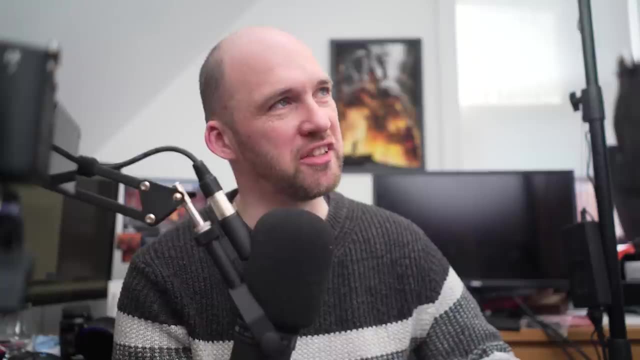 yeah, having like a car, like a weathering system or something like that- you can't do anything like that- that throws it in there, it will. i think it's such a really good way of doing it. yeah, so smart move, fantastic. sorry, i waffled on no sidetracked. you could say yeah, absolutely. 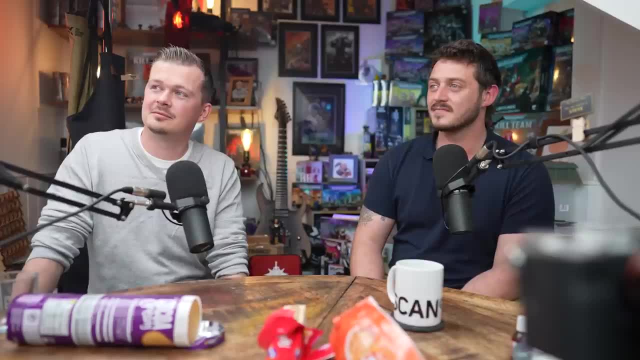 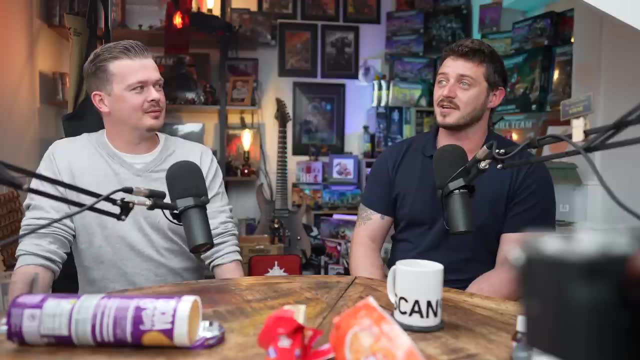 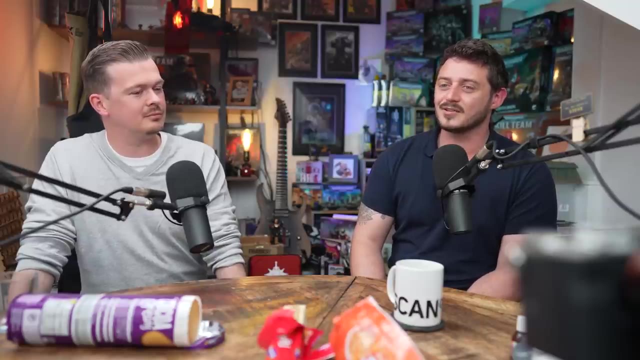 um, do you have any stretch goals planned for your kickstarter? nope, no, nope. we both don't really like stretch goals. yeah, um, because it means that if, if you don't meet them, then you're getting a worse game. yeah, it's like great. so i'm i'm expecting to get this really cool game with all these. 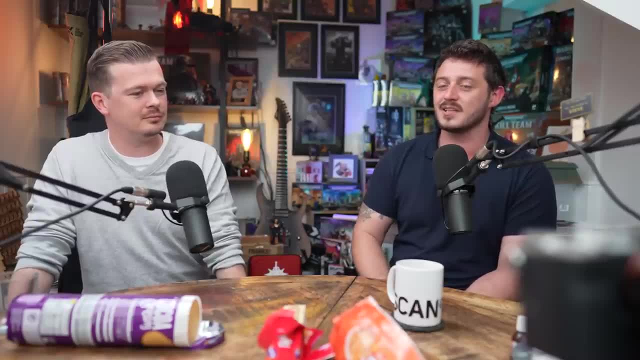 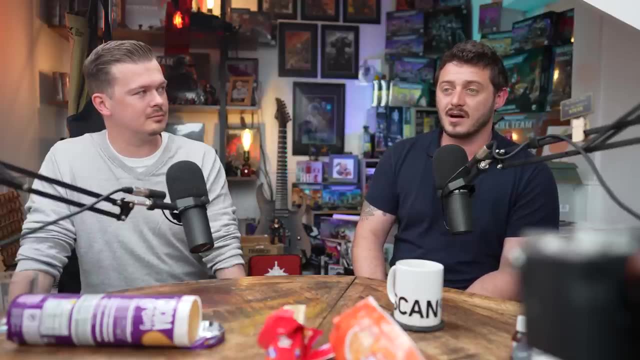 really cool moving parts and these nice little metal tokens and whatever it is like: yeah, oh, they're a hundred dollars, 100 pounds off 50, yeah, i don't know. whatever it is off. and now you're getting like card. yeah, it's like, oh, brilliant, no, no, we're. we're no stretch goals. what you see on. 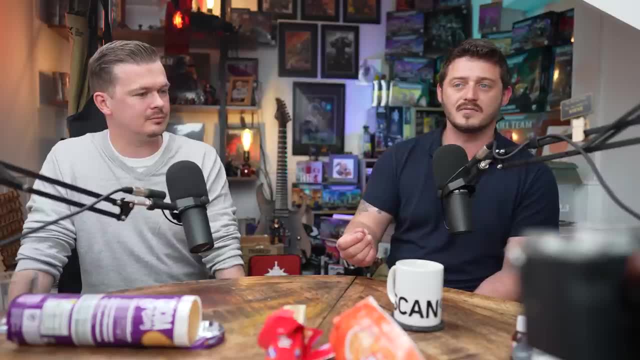 the kickstarter. yeah, is from the material the cards are made from. um the detail of the models is absolutely the best that we can give you. yeah, is is the best that we can give you. i can confirm that box set, when you handed it to us, is like the nicest. 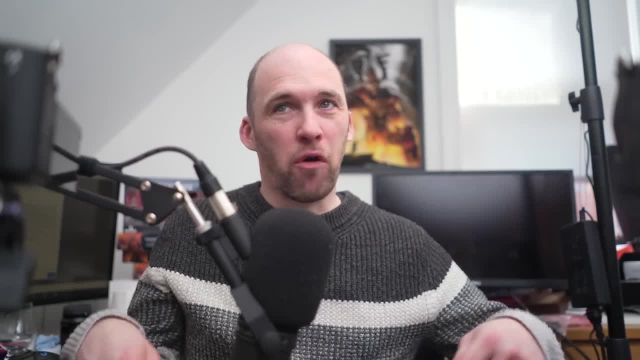 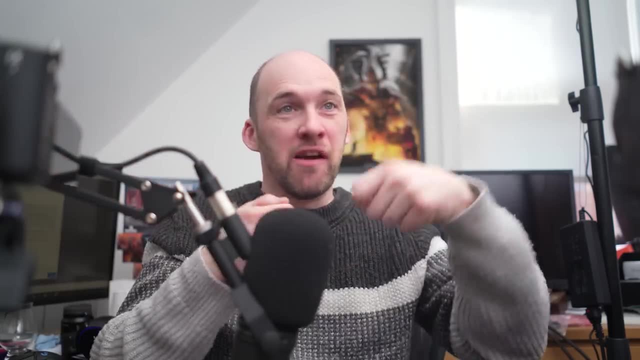 box that i've ever like got from someone, like, because you like fold it open, you've got all these. like, you got your, your. what would you refer to it? like, yeah, the grid, the grid, oh yeah, you lift up the next bit. and there's like the soldier you lift up. and there's like the cards. 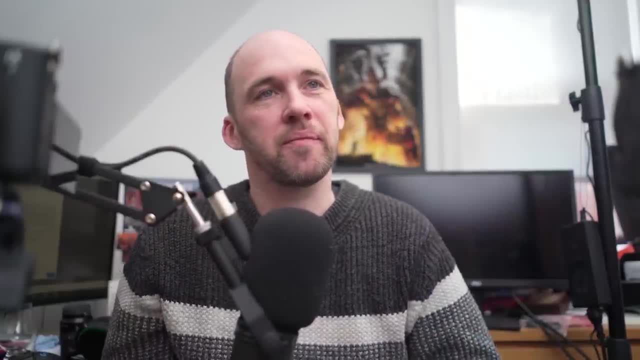 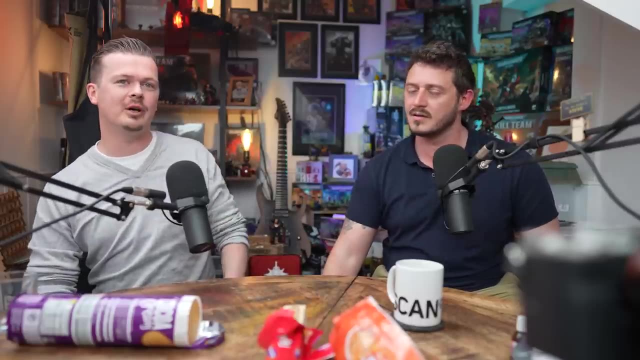 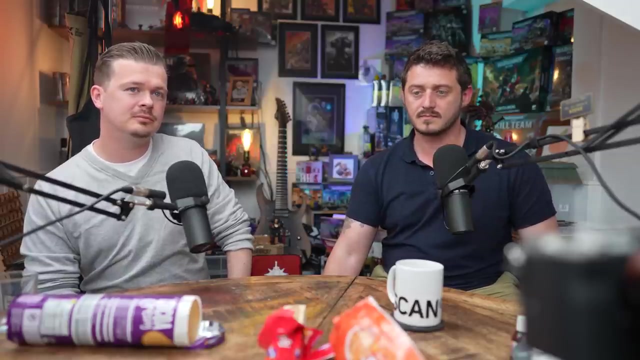 and stuff like that. oh my god, and like the tokens and things we wanted- to lack of a better word, we wanted it to seem classy. it was. it's very classy grown up. grown up, yeah, the way of yeah, yeah, no, it's really well packaged, really nicely done and yeah, testament to you guys putting a lot of effort and timing. so 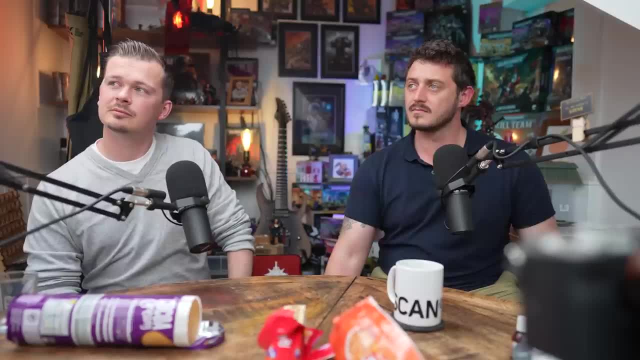 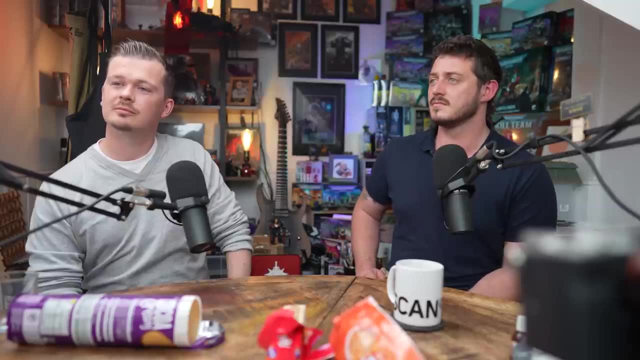 it's, it's. i would liken that to like i. i always lose sunglasses because i usually wear glasses and if i wear sunglasses i have to put my contacts in this, that and the other. i always lose them, i put them down, i forget about them, and i was, like you know, i'm 33 now and i invested in my first. 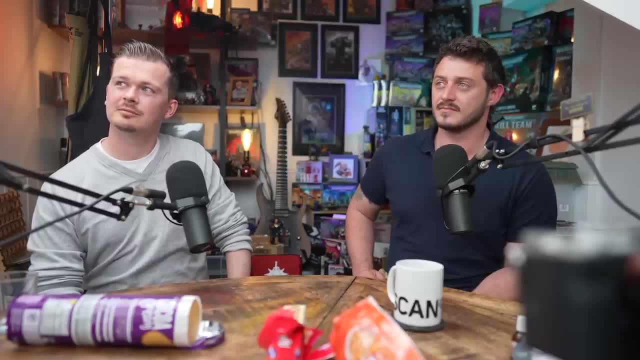 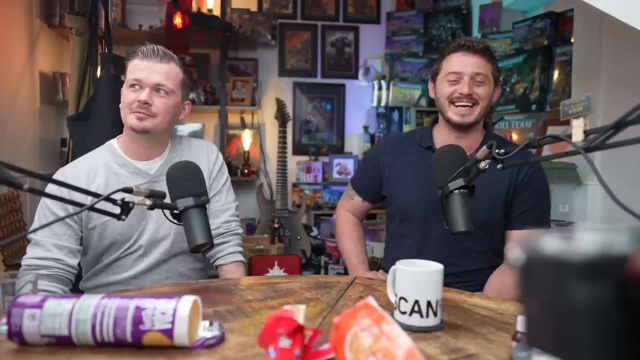 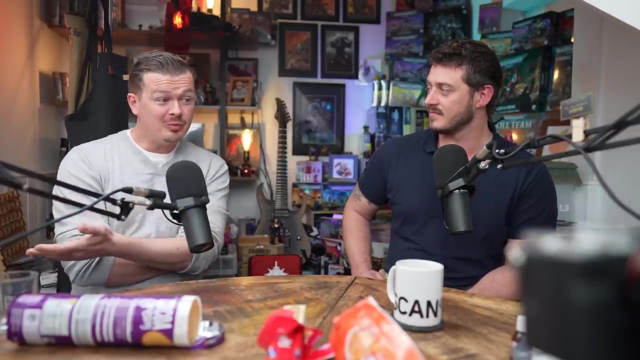 pair of like nice sunglasses and opening them was like an experience, like the packaging, and i was like, and that's like like, how did that box to yours at chillcon? it was just like i can't even make the noise because my throat is destroyed, almost ethereal. you know, dry ice should come out. yeah, yeah, i was another. we probably sort of 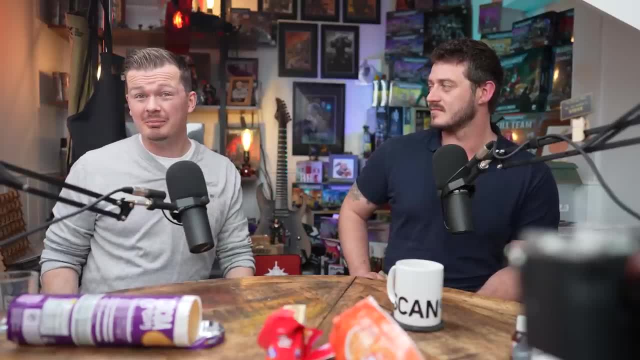 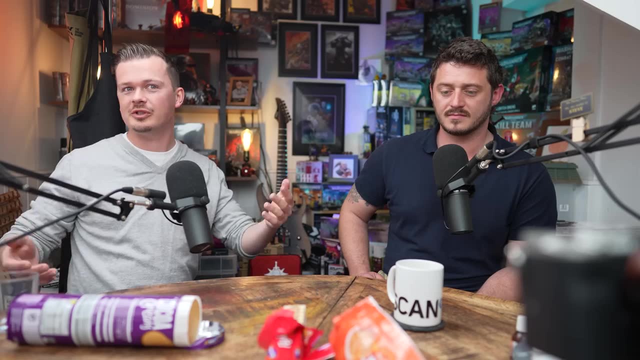 i think about it now. at the time we probably it was there subconsciously. it's people like unboxing stuff, like oh yeah, oh, you've only got to watch these reviews, these videos on on youtube. yeah, people just unboxing randoms and obviously the nicer. 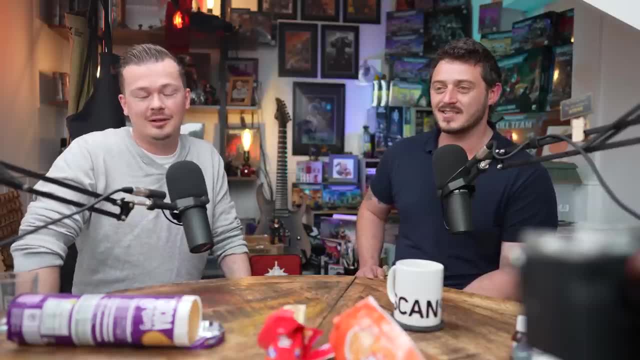 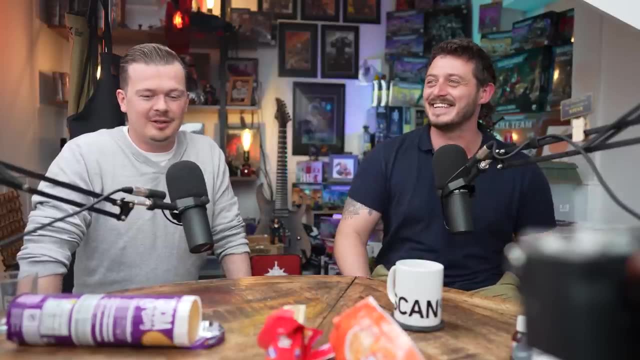 it is, and then everything's revealed after layer. Yeah, it's that, it's that internal monkey brain. It's just like: Oh, what's in box? Yeah, it's just like: Yeah, God, do it, Just open the box. So we wanted. 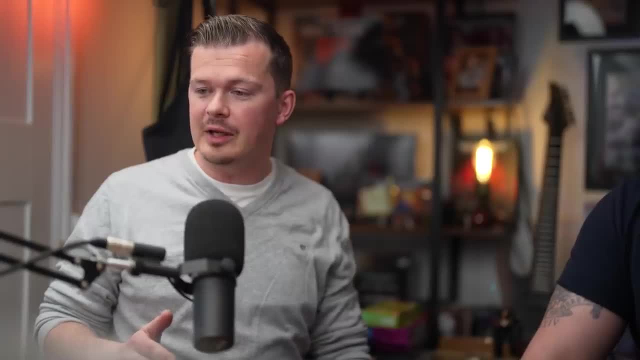 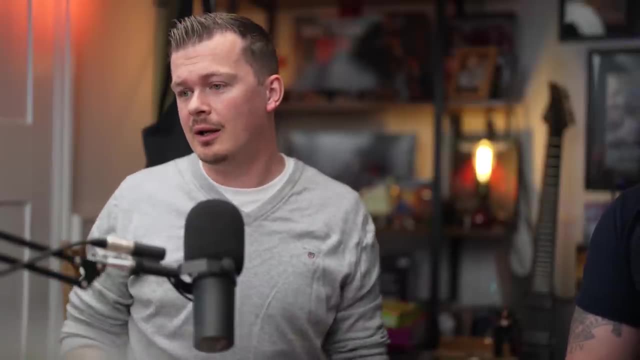 things to be like as like. so you, it's difficult anyway, because a lot of things you see on on Kickstarter tend to be more board games like completely self contained. Yeah. yeah, Be hiding quality behind stretch goals. Yeah, people have no real controller, So you might. 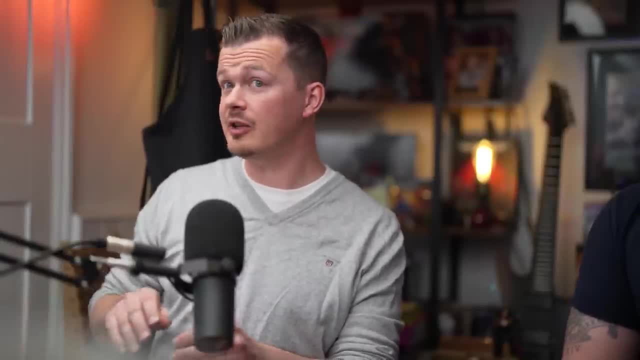 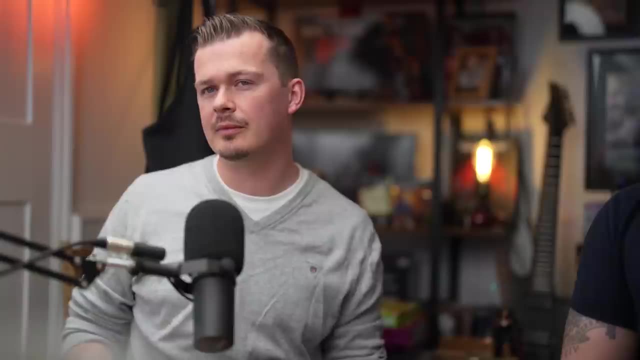 back thinking, Oh, if it reaches the stretcher- because I like those models, there's nothing further you can do to help them. Yeah, they get missed. And then, yeah, it can only really lead to disappointment. Yeah, that's a really smart way of looking at it, Because I never 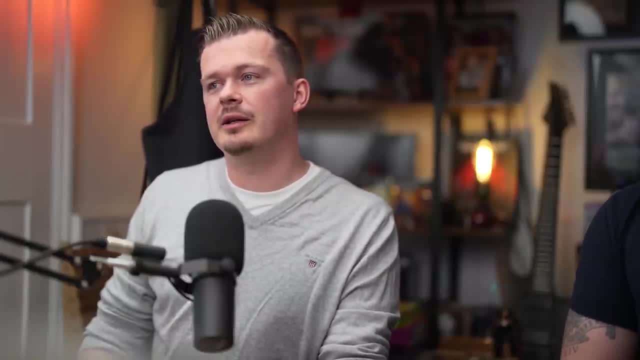 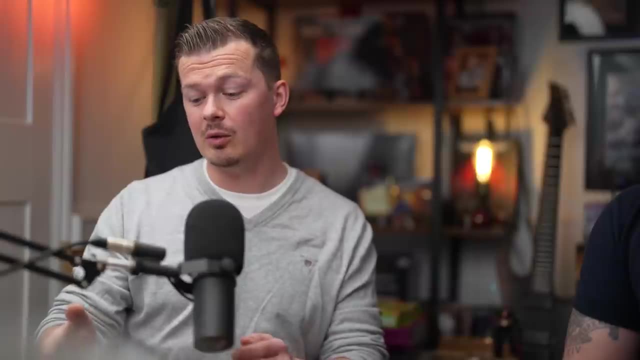 really thought about that. I was just like, yeah, you just get to the next tier If you, if you look, if it seems it's a very good. yeah, because hopefully, when the Kickstarter is like, if you go on there, the page is quite well laid out and clear, Because what we do 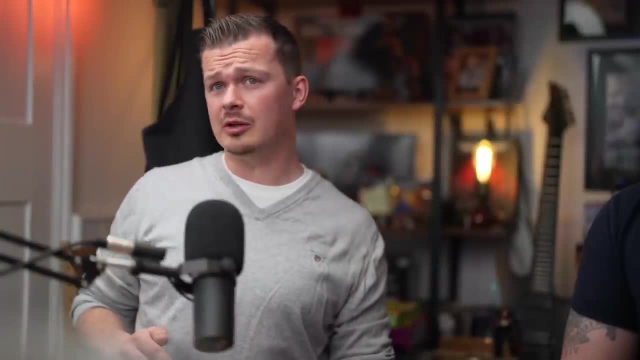 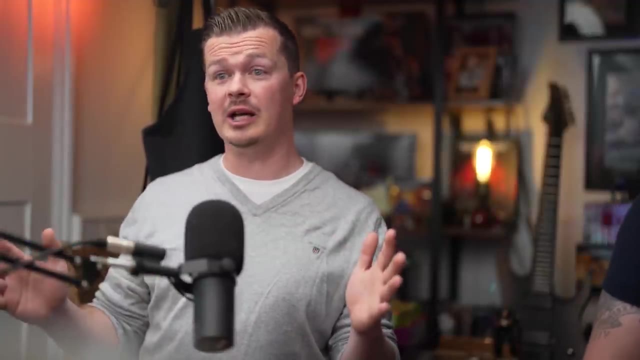 find I'm not knocking anyone, but what you do find is some of them are so long and complicated. You've got all these stretch going on, all these add ons. you think it seems like they're just trying to bombard you. So you, I don't know. I don't know what I'm getting. It looks 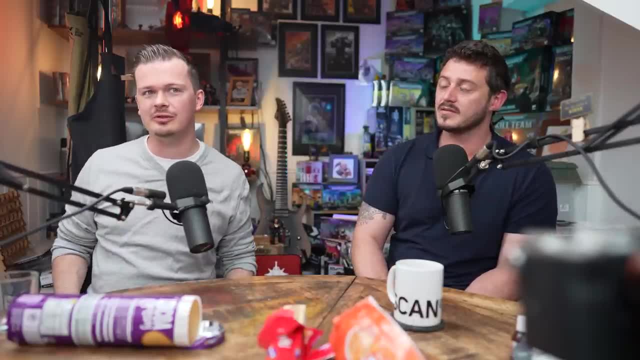 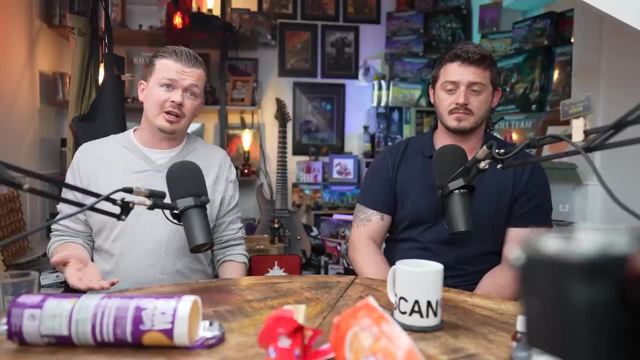 like I'm gonna get a lot. Yeah, yeah, Yeah And I think the stretch goals And also, yes, the starter boxes. self content: you can buy that, play the game and never have to get anything else. Yeah, But obviously because it's scalable. There are models that you can add on. Yeah, 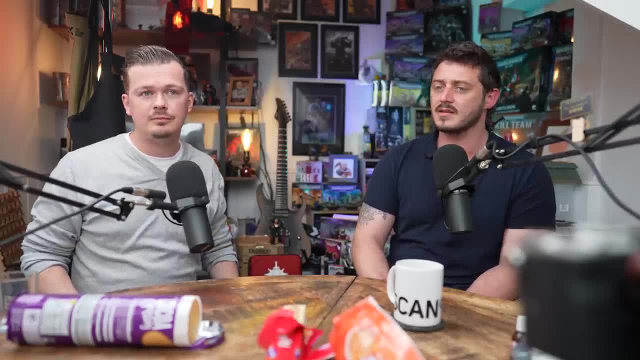 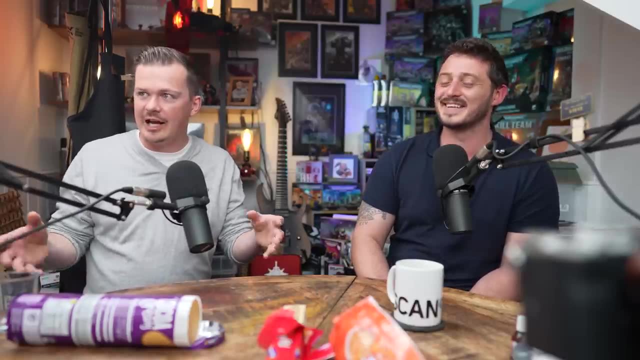 we've got add ons, Absolutely Yeah, But again, the add ons are what you're gonna get. Yeah, yeah, yeah. Everything we want to give you, We are giving you at the quality that we want to give it to you. Yeah, yeah, yeah, So right. 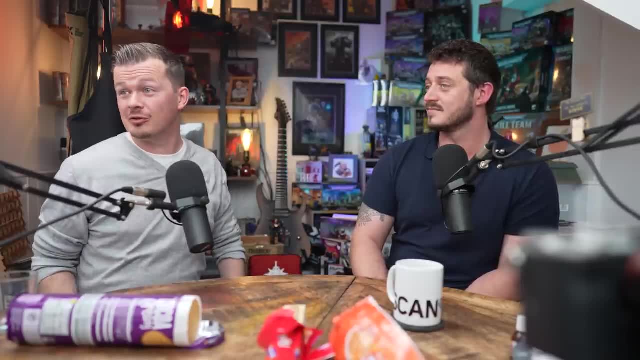 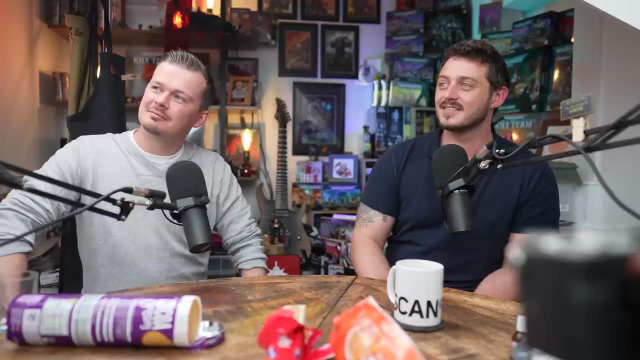 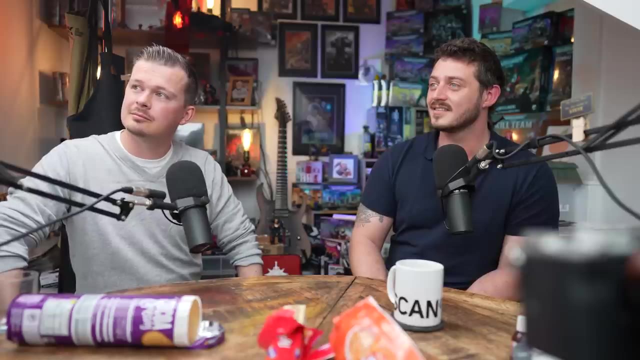 from the right from the get go. So also, yeah long, Yeah Long story short. no More of a slightly philosophical question from from Sam here. Are you, first and foremost, a game design company who use miniatures or a miniature company who designs games to? 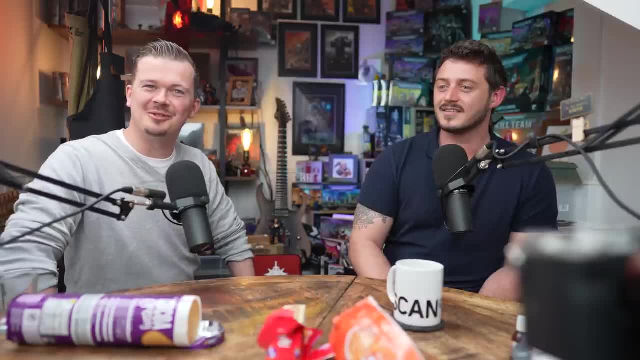 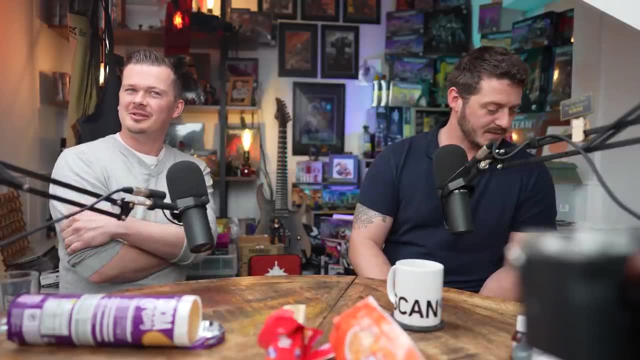 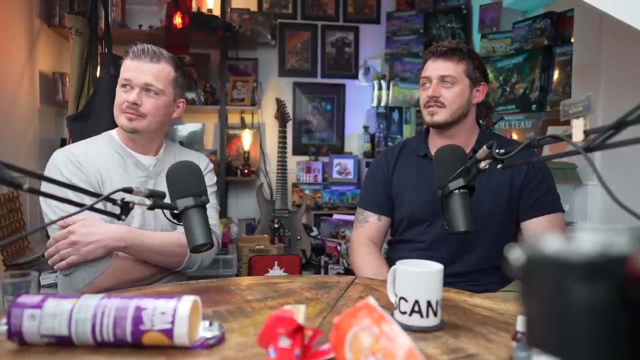 use miniatures. Oh, that's a callback to a conversation you had with a different person on hills. now, I think Is it? Yeah, because you Yeah? well, I think it was. you guys described games workshop. Yes, Yes, That was model. Yeah, Yeah, Yeah, Because they in their business statement they are. 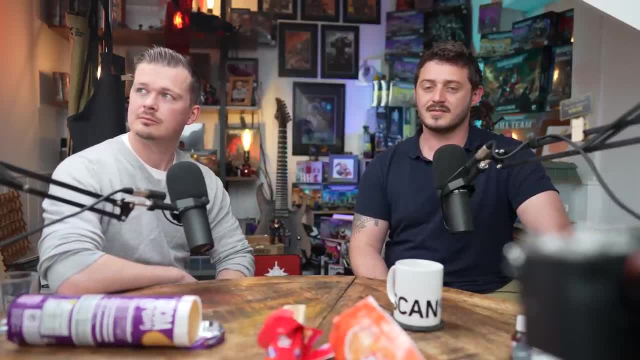 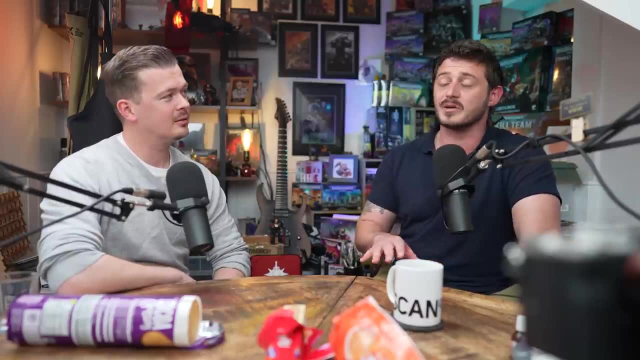 a miniature company. Yeah, And the games are a vessel to sell miniatures. Yeah, we were our company- Excuse my belly, by the way, if you can hear it- Our company's AWA game design. So war on terror isn't the company, war on terror is the game. Yeah, So AWA game. 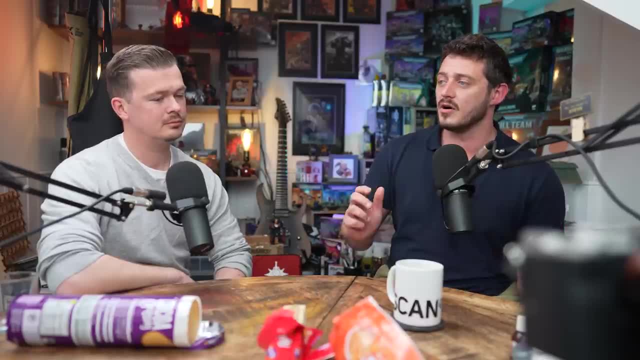 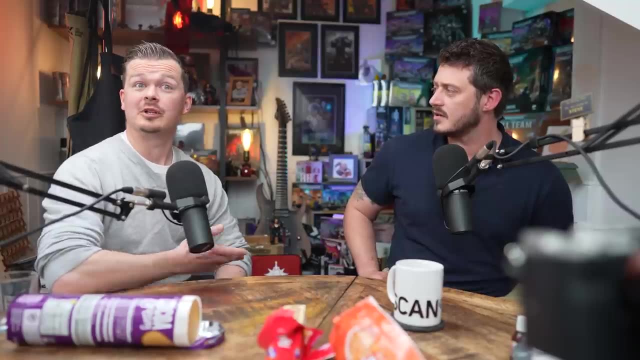 design. Yeah, Yeah, So we're designing games. Yeah, we've got three, four more games, Ideas There's. there's a few planned. Yeah, We're going to try to knock this one out first. But yes, we can roll. we've got a fantasy ball game. 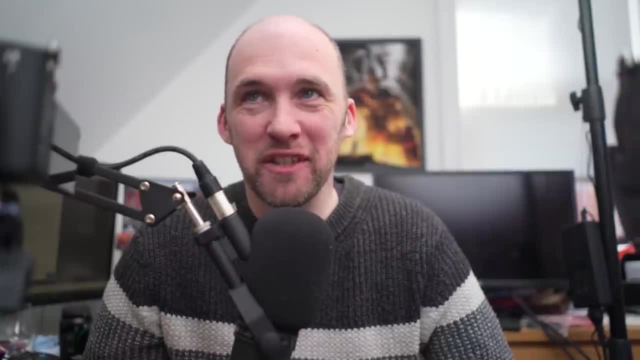 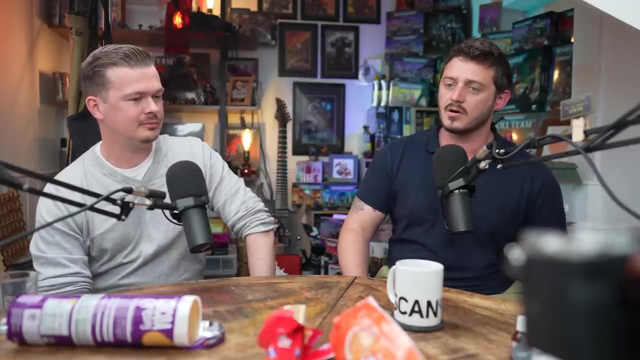 I was literally gonna ask you, like, as you're gonna keep deciphering and move to fantasy, So we've already got my interest. I want to fancy style tabletop war game as well in mind. we've got like a Total War risk style gain that we want to bring out. 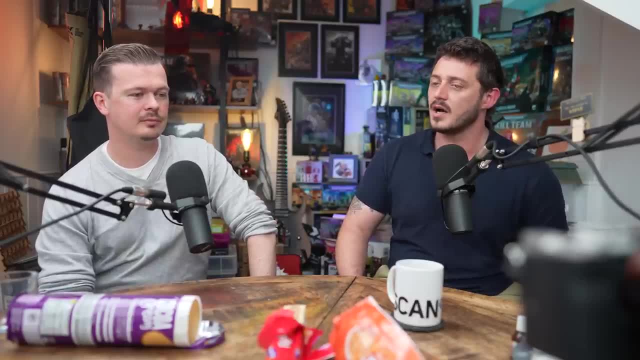 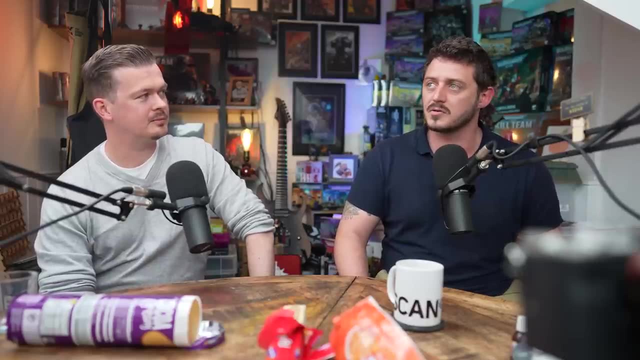 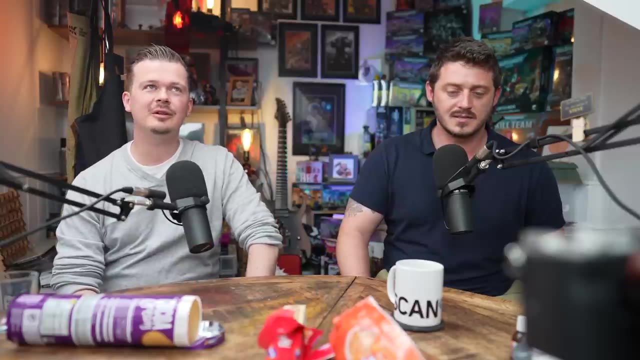 and so we're definitely a game company. uh, we, we enjoy games. yeah, um, but that doesn't- and that doesn't mean we're gonna like, forget about the models. yeah, so i would say we're a game company that designs. yeah, i think they have to, they have to work in tandem. yeah, yes, i think you'd be hard. 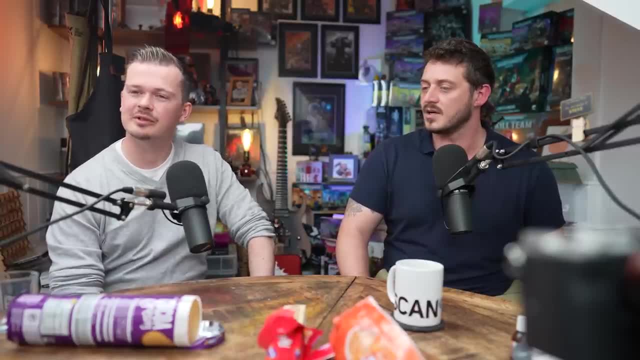 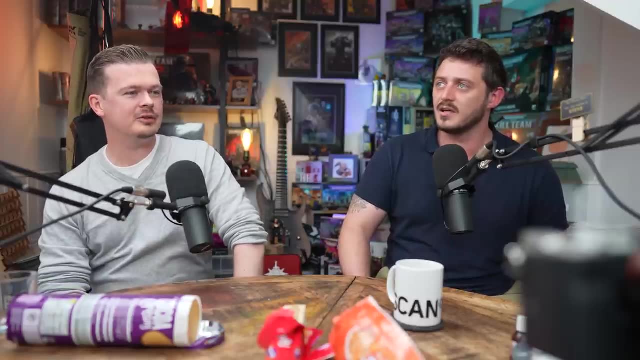 push to say it's one or the other, yeah, yeah, i'd rather people enjoy playing the game with worse models than people who have these absolutely stunning models with a rubbish game. rubbish game. yeah, the amount of times we got together to work on the game and ended up just playing it because. 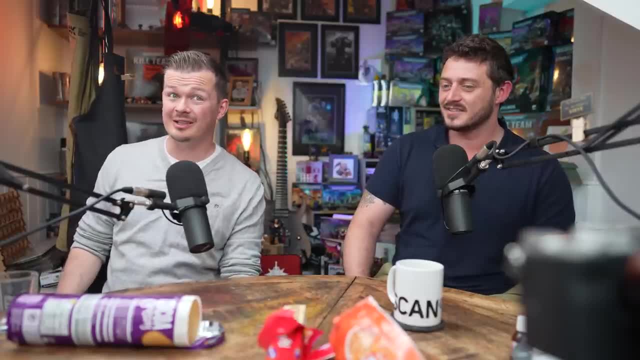 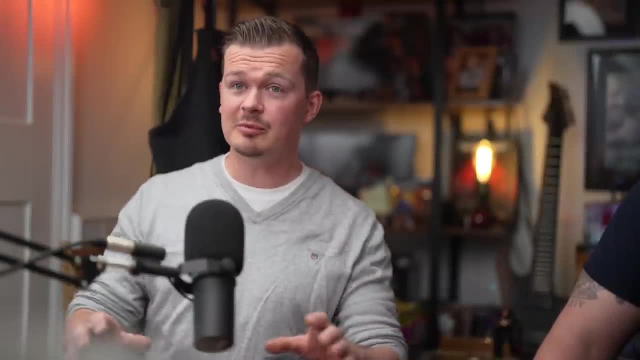 i know it's easy for us to say you know blowing our own trumpet, but it's. it's a fun game to play. yeah, yeah, but originally we had to play it with proxy models. yeah, using warhammer models the game was still fun. yeah, but then with our models, that just it all came together. yeah, it never felt like. 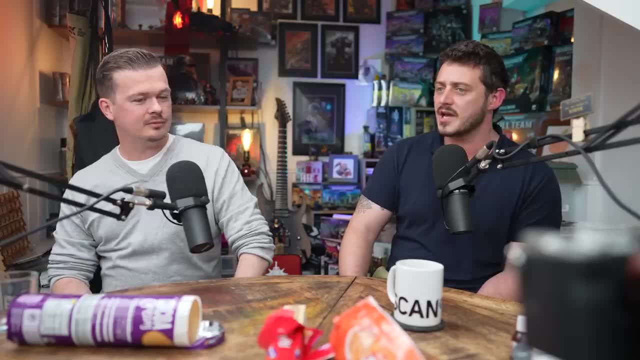 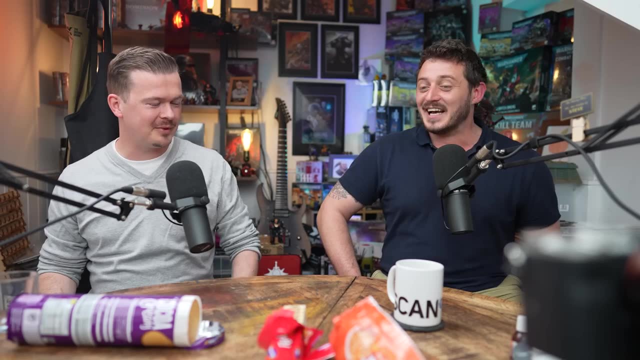 war and terror when we were playing with proxies. yeah, yeah, which was a shame, it just felt like a random edition of 40k because i had a lot of spare 40k models. yeah, is this what tenter be like? oh, no, no, I don't want to keep knocking. no, i mean, you know, they're an inspiration to a lot of people, you know. 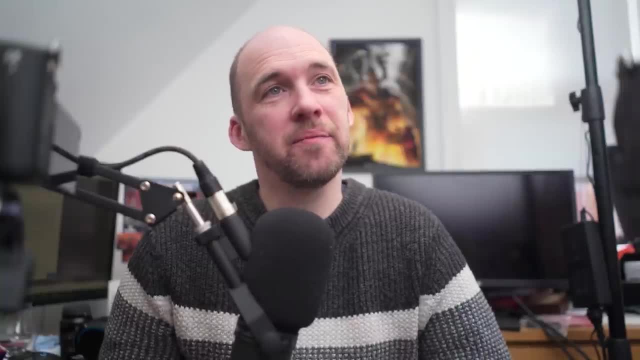 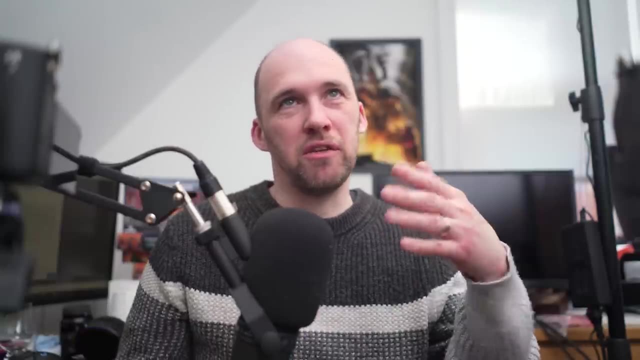 they're. they're a good yeah. yeah, if they hadn't been around and we would, i wouldn't be doing no, there's also nothing wrong with like having your own opinion and being professional about like how you- yeah, you see, like the competition- i wouldn't say competition, but you know, games workshop is- 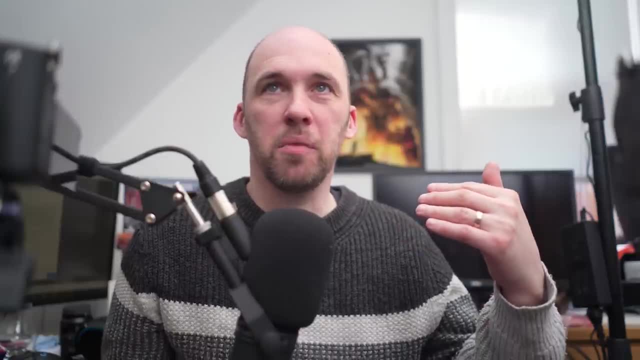 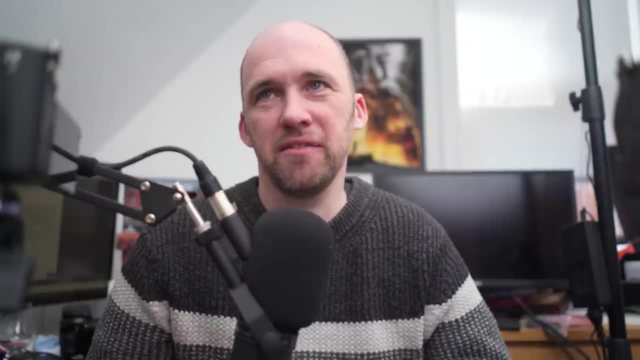 a love that i've had for decades, but it's not perfect. there's always things that can be better, there's always things that in like that's a weird decision or whatever. so, and we're not going to have to keep apologizing, we're not not going down the route or like: well, you have to play 40k or war and play both. yeah, play both. 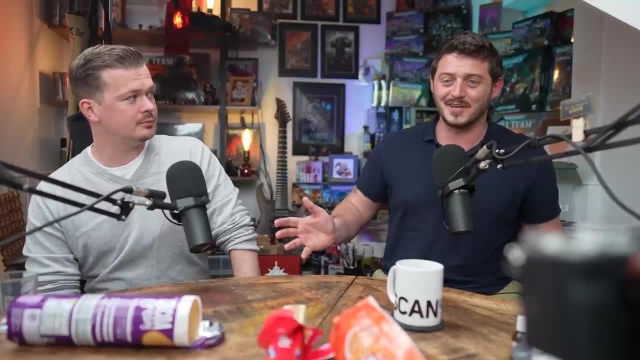 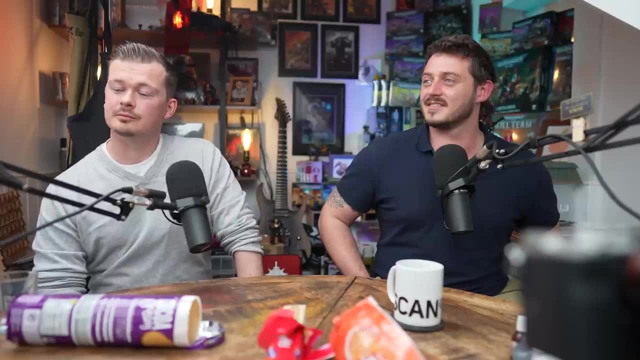 yeah, we've got loads of board games at home. you play all of them. yeah, you don't have to stick to one, play both, it doesn't matter. play more. yeah, play all the games. yeah, someone has said: with such a potentially bloated market, what do you think the USP for war on terror is and why is? 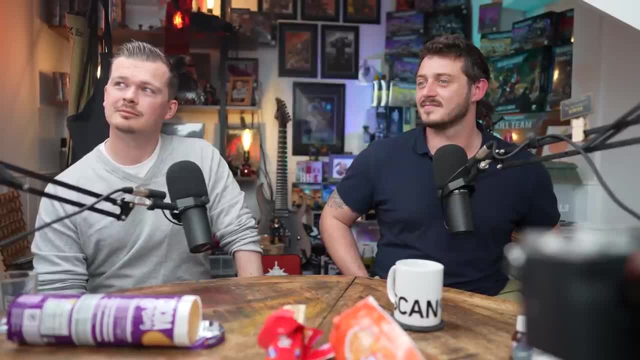 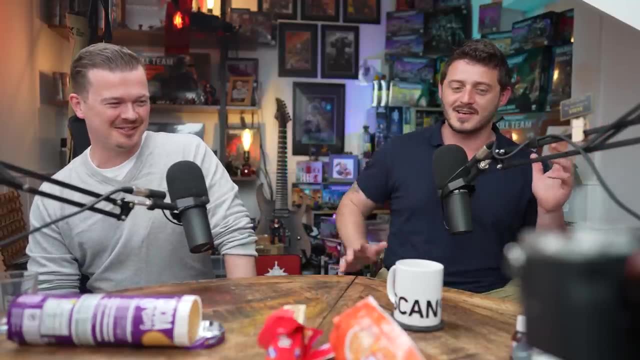 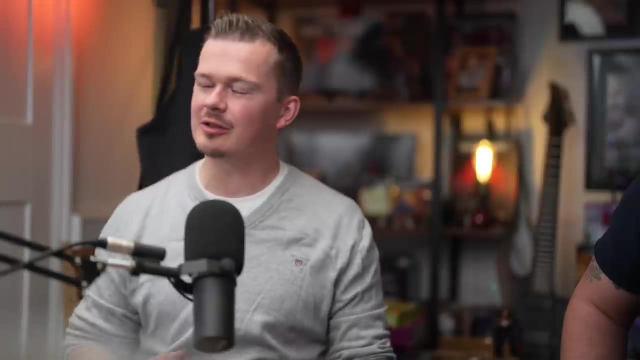 the answer because they look like amazing zurg aliens. no, no, that's, that's just the answer. they've already caught us out there. no, um, the us? uh, well, yeah, i've thought about so many times. we can, we could rattle off in all the ways that we think. 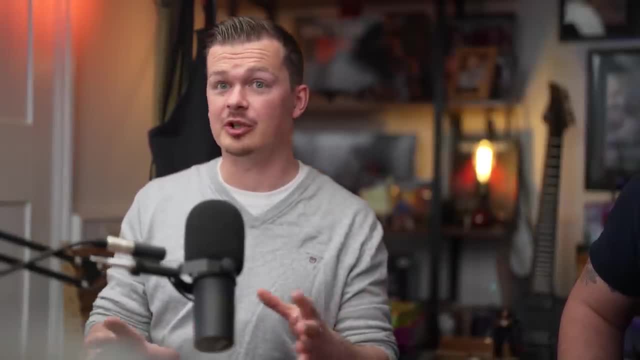 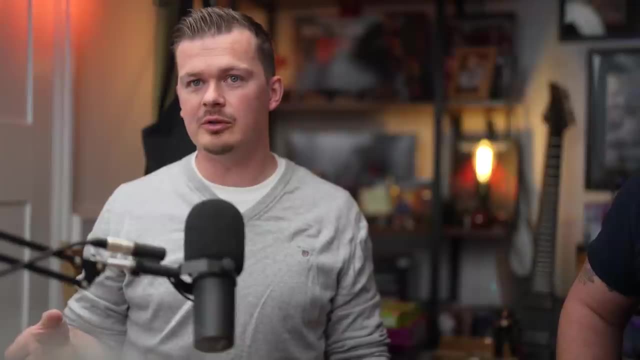 our game's different. you know, we've got rid of attachments. that's that makes a huge difference. yeah, it's streamlined because we've removed certain roles. yeah, like i'm rolling to hit you, then i'm rolling to wound you, and so i've succeeded in both those. oh, you've saved it. 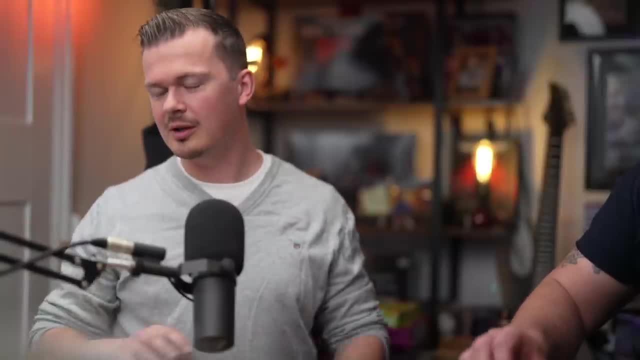 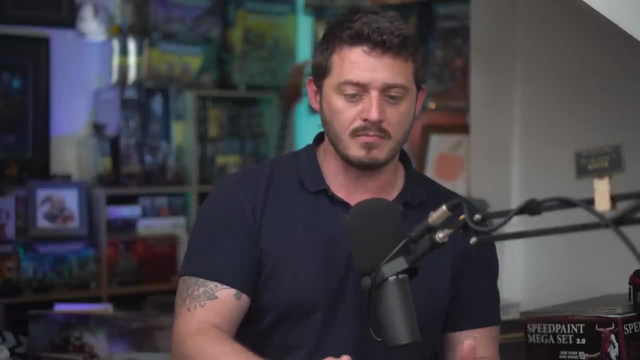 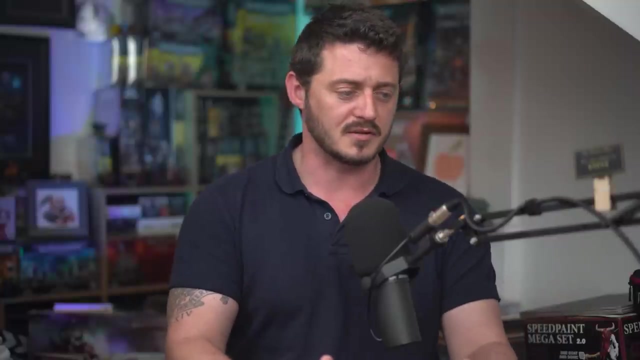 that never made sense, did they hit you, yeah, and wounded you, yeah. so yeah, an example of why i specifically wanted to get rid of that rule was: i mean, there are multiple stories of real world military um sort of tales. i suppose um didn't know i was going to finish that sentence. 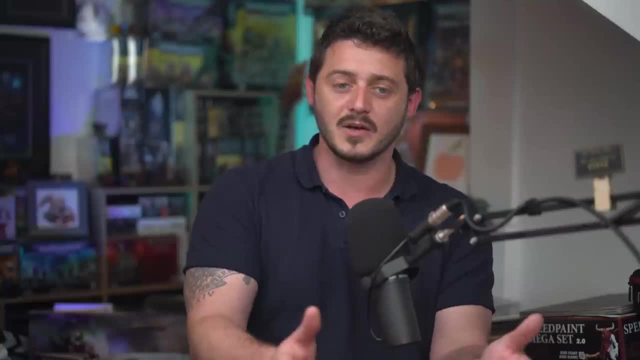 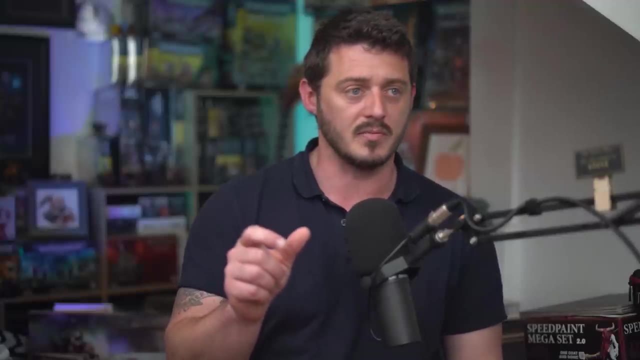 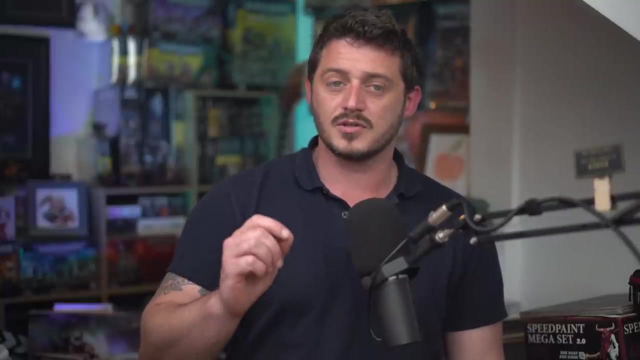 but people have been shot in the head. okay, and this is why you wear a helmet. yeah, the bullet has entered through the helmet, but the the air pocket within the inside helmet has curved the bullet around the skull, around their head, and out the other side of the helmet. wow so. 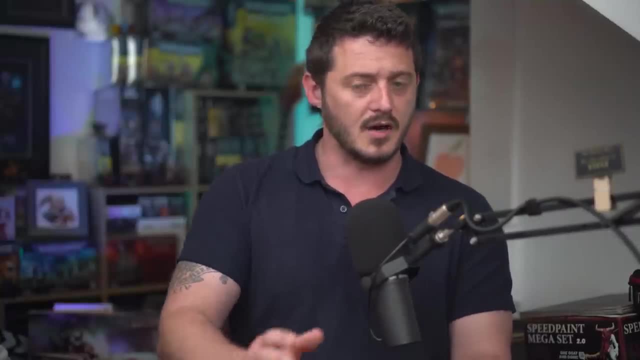 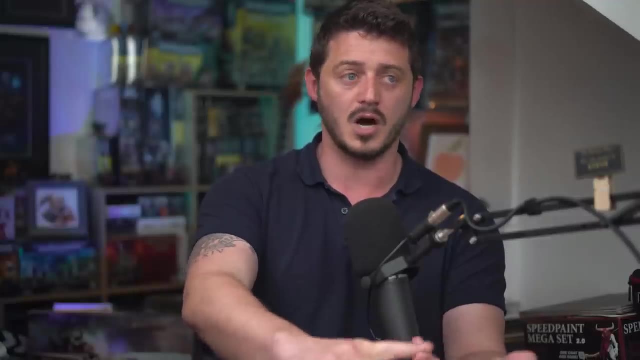 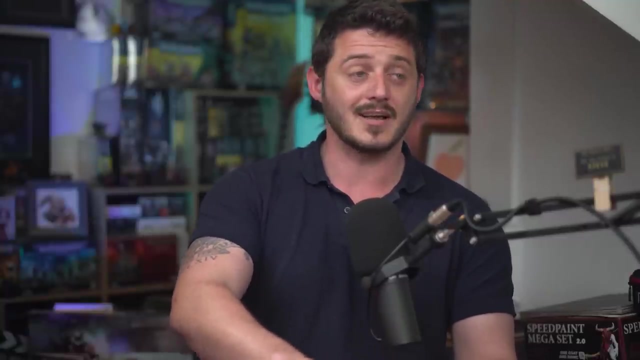 this is where 40k and i know they're getting away with the the role now in 10th i think, but previous editions it was: yeah, roll to to hit, roll to wound, armor save. all you need to do is roll the change the order. roll to hit, armor save. then you roll to wound. yeah, because that guy that. 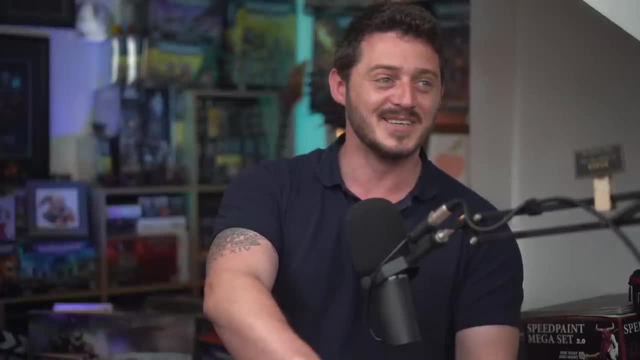 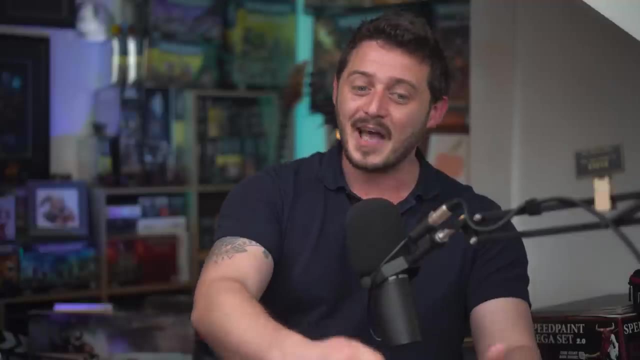 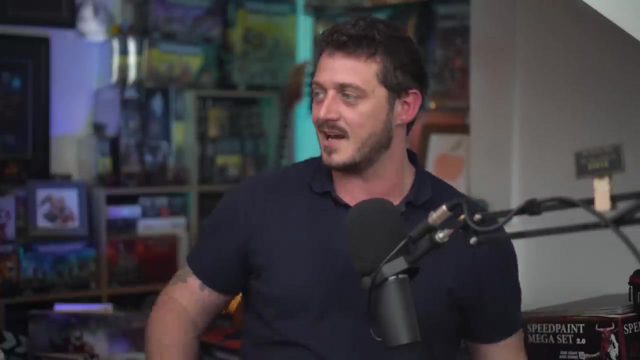 helmet, that armor failed, yeah, but it still failed to wound. yeah, yeah, so that to me that makes sense. so he, he got hit and his armor failed, but it didn't wound him. yeah, yeah, so that made sense. but doing in the wrong order, that never made sense. yeah, like that. that's, yeah, streamlining that rule. 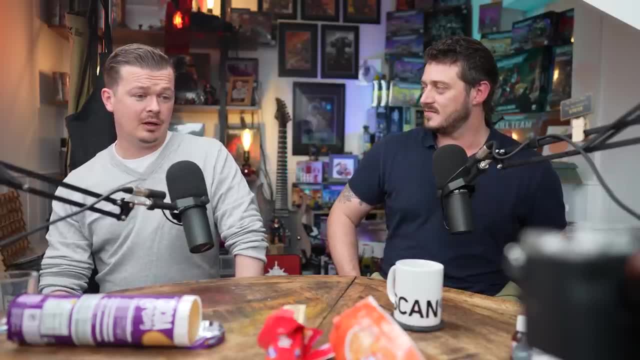 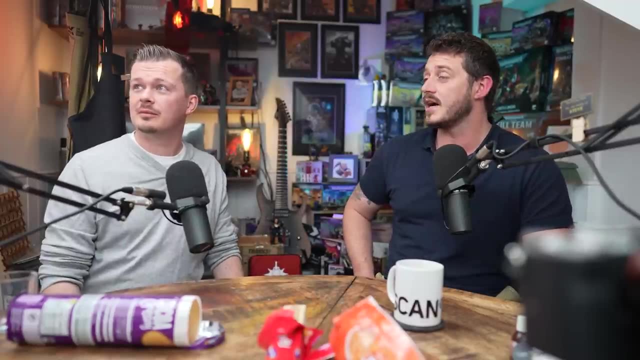 made sense. yeah, it's. um, another thing is because a lot of people ask us whether it's a skirmish game or an army. that as well, and oh, that's probably our main one. yeah, yeah, actually thinking about it. the scalability, yeah, so because, obviously, removing being- and i'll keep calling it- coherency. 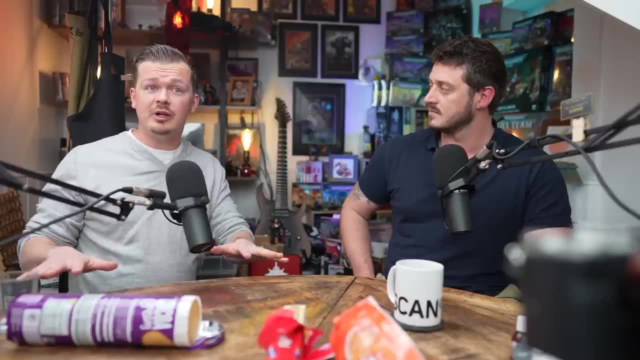 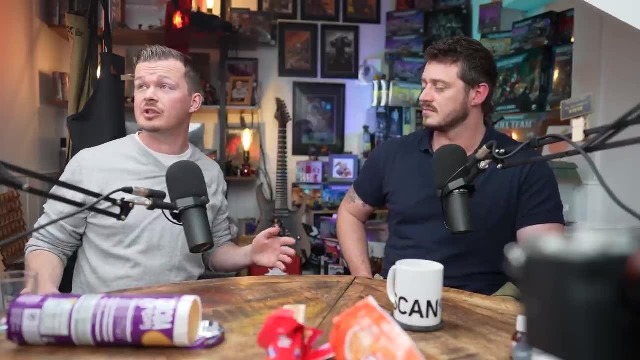 because that's probably what people might think about it, but it's a skirmish game and it's a more familiar with. but yeah, because you can spread out and each model is its own thing. you can play five versus five or five hundred versus five, complete the same rule. so yeah, um, all i'd say. 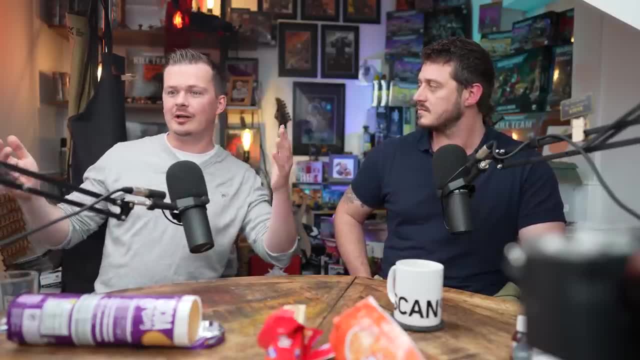 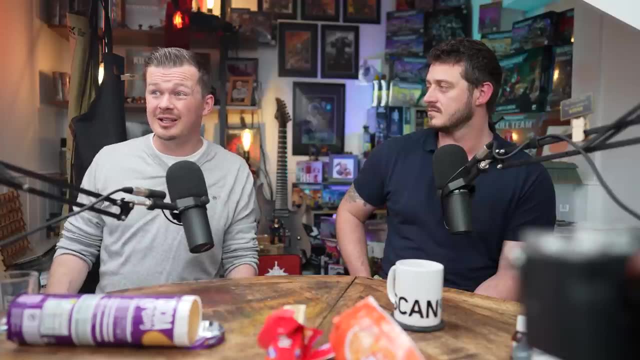 to discover it is. i know it sounds like you've got a thing going by, but if you play it, you'll understand what the unique selling point is. yeah, it's, yeah, it's. above all else, it's a fun experience to play again and again. i know it's. you don't want to say it, because you're trying to say it. 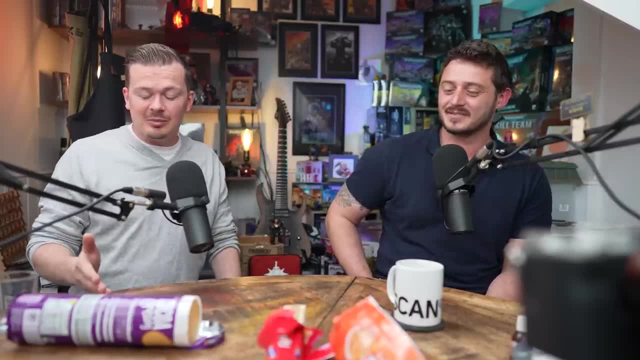 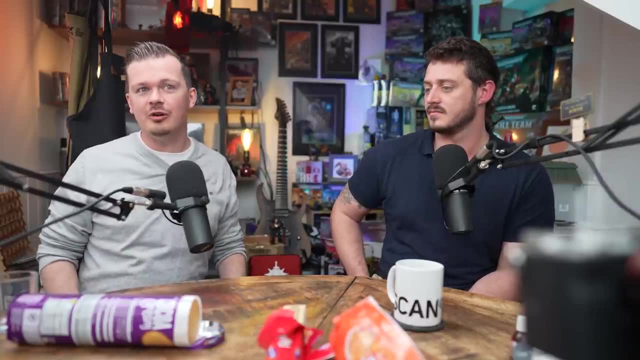 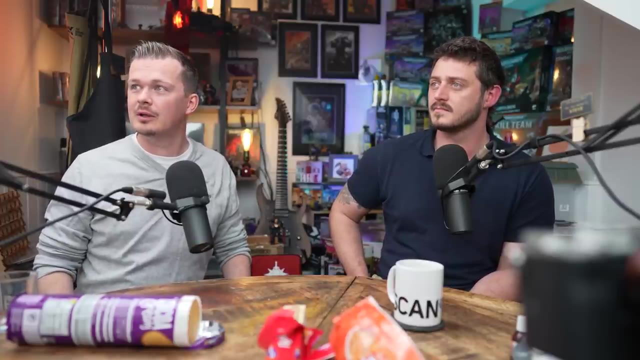 yeah, yeah, yeah, but it's generally. we created it because we want, we like tabletop, but we wanted to play the most fun version thereof and if we had to create that version, then, yeah, that was the way to go about it. yeah, someone's asked three questions, but i think we've covered quite a lot of them already. but they do say i love. 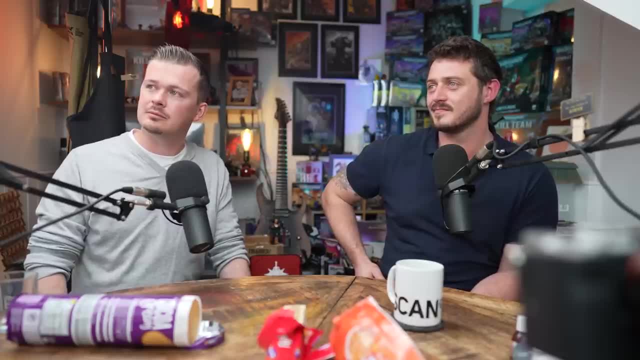 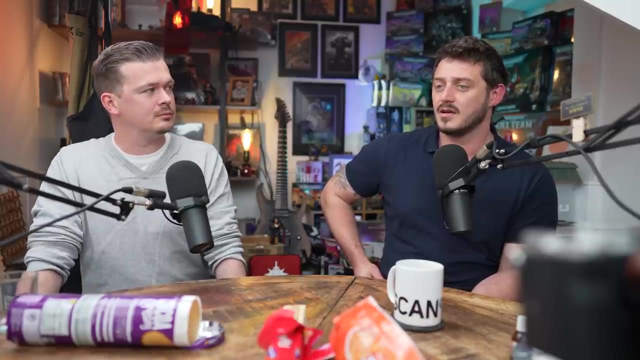 the varied dice types and different mechanics, both additive and subtractive roles- yes, some kind. sometimes combining the two you could get even more granular and interesting than necromunda even um. so the the additive and subtractive dice rolls were well, they helped us get around cover. 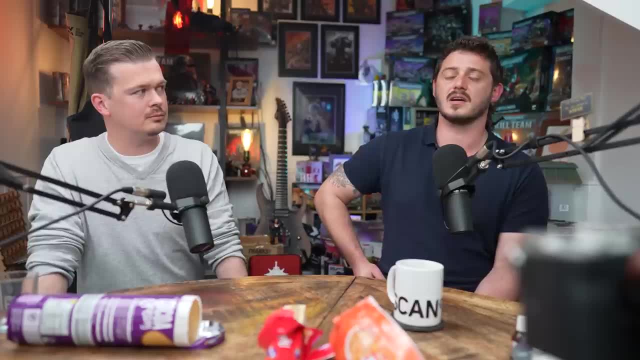 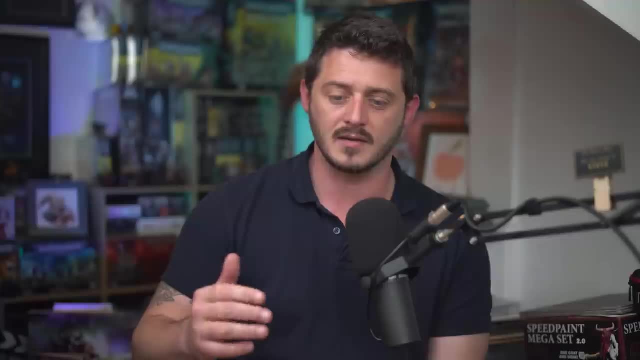 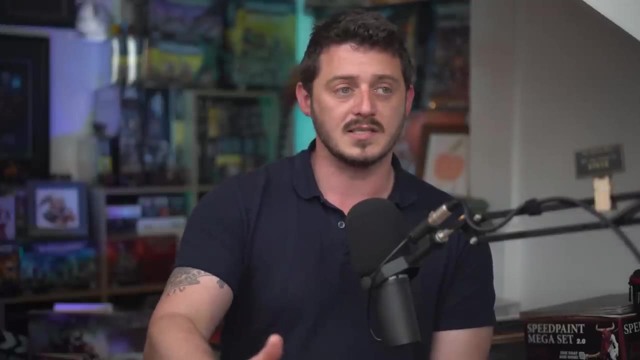 cover save in terrain. were there's no such thing as a cover save um in the game, it's. terrain gives you certain additives and subtractives, and by that we mean if the enemy can see not 100 but more than 50 percent. if you need a 13 to hit because they're slightly hidden. you need to. let's say, on a d20 you roll a 15. well, you've got a subtractive d6, so you roll another d6 and you subtract the total. so then you, if you've rolled two or more, you've missed, yeah, um or three. 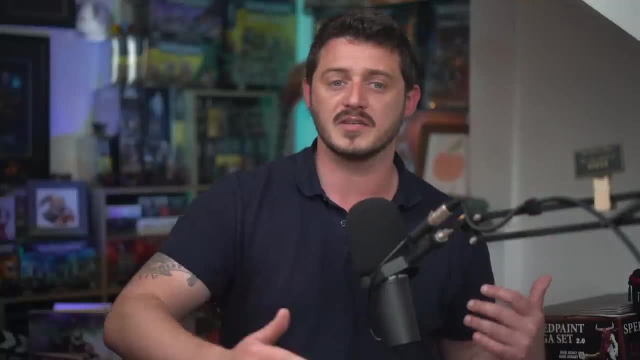 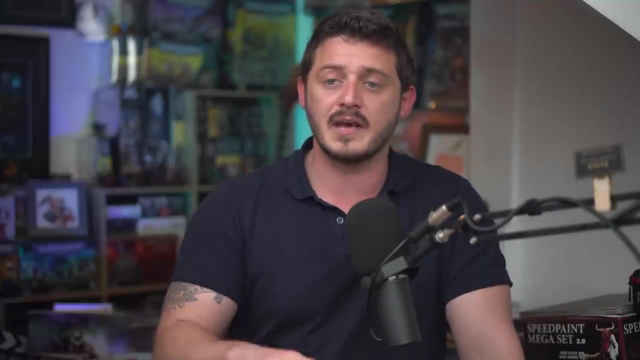 or, more sorry, um. but then you can have more than that. you can have a subtractive d12, which makes getting hitting people very difficult, and they're accumulative so, but they never add together. so if it says 2d6, we mean 2d6, they don't become a d12. yeah, because 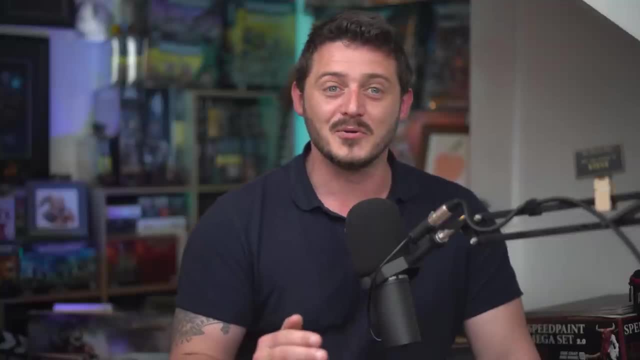 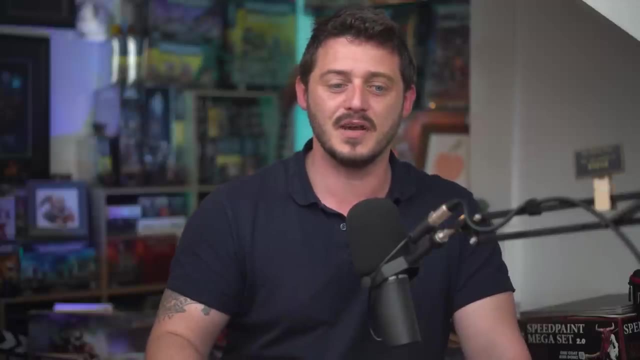 i'm 2d6, you can't get a one. yeah, so it's actually beneficial for you. yeah, so roll 2d6 instead of a d12. yeah, so the maths works and we've kept it true to that. so if you've got a shield, everything. 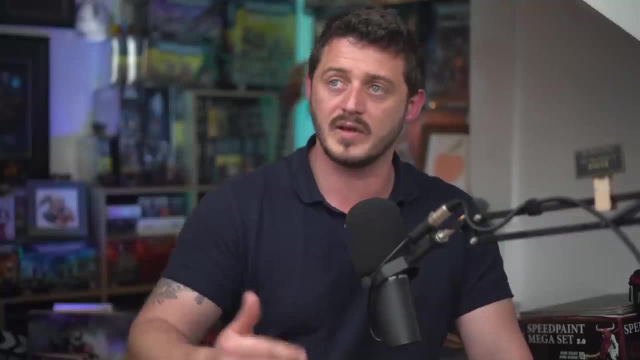 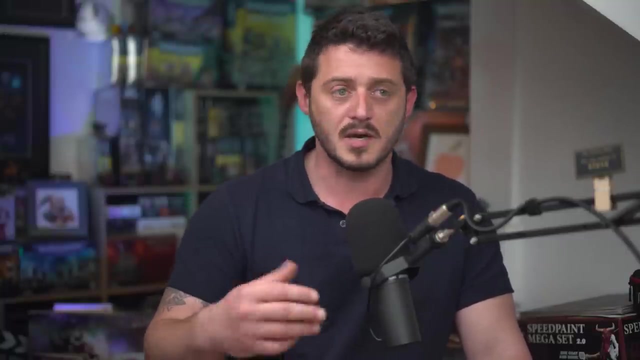 attacking, you has to roll the hit. roll with a subtractive d6, yeah. however, if that guy with the shield is behind cover with a little bit of cover, minor cover, that's 2d6 to hit him and it makes it very difficult. sniper fire. get no uh, heavy weapons if you stay still for the turn, set up a. 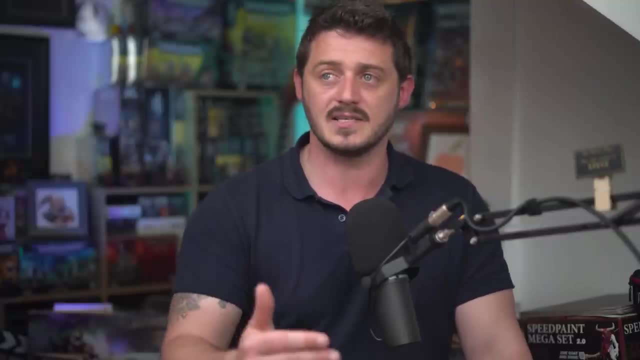 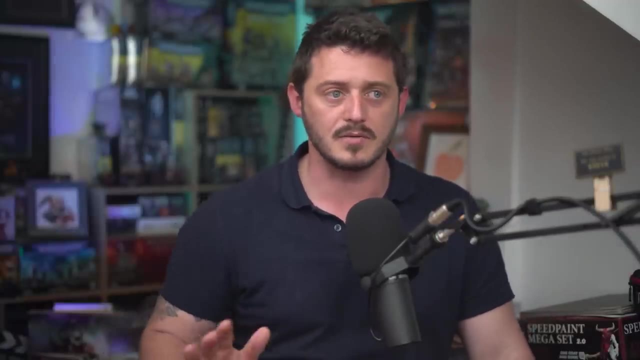 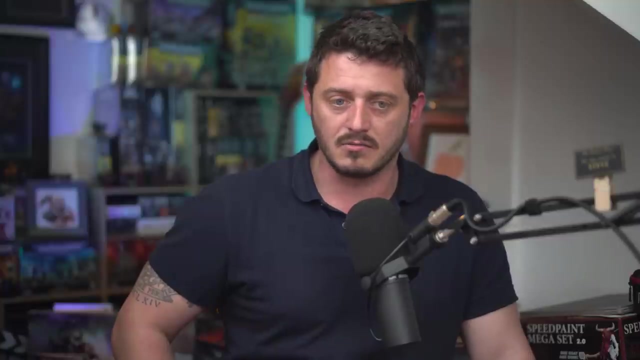 proper firing line, uh firing position, and you get additive d6 to your hits. certain cannon rules and things like that get additive d12s if you're only firing the cannon and you haven't moved. and it just gave the scope, the game such a wider scope, hiding behind terrain and it feels like 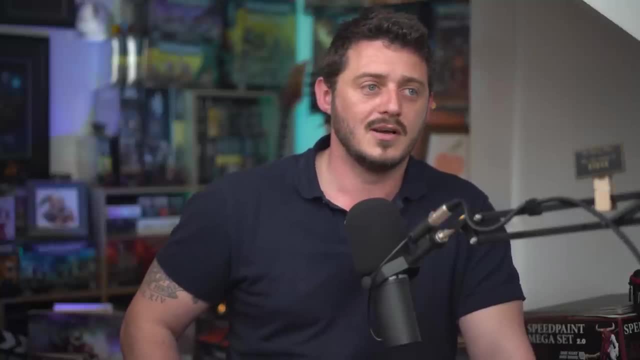 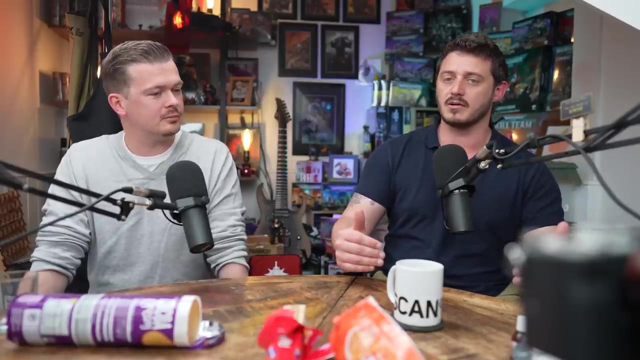 sometimes moving up the board like playing gears of war, yeah, yeah, where it's all about hiding behind terrain and poking out and shooting and then jumping back in and i've been replaying gears. oh, and it's fresh in mine then. yeah, it really fit. terrain is so beneficial in war on terror. 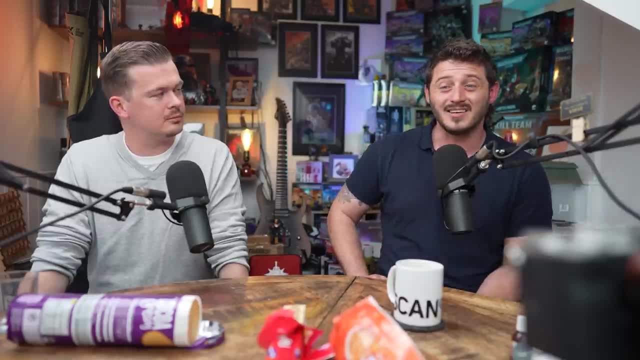 whereas all my time playing 40k when i was younger, i never actually considered a lot of terrain. yeah, it just didn't make sense to me. and another thing that didn't make sense in some games is you only get one save roll. so like, if you have, let's say, you're playing a space marine librarian, you have. 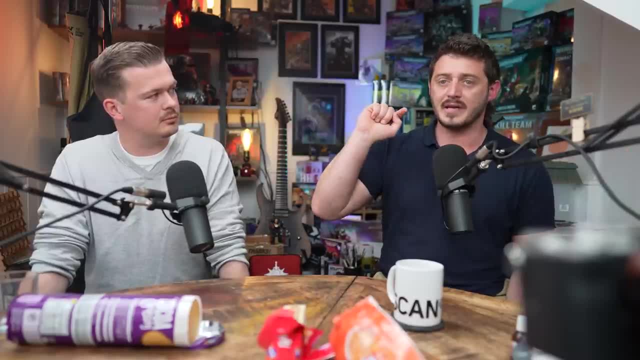 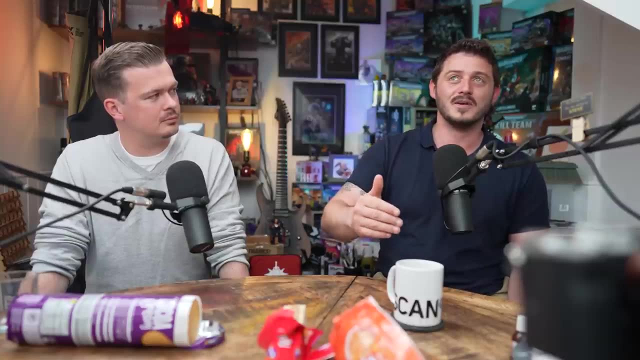 that invulnerable psychic shield around you. the bullet makes it through that. well, it still has to come here, yeah, yeah. so why does it? why can i only roll one? and then if i'm behind a wall, then surely i'd get to have multiple saves, because then it has to get past the wall, then it has to get past. 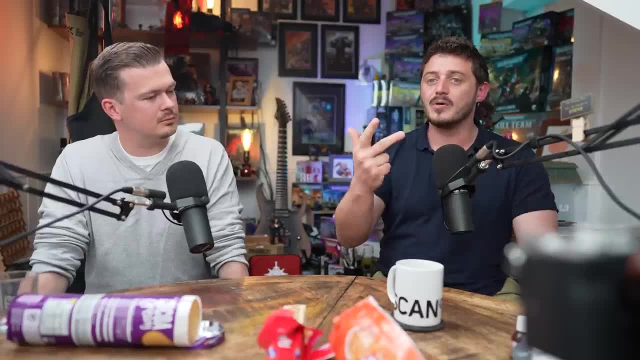 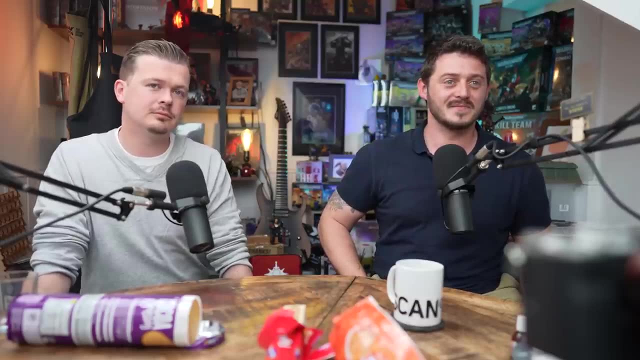 the shield and no psychic shield, then it has to get past the armor. but i'm only allowed to choose one. yeah. see why i always yeah, because there's a time where that would make sense in time that wouldn't make sense. so if you got hit by a plasma gun, your armor wouldn't, because it's like i don't. 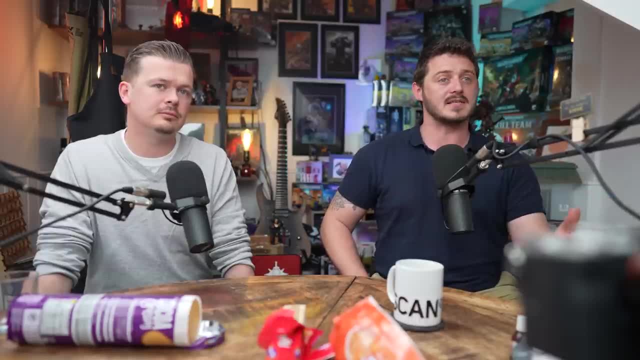 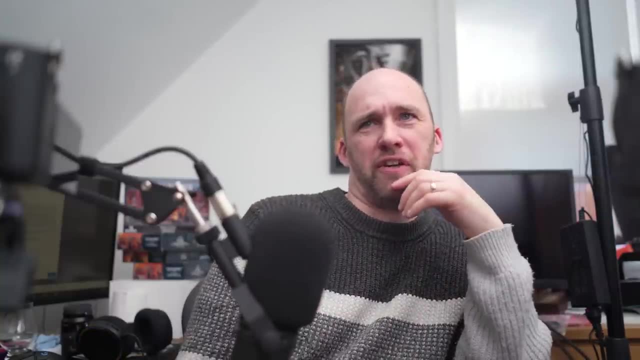 know i'm a piercing. whatever it immediately goes through, you have to use that, but then you will not, because it will just melt it. yeah, but if it's like a gas machine, a las gun, you're like, well, i'm going to use my force field first and then, if it gets through, that then sure, which makes then. 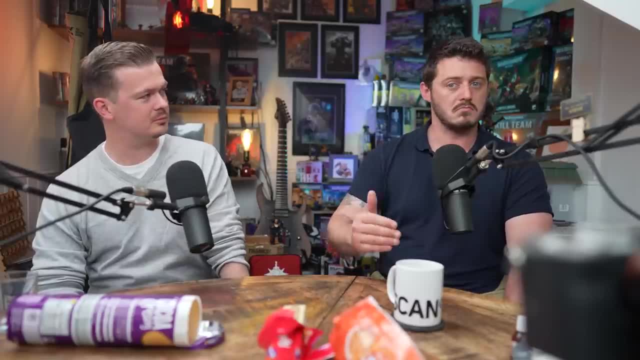 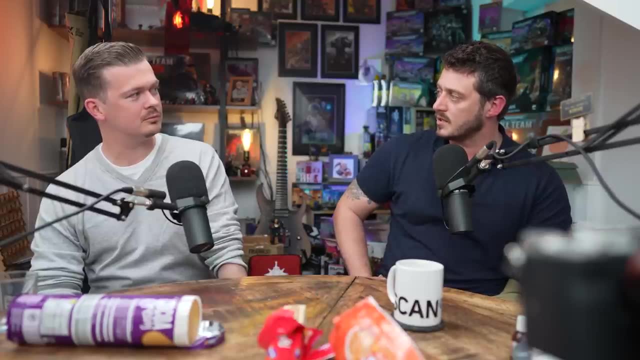 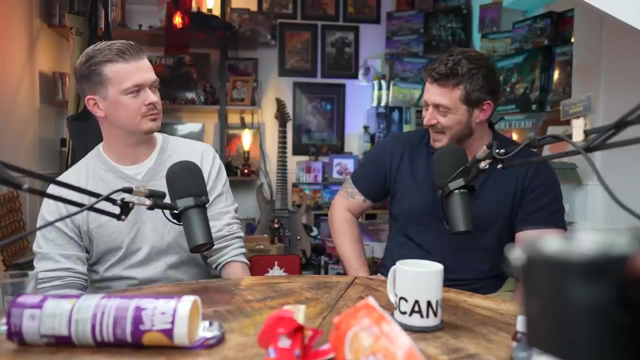 having bringing setting armor penetration weapons for certain things much more valuable, yeah, but still only allowed to choose one. so that didn't make sense. so it probably took us the longest- i'd say a good two to three years- of just trying our best to ignore it. actually, i want to say 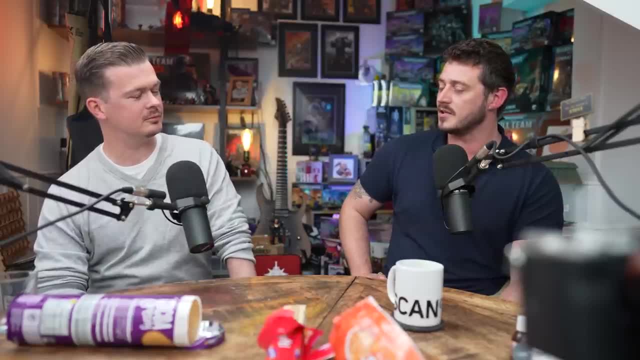 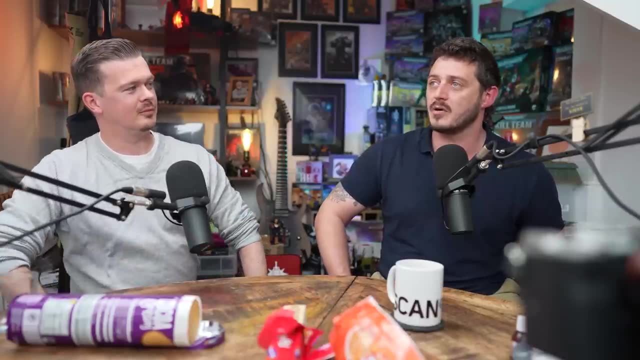 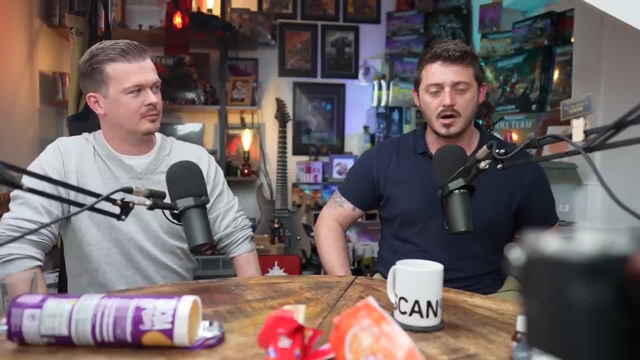 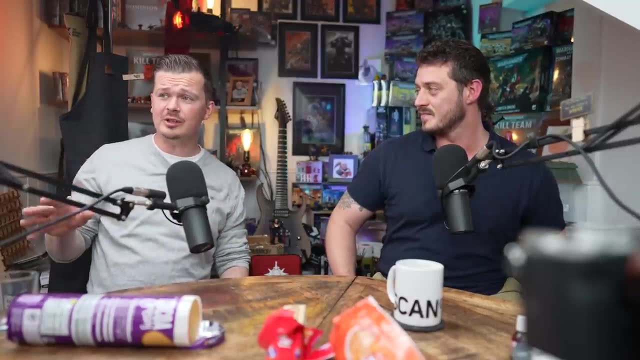 role. and then we were like, oh, that's a good idea, oh, that might work with this. oh, it does. oh, let's, let's do the cover the amount of examples. that might start to sound complicated, but it's. it's really not, and the way we've used it with so many different elements, it just 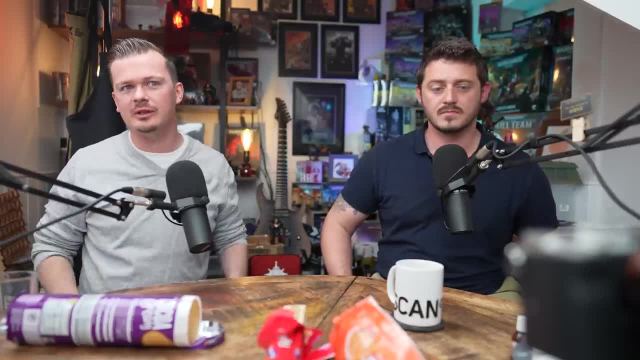 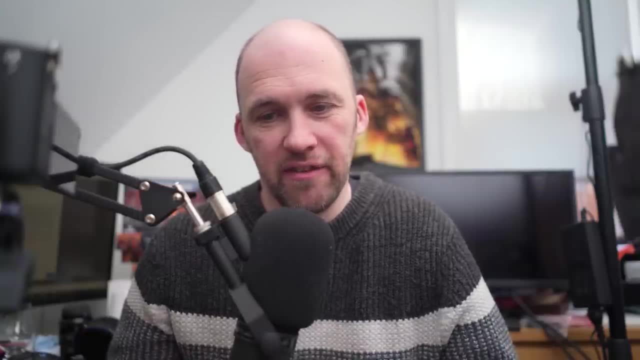 yeah, it makes everything work and everything have a reason to. from a wargames point of view, it's like a lot of war game. uh, certainly, like myself. like you make scenery, you want to make it look like it's livable and usable, but a lot of rule systems out there just don't account for this, so they just 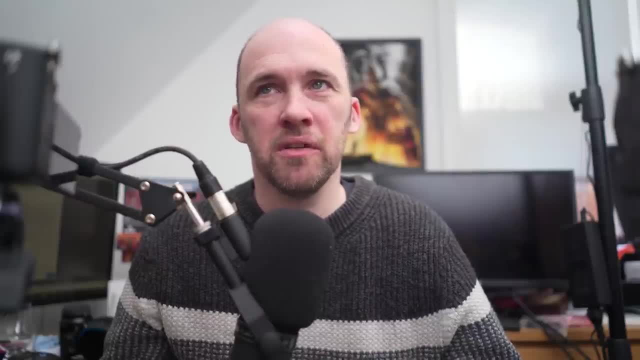 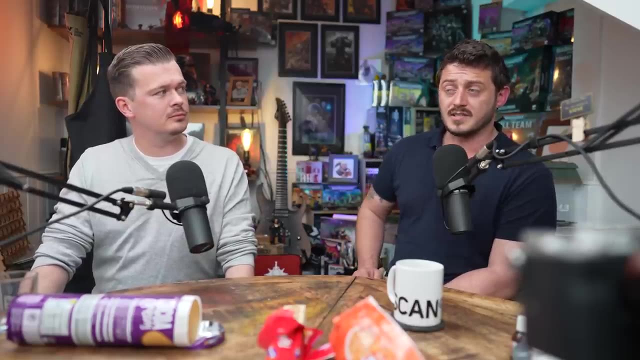 become interesting line of sight blockers, as opposed to if you can see any part of the model, you can shoot. yeah, and it doesn't matter if it's the tiniest little hole for a window, the shot is there. yeah, it's going to be a detour subtractive d12, but 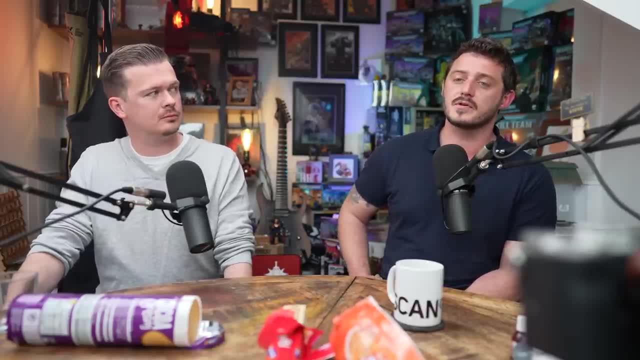 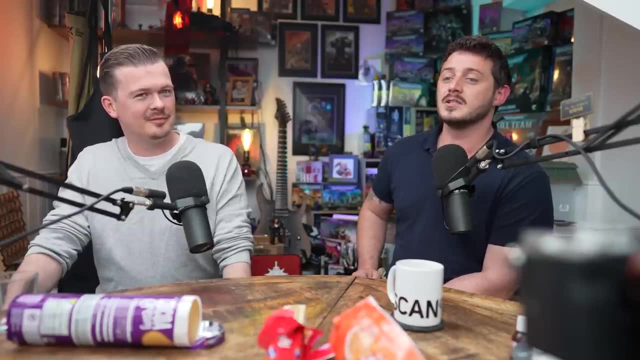 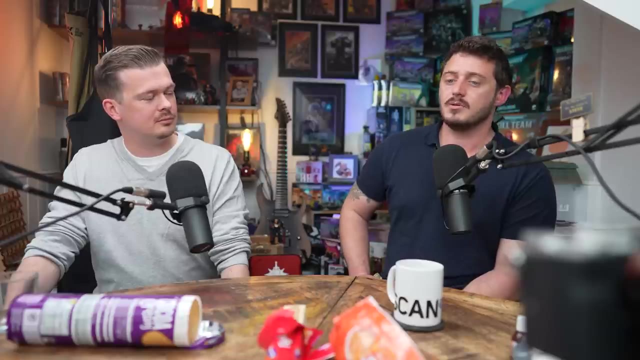 and there are impossible shots. you can throw a fire through into infantry in war and terror, but there is a grid, firing through attachments grid- everybody loves a grid- and depending on who you're firing through- whether it be friendly, light, friendly heavy enemy, light enemy, heavy infantry- it makes your hit harder, so it gives a bonus. so if you're firing through, 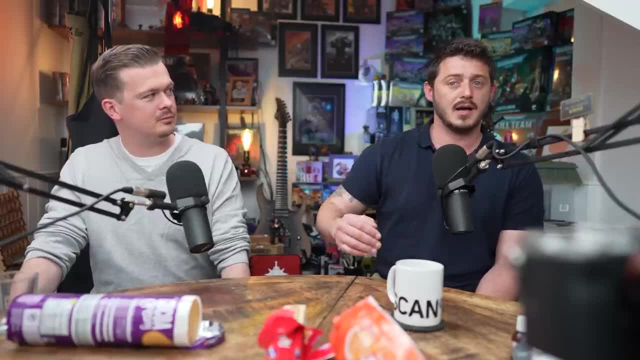 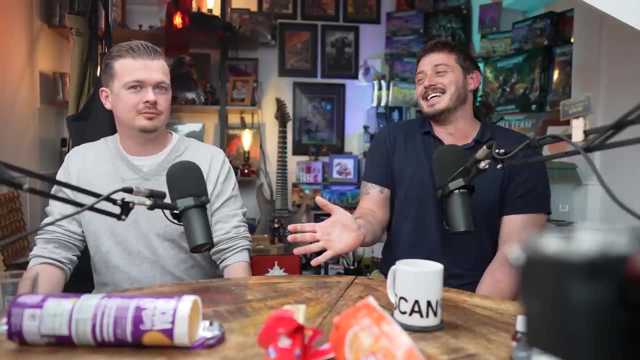 a couple of light and friendly light infantry and they're also behind a wall. yeah, i'd give it a go, and we've had a couple of shots like that where it's like i need a 19 or 20.. that's quite cool as a- i suppose, a scenario. you've got like some big bad leader and there's all these guys in the 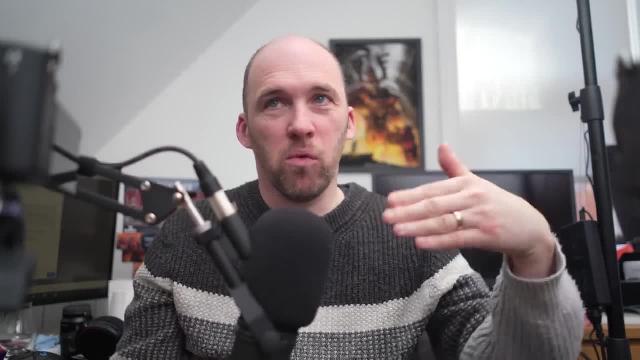 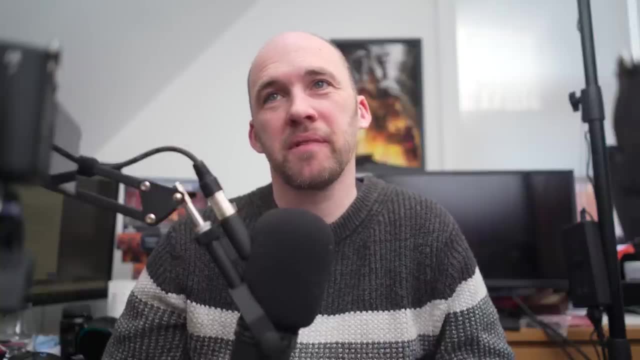 way in walls. you just want to get your sniper to take out the big bad leader. you've got to work your way through these absolutely things and it's like, yeah, it's the impossible shot, but there's a chance you could do it. yeah, and in war on terror, you don't want your captains in front. 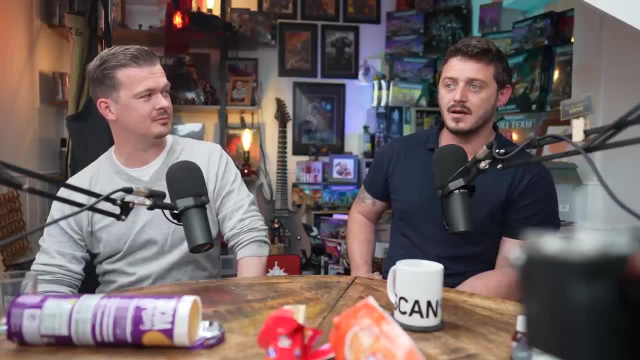 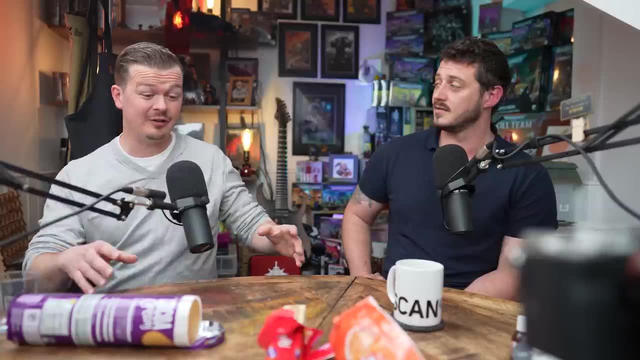 yeah, because you want to have that. well, yeah, you want to have that human cover. yeah, you want. you want that cannon fodder. yeah, yeah, operation meat shield. but that being said, if you're all out in the open, just because you are at the back, it doesn't mean he's perfect. yeah, yeah. 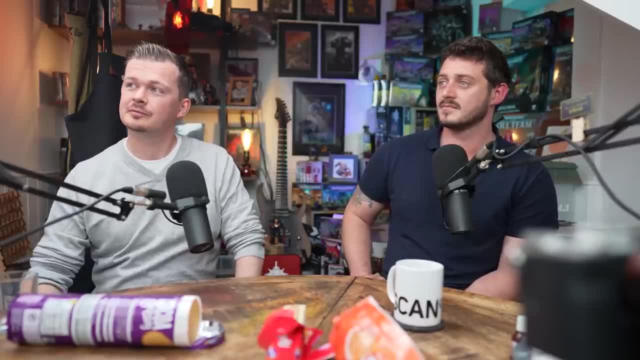 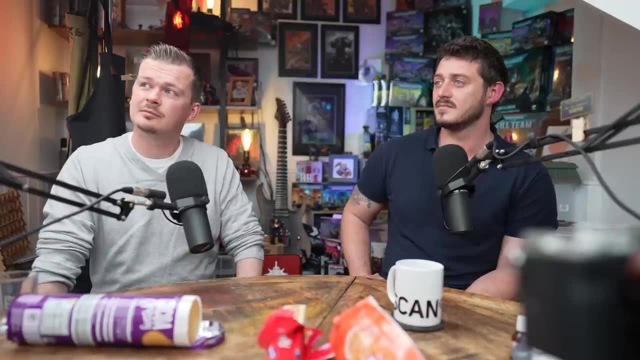 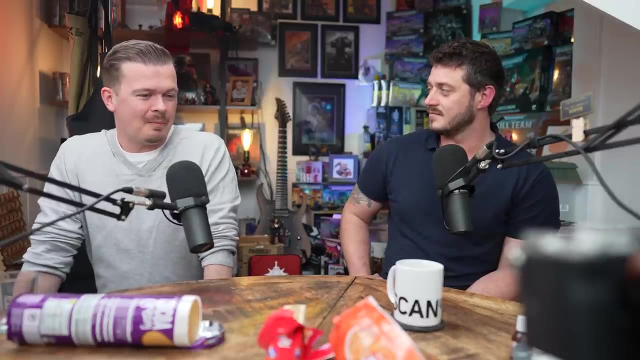 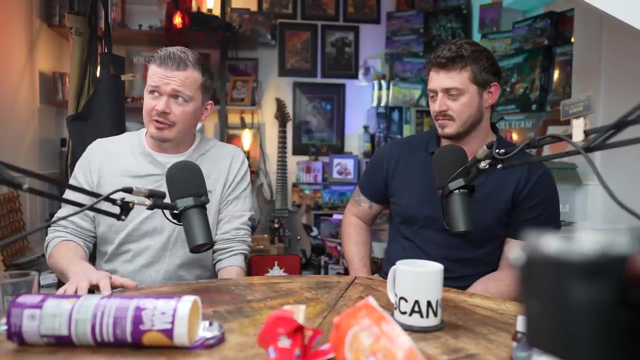 yeah, yeah, genius. yeah, that's really interesting. um, one of our patrons has also asked um what are the three most important steps to complete before taking a game to kickstarter? oh, wow, okay, um, i guess i really like that one. i think- and i know this might sound obvious and stupid- but having a game, a finished game. 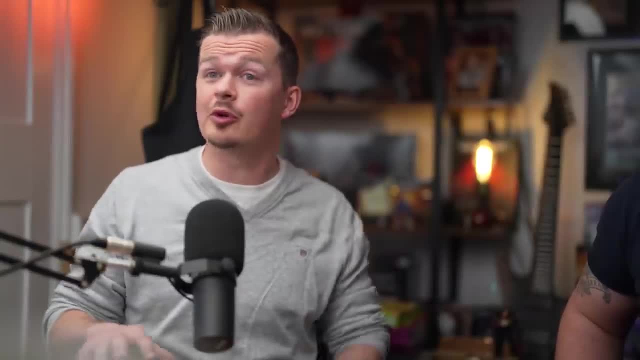 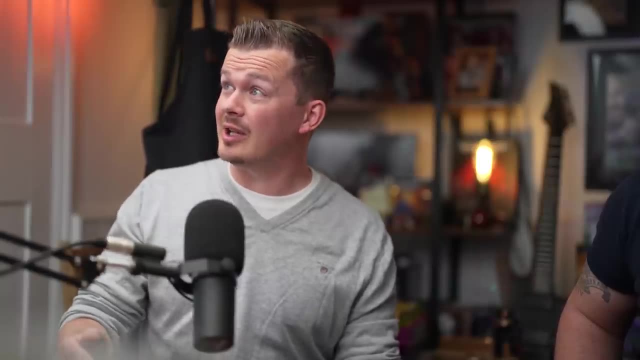 to yes to kickstarter, yeah, the amount- and again i'm not knocking them- yeah, different ways of doing anything but the, uh, the amount of kickstarters. you do see where it's all it's. basically they're telling you their ideas and concepts. okay, yeah, yeah, um, so in their mind it's, it's kick-starting. 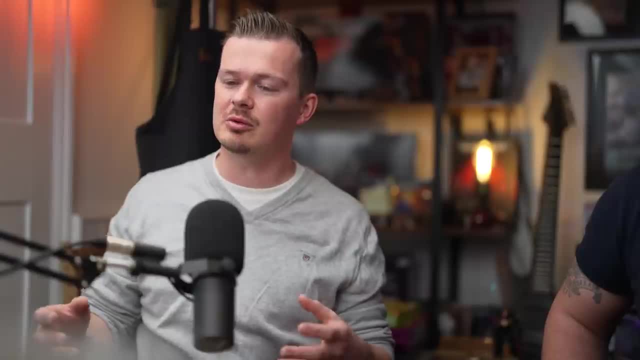 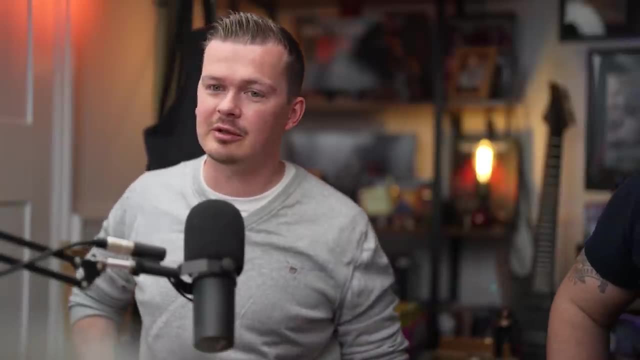 to getting it to be an actual product. yes, in my mind, kick-starting is you. it should be, no, you have the products. you want to show people they're going to get something, yeah, yeah, and the kickstarter is to get it, you know, get it in people's hands, so so i guess in in. 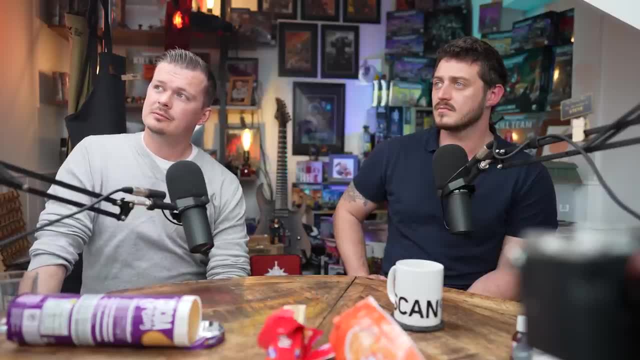 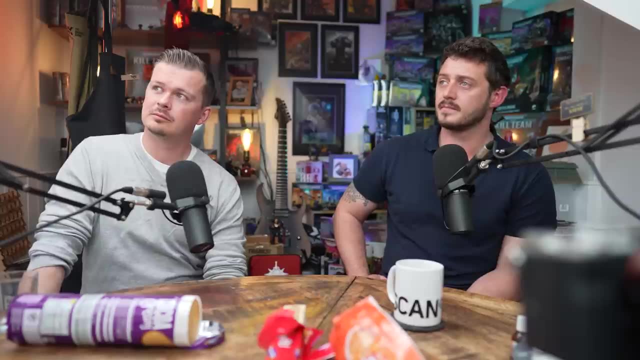 i guess the thing that springs to mind in my mind in in like wargaming painting, is duncan, uh, kick-starting his own paints. they did have them all yeah formulated. they had the product yeah. so that makes, yeah, a lot of sense. it's a big one and that's that's where stretch goals. 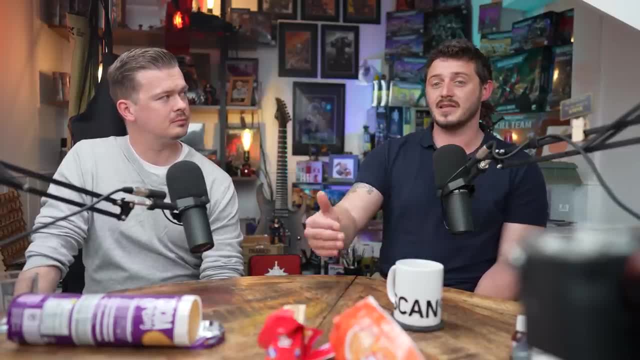 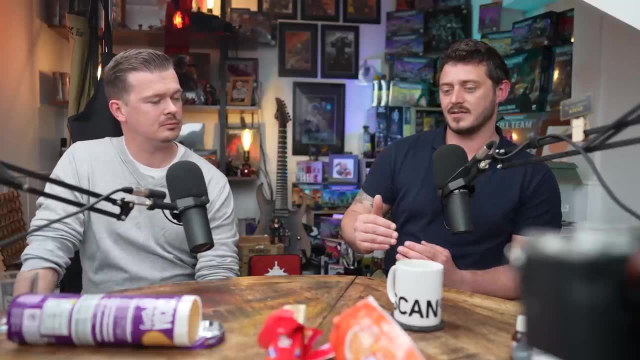 come into it as well. it's just like, if they've got stretch goals, if we meet this much, we'll be able to get the product like this and it's like: so you don't already have the product, good to go. yeah, you, you have an idea, yeah, and you think, oh, we might be able to make it in metal. 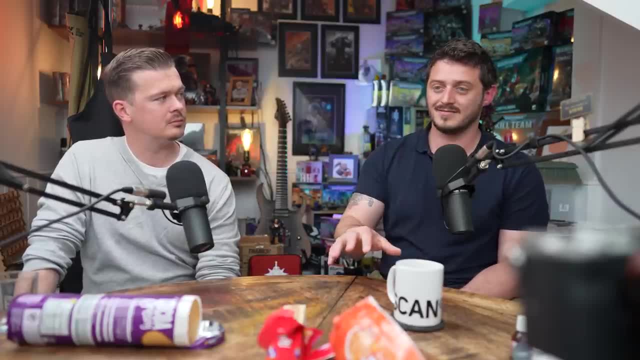 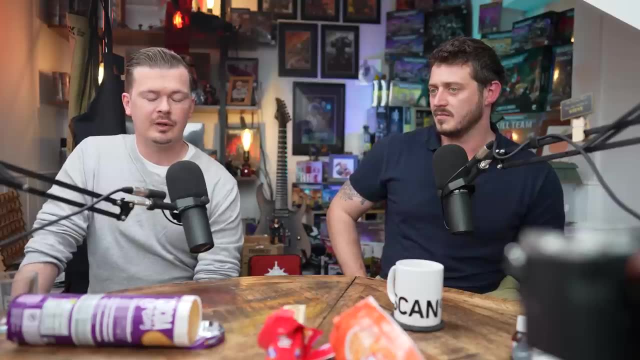 if we had this map. it's like, no, just get it, just figure it all out and then go: yeah, yeah, um, it's hard to think of like another couple it yeah well, yeah, because that's sort of all encompassing it's. yeah, i suppose the second biggest thing is obviously you need to get your name out there. 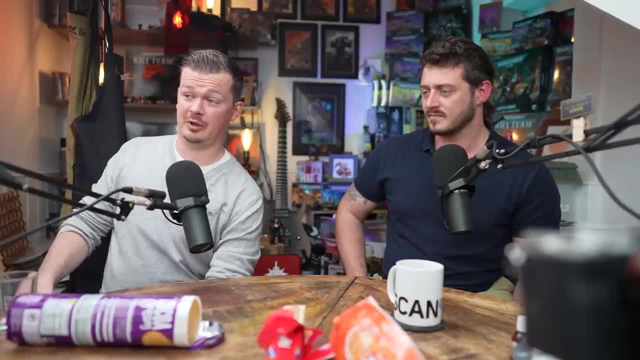 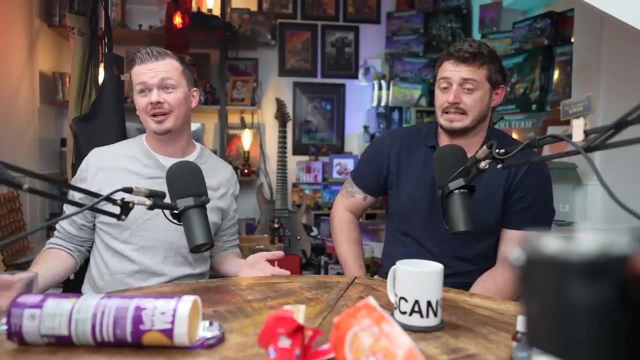 yeah, um, obviously, by the time this video goes out, the kickstarter will be live. it is our first kickstarter, so it's difficult to comment because we don't quite know. yeah, i don't suppose you ever know until yeah, it's there. i mean, yeah, you want to have your name out there, you want to have a bit of a following. 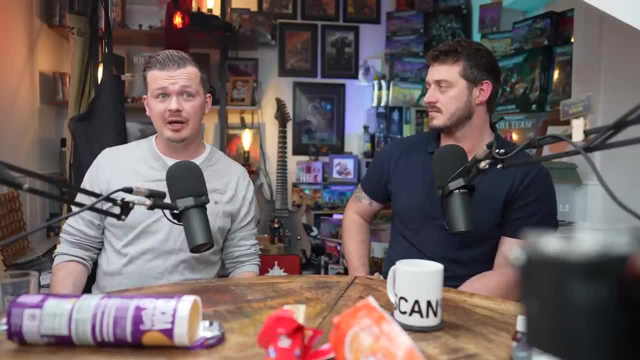 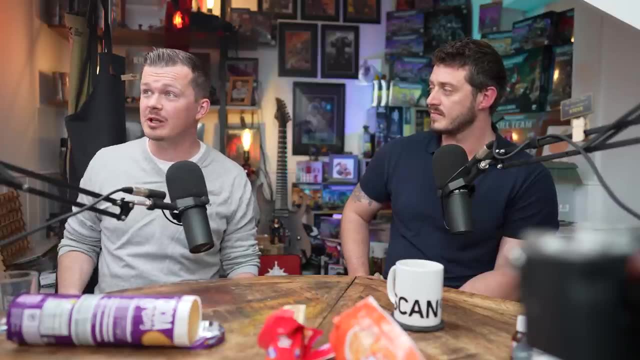 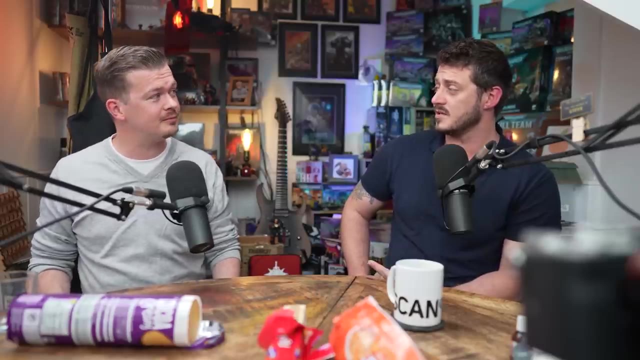 uh, we've got a small backing, um, comparatively, um, yeah, so obviously, the yeah the more you can get, the more you can get your name out there. you want to talk to people, you want to contact people like yourselves. yeah, yeah, um and yeah, and i'll just try. actually got one and it's it's attached to. 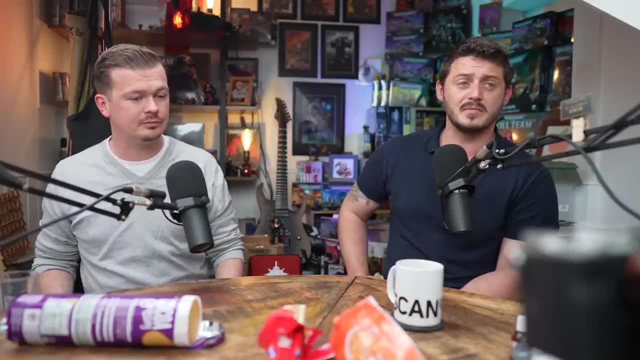 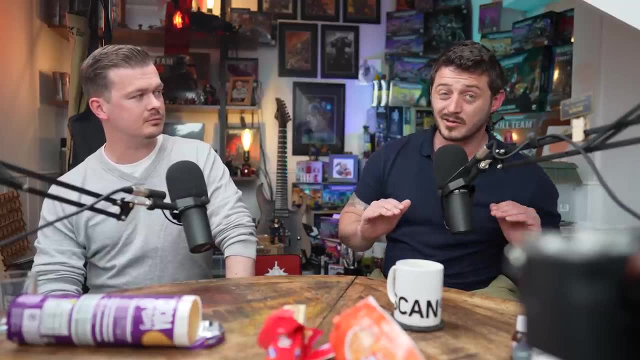 that one make friends. yes, yeah, go to conventions, talk to people. it's it's well. it's how i started in the zoo. it's like started in a gift shop. i ended up just talking to people. make some really good mates, making some good cup of teas and coffees, by the way, it really gets you far. 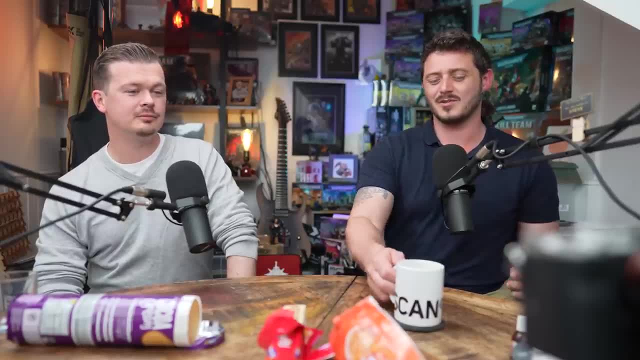 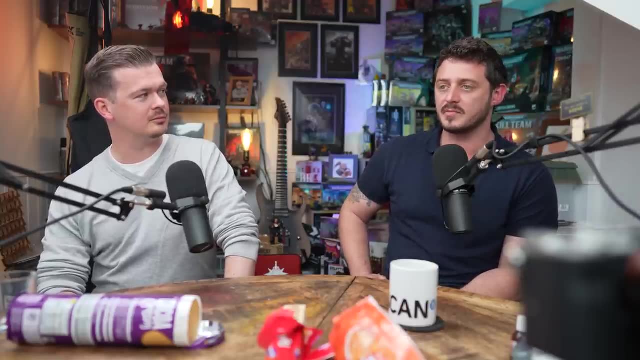 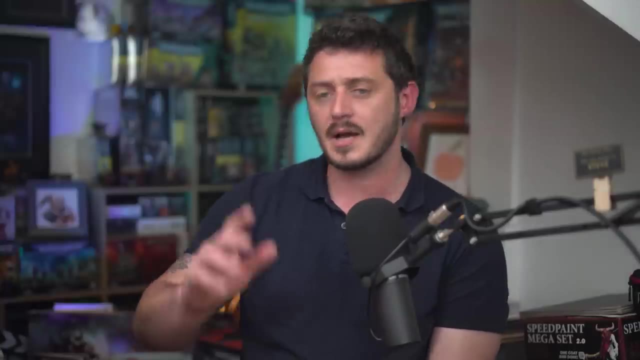 that's a tip for life. yeah, sorry about that coffee. yeah, well, i'm not gonna say anything, but, um, just chat to people, make friends. you'd be surprised how many people know other people. yeah, and then as soon as they start knowing your name, they're like: oh yeah, i know you guys. oh, 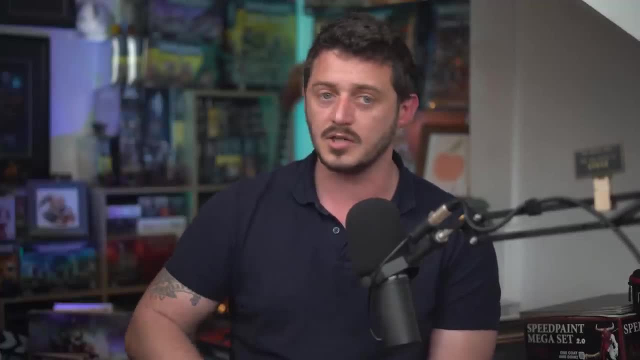 absolutely. yeah, no, that's cool, we're doing this. uh, do you want to come along? yes, yeah, yeah, just be friendly, be nice. it's a nice community. get involved. yeah, yeah, i'll take. get yourself on some podcasts. i mean, i found that when i left workshop, loads of people like would say: would? 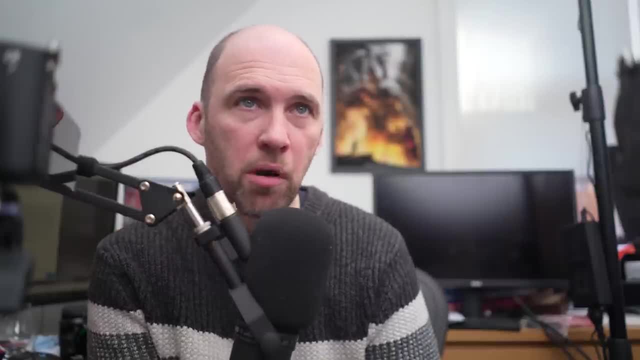 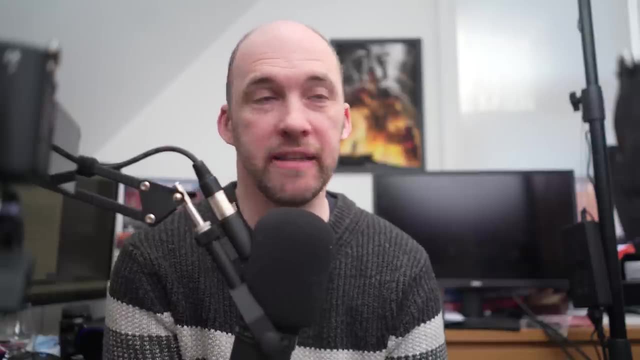 you want to come on the podcast and you'd be like sure, uh, i'm not a very big podcast, you know i've not got a huge one, i don't care, i just want to talk hobby, and there's going to be like one or two people that might be interested by what i've got to say and that that's one or two extra. 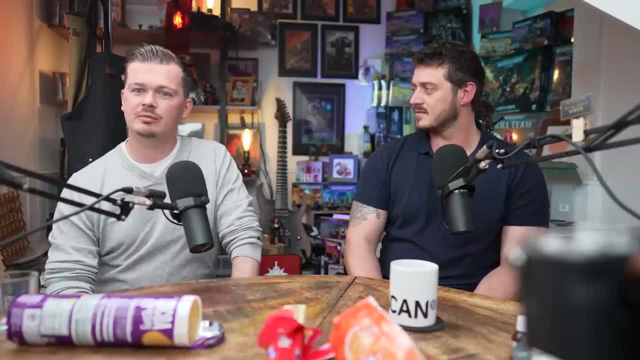 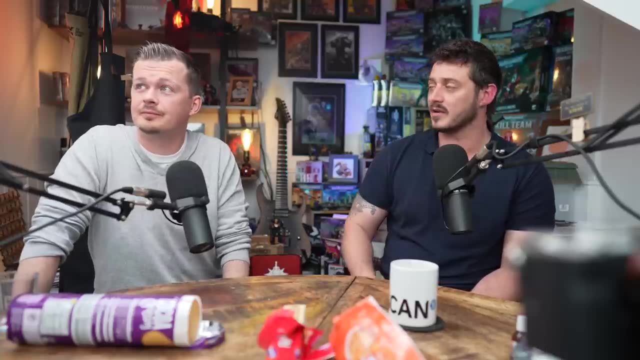 followers for the channel. i mean, the last couple of years we've gone to several conventions with nothing to sell. yeah then, hello, here we are. yeah, this is our name to do and yeah, yeah, a couple of people have come up to us and they're like: oh, i'm not the biggest painting. 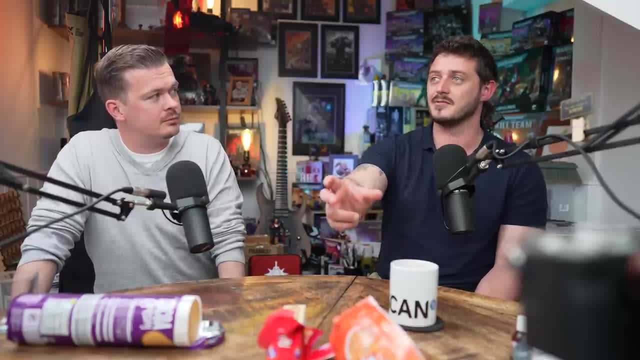 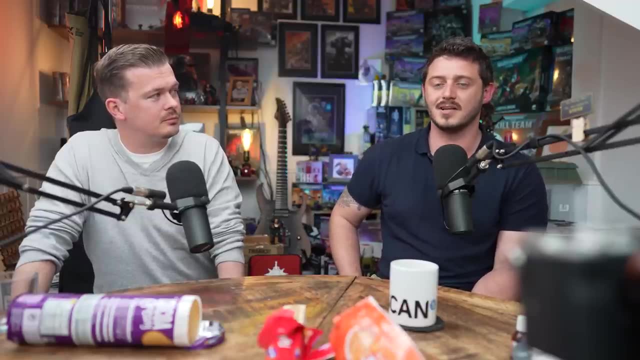 channel. i've literally just started. i'm like cool, have a model, yeah, have this, have this little tesla marine. oh really, i'm not that great, doesn't matter. there you go, yeah, go ahead, yeah, do what you can with it, like looking forward to it, tag us in it, let us know and then we'll tag you and we'll help. 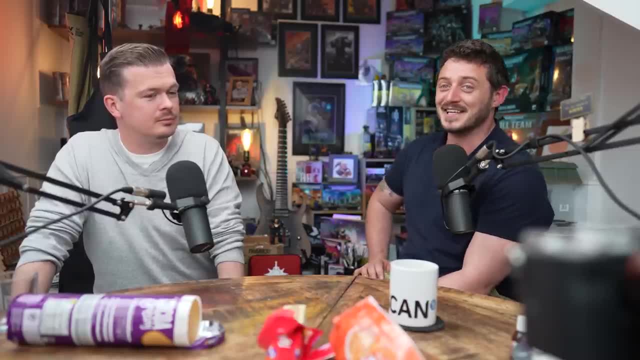 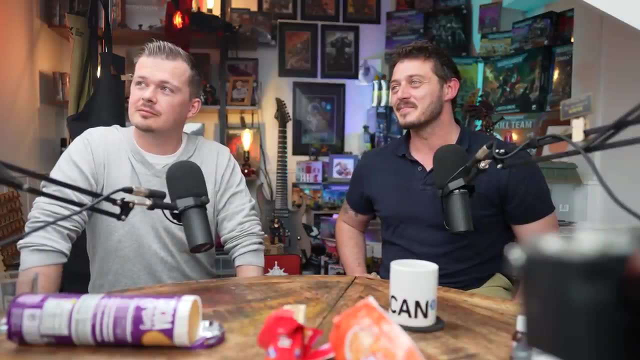 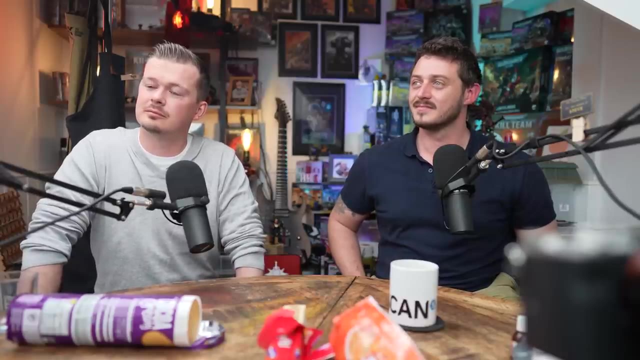 you as well and just, yeah, make friends, yeah, be nice general life. that's it really. yeah, i'd like, like, um, that's something i've always tried to do in my wedding business. now i think it's worked for me quite well. um, but say, having dave on the on the show, ms paints. 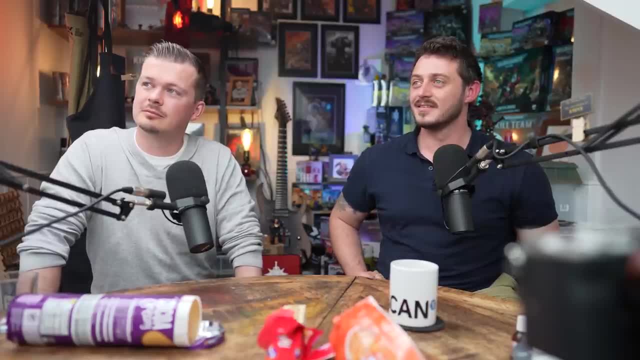 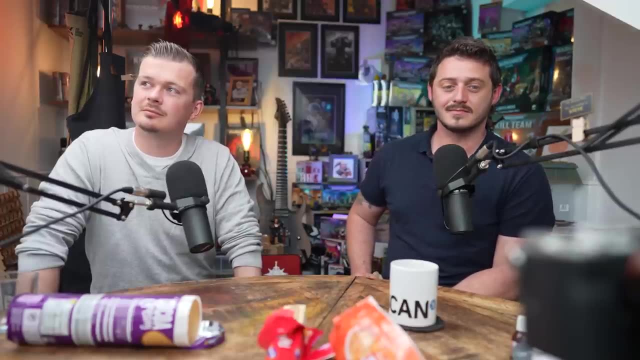 obviously put us in touch with you guys. um, wayland games got in touch with us, um, because they were like, oh yeah, cool, yeah, we saw dave was on there and we do some stuff with him and and just like, just just through chatting to dave and having him on the show and talking about miniatures and 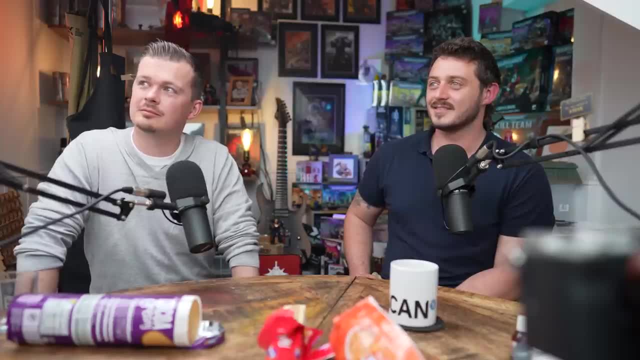 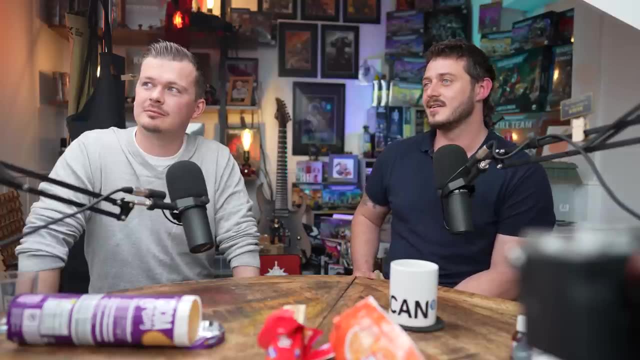 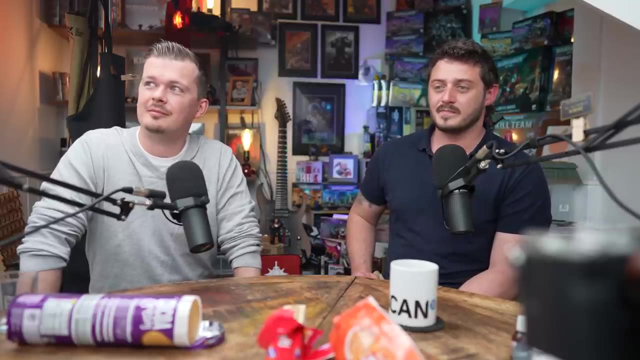 having a giggle. um has opened like so many doors for us. yeah, um, it like unintentionally, um, it's not, like i thought, oh, this is going to be a great business opportunity, but it, but it. it turned out that way. yeah, it's amazing. yeah, yeah, it's like you know. go going to. 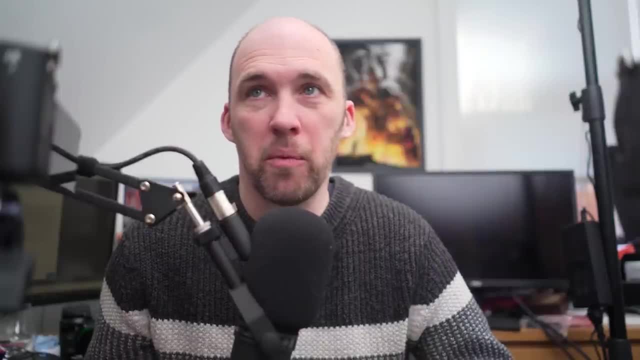 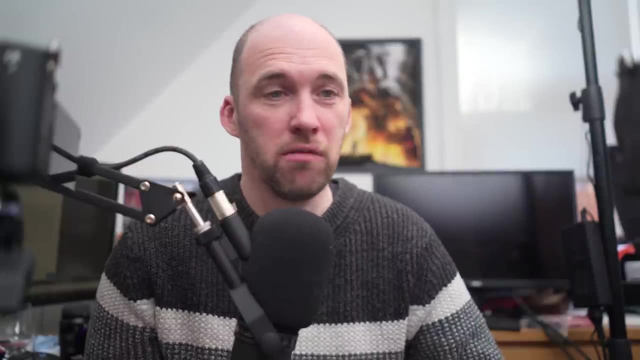 salute and chatting to people. um, you know, we've got a couple more people want to get on the channel. just by just saying hello, yeah, i say just be nice and saying hello and just, oh, fancy coming the channel. yeah, i'd love to come on. yeah, oh, i thought you'd say no, yeah, that's a walk week. yeah, we. 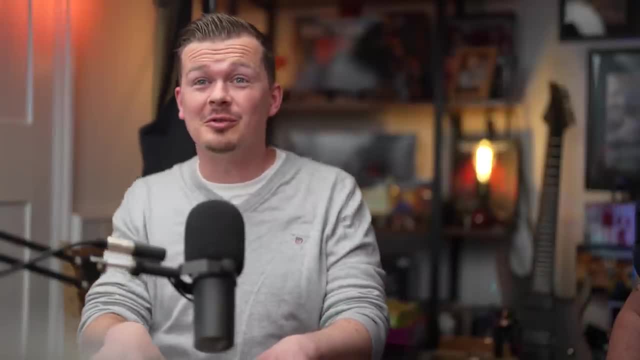 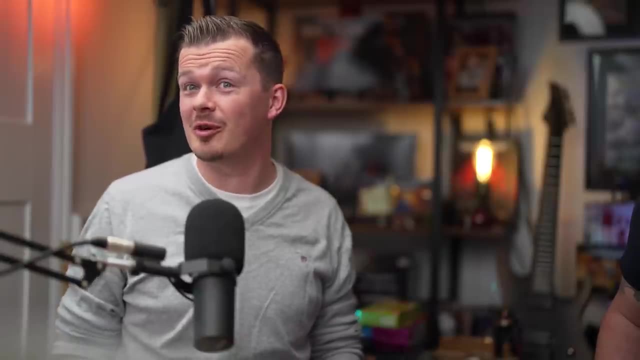 thought, um, yeah, i didn't think it would be a good idea to do that. yeah, i think it would be a good thing, you'd say, because obviously we saw davis on it. yeah, yeah, that's when i contacted you, but i hadn't contacted you before, because i mean, you're congratulating your channel's growing and 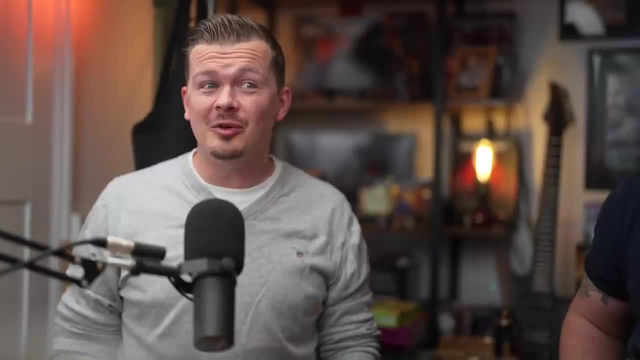 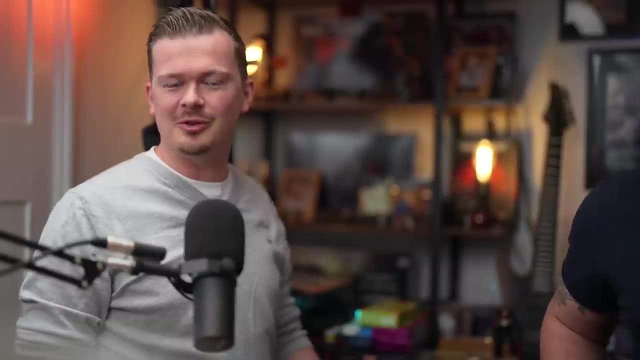 growing. yeah, enjoy, enjoy watching the videos. and we thought, you know, basically we're relatively unknown. this is yeah, yeah, well, we're completely unknown. yeah, yeah, um. so i thought, yeah, we just assume people are going to be like: yeah, that was good. yeah, you got an award, didn't you for uh. 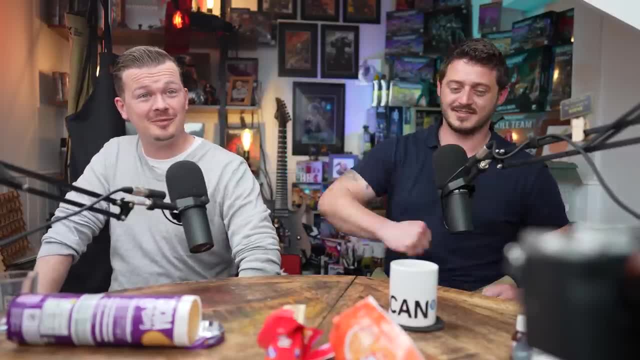 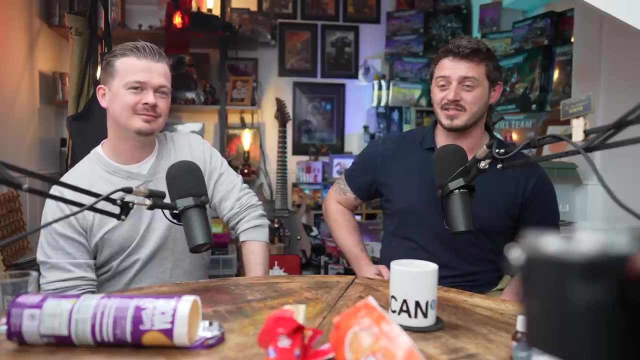 yeah, best participants, best participation game in show. nice, i love that little um. yeah, little awards. yeah, well, you had a nice display board and a nice little uh. well, oh, it's in my cabinet board. yeah, little little things in my cabinet. yeah, brilliant, fantastic yeah. and then 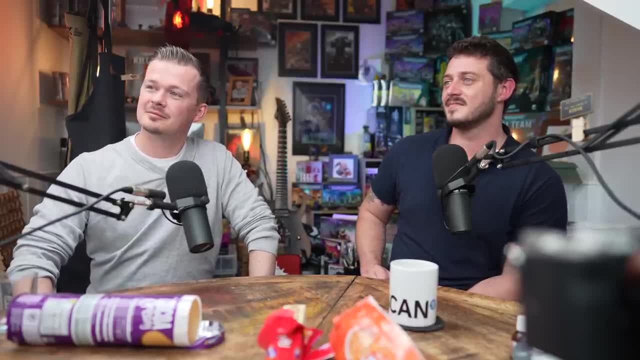 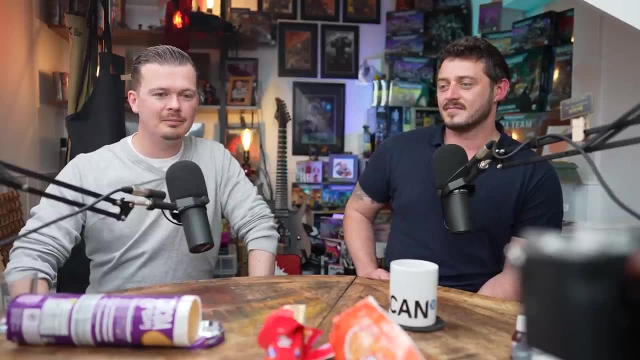 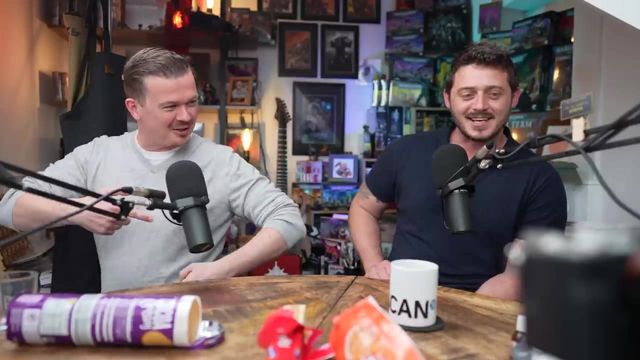 the last question, uh, that i think i'll get time to read out today from our patrons, is: if you were given one sentence to persuade me to play war on terror, what would you say? um, by war on terror, i'll kill this cat. yep, that's the one, that's. that's, that's the one, um. 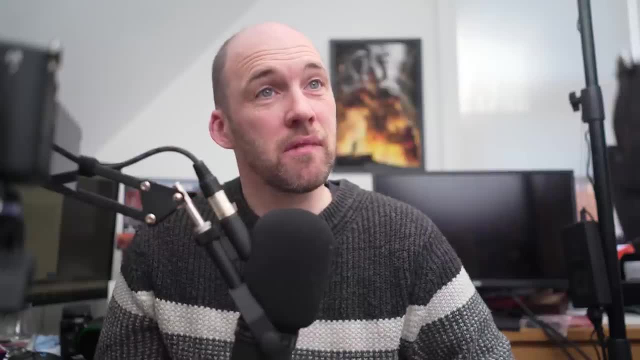 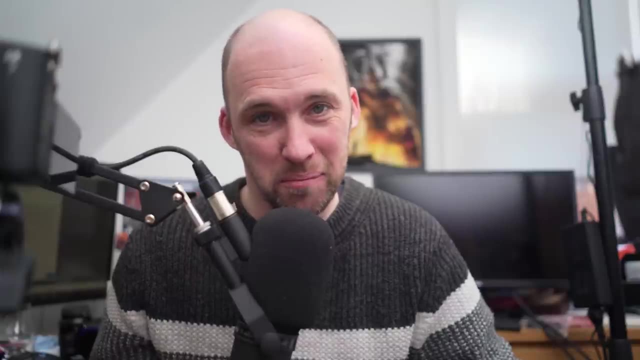 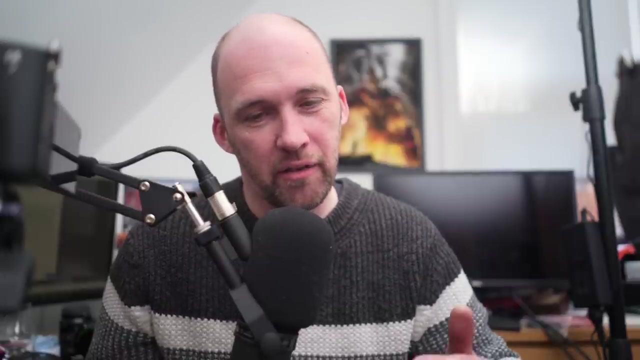 and then, yeah, i've got one. if people, if they're not cat people, oh well, it's changing. yeah, i was gonna say: if you, if you like skirmishes, you like sci-fi, you like painting toy soldiers, uh, and you like x-com, yeah, it's all of them. uh, no, i think, um, if it was me, because the way i've not played. 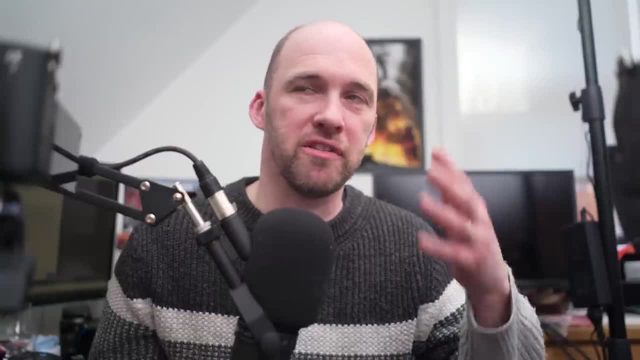 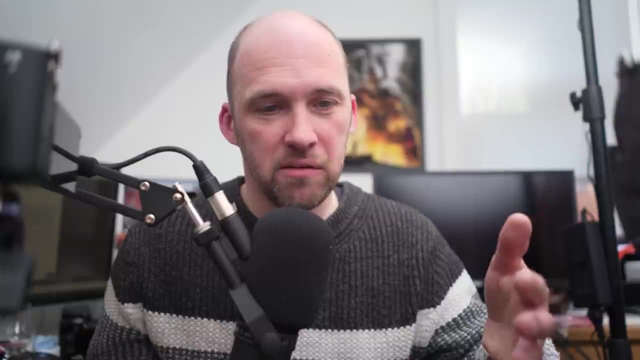 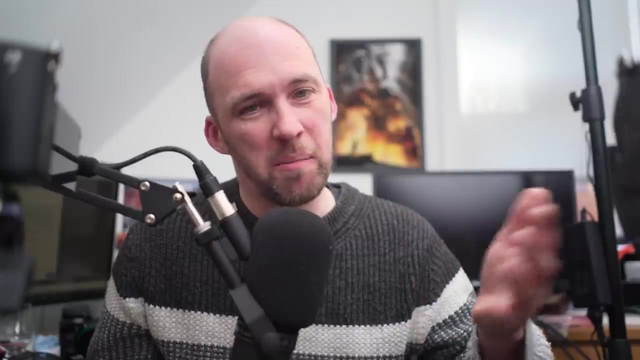 i've read through the rules, skim through. i have to play several times for it to connect. that's the way my brain works, but i think it's super um well laid out. it's um easy to get to grips with. um, you don't have to go mad, paint lots of stuff um, and you can make. 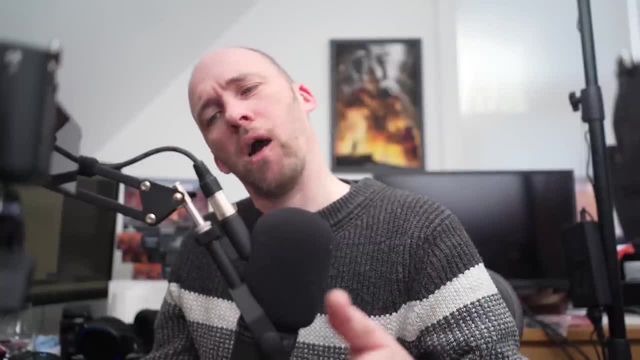 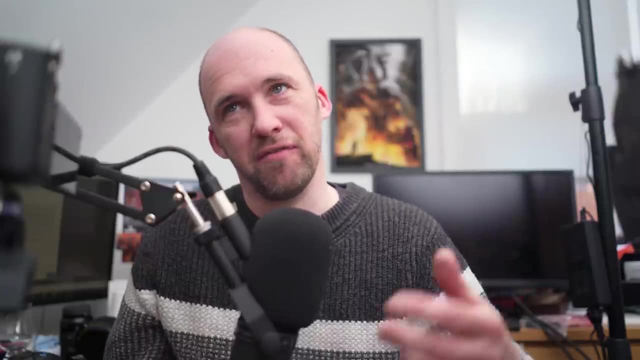 it your own. you can do anything you want with it, really it's. it's kind of like i want to say generic sci-fi, because you've got your own law and background, but you could do so much more with it and i've got a figure to give you. i've not used it, i've used a workshop human head on it, so it's. 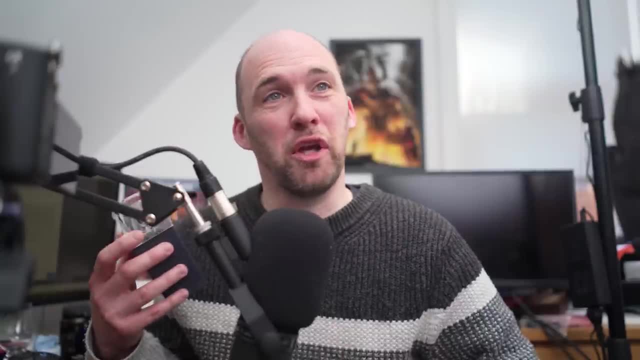 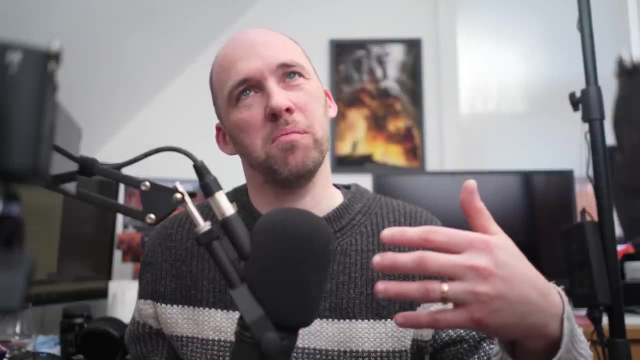 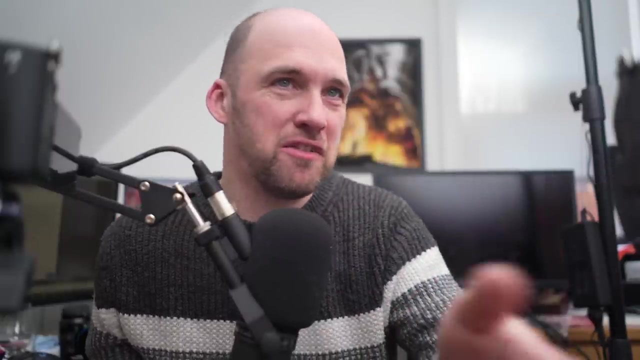 very customizable as well. uh, so yeah, you can literally do what you want with, with the- i suppose it's not the rule system, but you can. you can play out what you want. yeah, the movies you want to play out. you know we've touched on like: oh, it's like destiny, oh, it's a bit like, you know, gears of war. 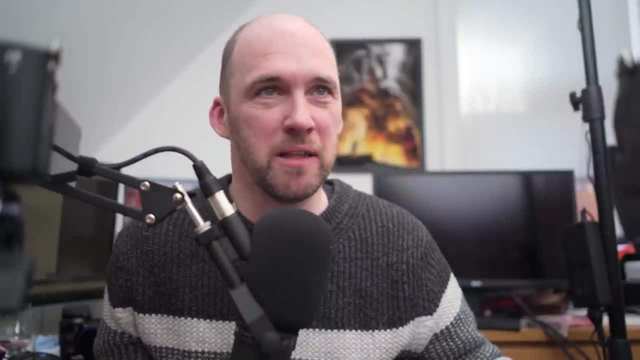 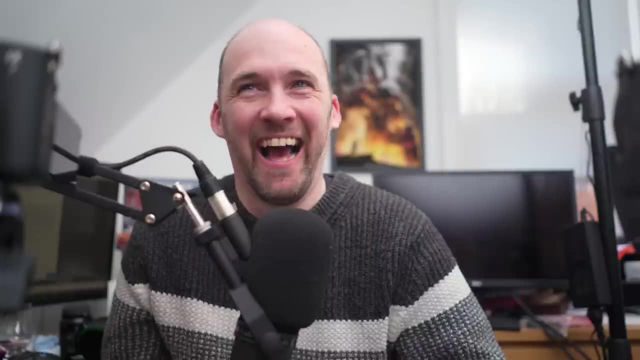 if you, if you really want to play gears one, there's no game out there. you could use this as a mechanic and set up the terrain the right way and absolutely, it's got so much legs, so much. uh, expanse, you could do expanse. yeah, what i'd say is: um, due to the scalability of the game, it's super cheap. 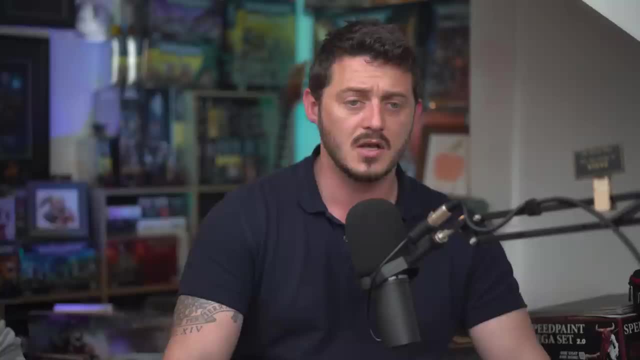 if you don't like it. great. if you like the rules, but you don't like the play style of the force, buy another couple of models and see how you play. so it's it's dirt cheap to get into and it's super easy to learn like extremely difficult to master. yeah, and that's, that's what. 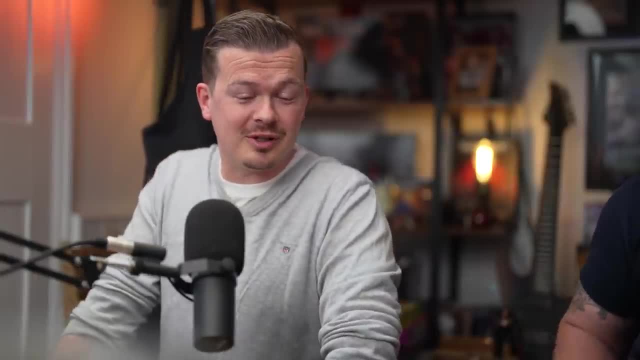 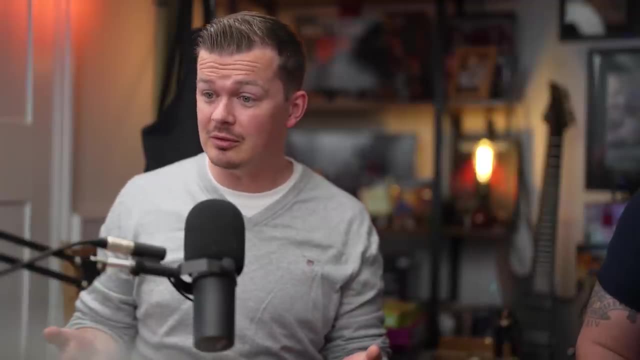 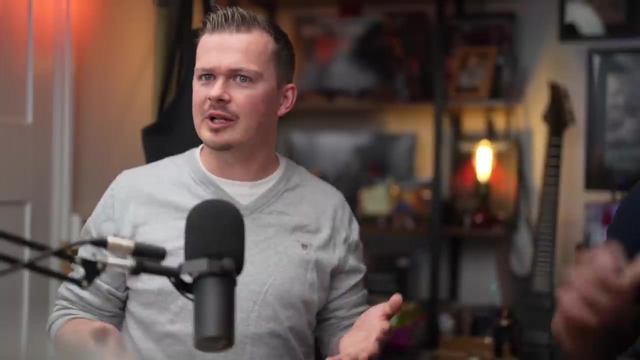 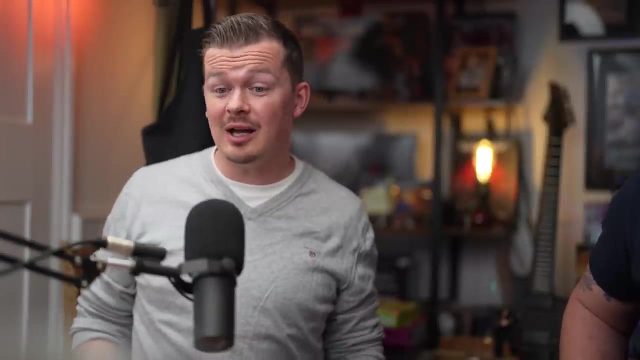 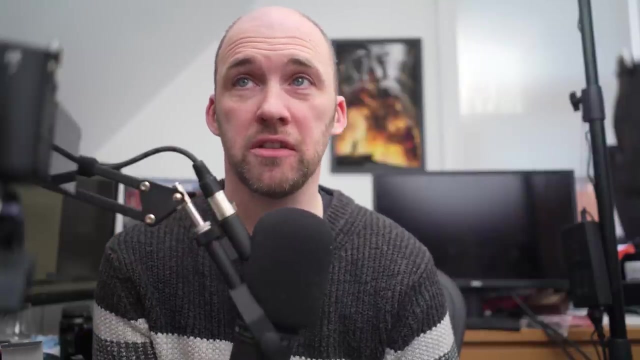 we wanted and i, i suppose i'd throw my two cents in. i i would say, first and foremost, the game is fun. yes, yeah, it's crazy to be fun. from my point of view, who that doesn't come from? like a solid character, set up and go. 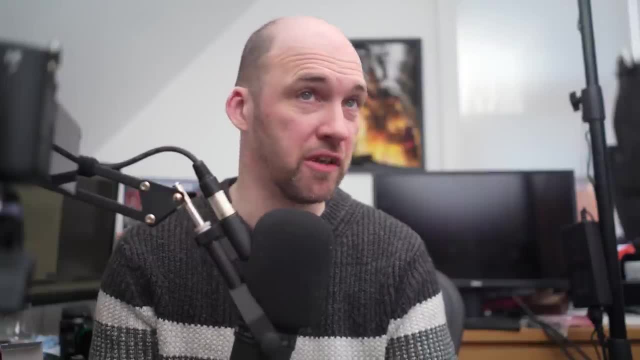 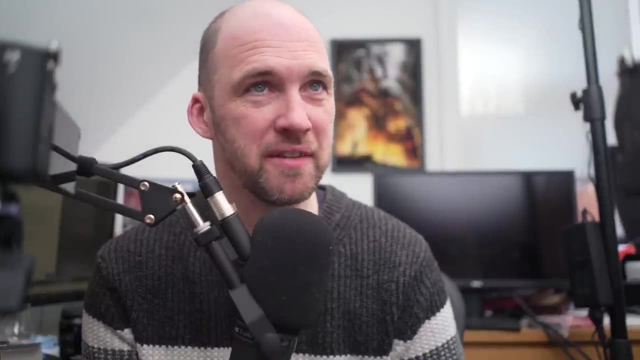 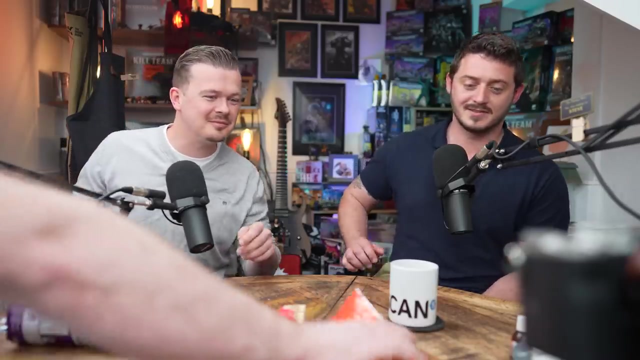 with one of them coming in, so you just have toais. it didn't just happen to happen to you because i was way short, painted him in the colors of the painting phase, so he's not a faction that exists in your. we're gonna call him Steve because for some reason the 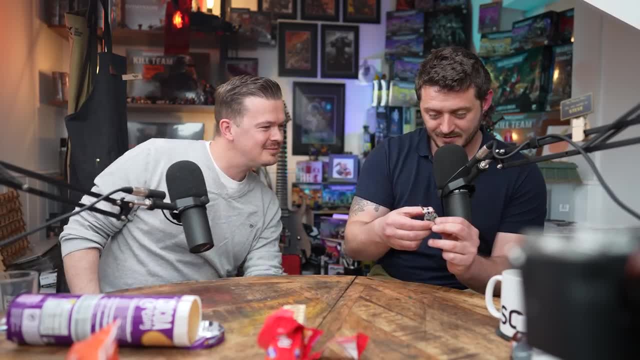 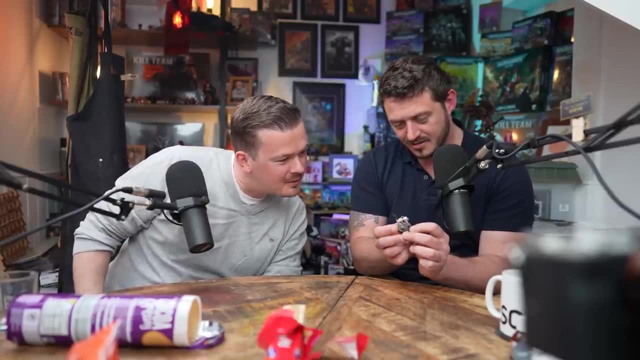 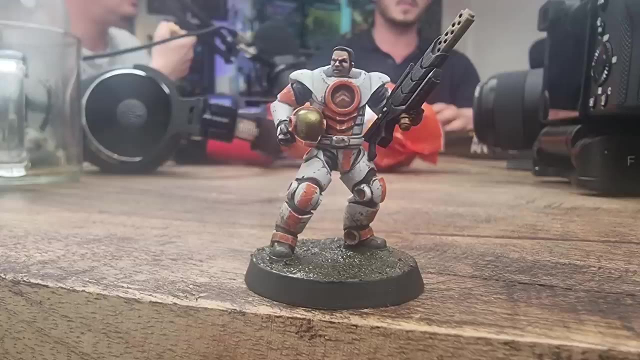 channel, we keep referring to ourselves, as Steve say: yeah, I've got my white armor. I've not taken a photo of him yet, so probably yeah, but yeah, so I just used a human head. a human head, oh, don't worry, he's there for you guys, he's pretty well. 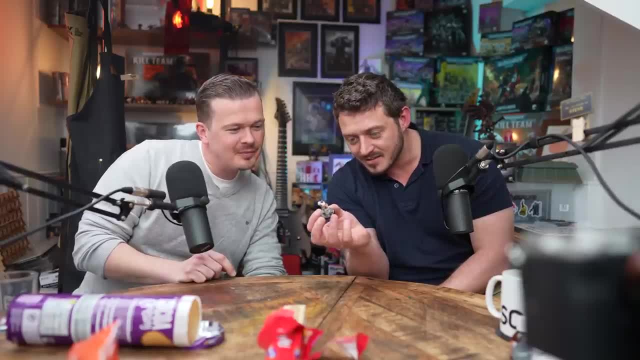 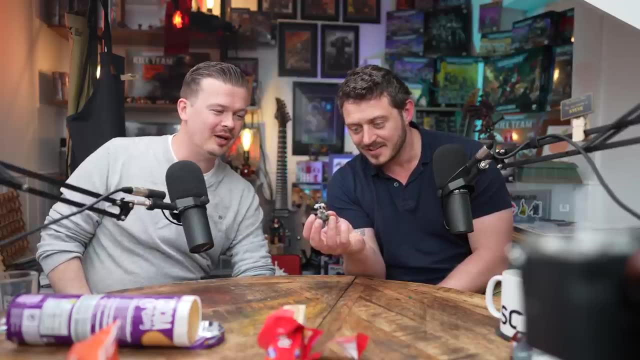 glued. but yeah, he's yours, you can have him. I love how you do the, the battle scars and the weather, because the ones you'd posted on it's just a bit of sponge way beyond. I know you say like it's an easy thing and then I try and it's like 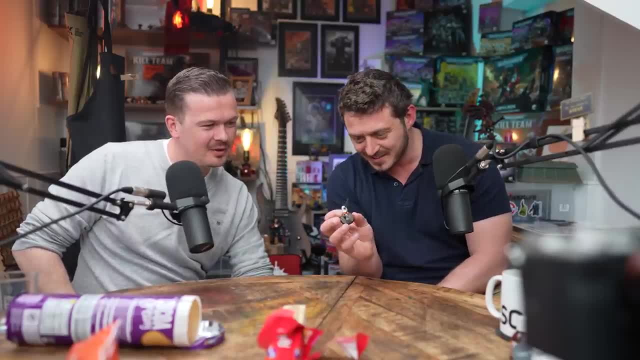 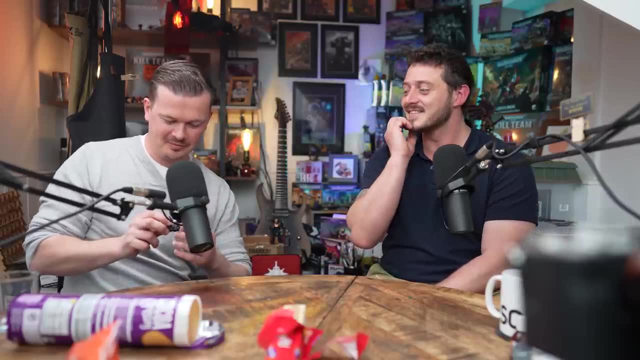 get out of it with a bit of sponge. yeah, well, I think, going back to, I guess, one of the going full circle to talk when we're talking about the miniatures at start, yeah, something I love about these, like I say, is they're not, I think I see. 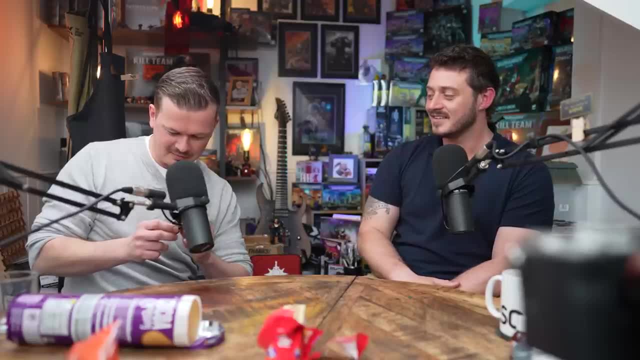 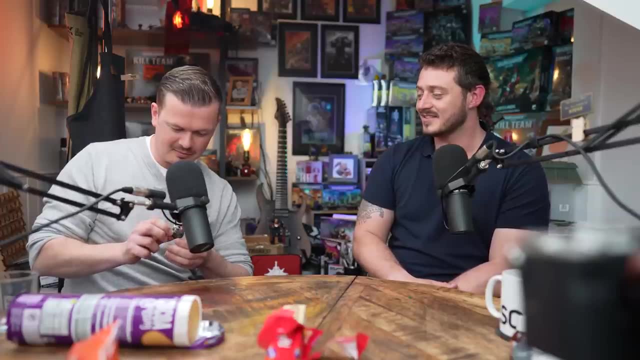 lots of 3d companies and that they're kind of like you know, each technique is, I think, really well. I don't have much detail on it, you know, because I think it's just way too much detail on the miniatures where I think I think this and similar to to like a Space. 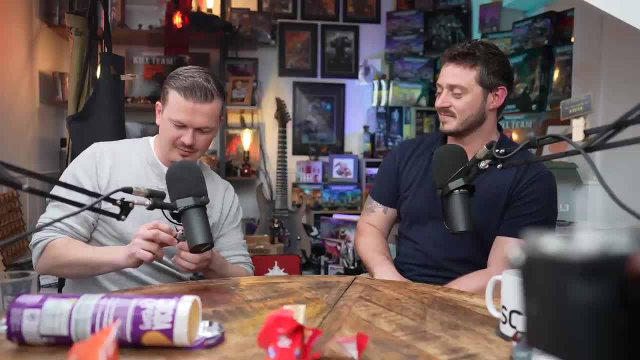 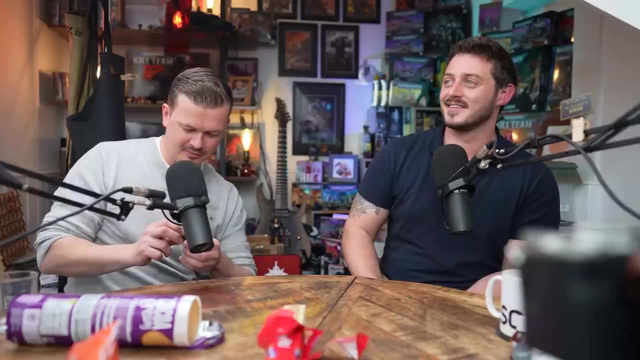 Marine, you have your big panels that you can, yeah, put markings on you. still, if you can put weathering on yourself, you could do loads of glazing on it if you wanted to like. you really have a room on the miniature to give it. it's all your. 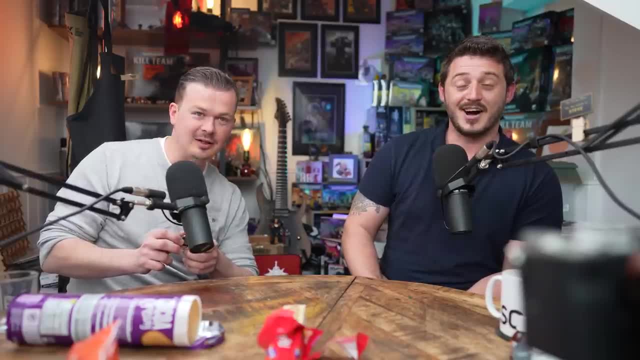 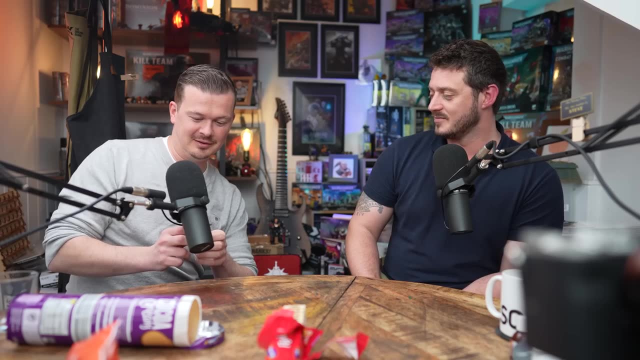 flavor, yes, which I don't offer. I don't see that often from other companies. so I think what you guys are done is it's amazing. it says TPP at the back. oh, I've noticed the painting phase be terran planter. uh, planetary protection, it could be whatever. it could be whatever you want to call. 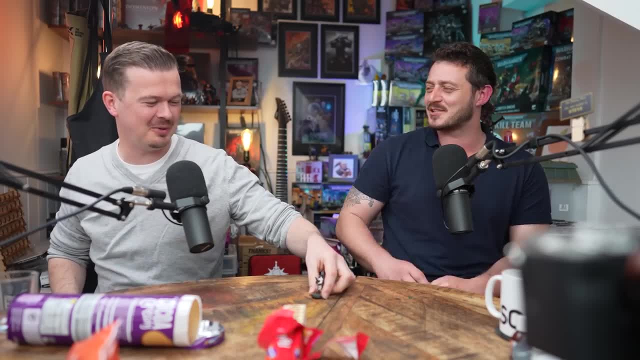 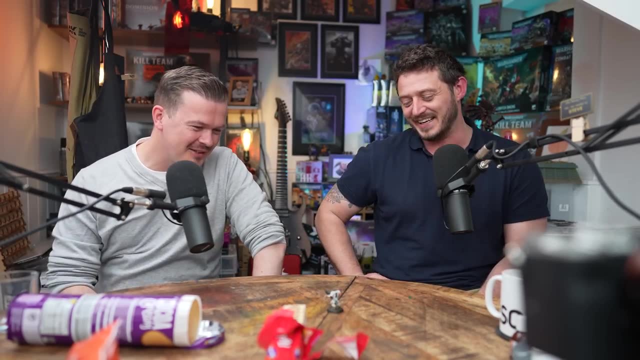 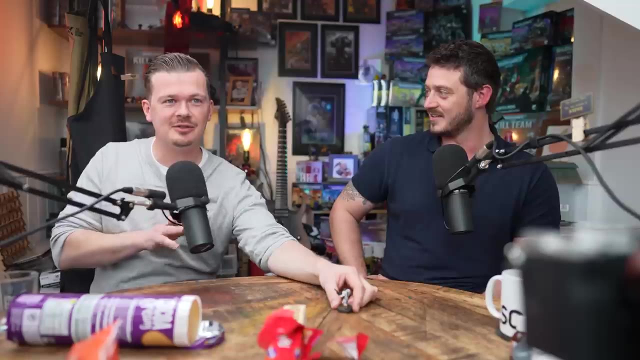 it: toilet paper police, the toilet paper police. that's the first one i came up with. oh, that would be. yeah, yeah, that guy's called charming. uh, captain charming, i'm steve, steve charming. what i like about that is that's the first time i've seen one of our models that hasn't got the 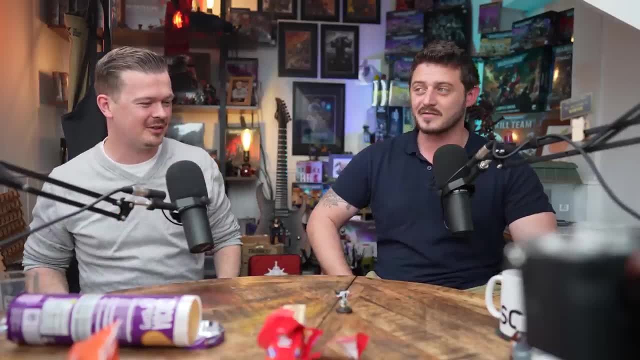 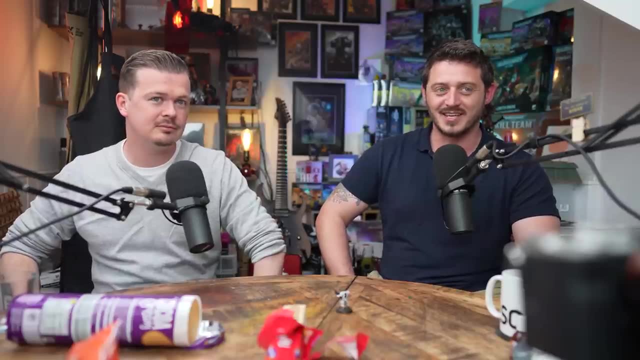 helmet actually. no, that's that's true. that is weird. yeah, so because obviously learning to model and humans being very difficult, as i've said, yeah, faces, just i'm not painting faces. yeah, i'm modeling them. i i haven't even tried touching modeling a face, because that's an alien face. 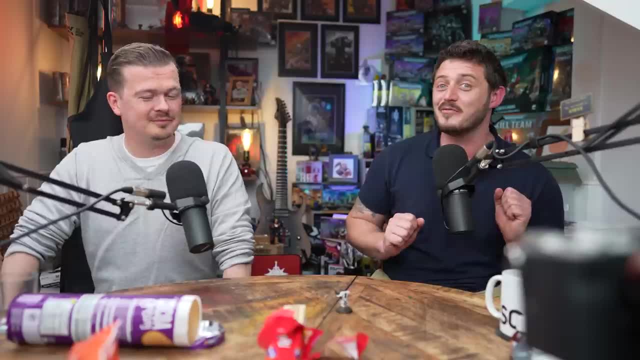 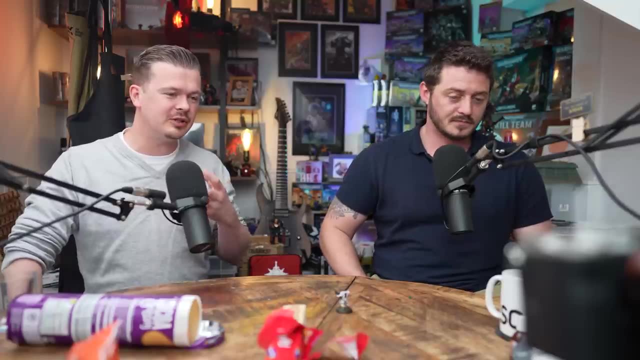 bring it, bring an alien face. you don't know what you're looking at. yes, you don't know if it's wrong. yeah, that's not. that's not even particularly why we did it. i liked, i like the look of a faceless army. yeah, yeah, yeah, yeah, because even with a helmet, because everything else kind of has. 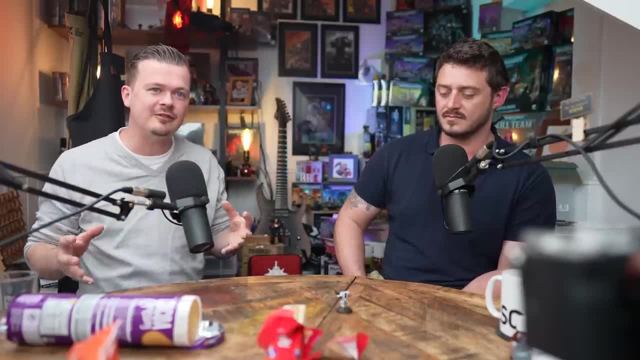 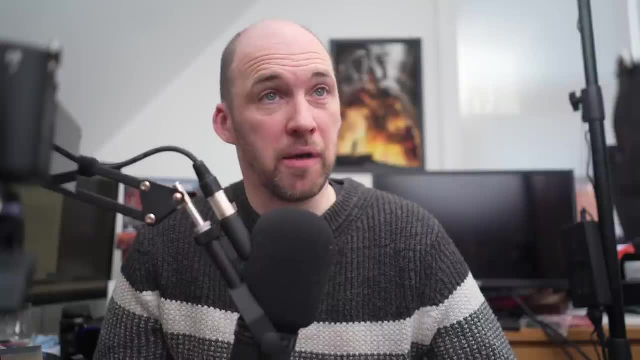 space marines. to an extent, you still have the eyes still, yeah, you know, yeah, everything has a face, whereas this is just so. there's something that, when i've looked at the stuff you painted on your uh, demo, uh, the thing that instantly clicked with me was even the humans looked a bit. 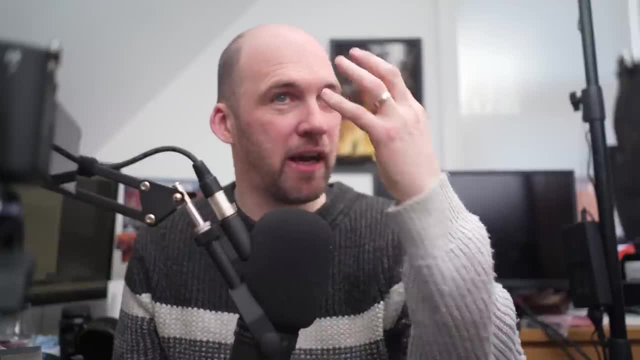 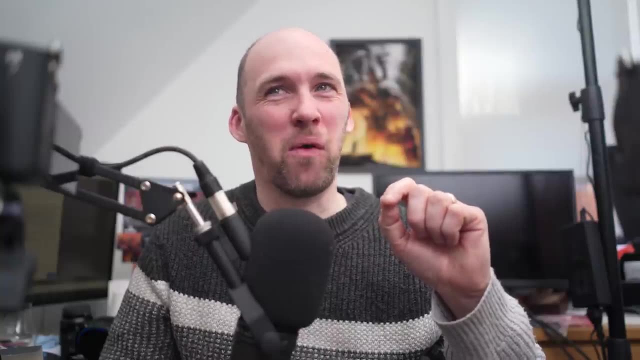 alien in the way, because they had like the black jet, black glossy helmets and it reminded me of: uh, is it a widgetty grub? yep, and i was just like looking at: good, yeah, they look a bit freaky, weird, shiny. yeah, that's cool. yeah, i was just like looking at going, oh, are they alien all. 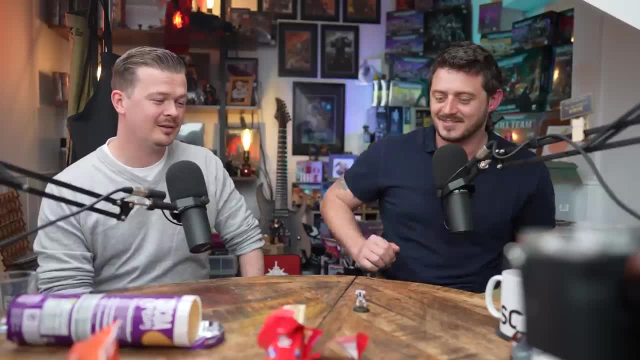 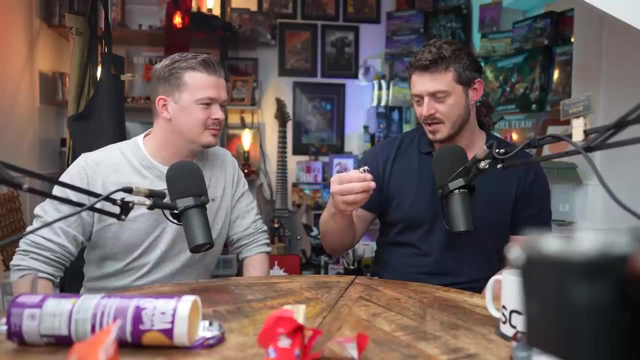 right. are they human, i don't know. aliens in disguise? yeah, yeah, but um, yeah, i used the reloading guy so it looked like his horn. yeah, no, that's cool. no, that's really cool, that's cool. he is missing a mag from his rifle, but it's just so. he's just lost. he can hold his helmet. he's just lost it. 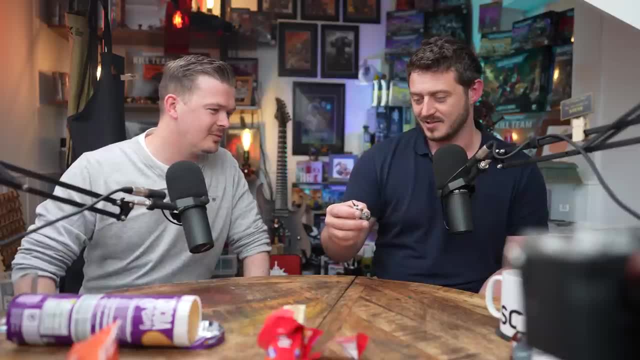 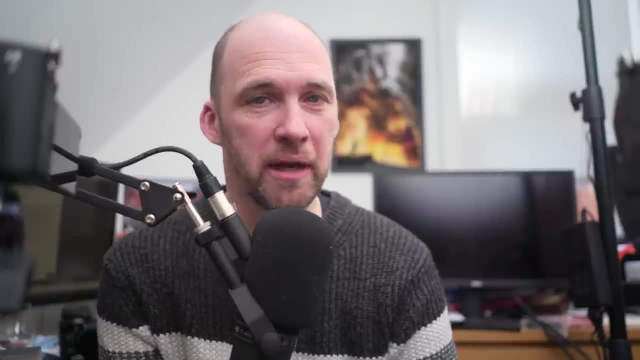 no one will notice, no one will know. no, i don't want to do that. that's all using ak paints. there, pat as well. he's nothing but ak, because they're uh getting used to like a new range of paints that we're playing around with and they've got some really nice colors and tones and finishes. 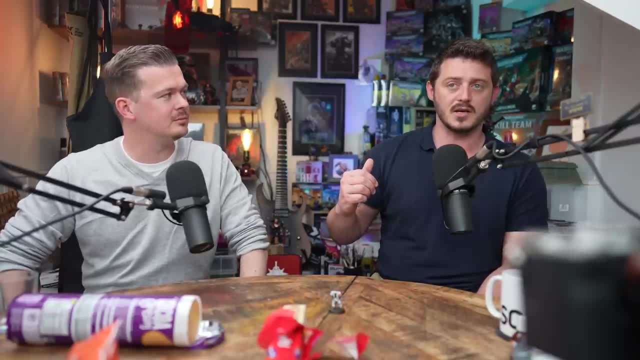 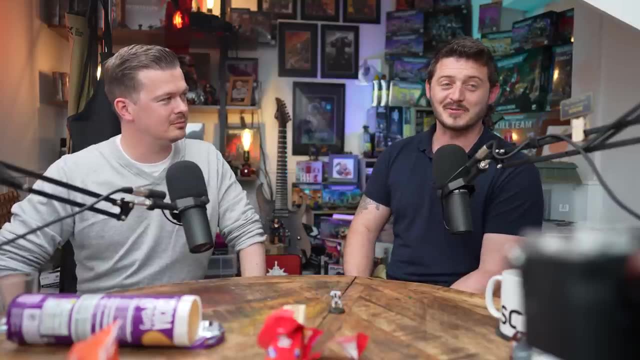 turbo dorks. nostalgia paints. i picked up last year- and i literally have just managed to start using it- a proper codex gray. oh, i've got a bolt gun metal off them. i've got a codex gray off them and i was like those two colors were everything. yeah, yeah. 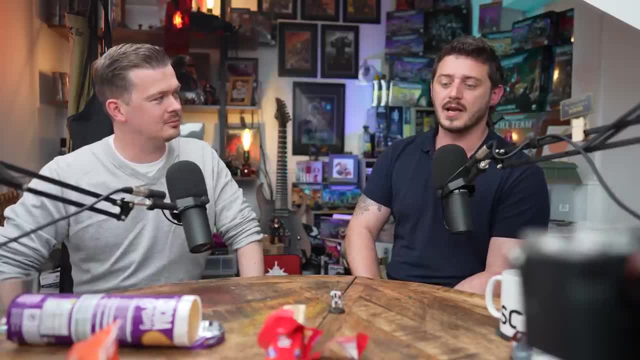 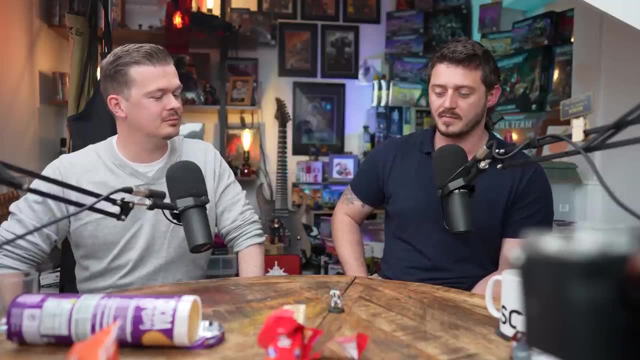 and uh, i'll tell you what it layered. the codex gray layered one of these so beautifully and finely. i can't recommend it enough. it's a beautiful paint range. um, it's really nice just to see the color of codex gray. again, if you want to highlight any black, there's always a. 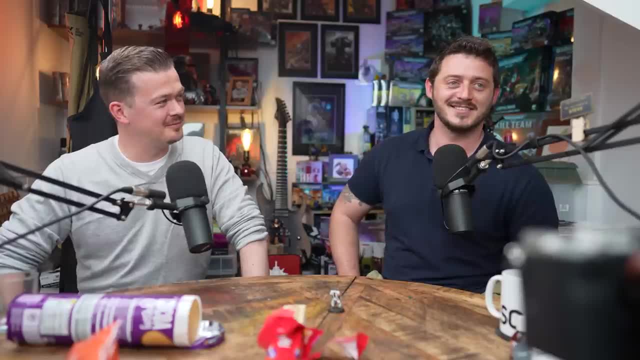 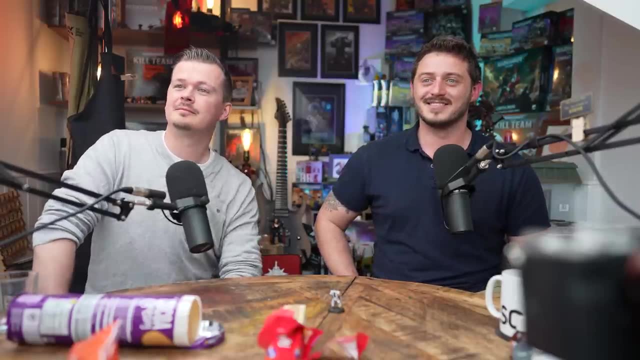 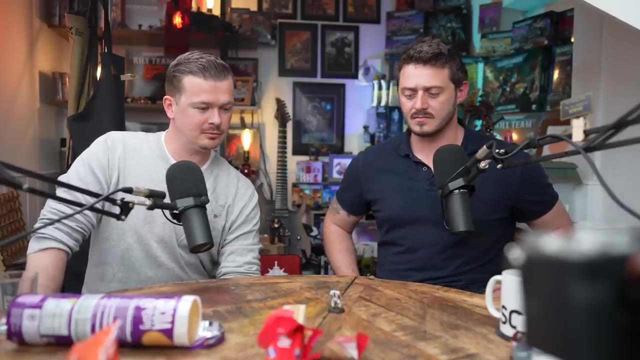 codex gray dry brush. it was perfect, like yeah. so i was like i'm getting that amazing. yeah, i can see some of my cameras, uh, giving me some heat warnings now, so, no worries, explosion. yeah, we might have to wrap up, yeah. well, uh, we'll put a picture. i'll try and get one posted on on me, me grams as well. just get pat on myself, just do. 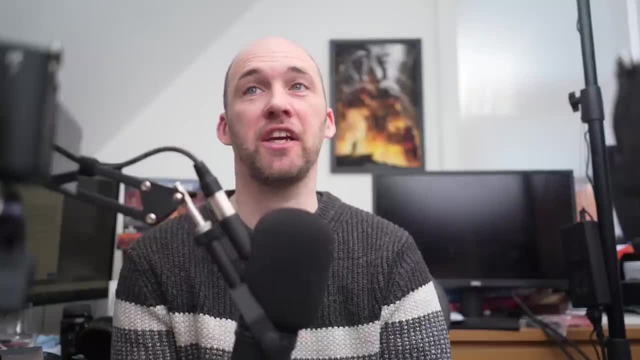 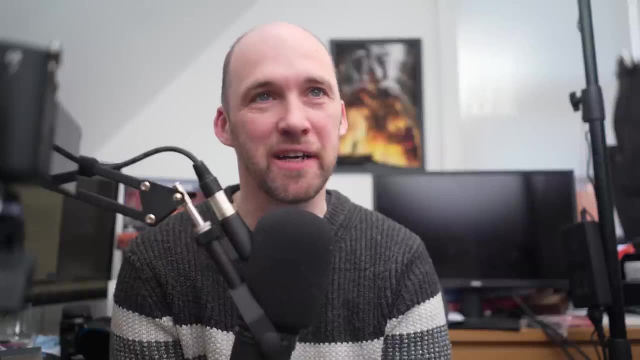 one with me before we go, but that's yours to take. uh, thank you so much for coming on the show. thank you for having us. yeah, it's today, because today is out. this video is out. your kickstarter is live. it's made the first. it is may 1st today. 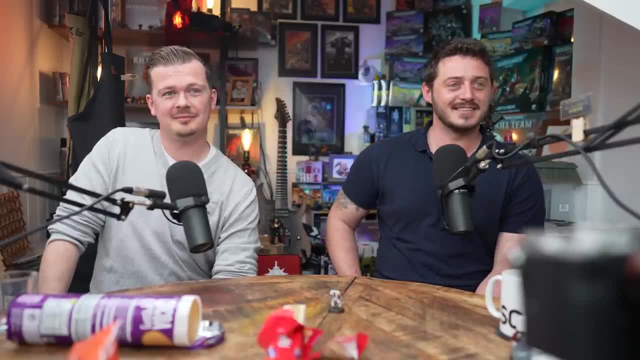 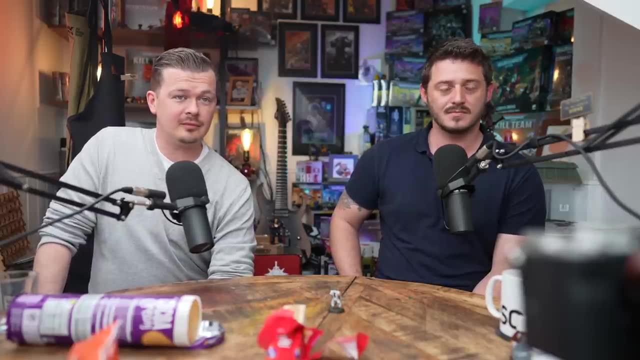 it is i expect you to be. you know, selling out of everything that you'd ever expected to sell out of you've made a million. i want it to be that way, uh, touching wood, hoping that happens. um, and i can't wait for the future, personally, because, yeah, uh, more games, expansions, different game styles. 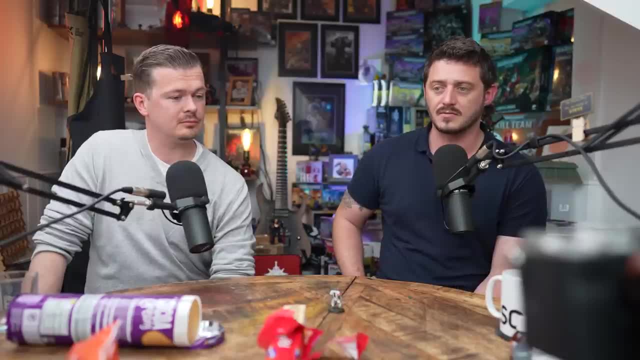 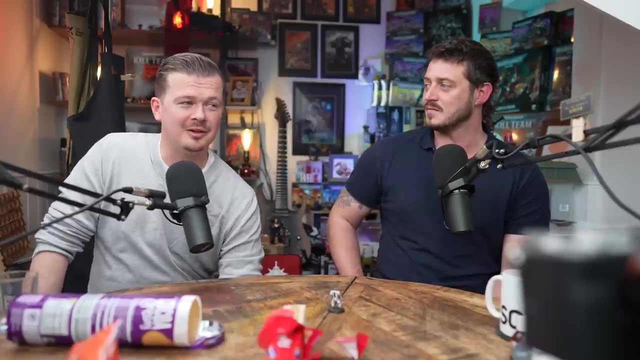 well, the kickstarter's coming out with two added added game styles: mass objective and wakazinan, which changed the game entirely but all play within the same rule set. oh, fantastic, awesome. i know we're wrapping up. i'll just touch on that because it's really one of those. 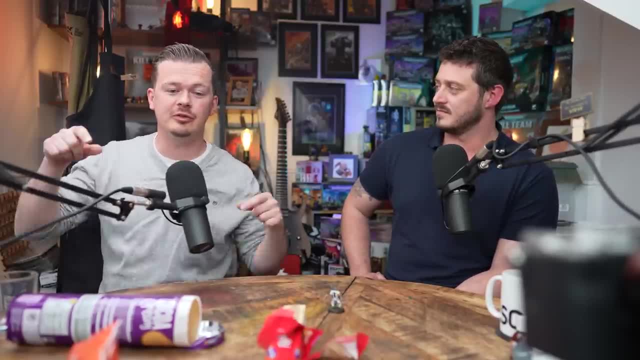 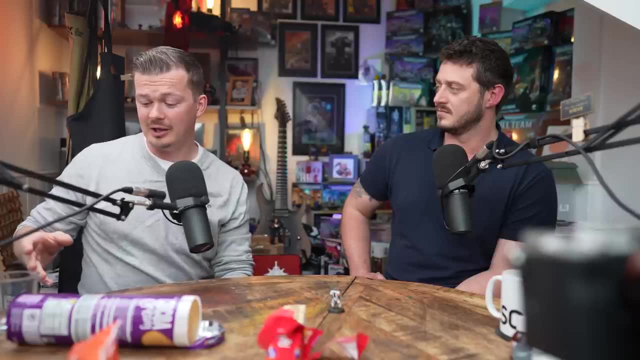 yeah, the wackazino. it's like a whack-a-mole from a fairground. so you, you set um markers across the board and then this comes with like an additional 56 miniatures: yeah, oh, wow, um. and then, through card draws and dice, it tells you what creatures, and how many of them, pop up at various 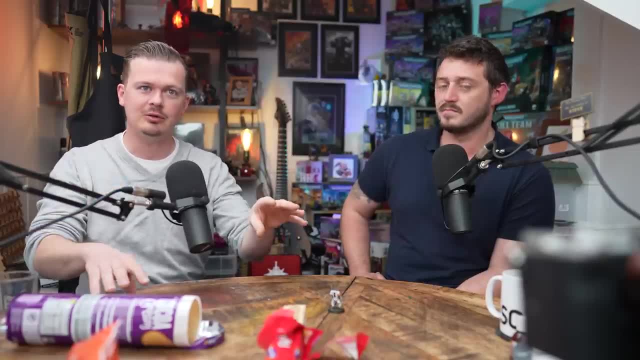 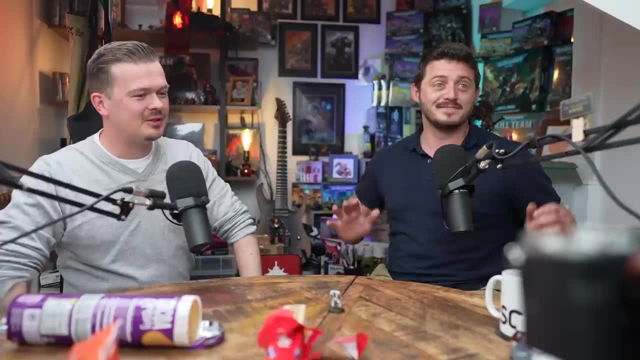 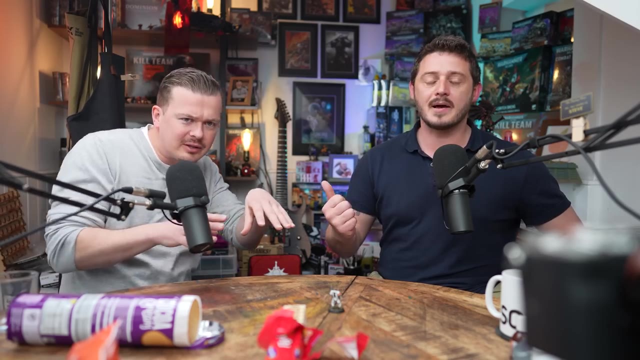 points. uh, as well as trying to kill your enemy, you're also trying to kill these score points, and then they only last a turn it's. yeah, you didn't whack them. yeah, it's amazing, but yeah, they completely changed, say, because i'm quite, i stay back. he's a camper and then yeah, he's.